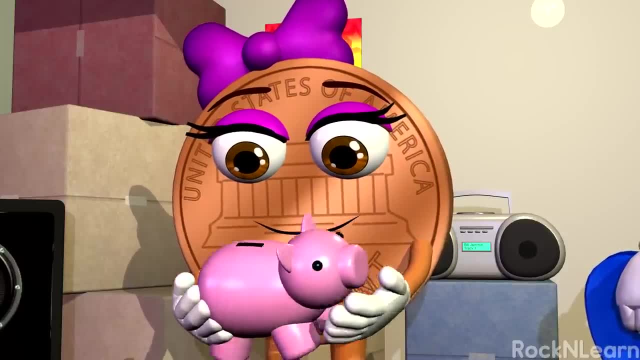 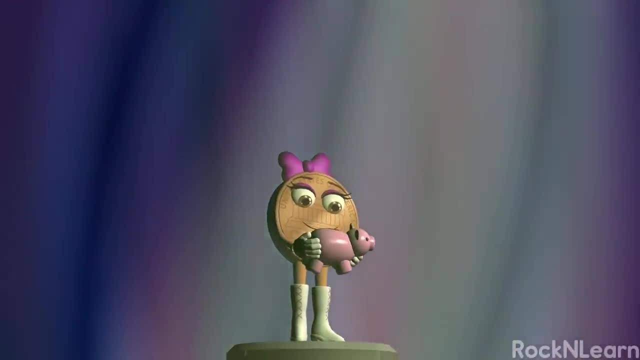 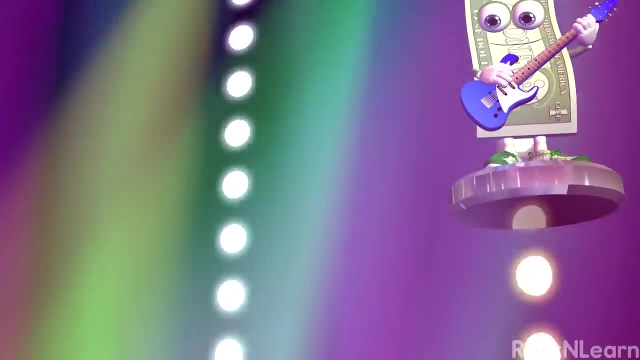 I bet there are all kinds of coins inside my piggy bank. I can't wait to see what they look like. Let's sing a song to learn about the different coins. Here we go, Here we go, Here we go. Let's see who is the Chaos. 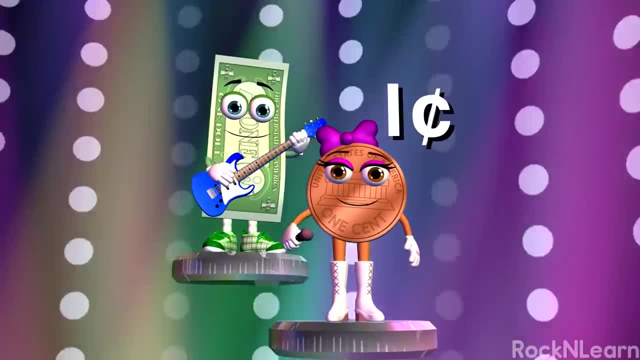 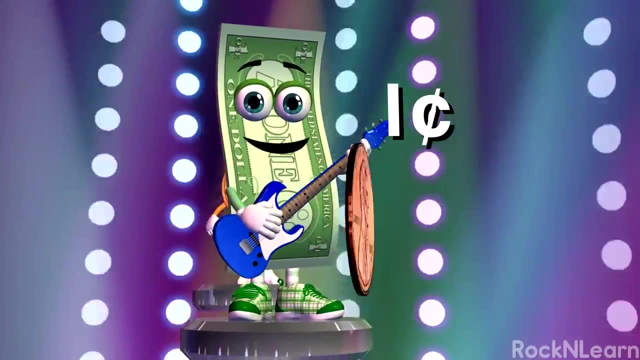 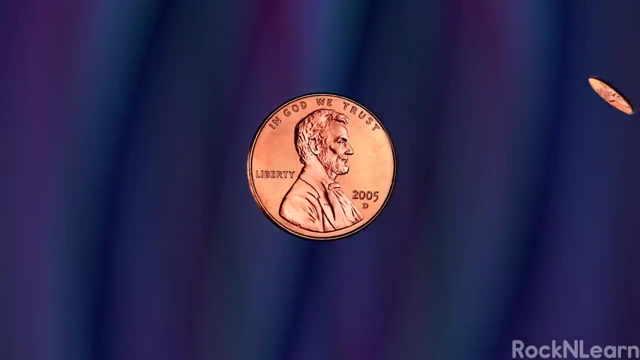 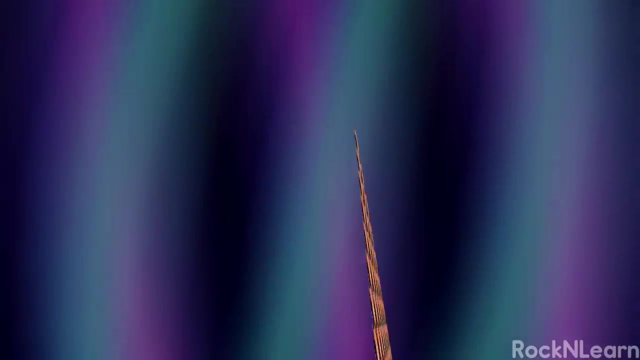 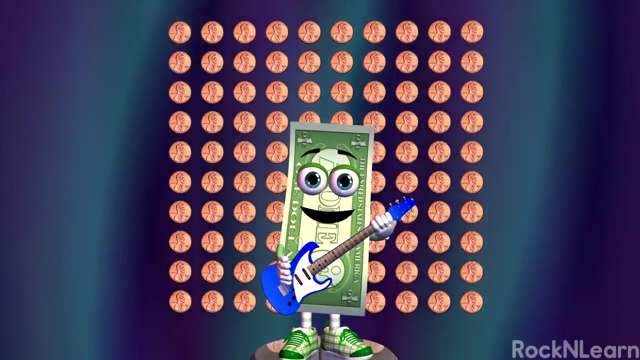 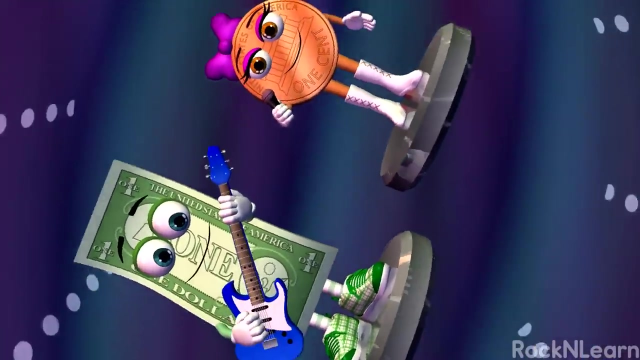 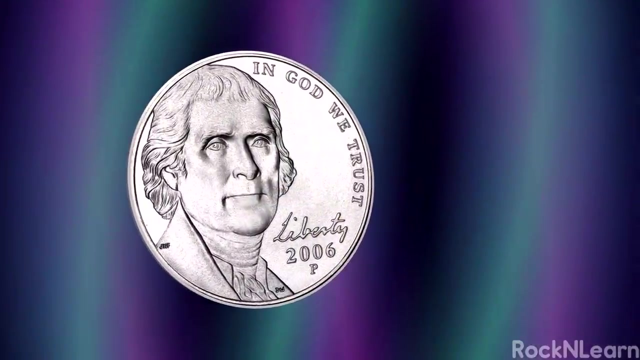 Yes, Yes, The coin that's worth one cent- That's the smallest amount- Is the copper colored penny, And each penny gets one count. Abraham Lincoln is on the front of the penny. One hundred make a dollar. Wow, that's so many. The coin called a nickel is worth five cents. 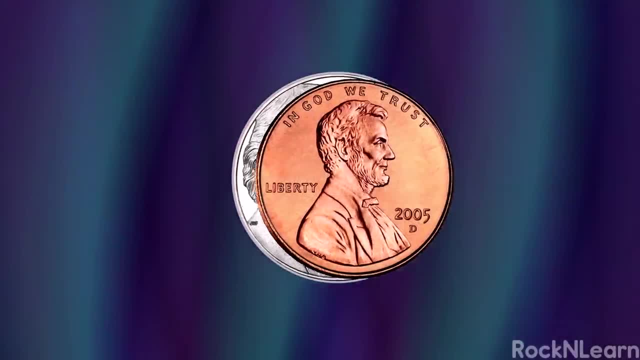 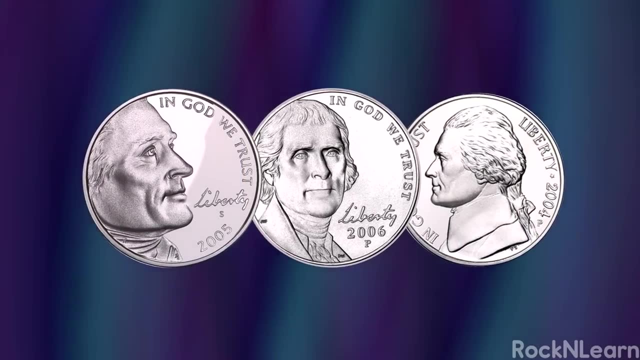 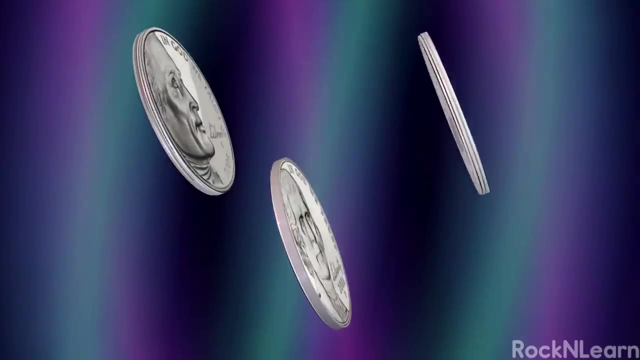 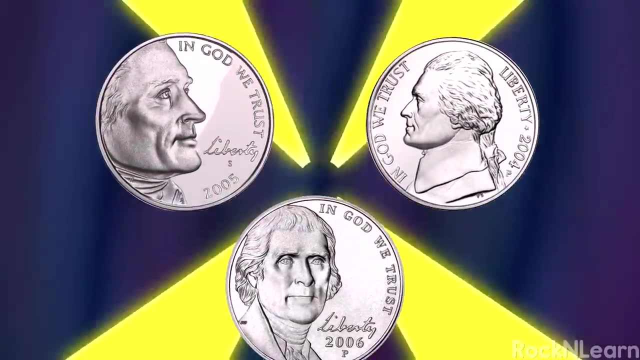 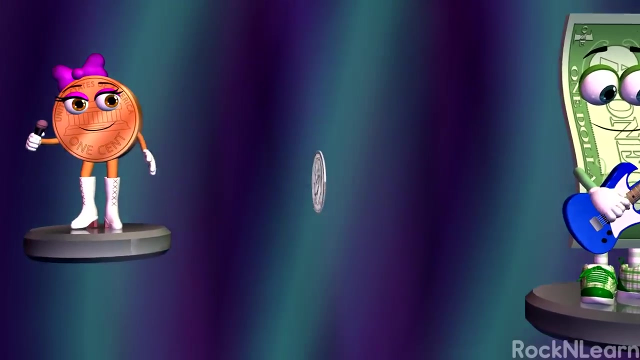 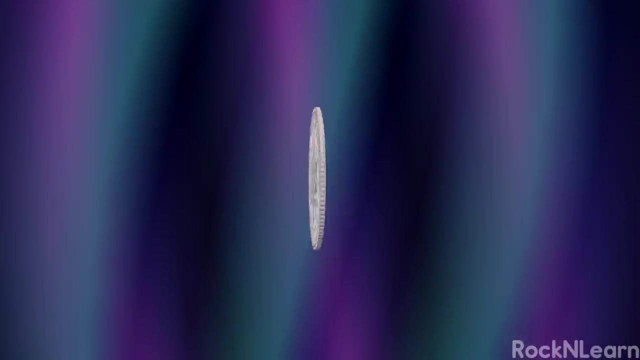 It's bigger than a penny, Now that makes sense. On the front of a nickel is Thomas Jefferson. The Declaration of Independence draftsperson. The Declaration of Independence draftsperson. The Declaration of Independence draftsperson. The smallest coin we have is the thin little dime. 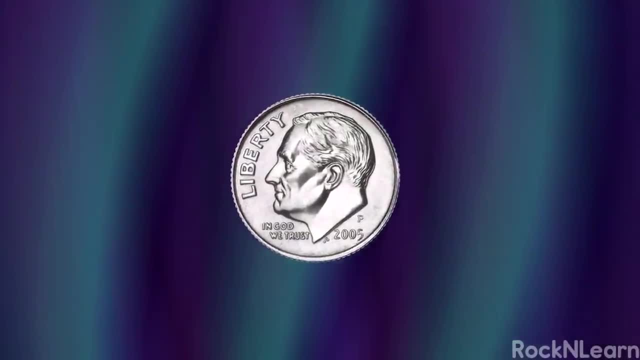 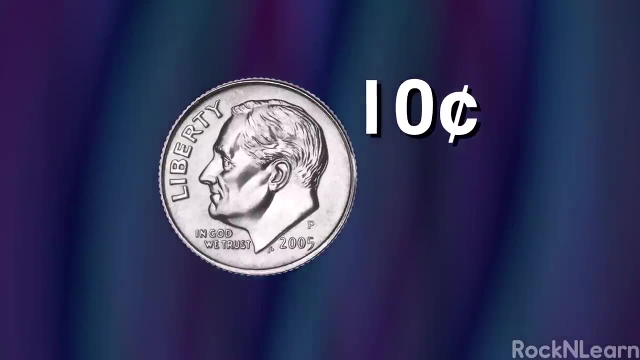 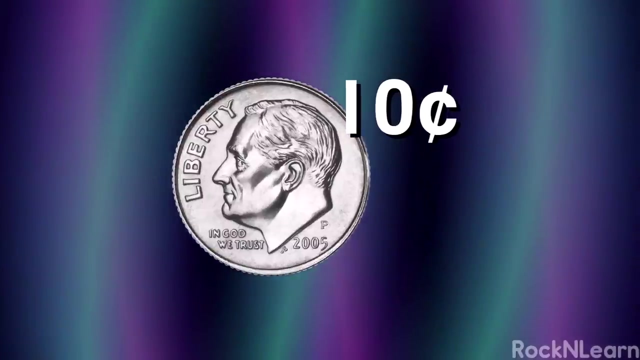 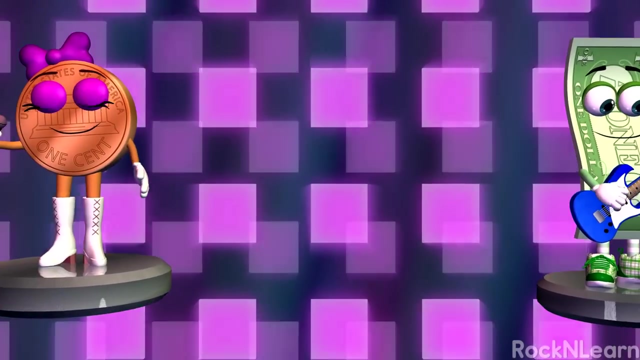 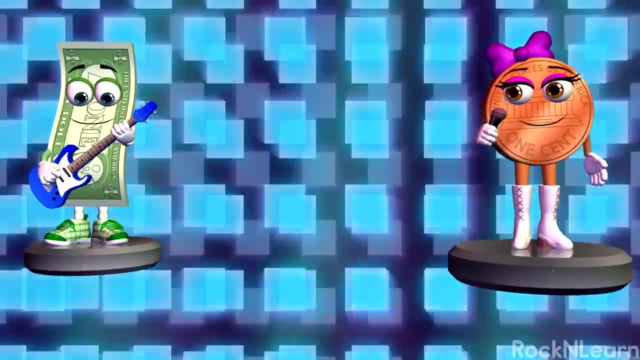 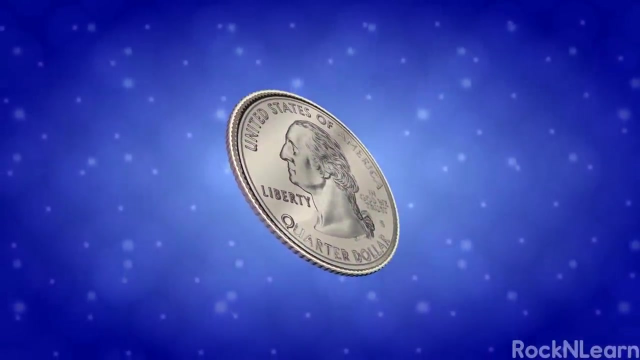 With Franklin D Roosevelt on the front at this time. Ten cents is the worth of the dime. It's easy to remember as we sing this rhyme. It's easy to remember as we sing this rhyme: This coin is a quarter. The edge has many grooves. 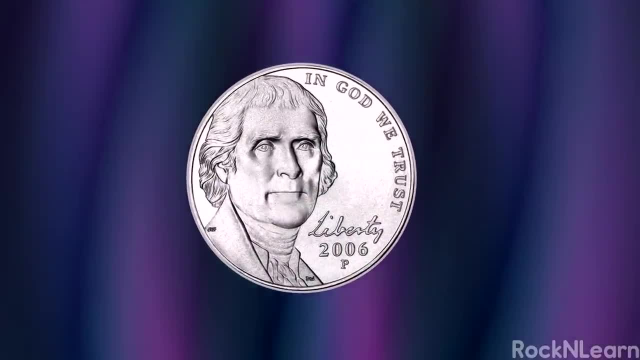 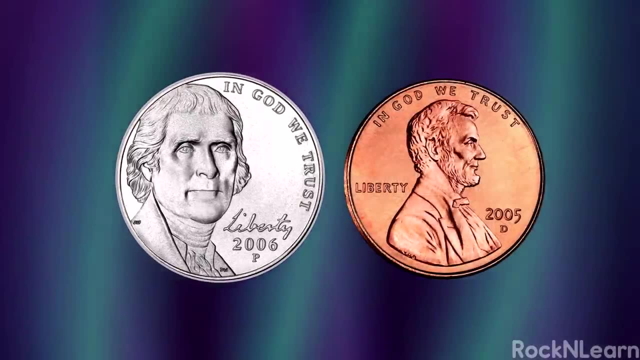 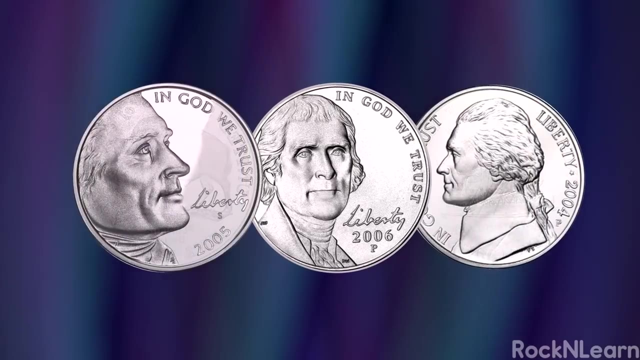 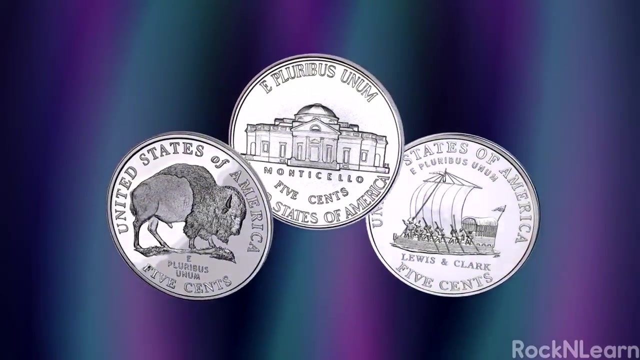 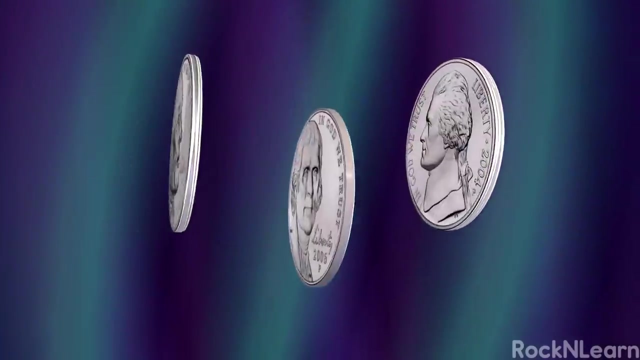 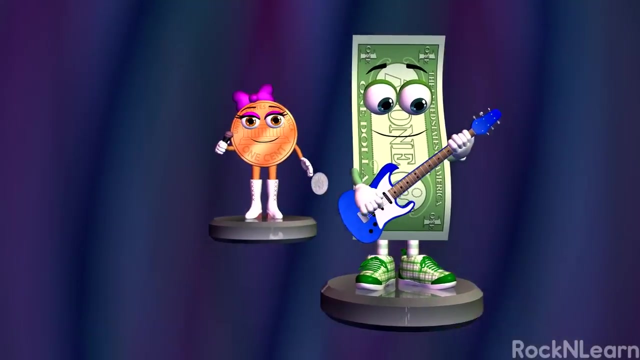 The coin called a nickel is worth five cents. It's bigger than a penny. Now that makes sense. On the front of a nickel is Thomas Jefferson. The Declaration of Independence. draftsperson. The Declaration of Independence draftsperson. The Declaration of Independence draftsperson. 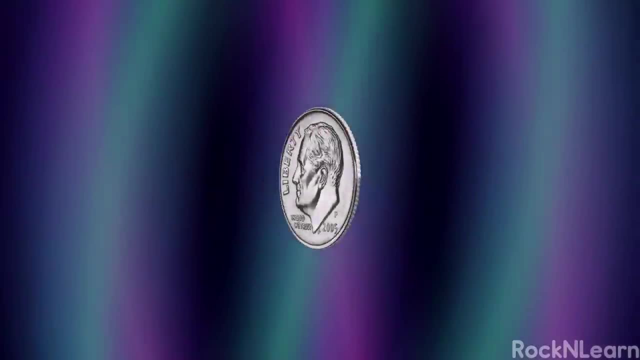 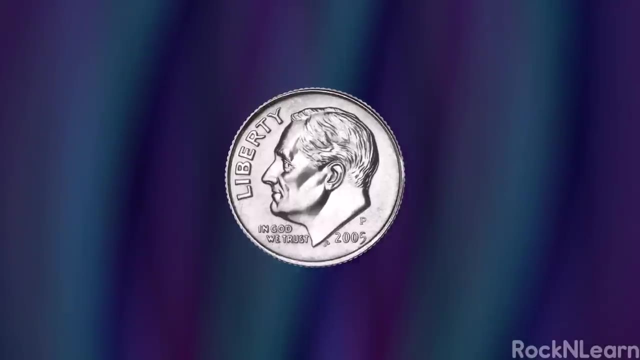 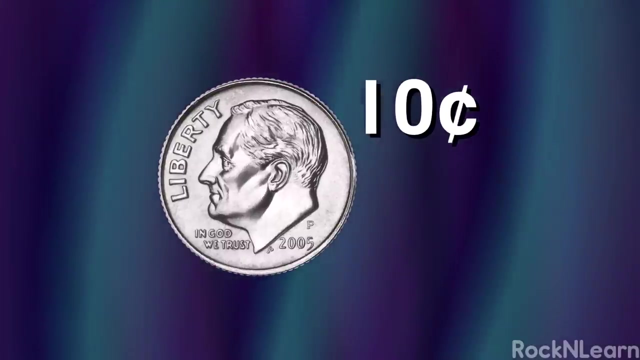 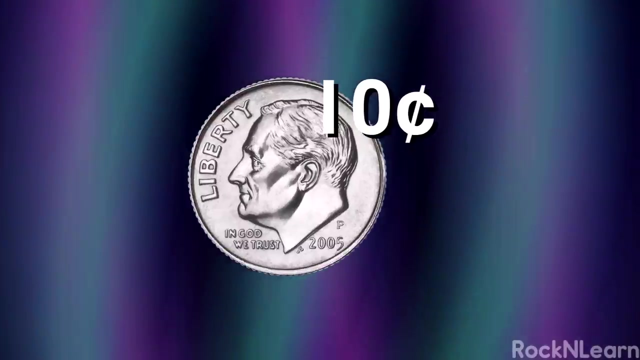 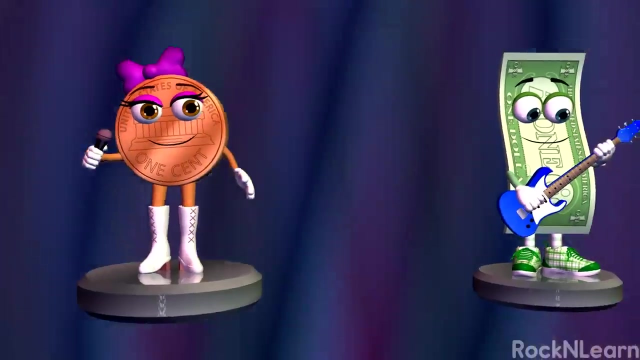 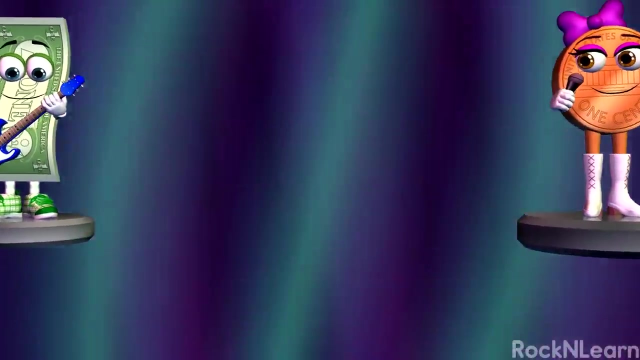 The smallest coin we have is the thin little dime With Franklin D Roosevelt on the front at this time. Ten cents is the worth of the dime. It's easy to remember as we sing this rhyme: Ten cents is the worth of the dime. 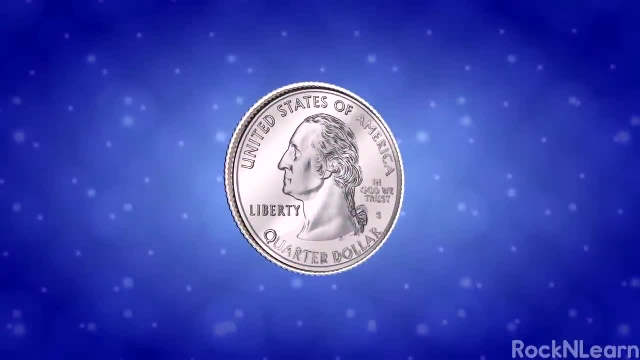 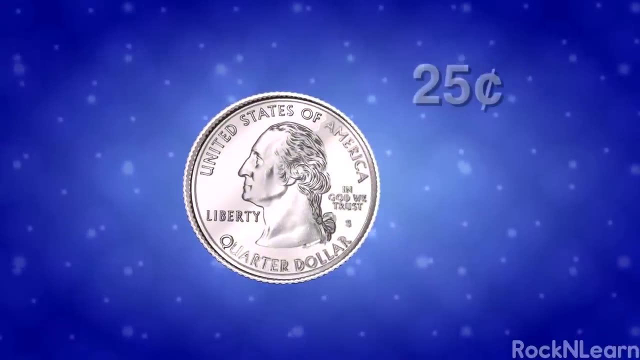 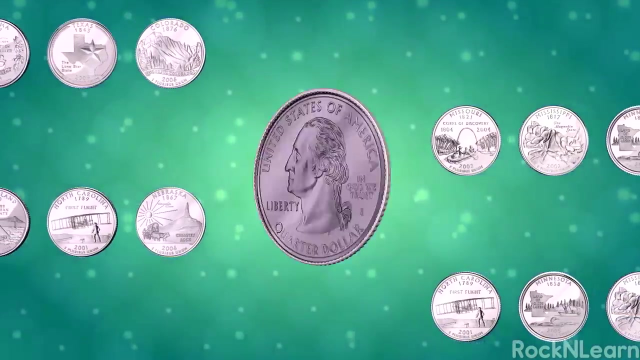 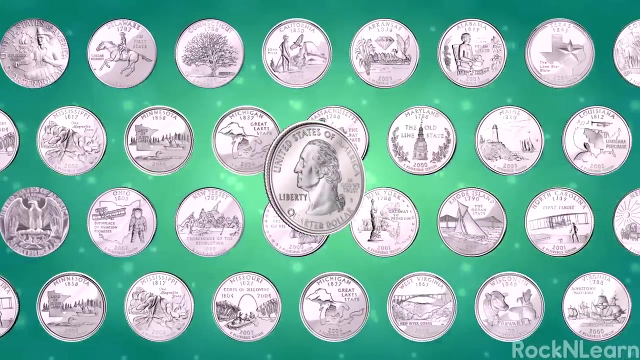 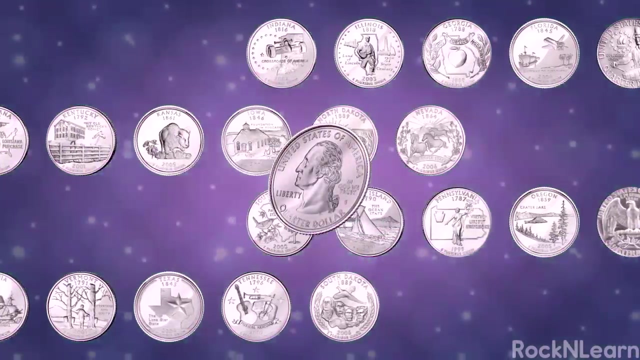 This coin is a quarter. The edge has many grooves. It's worth twenty-five cents. Now check out these moves. Oh, so many quarters, All different on the back. Variety is one thing, the quarters do not lack. George Washington's. 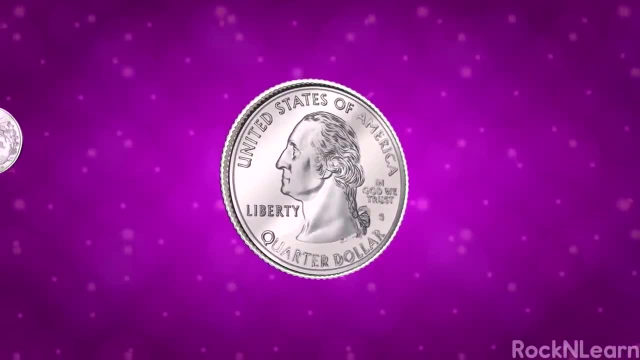 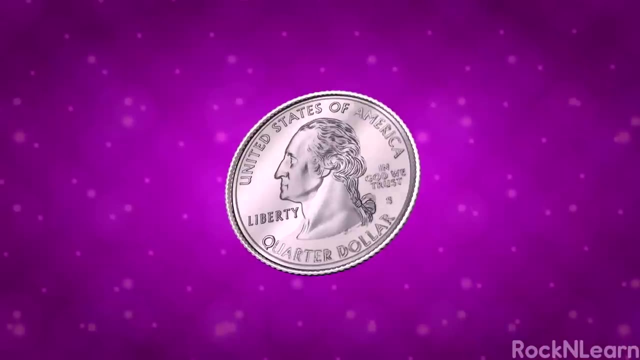 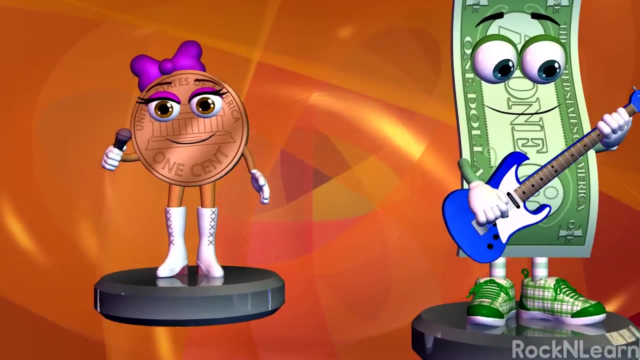 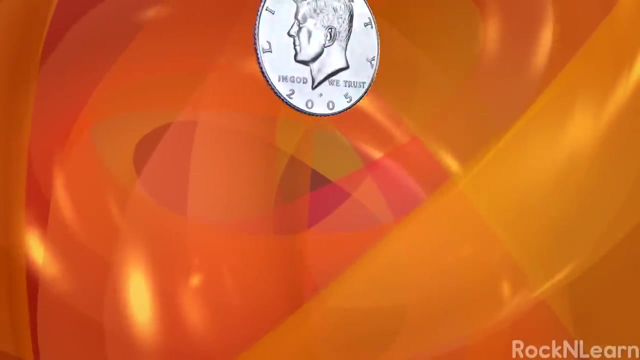 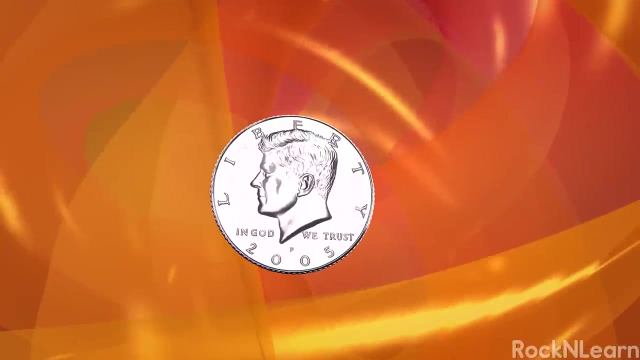 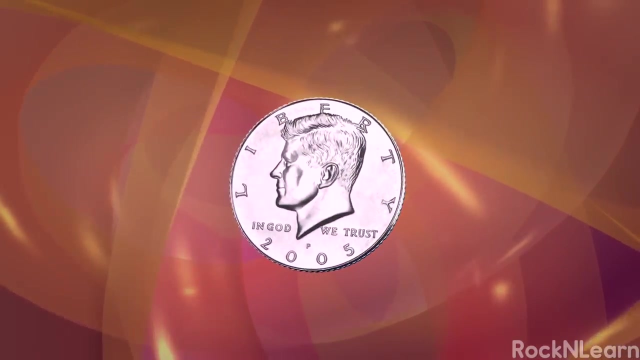 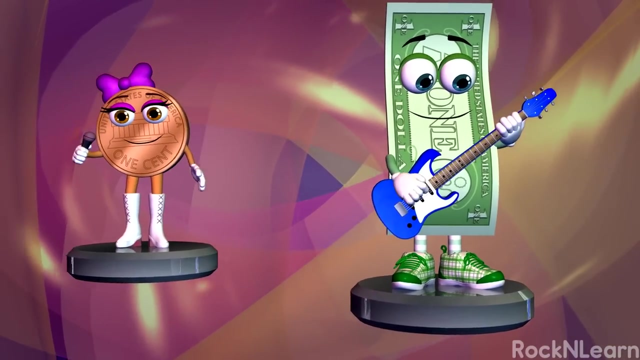 been on the front- it's true Of the quarter of a dollar- since 1932.. On the front of the half dollar is John F Kennedy. It's worth fifty cents. But you won't find many Dollar coins changed color From silver. 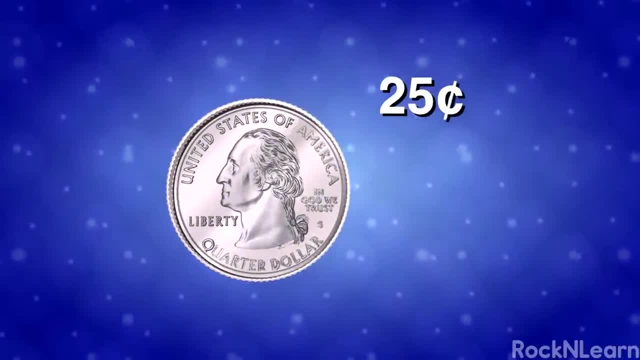 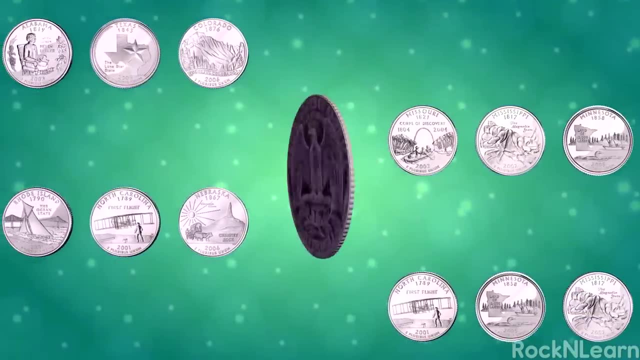 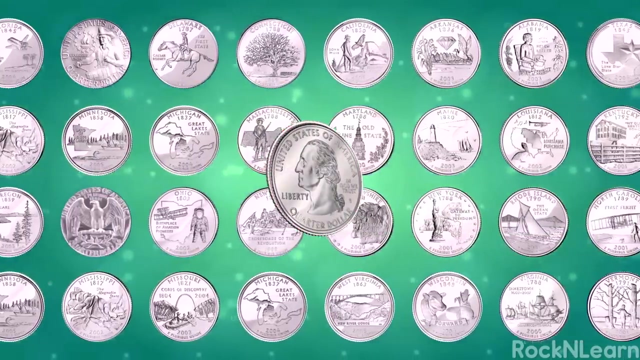 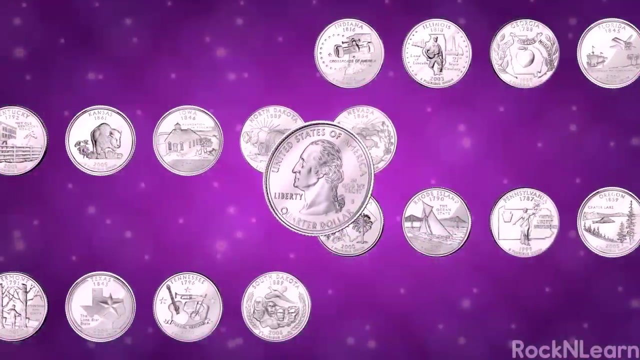 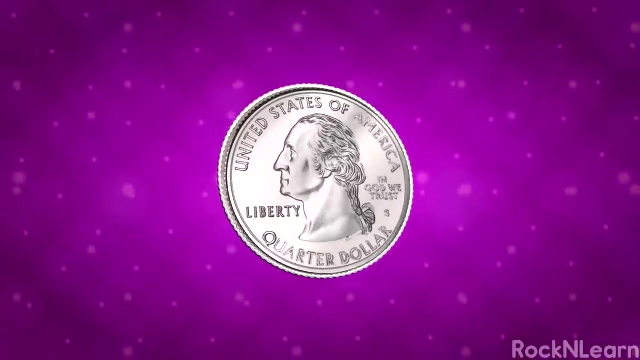 It's worth twenty-five cents. Now check out these moves. Oh, so many quarters All different on the back. Variety is one thing. the quarters do not lack. George Washington's been on the front. it's true Of the quarter of a dollar. 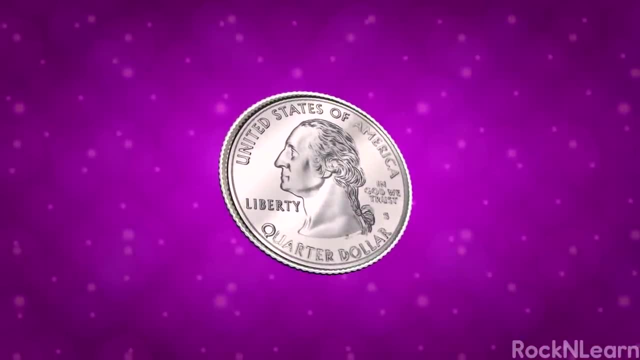 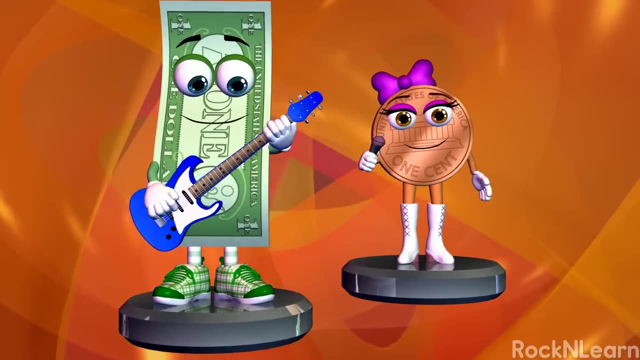 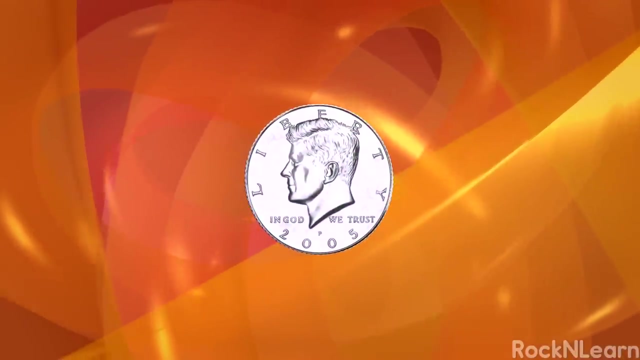 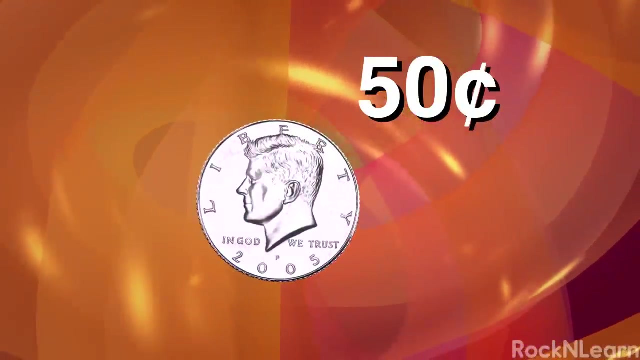 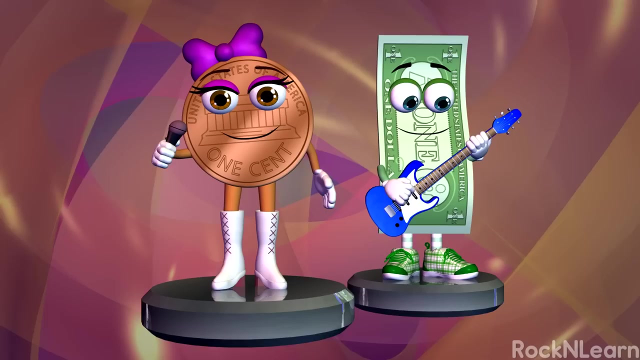 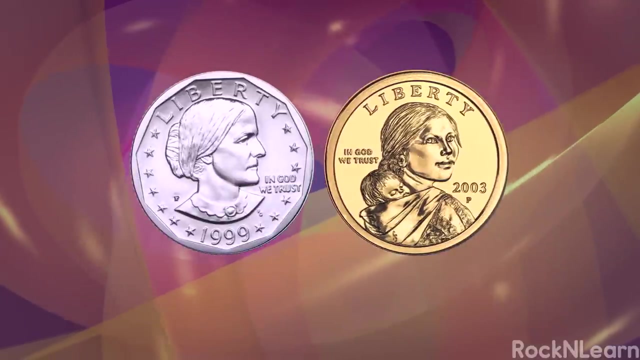 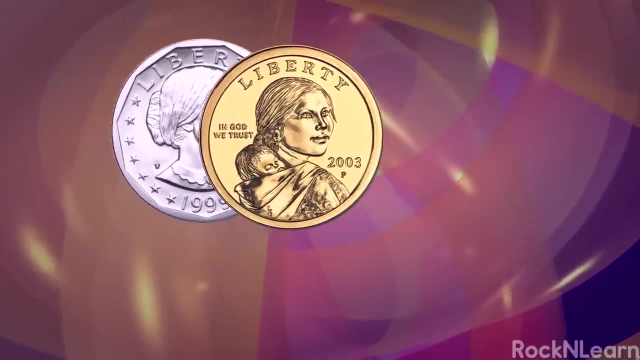 since 1932.. On the front of the half dollar is John F Kennedy. It's worth fifty cents But you won't find many Dollar coins changed color From silver to gold. It helps tell them apart From quarters, I am told. 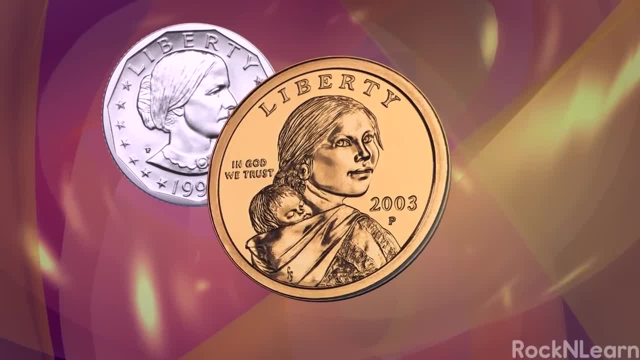 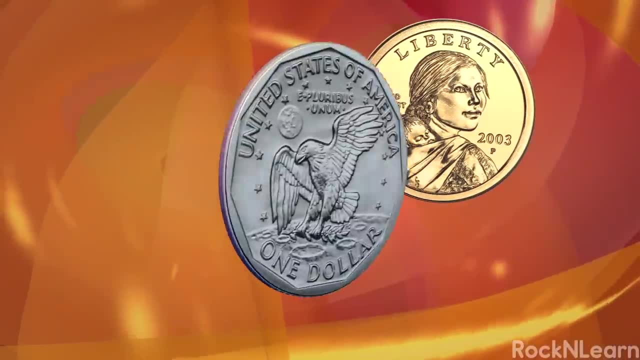 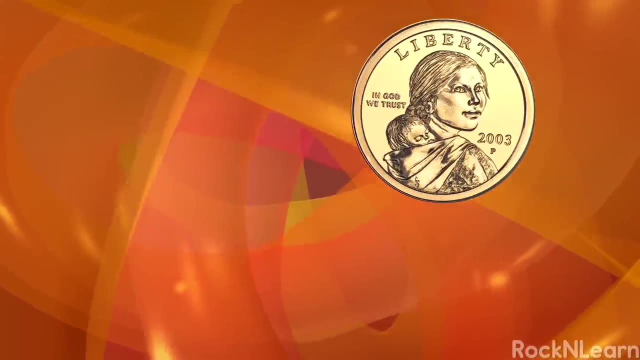 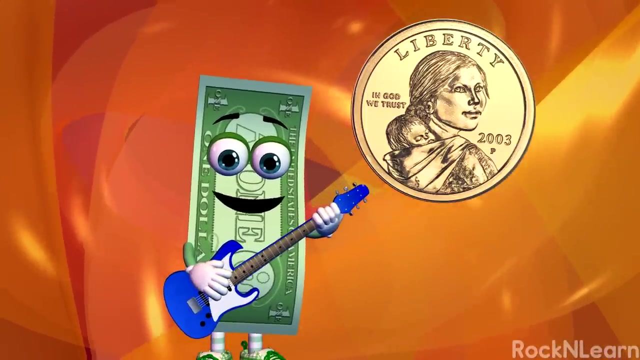 Sacagawea is on the one that looks gold, But Susan B Anthony is on the silver. one of old Who is Sacagawea? Sacagawea was a famous Shoshone interpreter and guide In the early 1800's. 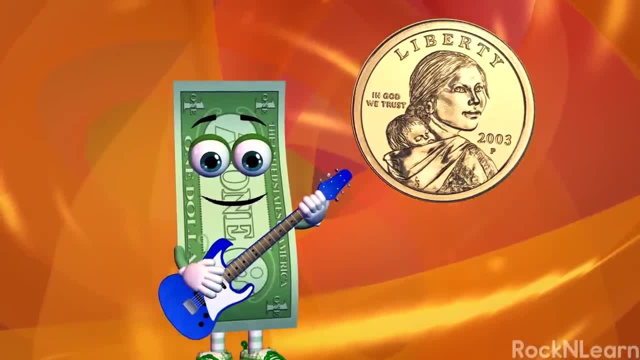 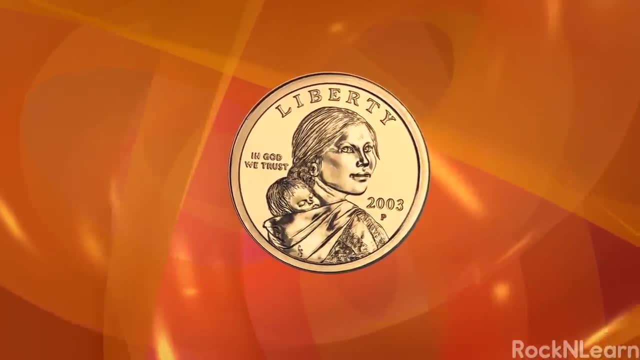 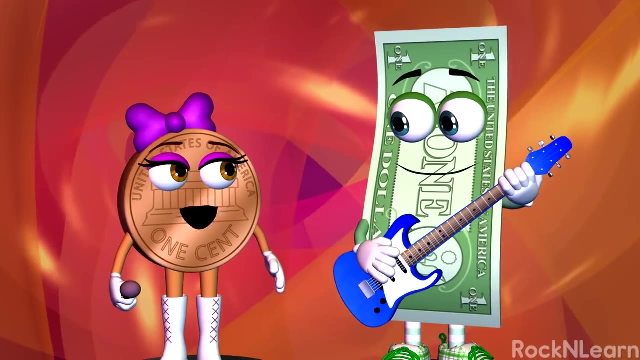 she helped two famous explorers, Lewis and Clark, discover new lands in the western part of the United States. If it wasn't for Sacagawea, Lewis and Clark may never have seen the Great Plains or the Pacific Ocean. Wow, Bill, that's a really neat story. 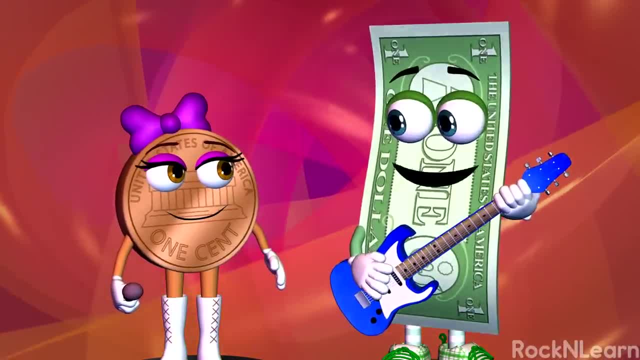 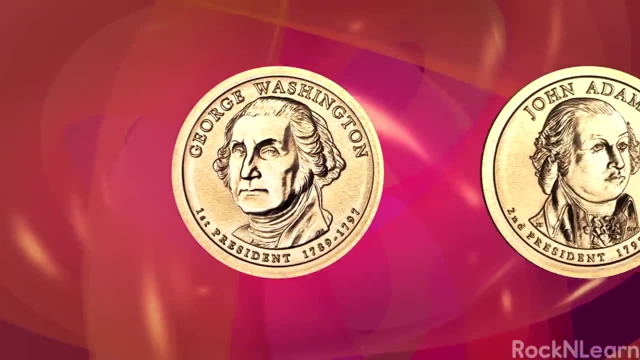 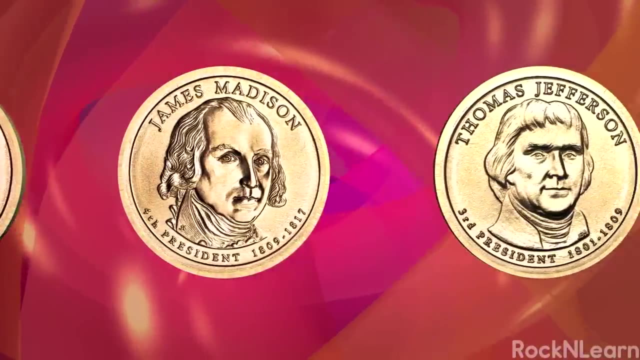 I guess all those people who were on the coins were important to the United States. That's right, Penny. In fact, starting in 2007, the US Mint began releasing four new dollar coins every year. Each one of these coins will have the 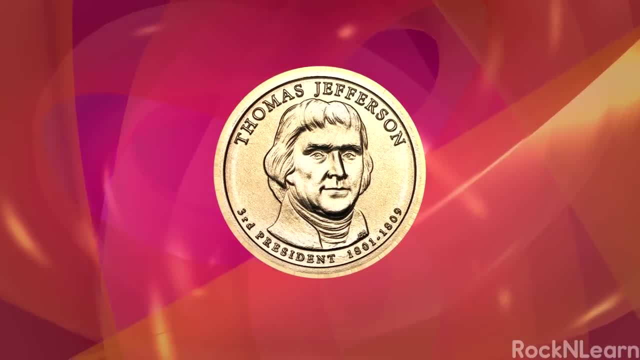 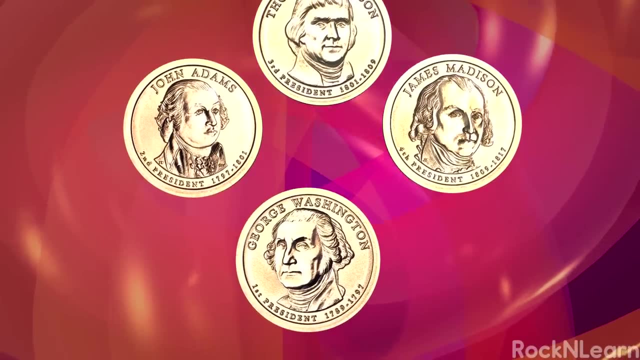 face of a different American President on the front, and all of them will have the Statue of Liberty on the back. Here are just a few of these coins. They're about the same size and color as the Sacagawea dollar, But look. 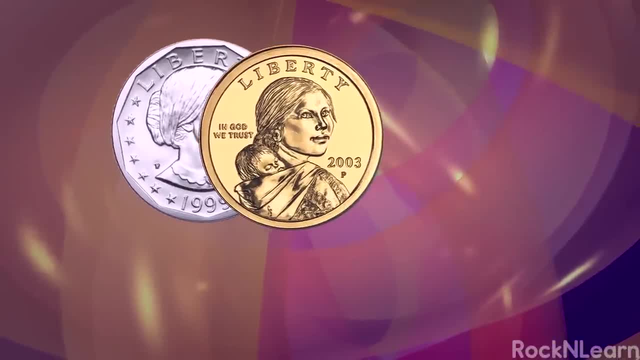 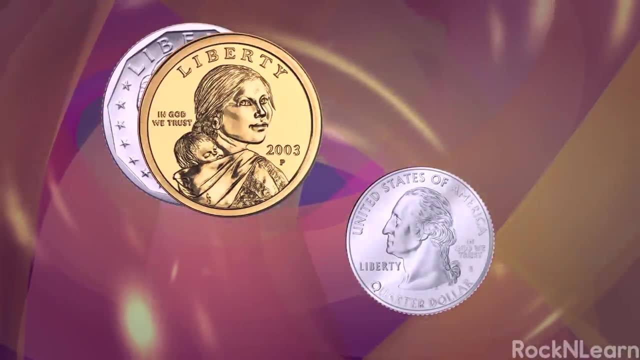 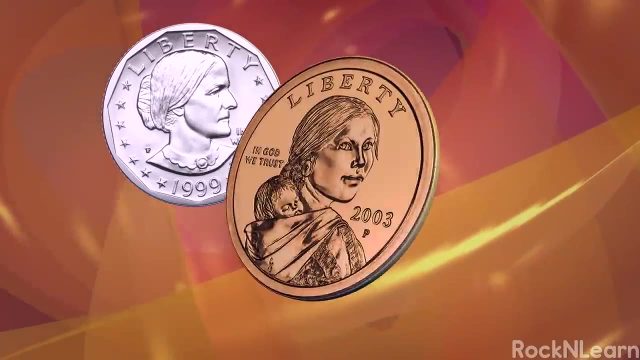 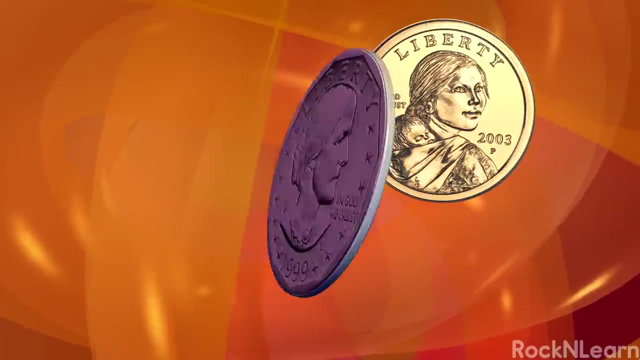 to gold. It helps tell them, apart From quarters. I am told Sacagawea is on the one that looks gold, But Susan B Anthony is on the silver. one of old, Who is Sacagawea, Sacagawea? 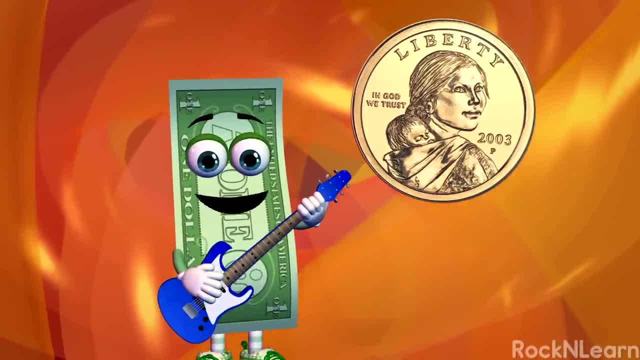 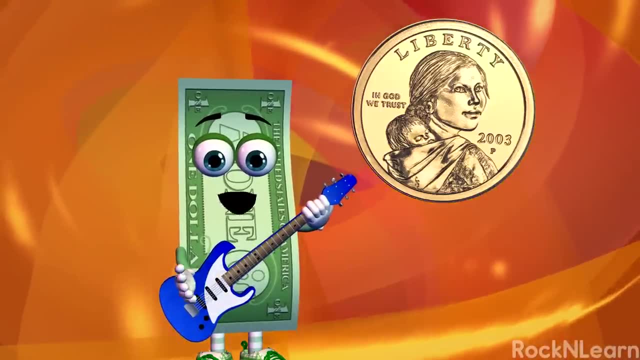 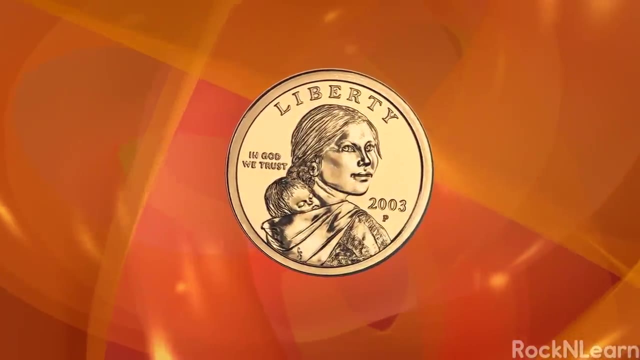 was a famous Shoshone interpreter and guide. In the early 1800's she helped two famous explorers, Lewis and Clark, discover new lands in the western part of the United States. If it wasn't for Sacagawea, Lewis and Clark may never have seen. 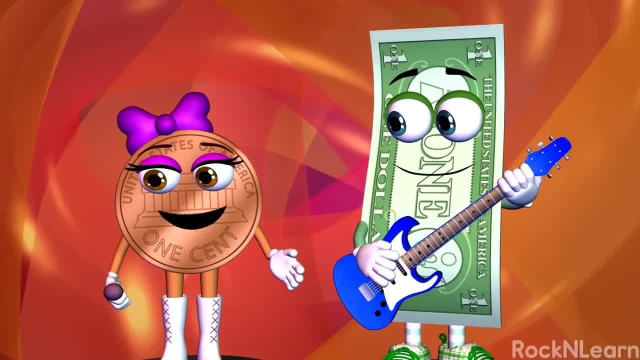 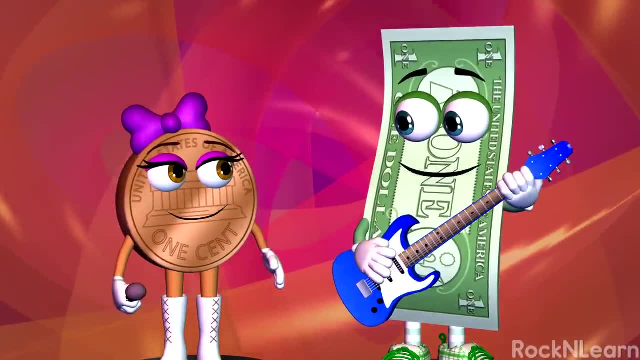 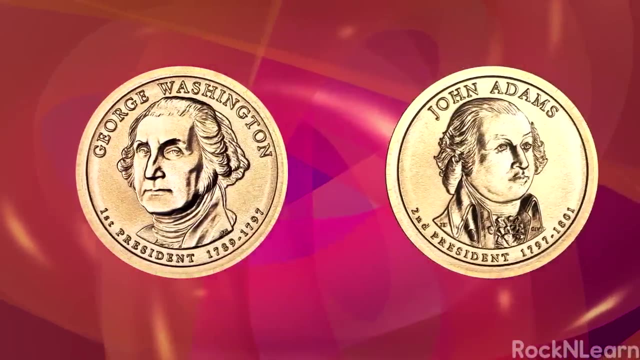 the Great Plains or the Pacific Ocean. Wow, Bill, that's a really neat story. I guess all those people who were on the coins were important to the United States. That's right, Penny. In fact, starting in 2007, the US Mint began releasing four. 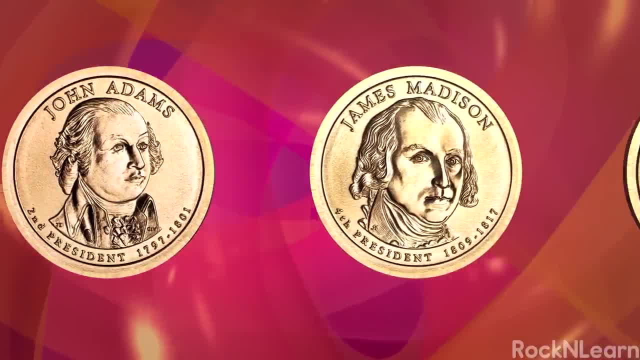 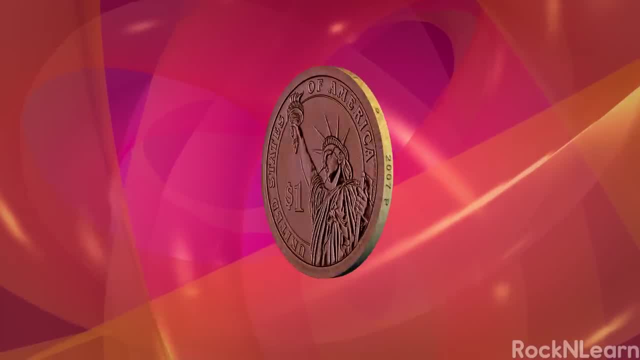 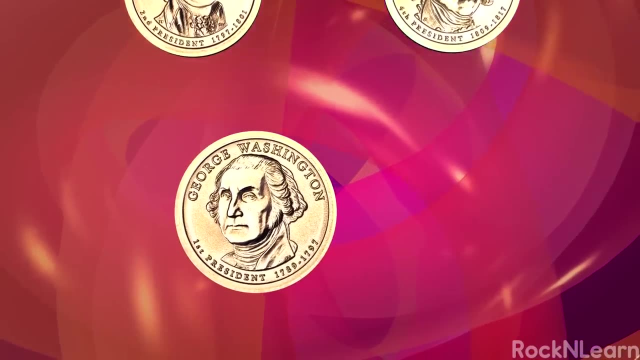 new dollar coins every year. Each one of these coins will have the face of a different American President on the front, and all of them will have the Statue of Liberty on the back. Here are just a few of these coins. They're about the same size and color as the. 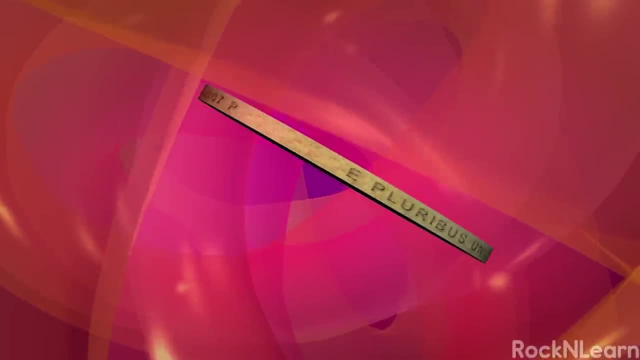 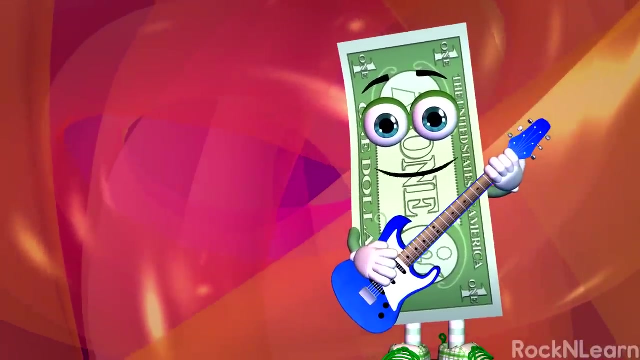 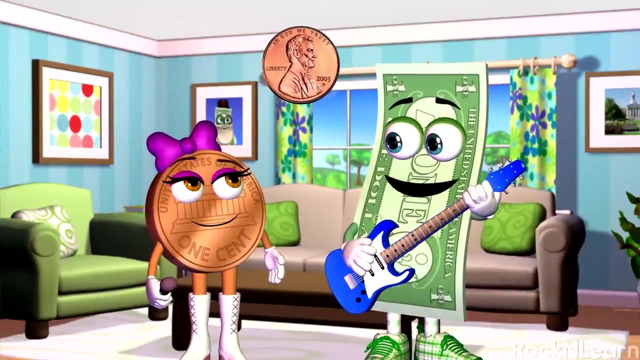 Sacagawea dollar. But look, They have writing on the edge. Now that we know what the coins look like, let's learn to count them. We'll start by counting pennies. Wow, Penny, it kind of looks like you, I don't know. 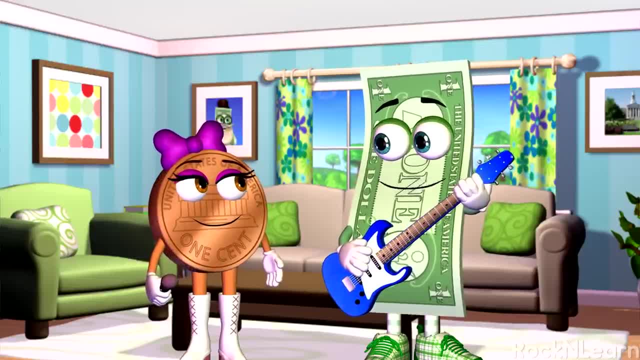 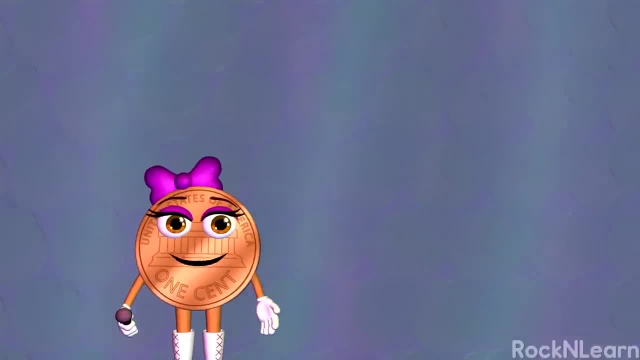 I don't really see the resemblance. Now, if we want enough pennies to equal a dollar bill, we'll have to count 100 pennies. We could count them one by one or, to make it go a little faster, we could count by twos. 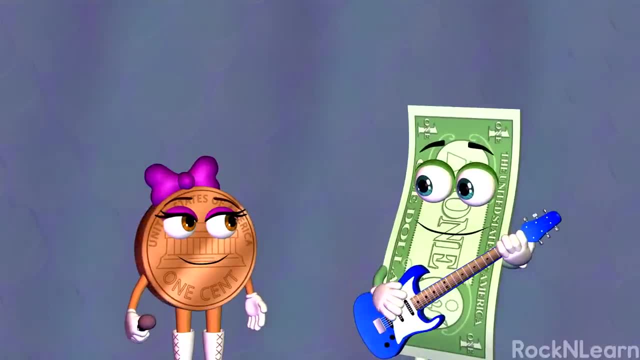 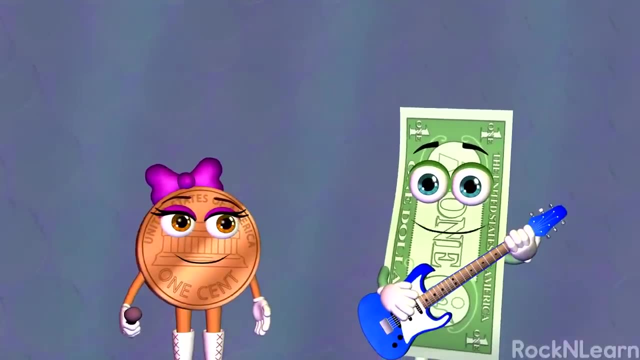 Pulling two pennies toward us each time we count. That sounds like a good idea. One penny is also called one cent, So two pennies are two cents. Let's count by twos until we have a dollar or 100 cents. 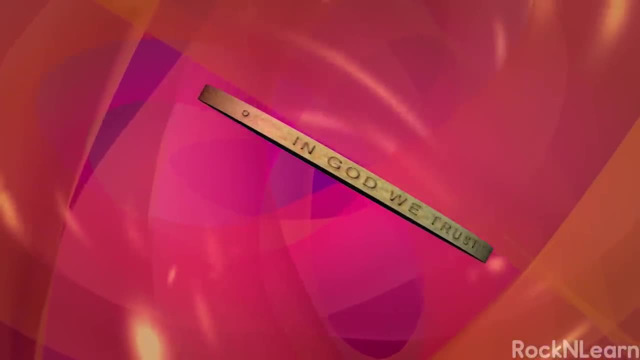 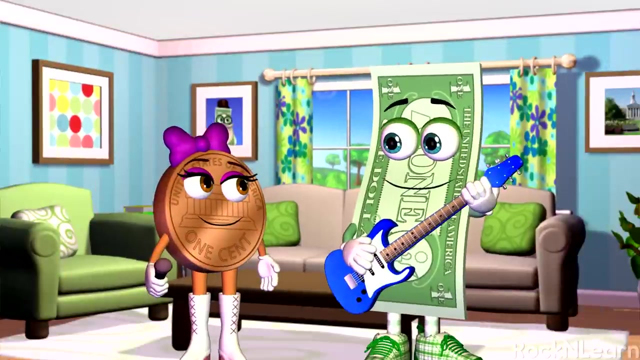 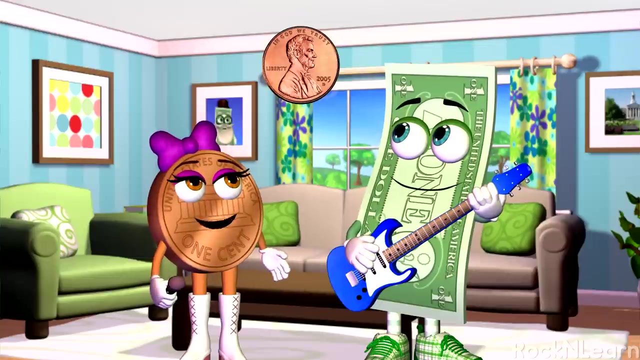 They have writing on the edge. Now that we know what the coins look like, let's learn to count them. We'll start by counting pennies. Wow, Penny, it kind of looks like you, I don't know. I don't really see the resemblance. 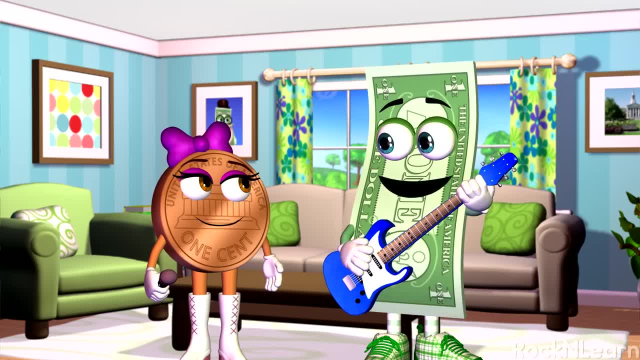 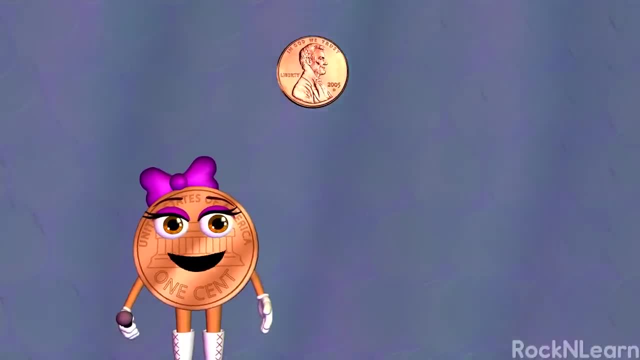 Now, if we want enough pennies to equal a dollar bill, we'll have to count 100 pennies. We could count them one by one or, to make it go a little faster, we could count by twos, Pulling two pennies toward us each time we count. 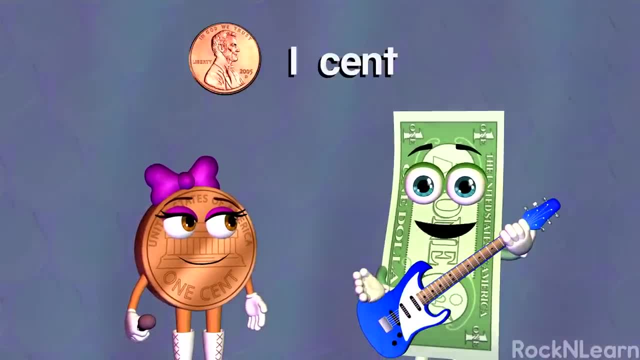 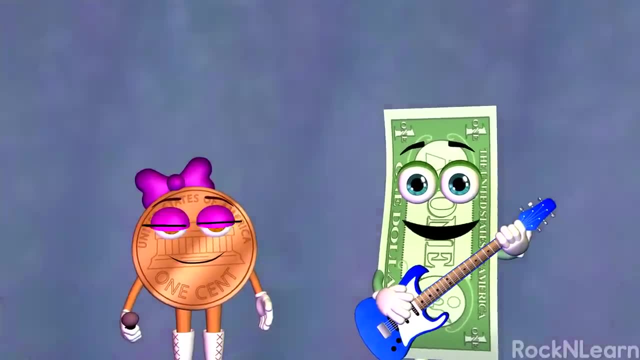 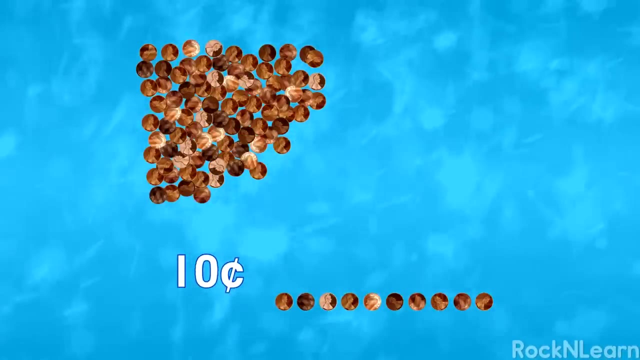 That sounds like a good idea. One penny is also called one cent, So two pennies are two cents. Let's count by twos until we have a dollar or 100 cents. 2, 4, 6, 8, 10, 12, 14. 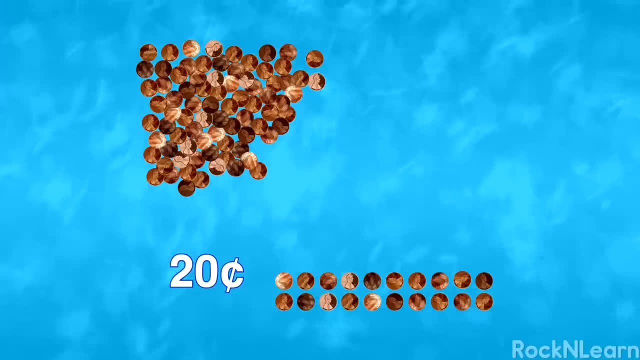 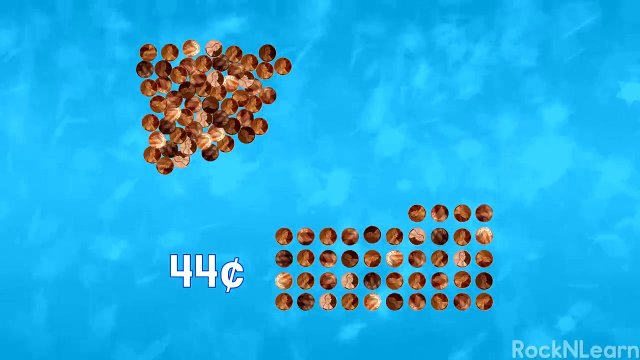 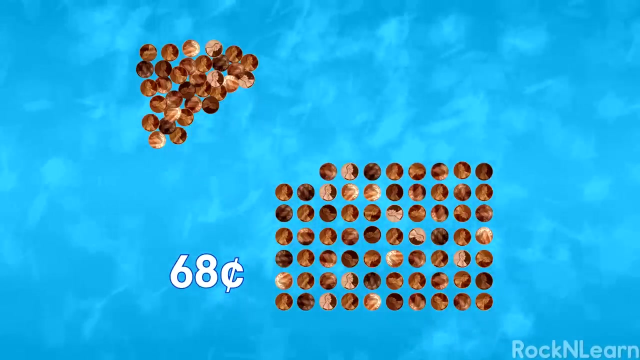 16, 18, 20, 22, 24, 26, 28, 30, 32, 34, 36, 38, 40, 42, 44, 46, 48, 50, 72, 74, 76, 78, 80, 82, 84, 86. 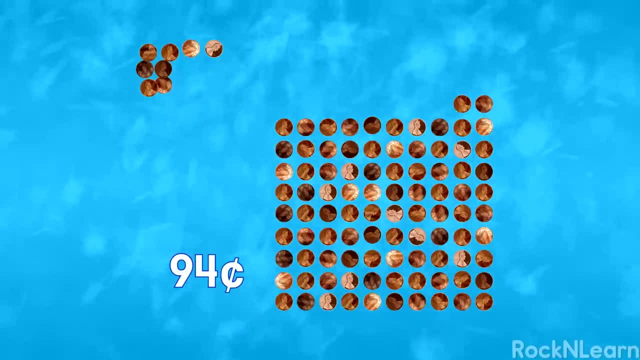 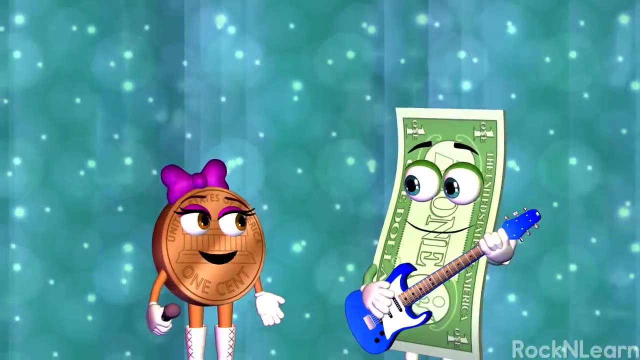 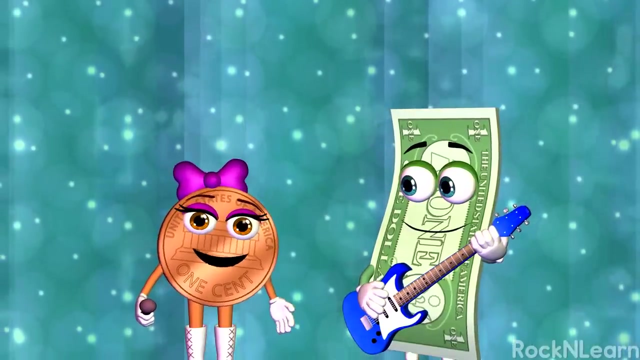 88, 90, 92, 94, 96, 98, 100. Hooray, we counted 100 cents. That's a whole dollar. There are other ways we can count pennies too. We can put them in stacks of 5 or 10. 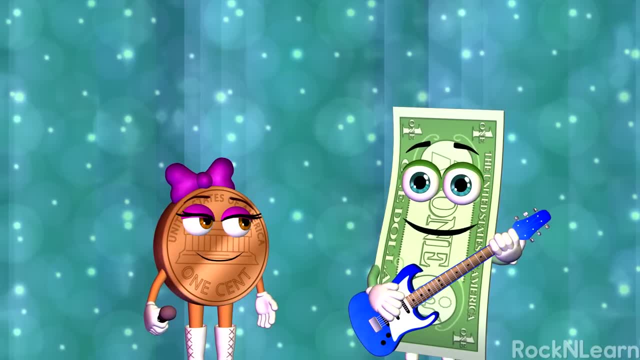 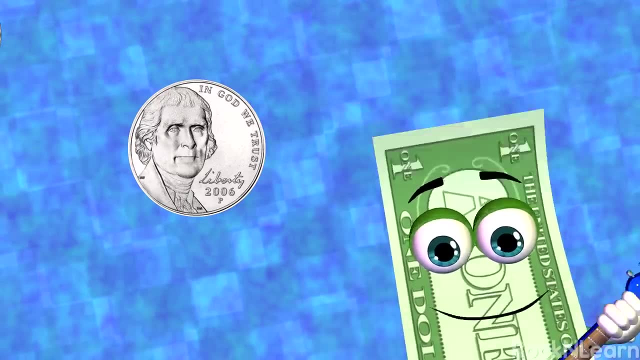 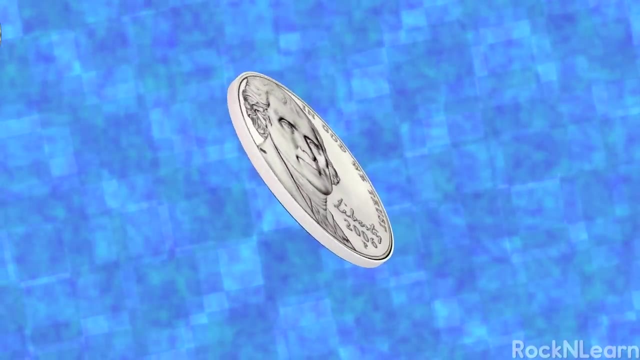 and skip count using the stacks. Putting pennies in stacks also makes it easier if we have to count them with other coins, Like the nickel. Nickels are the silver colored coins with Thomas Jefferson on the front And they have a very smooth edge. 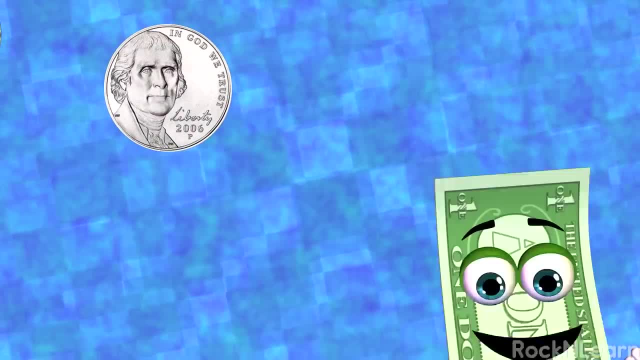 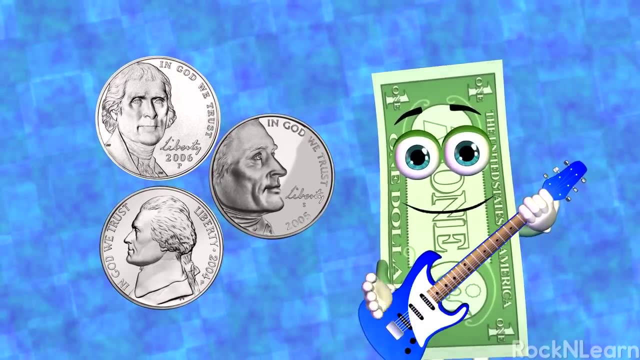 They're also thicker and heavier than pennies. That's right Now. remember. nickels can have different designs on them. They're made that way by the United States Mint. I love mints, Especially chocolate mints. No Penny. 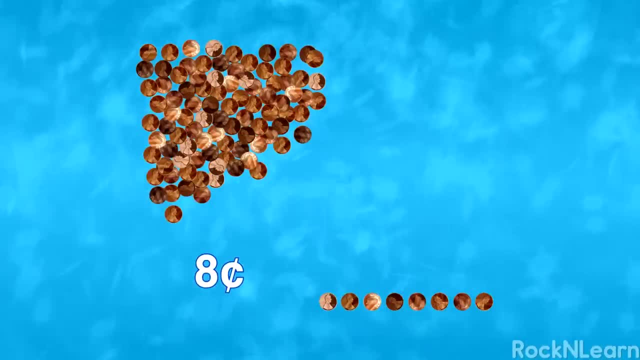 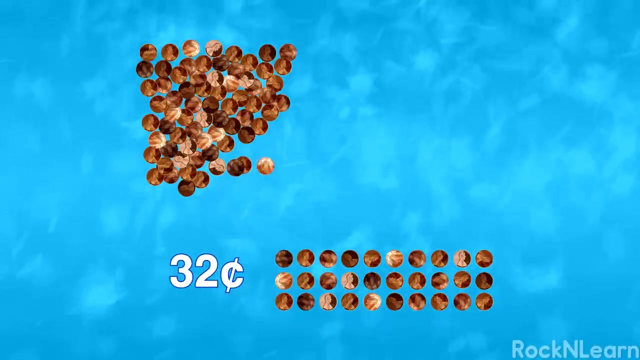 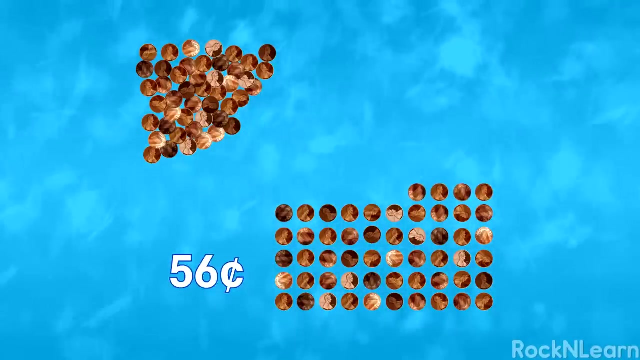 2, 4, 6, 8, 10, 12, 14, 16, 18, 20, 22, 24, 26, 28, 30, 32, 34, 36, 38, 40, 42, 44, 46, 48, 50, 72. 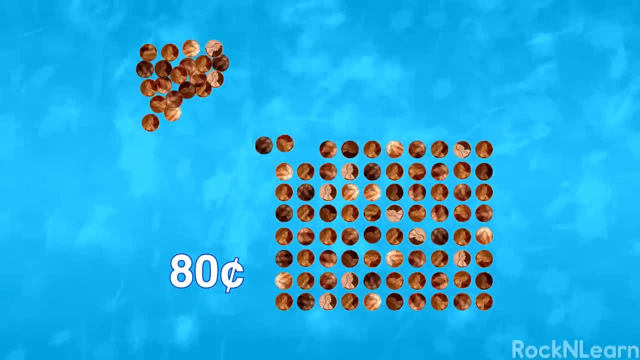 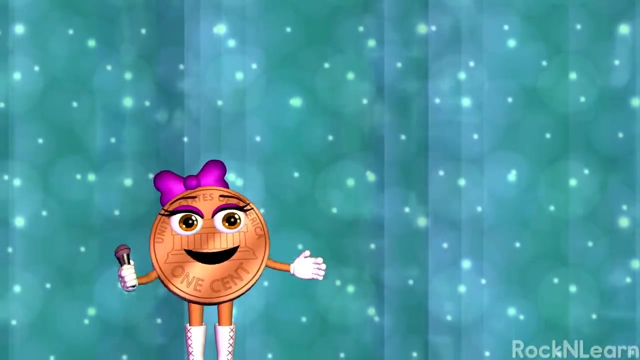 74, 76, 78, 80, 82, 84, 86, 88, 90, 92, 94, 96, 98, 100. Hooray, we counted 100 cents. That's a whole dollar. There are other ways we can count pennies too. 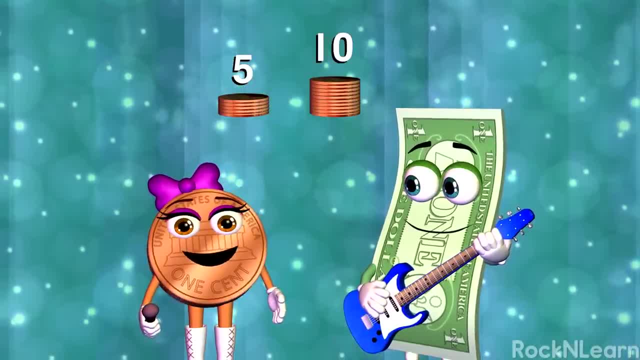 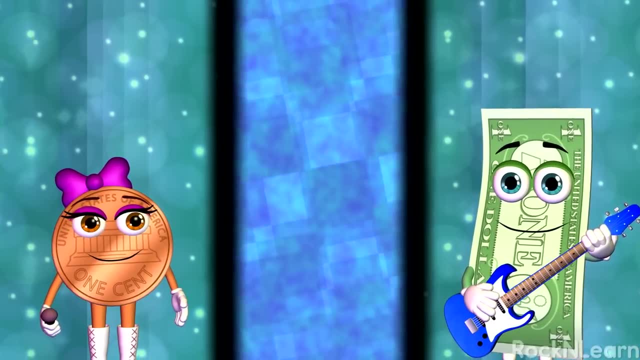 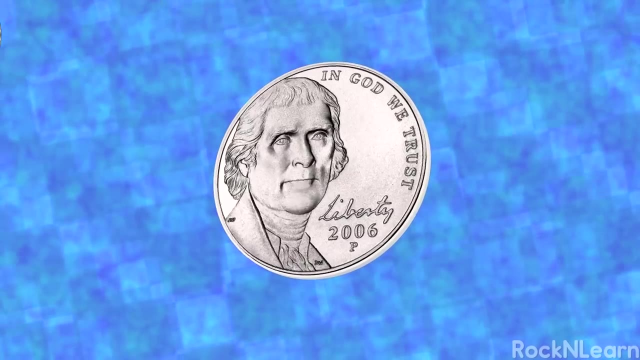 We can put them in stacks of 5 or 10 and skip count using the stacks. Putting pennies in stacks also makes it easier if we have to count them with other coins. Like the nickel Nickels are the silver colored coins with Thomas Jefferson on the front. 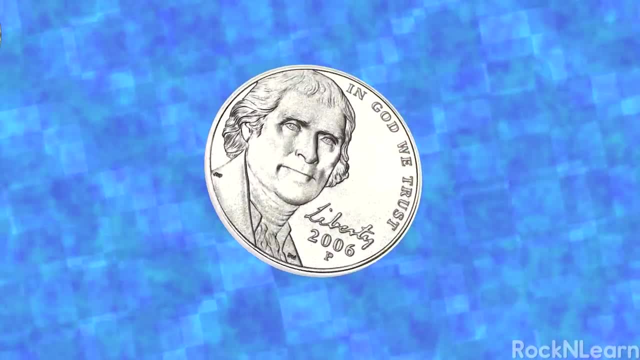 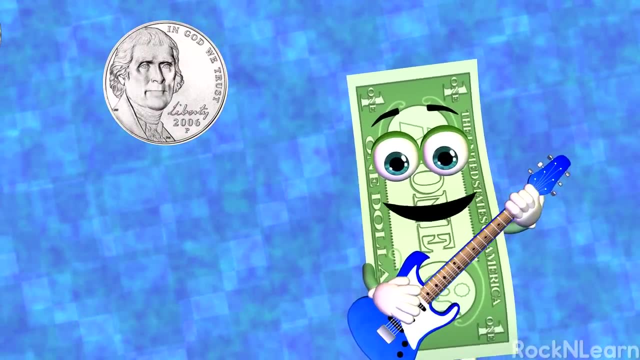 And they have a very smooth edge. They're also thicker and heavier than pennies. That's right Now. remember nickels can have different designs on them. They're made that way by the United States Mint. I love mints, Especially chocolate mints. 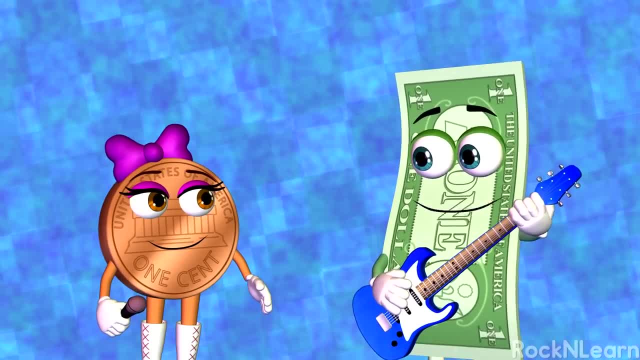 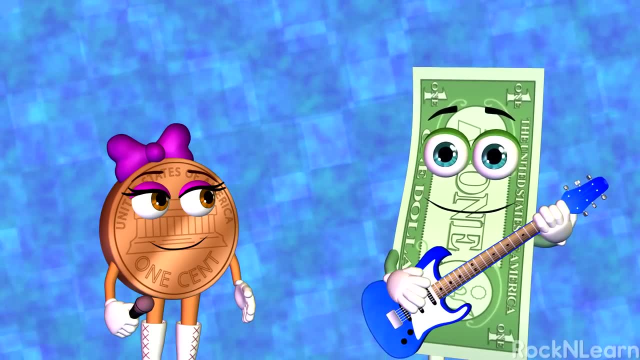 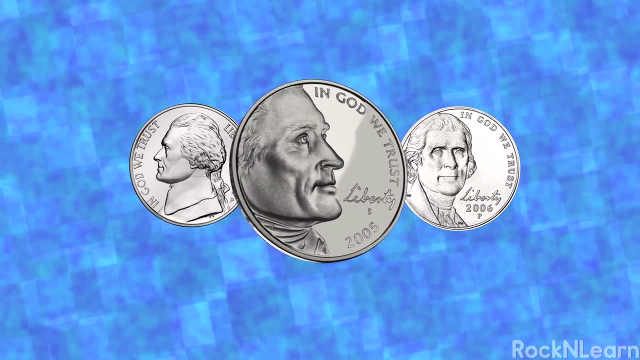 No, Penny, Not that kind of mint. When we are talking about coins, the word mint means a place where the coins are made. Take a look at these nickels. They all have Thomas Jefferson on the front, but this one has a close-up of him. Even though they look a little different from each other, each nickel is still worth 5 cents, So counting nickels is like counting by fives: 5, 10, 15, 20, 25, 30, 35, 40, 45, 50. 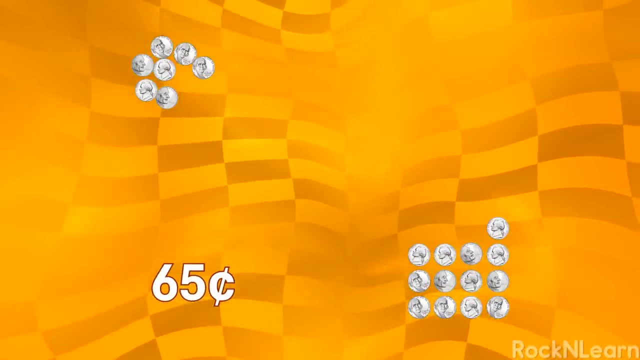 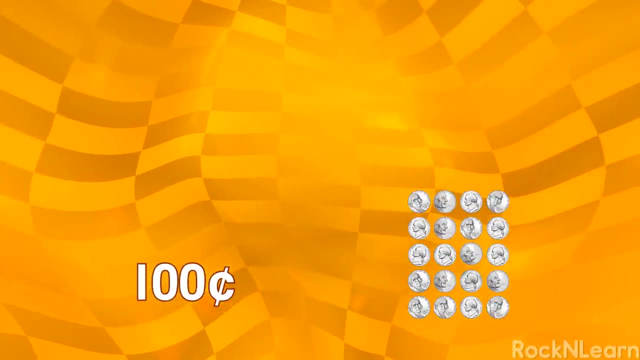 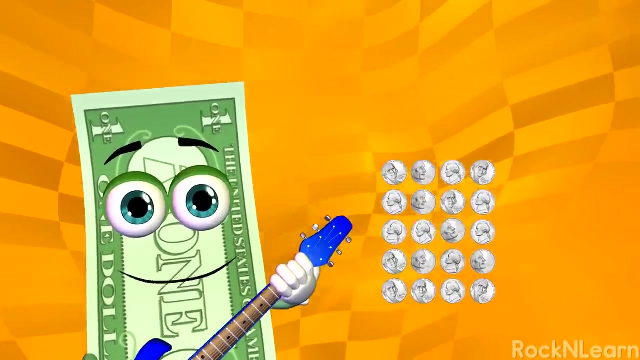 55, 60, 65, 70, 75, 80, 85, 90, 95, 100. Now that we've counted the nickels up to a dollar, let's see how many nickels it took to make that dollar: 1, 2. 3, 4, 5, 6, 7, 8, 9, 10, 11, 12, 13, 14, 15, 16, 17, 18, 19, 20. So to make a dollar we need 100 pennies or 20 nickels. 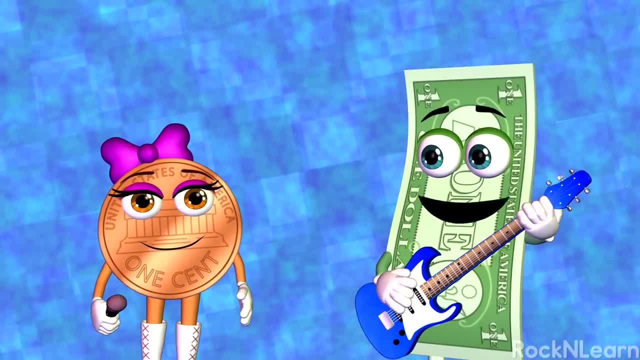 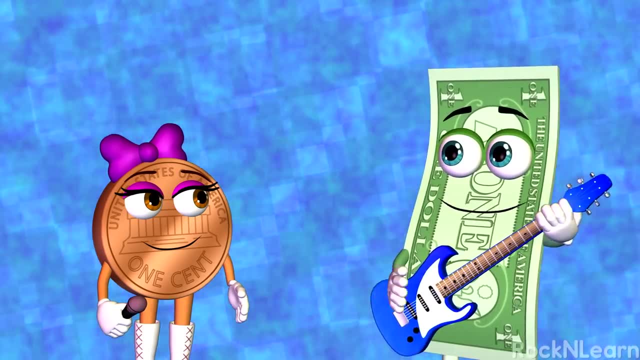 Not that kind of mint. When we are talking about coins, the word mint means a place where the coins are made. Take a look at these nickels. They all have Thomas Jefferson on the front, but this one has a close-up of him. Even though they look a little different from each other, each nickel is still worth 5 cents, So counting nickels is like counting by fives: 5, 10, 15, 20, 25, 30, 35, 40, 45, 50. 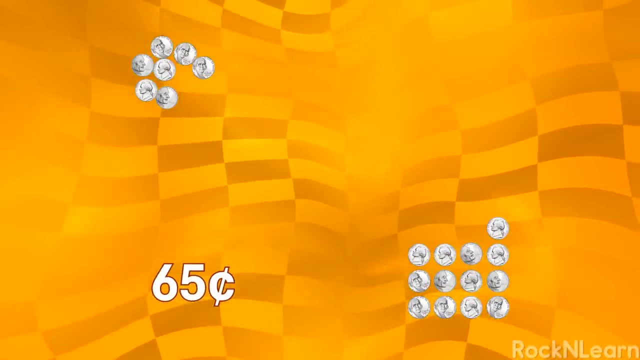 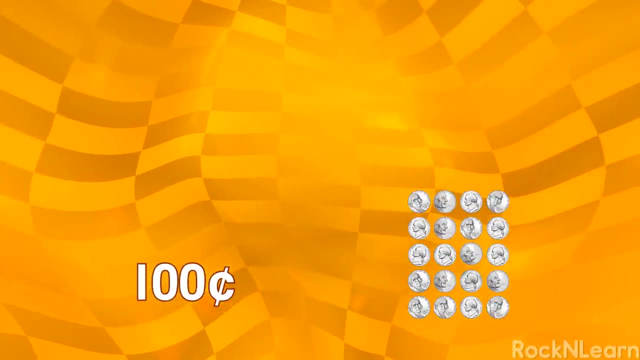 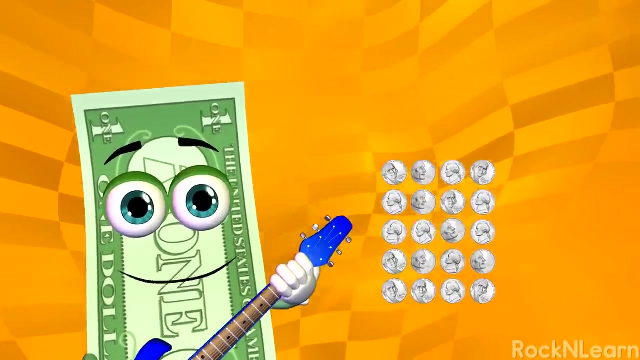 55, 60, 65, 70, 75, 80, 85, 90, 95, 100. Now that we've counted the nickels up to a dollar, let's see how many nickels it took to make that dollar: 1, 2. 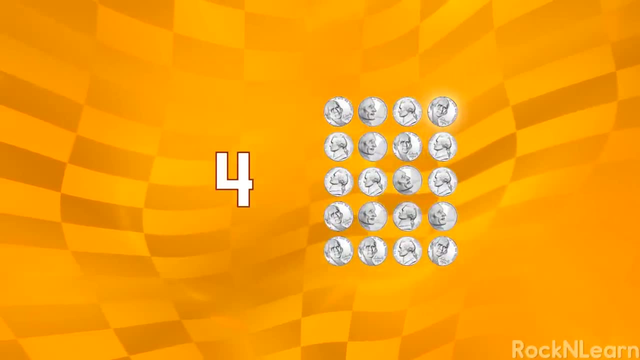 3, 4, 5, 6, 7, 8, 9, 10, 11, 12, 13, 14, 15, 16, 17, 18, 19, 20. So to make a dollar we need 100 pennies or 20 nickels. 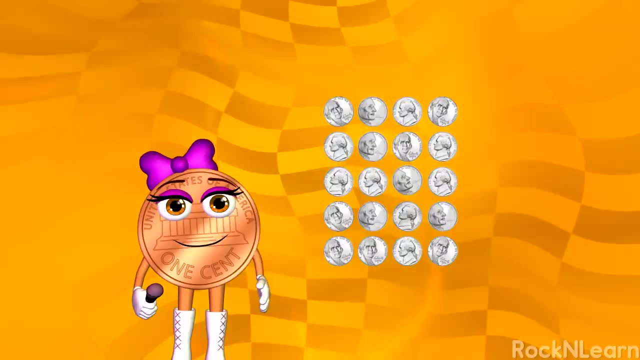 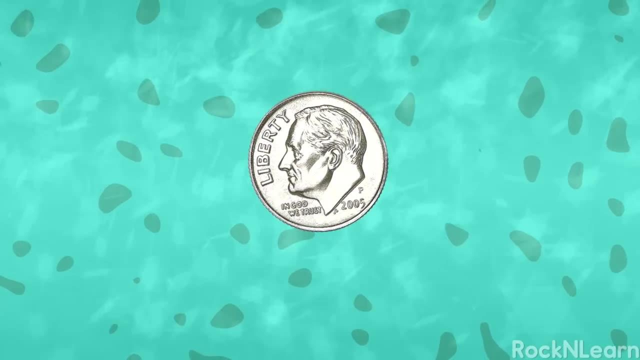 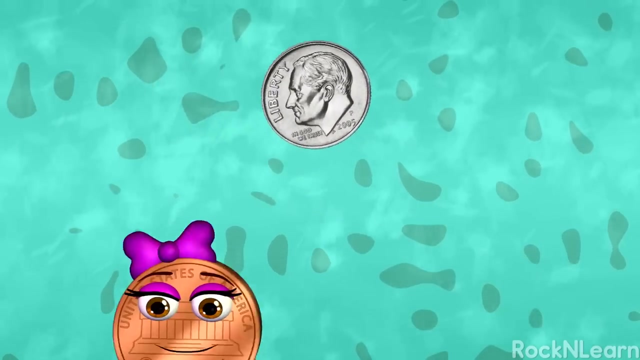 Let's see how many dimes we need to make a dollar. 1, 2, 3, 4, 5, 6, 7, 8, 9, 10, 11, 12, 13, 14, 15, 16, 17, 18, 19. 20, 21, 22, 23, 24, 25, 26, 27, 28, 29, 30, 31, 33, 33, 34, 35, 36, 37, 38, 39, 40, 41, 42, 43, 44, 45. 46, 47, 48, 49, 49, 50, 51, 52, 53, 54, 55, 56, 57, 58, 59, 60, 60, 61, 62, 63, 64, 65, 66, 67, 68, 69. 70, 71, 72, 73, 74, 75, 76, 77, 78, 79, 80, 81, 82, 83, 84, 85, 86, 87, 88, 89, 90, 91, 92, 83, 84, 85. 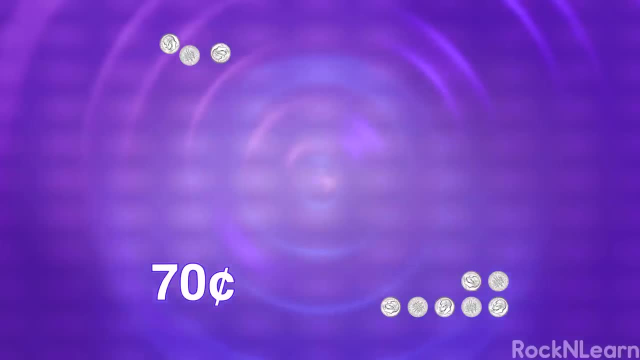 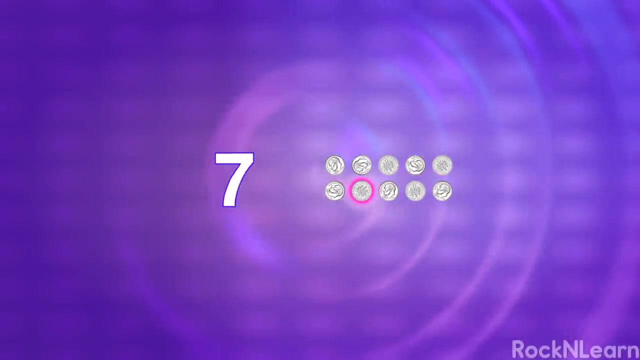 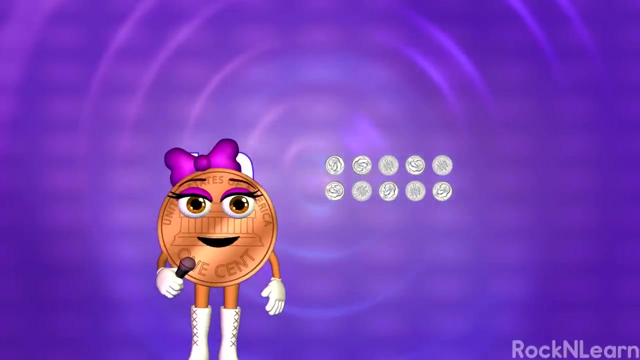 86, 87, 88, 89, 90, 91, 92, 93, 94, 95, 96, 97, 98, 99, 100, 10, 20, 30, 40, 50, 60, 70, 80, 70, 60, 70. 51, 67, 60, 75, 66, 7, 7, 6, 6, 7, 8, 8, 9, 10, 11, 12, 13, 14, 15, 16, 27, 29, 28, 30, 30, 31. 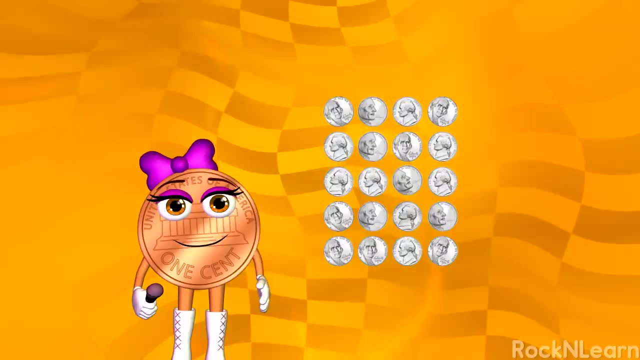 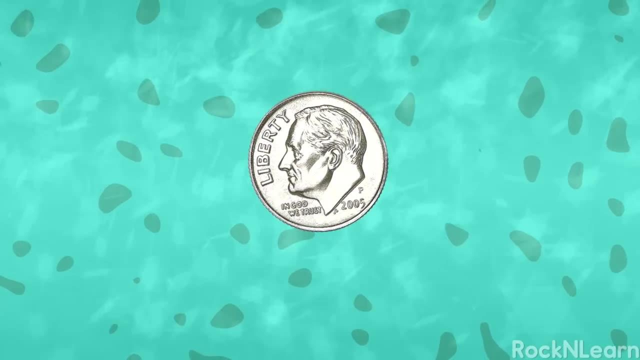 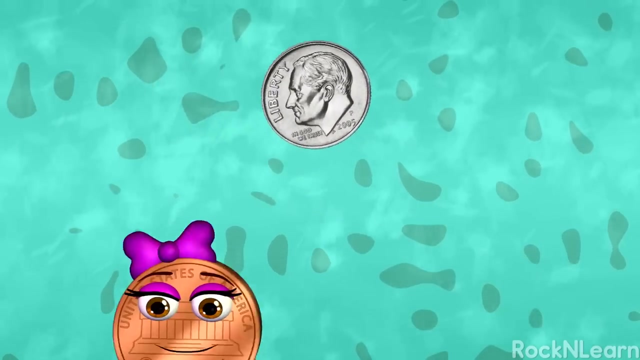 Let's see how many dimes we need to make a dollar. 1, 2, 3, 4, 5, 6, 7, 8, 9, 10, 11, 12, 13, 14, 15, 16, 17, 18, 19. 20, 21, 22, 23, 24, 25, 26, 27, 28, 29, 30, 31, 33, 33, 34, 35, 36, 37, 38, 39, 40, 41, 42, 43, 44, 45. 46, 47, 48, 49, 49, 50, 51, 52, 53, 54, 55, 56, 57, 58, 59, 60, 60, 61, 62, 63, 64, 65, 66, 67, 68, 69. 70, 71, 72, 73, 74, 75, 76, 77, 78, 79, 80, 81, 82, 83, 84, 85, 86, 87, 88, 89, 90, 91, 92, 83, 84, 85. 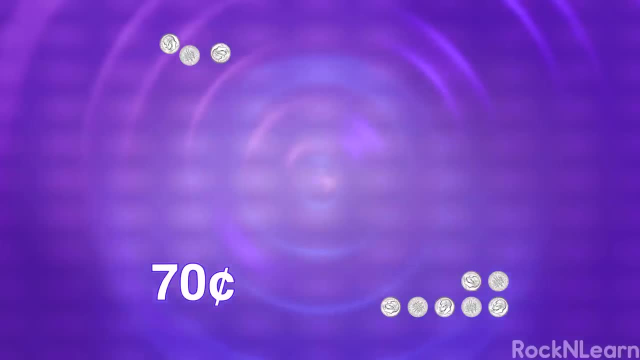 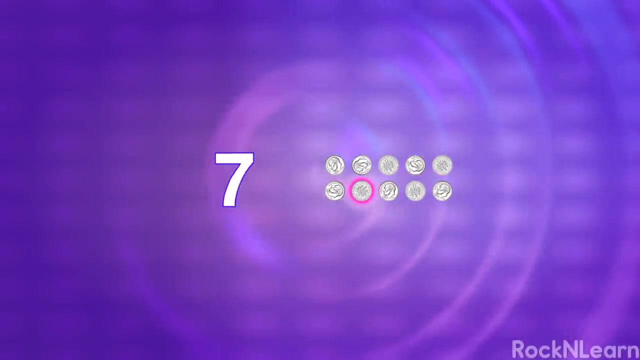 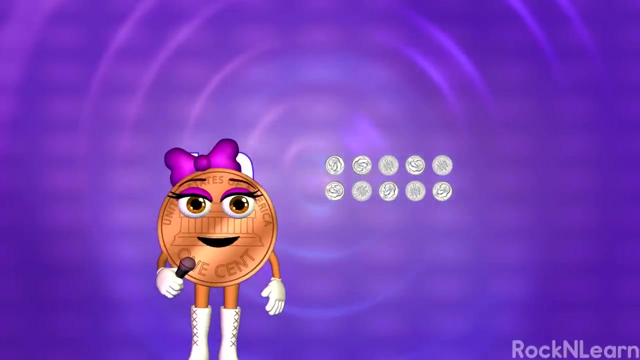 86, 87, 88, 89, 90, 91, 92, 93, 94, 95, 96, 97, 98, 99, 100, 10, 20, 30, 40, 50, 60, 70, 80, 70, 80, 80. 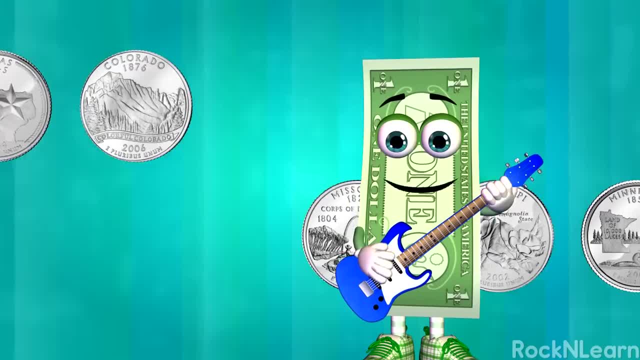 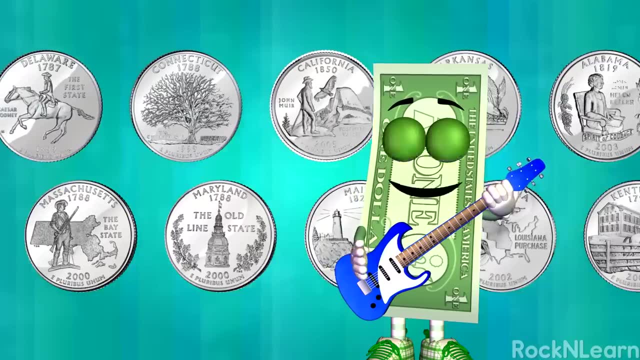 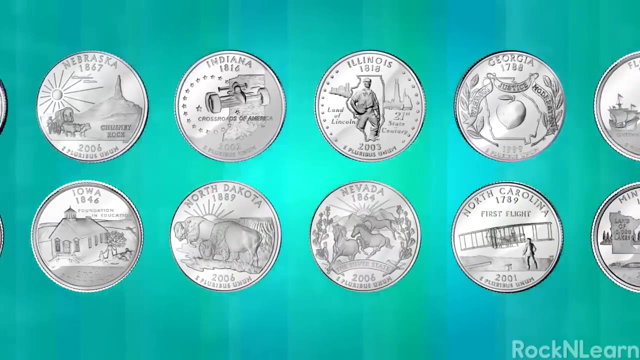 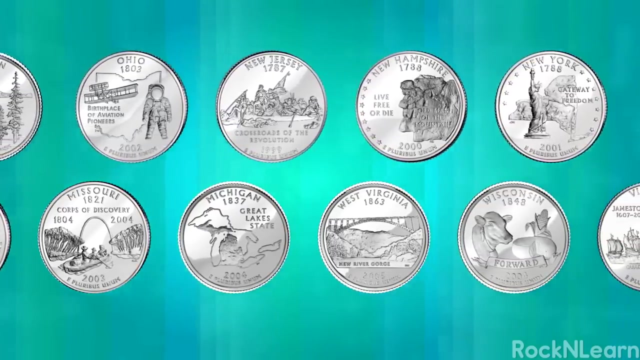 80, 80, 80, 80, 90, 90, 70, 80, 90, 90, 90, 90, 90, 90, 91, 91, 92, 93, 4, 4, 3, 2 1, 1, 2 1. 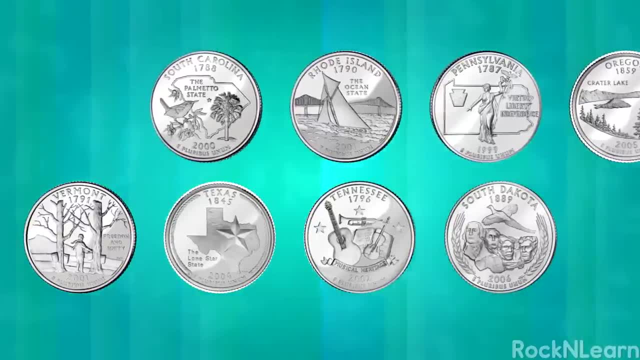 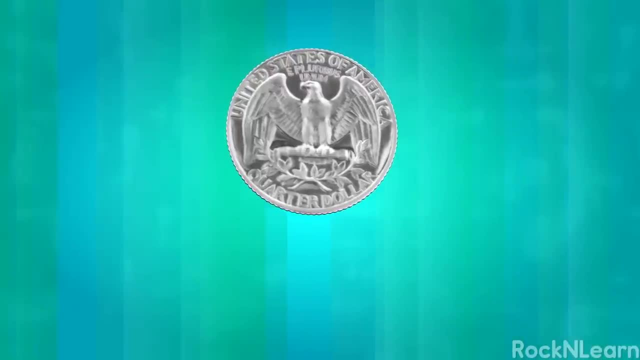 In 2008,. the Mint has changed what is on the back of the quarter. Quarters made before 1999 have an eagle on the back, But all quarters have our first president, George Washington, on the front. I've always thought counting quarters was fun. 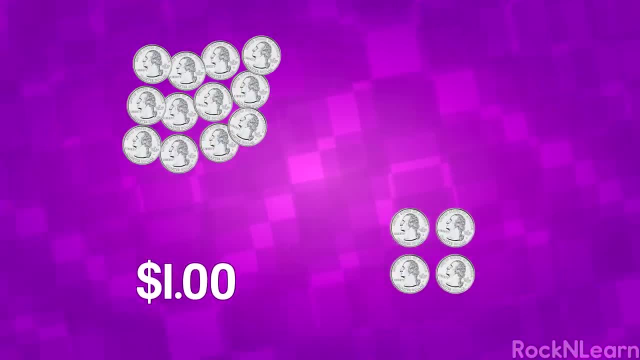 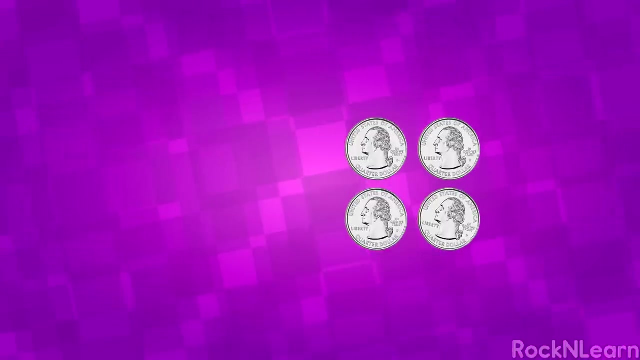 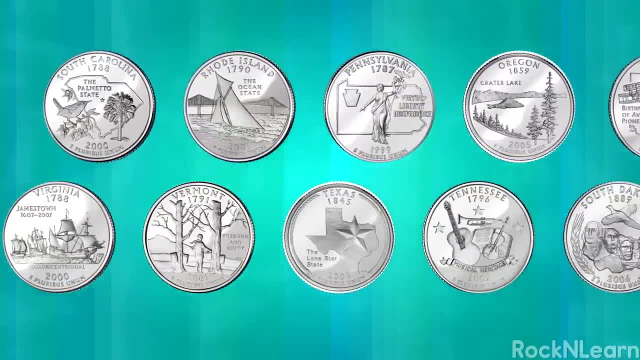 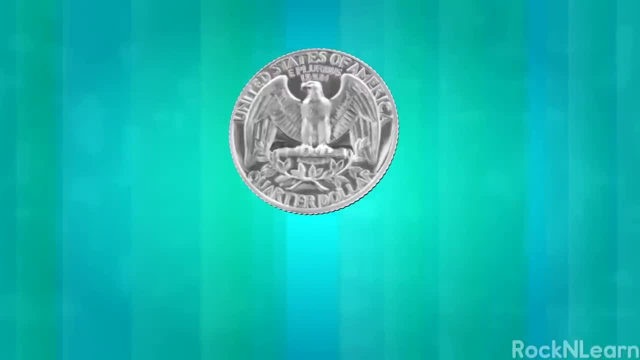 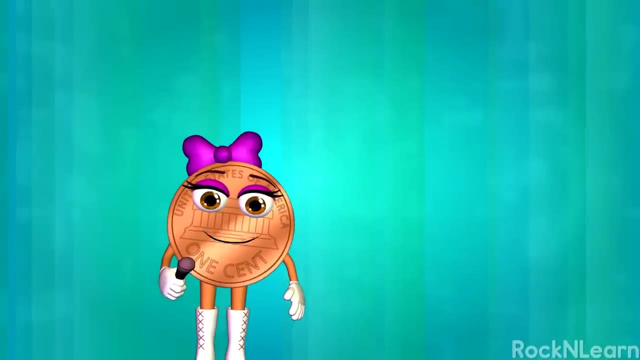 32 In 2008,. the Mint has changed what is on the back of the quarter. Quarters made before 1999 have an eagle on the back, But all quarters have our first president, George Washington, on the front. I've always thought counting quarters was fun. 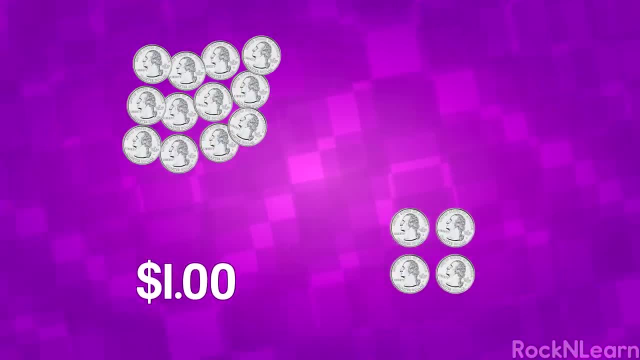 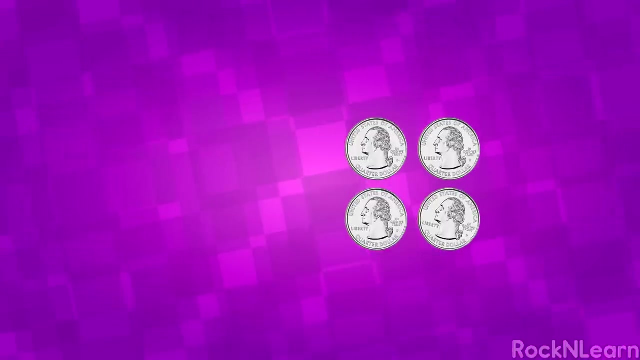 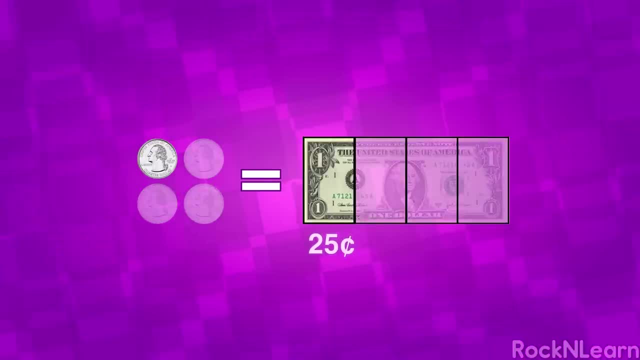 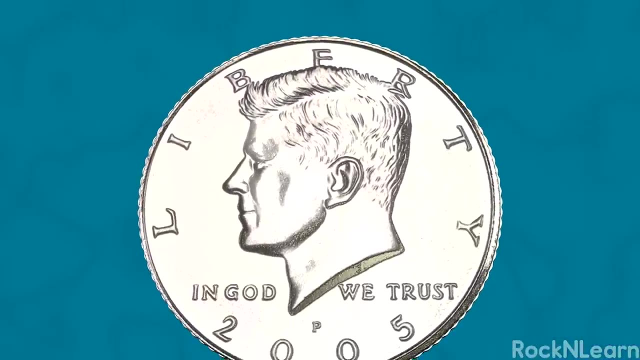 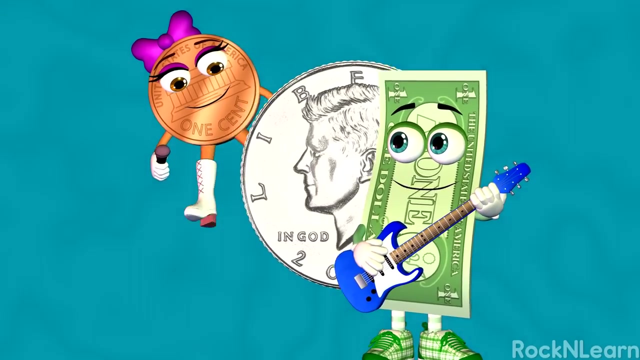 That's because a quarter is one-fourth of a dollar, or twenty-five cents. Look, Bill, this coin is really big. Yes, Penny, it is. And you know what else? Yes, It's worth even more than a quarter. 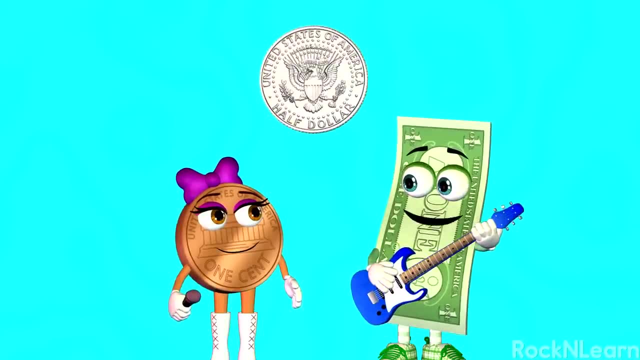 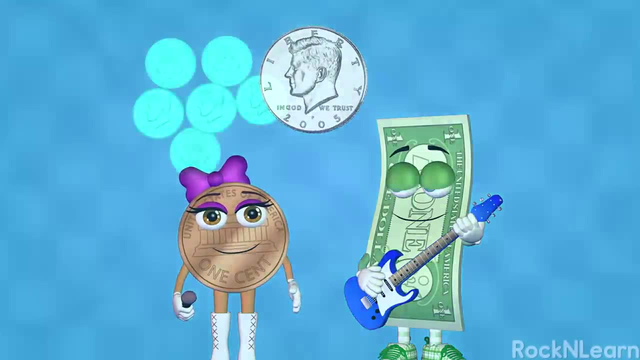 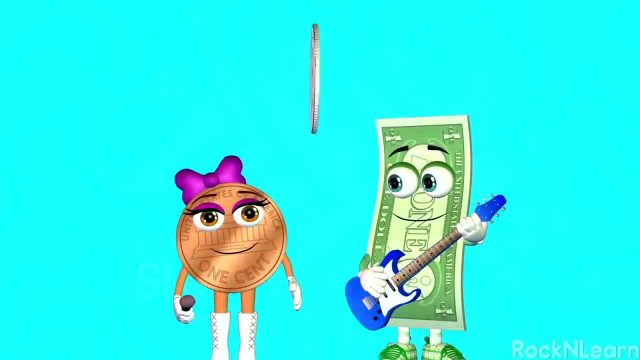 No really. Yes, A half dollar is worth fifty cents, So we only need two of these half dollars to make a dollar. Fifty cents a dollar. Fifty cents a dollar. Fifty cents a dollar. Two half dollars make one dollar. 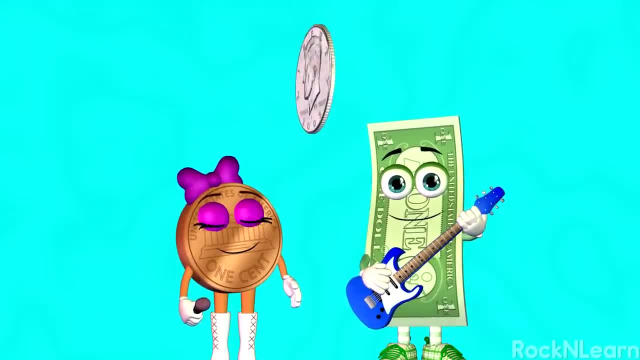 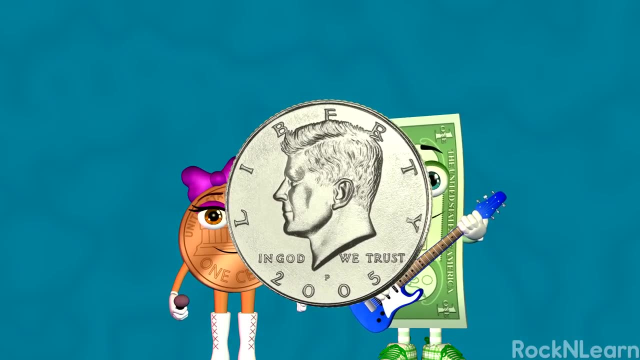 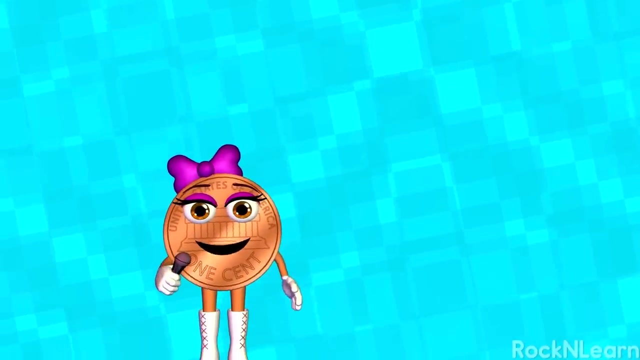 That just makes sense. But we usually don't see many of these half dollars around. They are a lot bigger than quarters And they have John F Kennedy on the front. The next coins are the dollar coins. We have the Sacagawea coin and the Susan B Anthony coin. 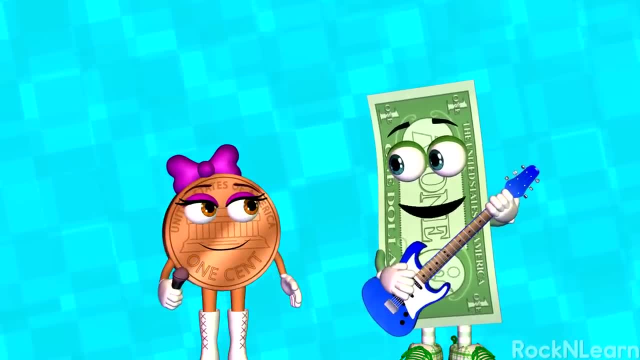 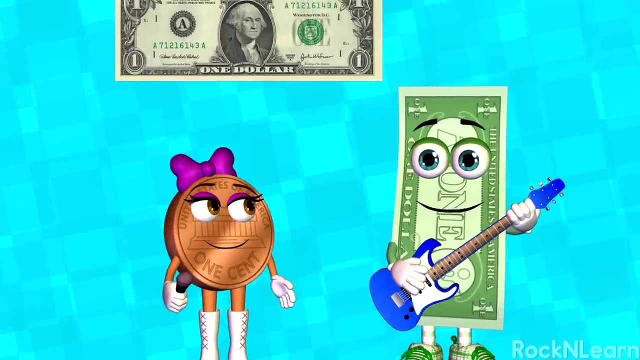 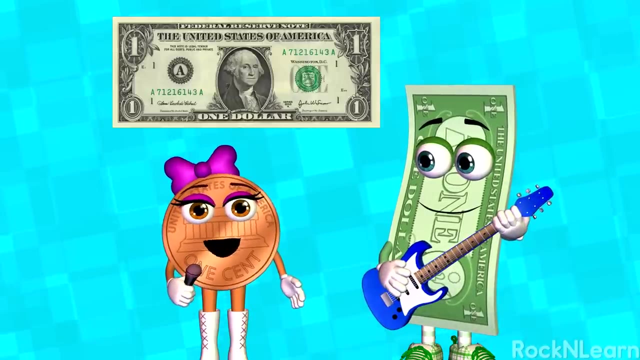 Each is worth one dollar, just like the presidential dollar coins. But the dollar also comes in paper form: the dollar bill, The dollar bill, The dollar bill. Like coins, The way paper money looks changes from time to time, But don't worry. 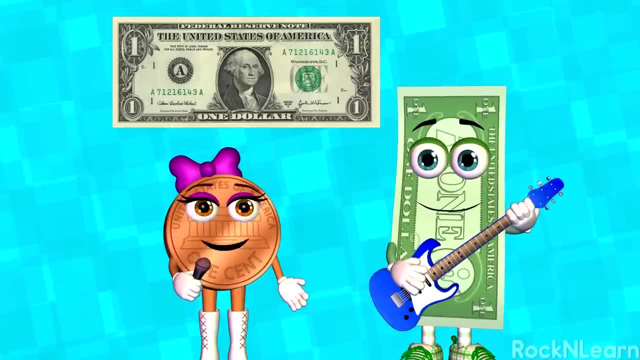 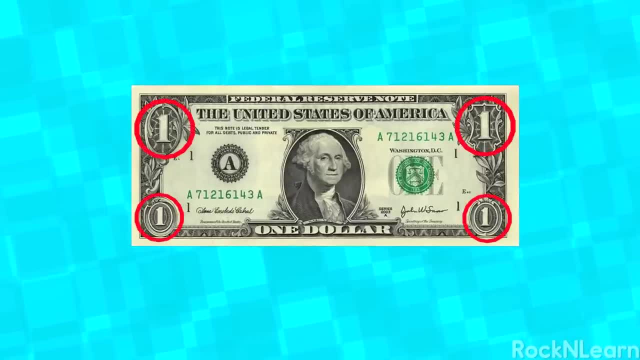 You'll be able to tell how much each bill is worth from the number printed on it. Look at this one dollar bill to see what we mean. You will see both the number one and the word one printed on the bill. We have several different kinds of bills in the US. 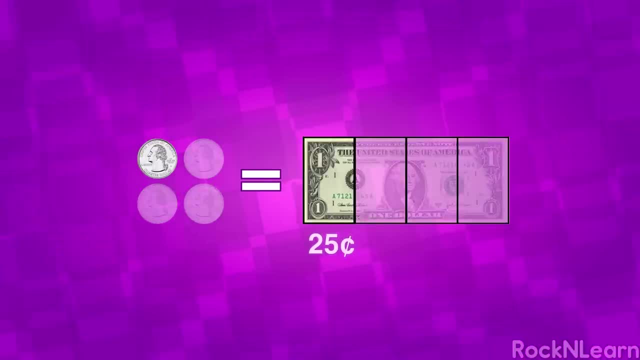 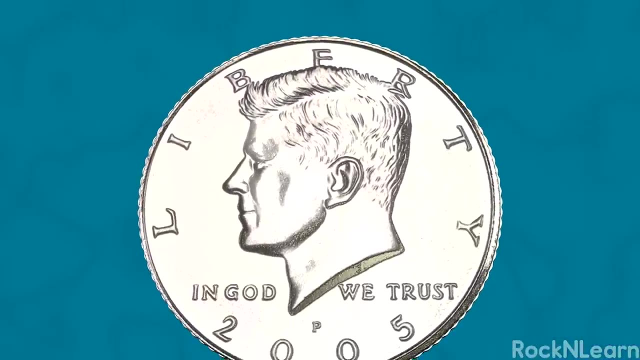 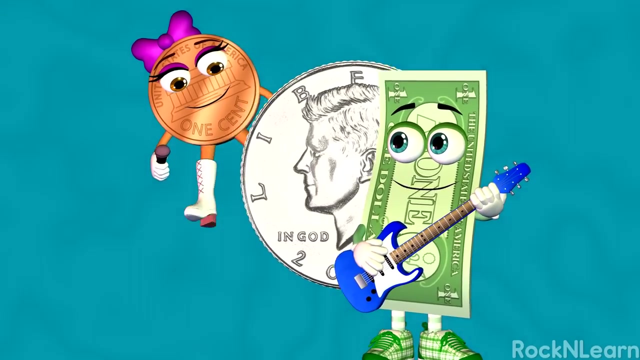 That's because a quarter is one-fourth of a dollar, or twenty-five cents. Look, Bill, this coin is really big. Yes, Penny, it is. And you know what else? Yes, It's worth even more than a quarter. 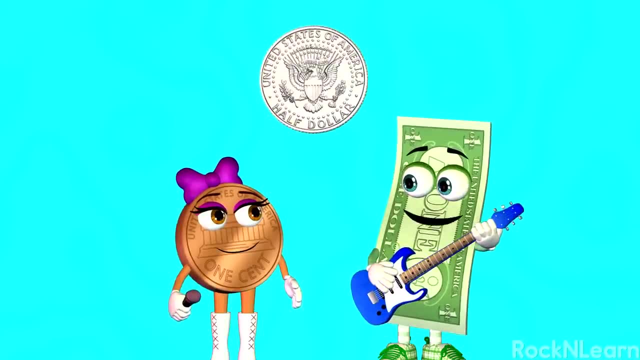 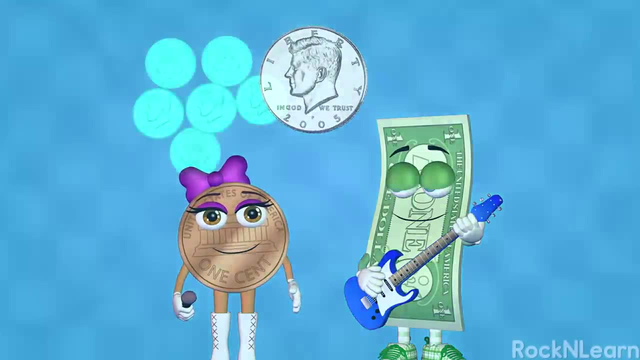 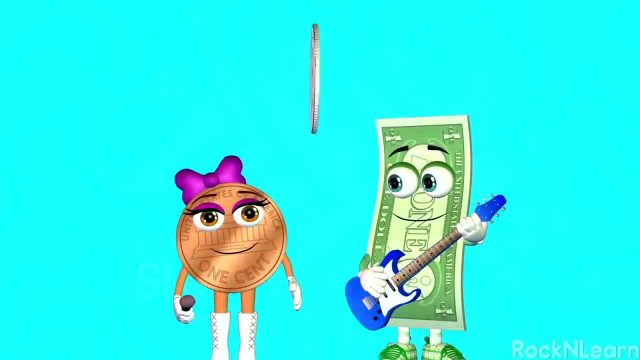 No really. Yes, A half dollar is worth fifty cents, So we only need two of these half dollars to make a dollar. Fifty cents a dollar. Fifty cents a dollar. Fifty cents a dollar. Two half dollars make one dollar. 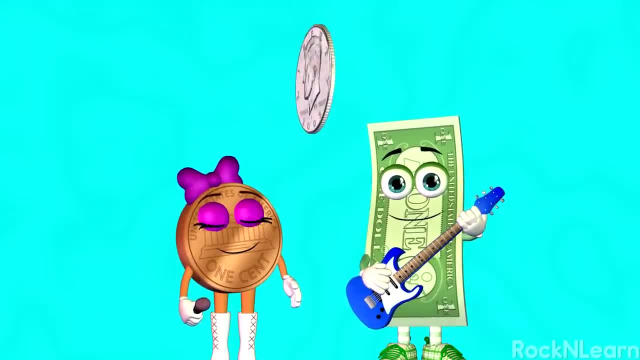 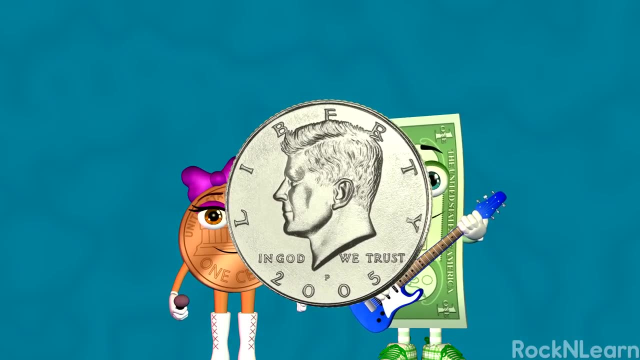 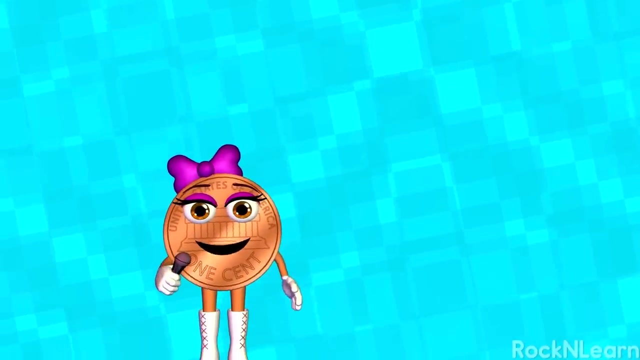 That just makes sense. But we usually don't see many of these half dollars around. They are a lot bigger than quarters And they have John F Kennedy on the front. The next coins are the dollar coins. We have the Sacagawea coin and the Susan B Anthony coin. 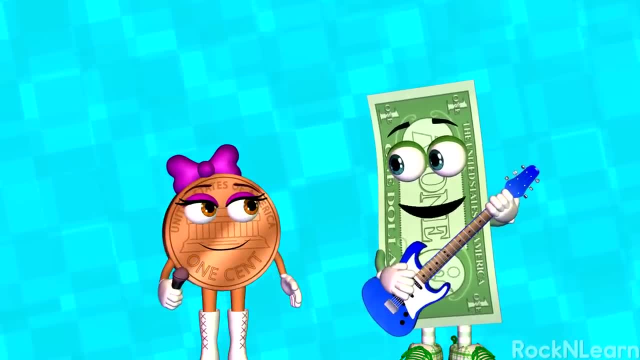 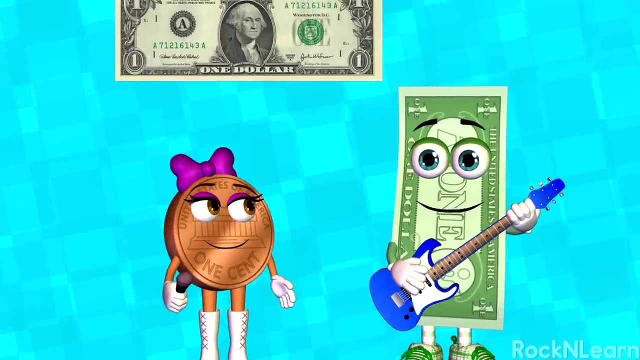 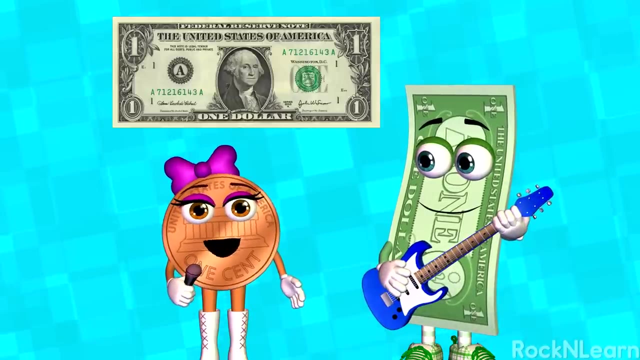 Each is worth one dollar, just like the presidential dollar coins. But the dollar also comes in paper form: the dollar bill, The dollar bill, The dollar bill. Like coins, The way paper money looks changes from time to time, But don't worry. 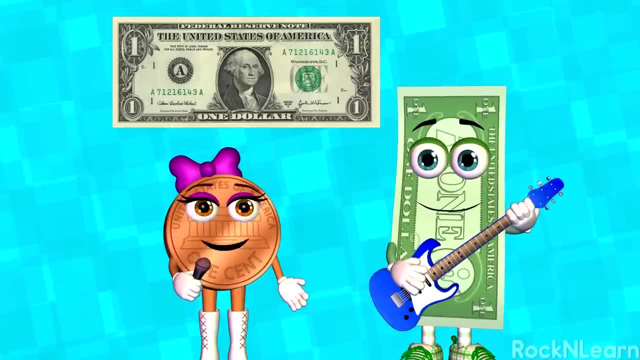 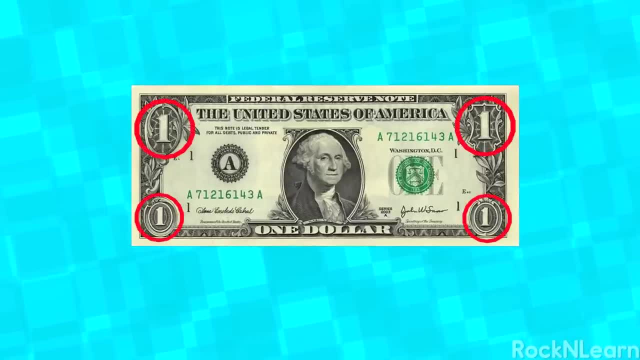 You'll be able to tell how much each bill is worth from the number printed on it. Look at this one dollar bill to see what we mean. You will see both the number one and the word one printed on the bill. We have several different kinds of bills in the US. 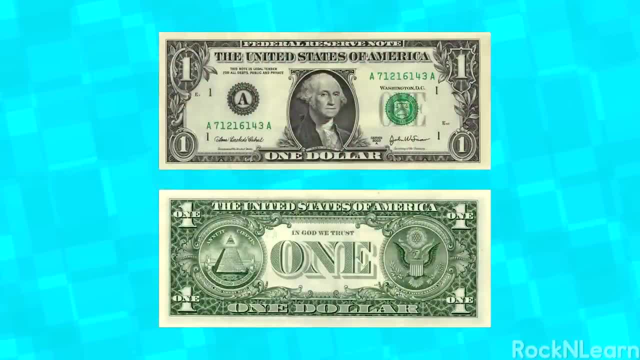 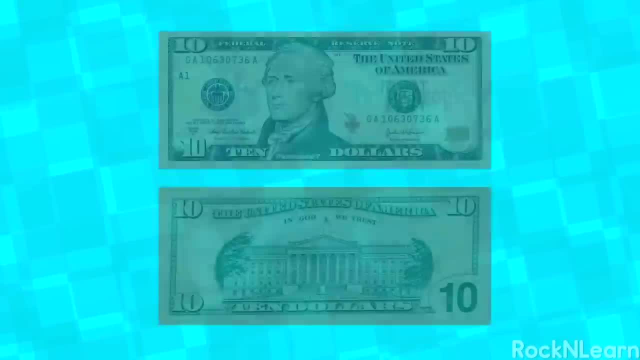 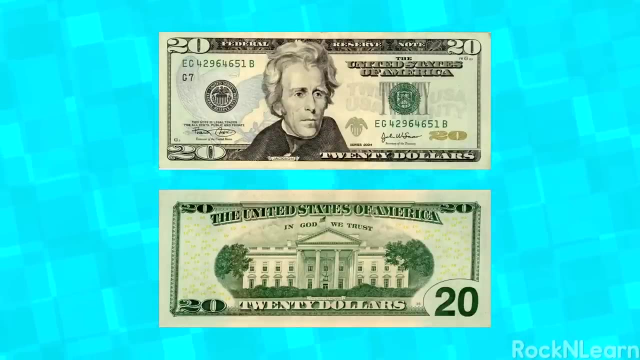 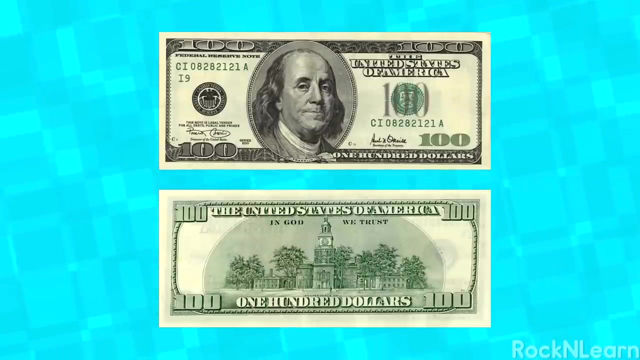 The most common are Ones, Fives, Tens, Twenties, Fifties And one hundreds. Wow, Um, may I keep one of those one hundreds, Just so I can remember what they look like. Um, let me see. 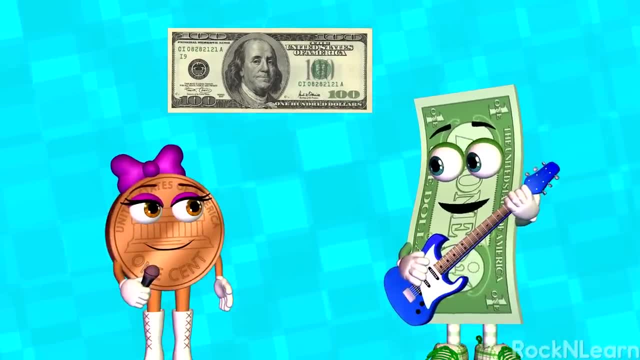 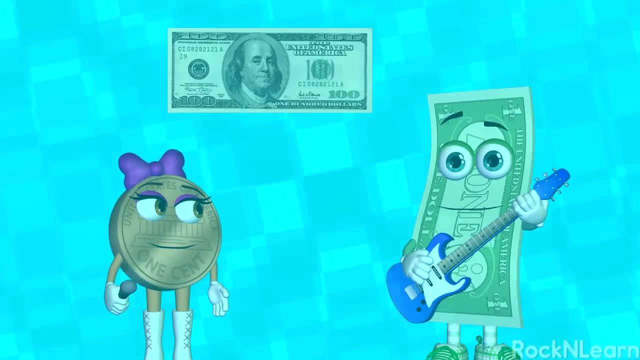 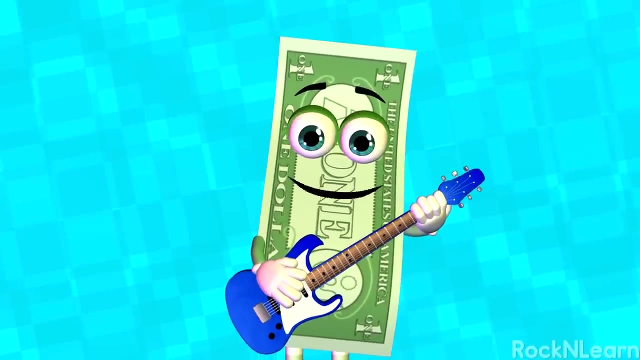 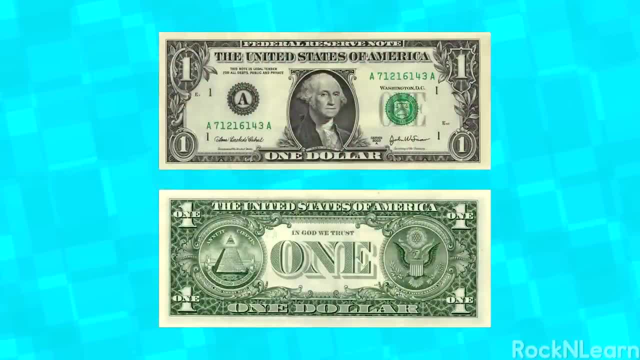 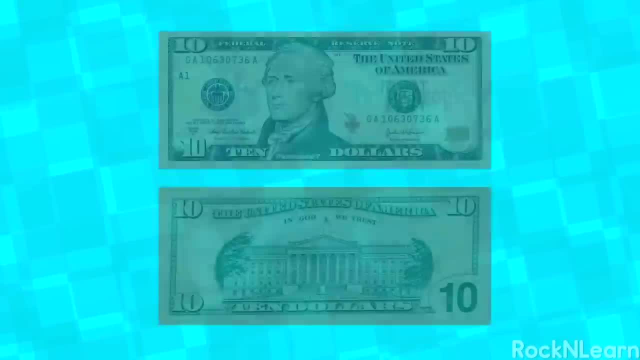 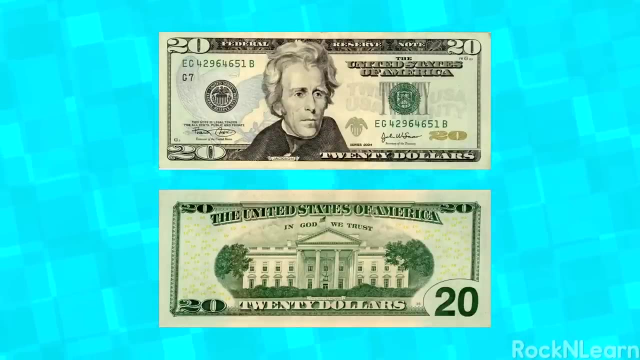 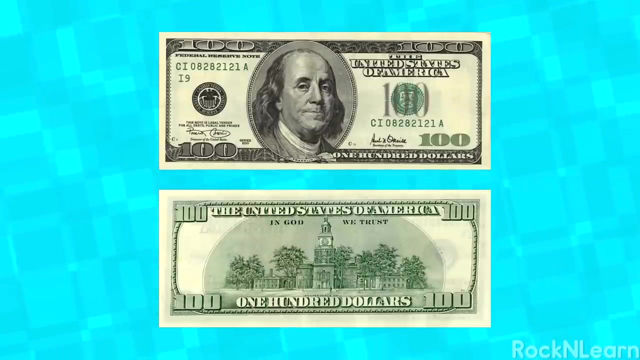 The most common are Ones, Fives, Tens, Twenties, Fifties And one hundreds. Wow, Um, may I keep one of those one hundreds, Just so I can remember what they look like. Um, let me see. 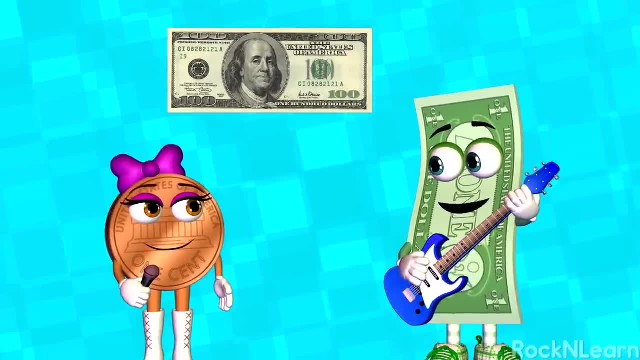 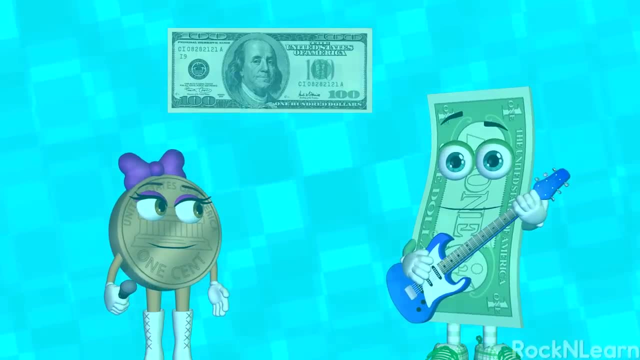 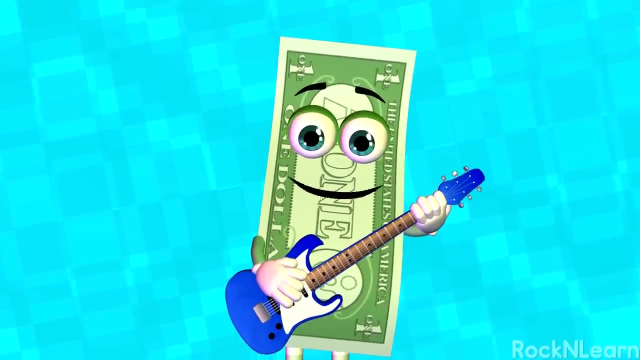 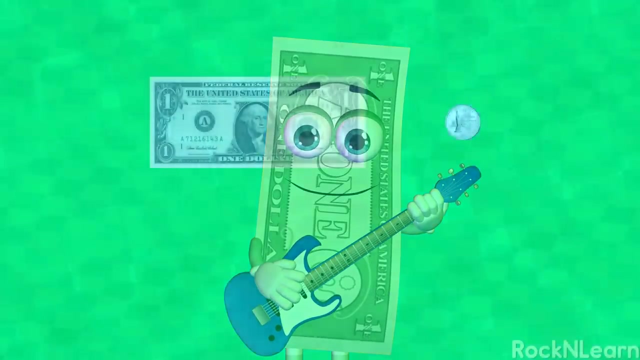 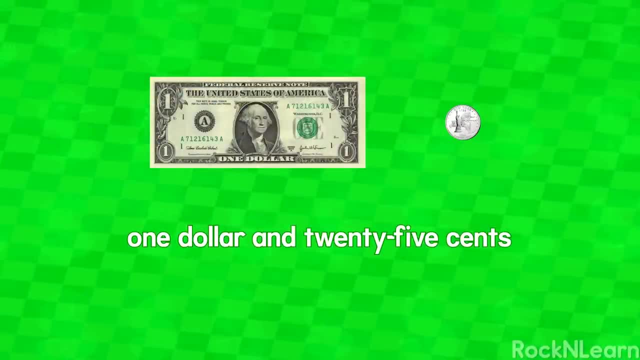 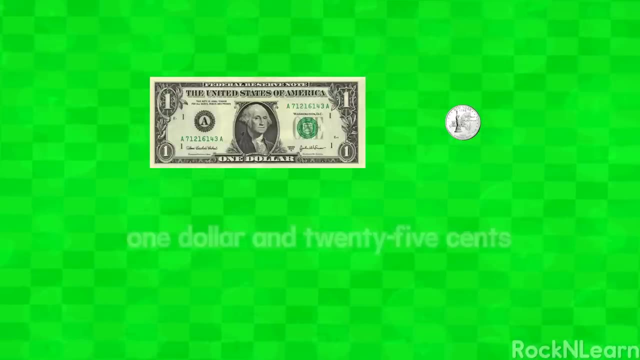 One: We can write every word, put the dollars, first The word and then the cents, So this would be one dollar and 25 cents. We use this way when we write checks. Two: We can use the dollar sign and decimal. 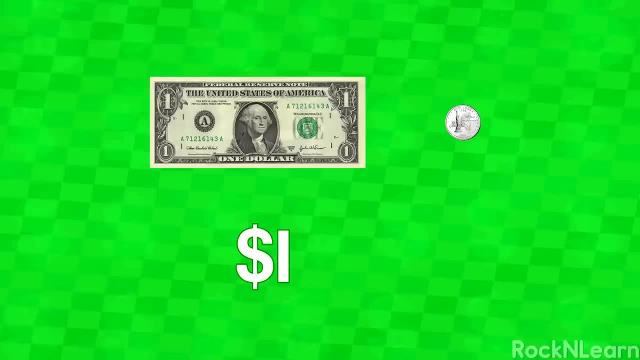 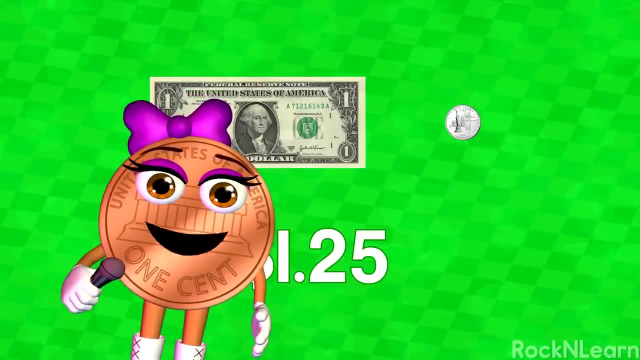 Write the dollar sign and only the decimal Two. put the number of dollars after it, then put the decimal point with the number of cents after that. this is the way you see prices written most often when we write money. this way we show the sense in two digits to the right of the decimal point. 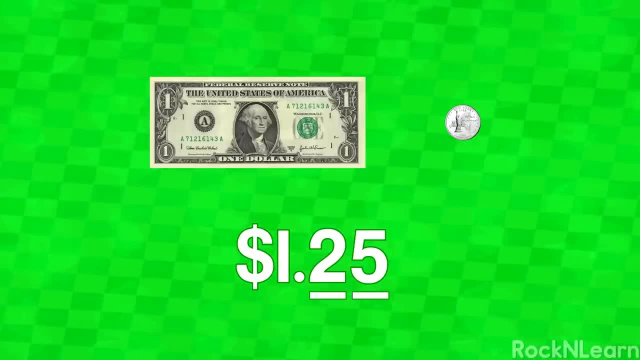 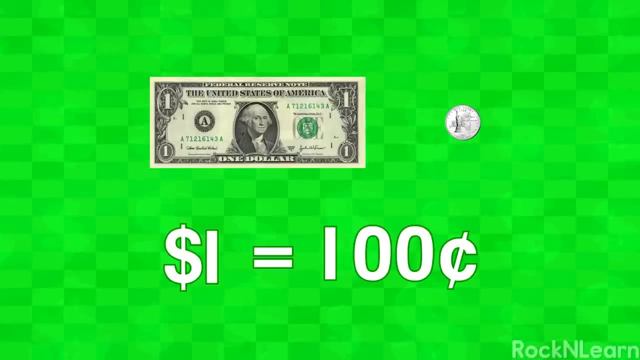 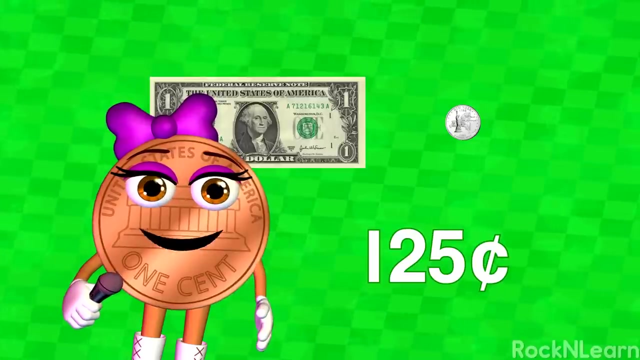 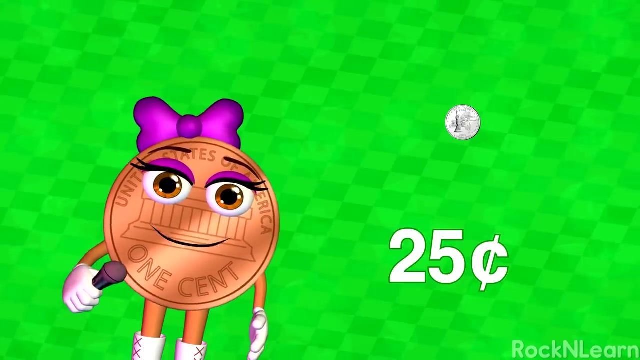 because they are one hundredths of a dollar. three, we can use the cent sign because a dollar equals 100 cents. we write a dollar 25 as 125 cents with the cent sign after it. but this way of writing money is usually used when writing amounts less than one dollar. I've seen it used a lot at garage sales. 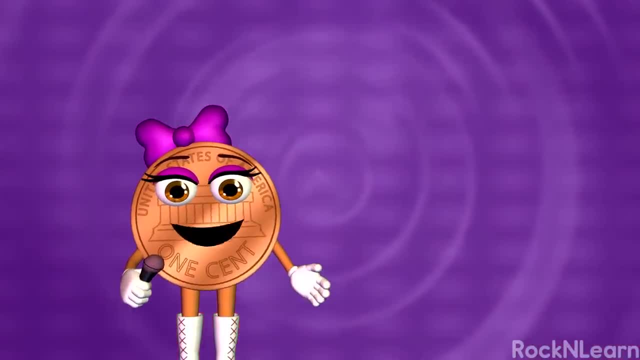 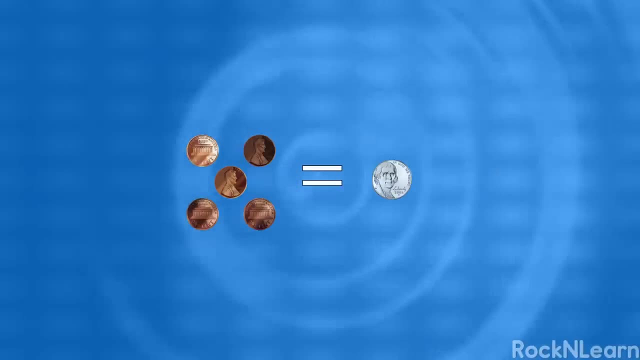 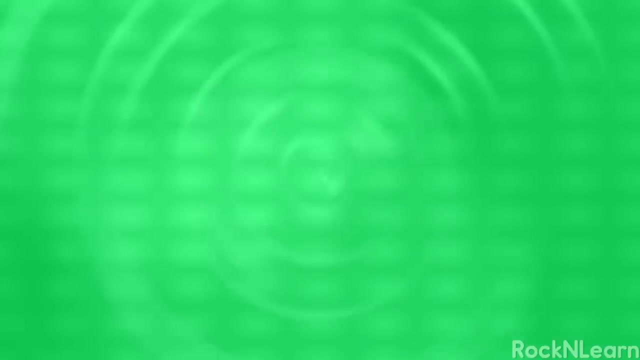 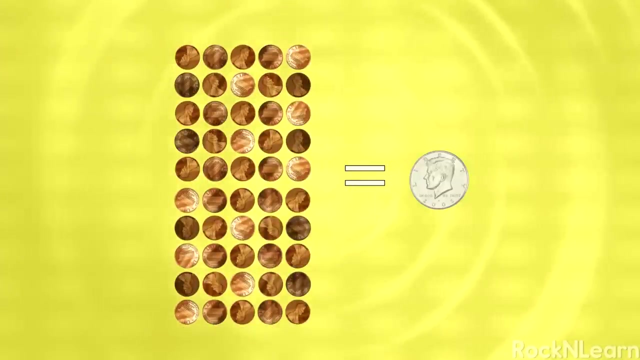 when counting change at a garage sale or anywhere. it's good to know about coin combination money nations. it takes five pennies to equal a nickel, 10 pennies to equal a dime, 25 pennies to equal a quarter, 50 pennies to equal a half dollar and 100 pennies to 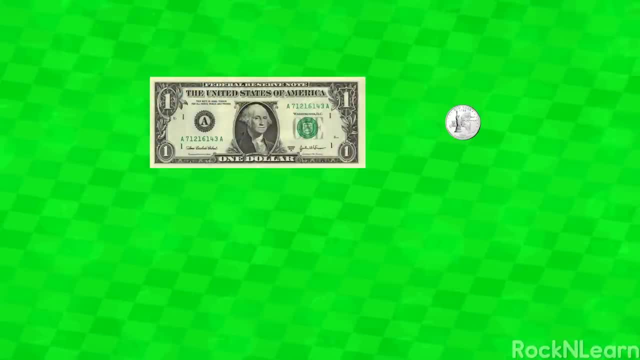 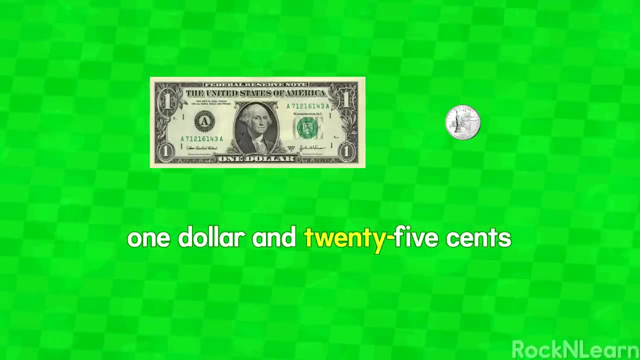 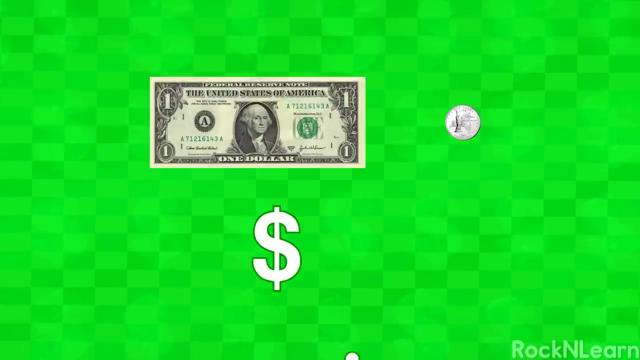 One: We can write every word out putting the dollars, first the word and then the cents. So this would be One dollar and twenty-five cents. We use this way when we write checks. Two: We can use a dollar sign and decimal. 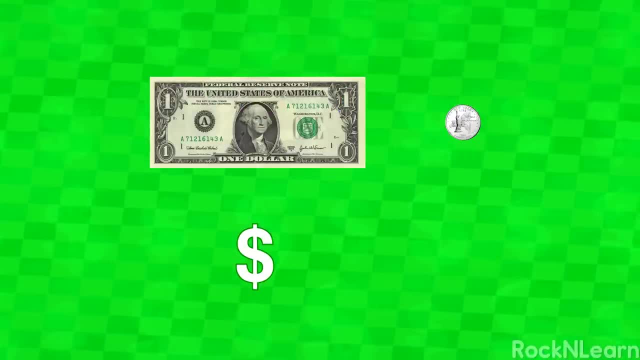 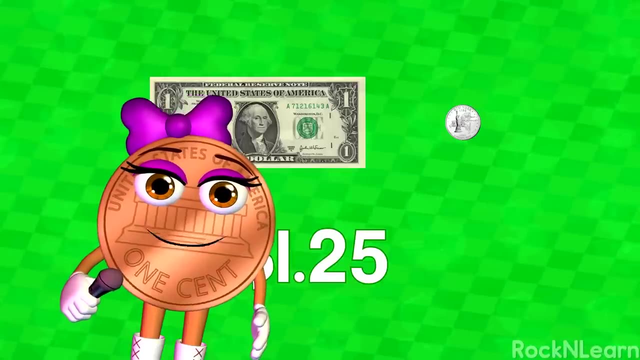 Write the dollar sign. We write it like that and put the number of dollars after it. Then put the decimal point with the number of cents after that. This is the way you see prices written most often When we write money this way. 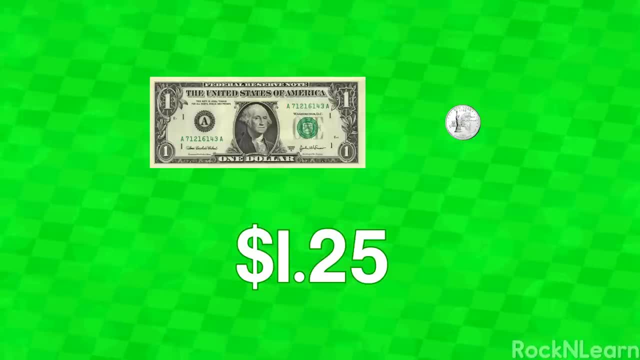 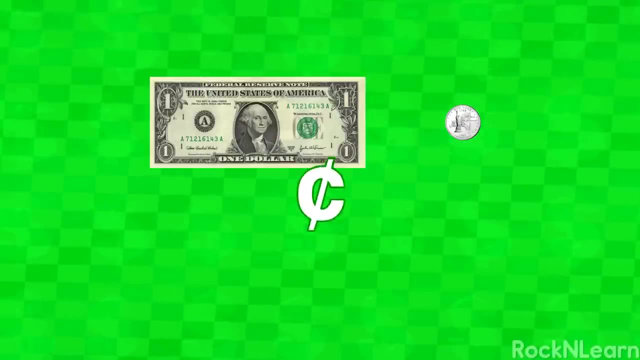 we show the cents in two digits to the right of the decimal point because they are one hundredths of a dollar Three. We can use the cent sign Because a dollar equals one hundred cents. we write a dollar twenty-five as one hundred twenty-five cents. 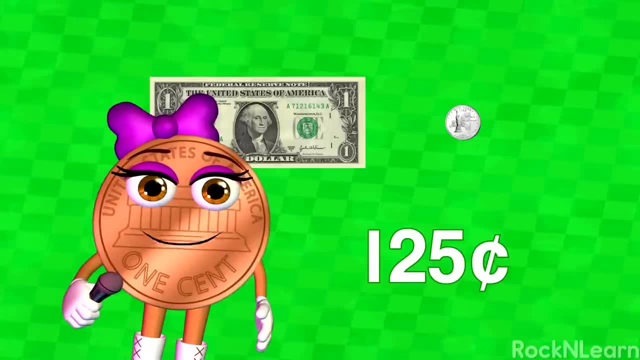 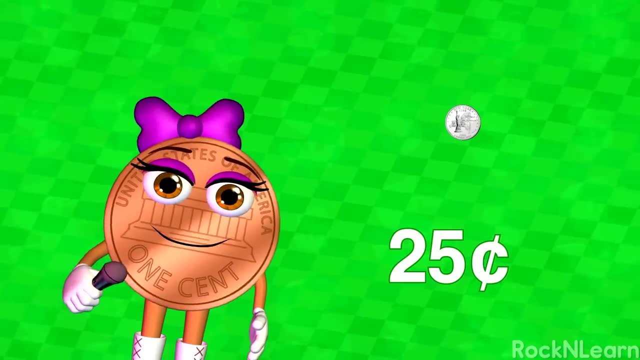 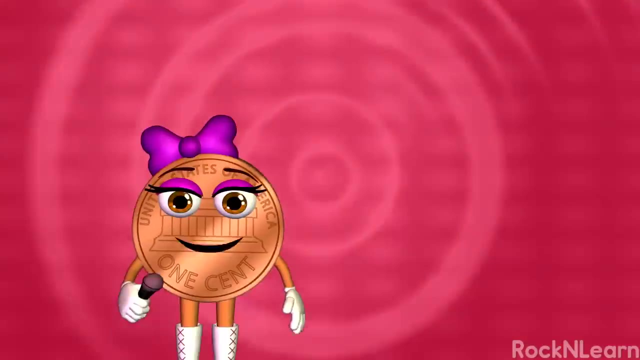 with the cent sign after it. But this way of writing money is usually used when writing amounts less than one dollar. I've seen it used a lot at garage sales. When counting change at a garage sale or anywhere, it's good to know about coin combinations. It takes five pennies to equal a nickel, ten pennies to equal a dime, twenty-five pennies to equal a quarter, fifty pennies to equal a half dollar and one hundred pennies to equal a dollar. That's a lot of pennies, Penny. 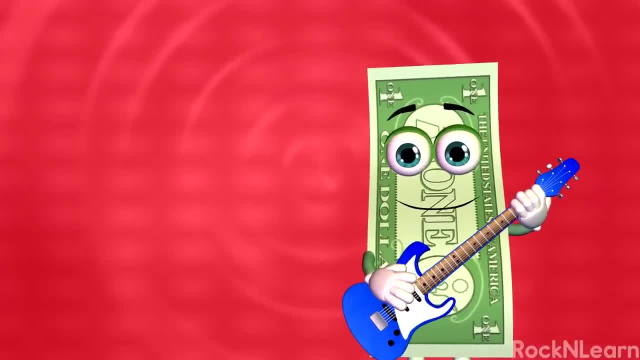 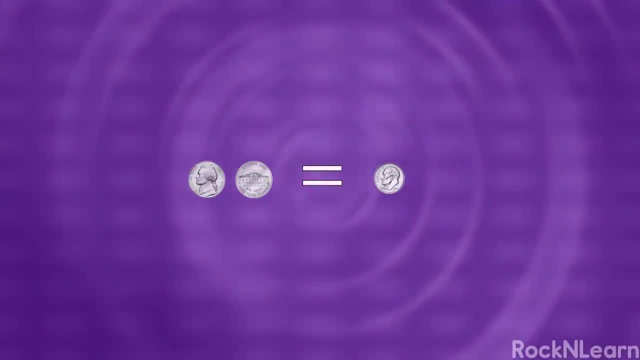 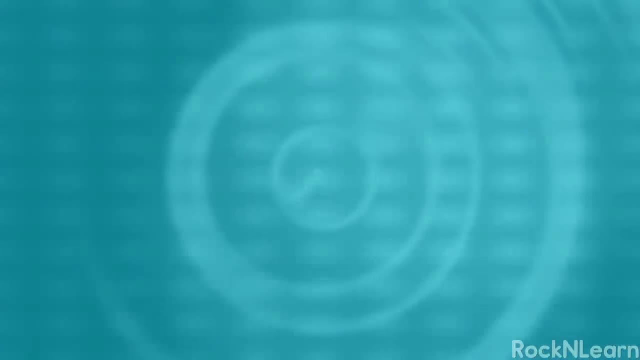 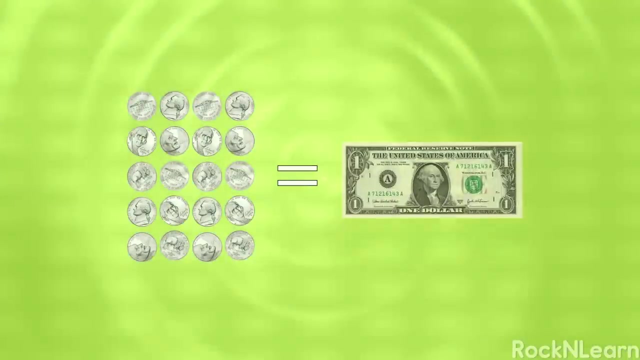 I like having coins that are worth more, like the nickel, because you don't have to carry as many. It takes two nickels to equal a dime, five nickels to equal a quarter, ten nickels to equal a half dollar and twenty nickels to equal a dollar. 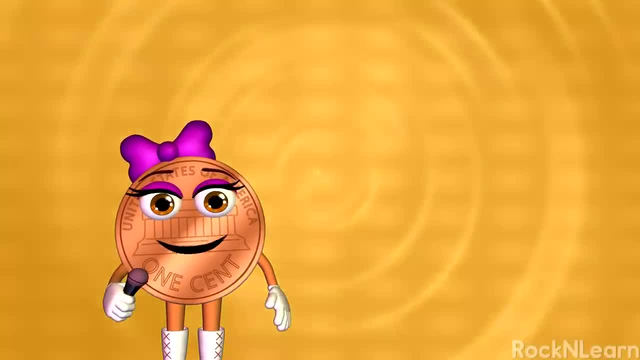 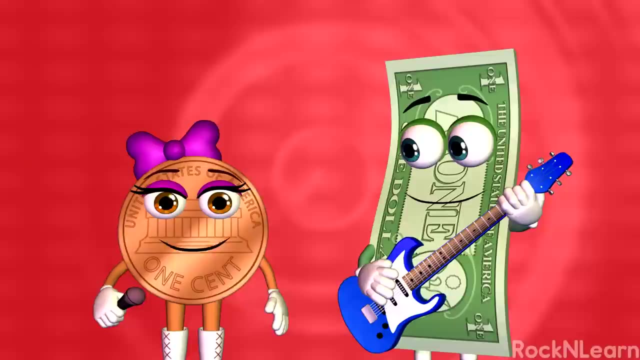 Dimes are pretty cool because they're worth more and they're smaller. However, they are kind of tricky. What do you mean dimes are tricky? Well, we can't use only dimes to equal a quarter. We need two dimes and a nickel to equal a quarter. 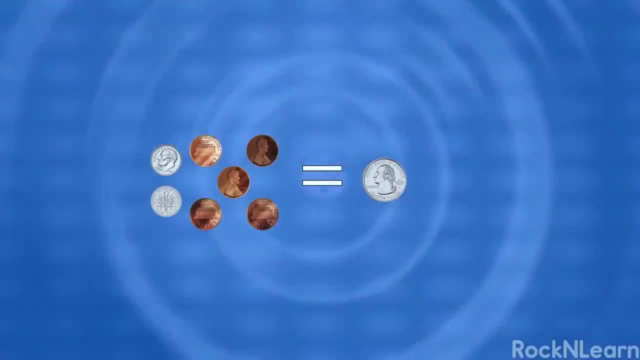 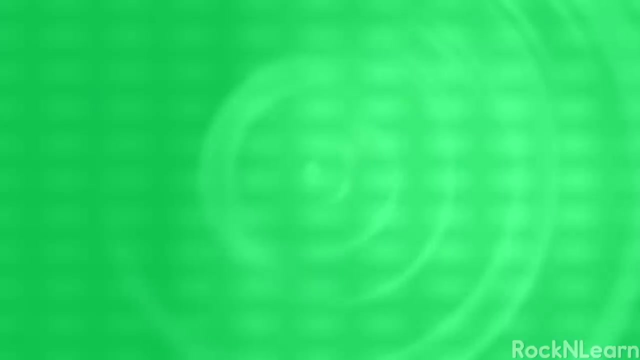 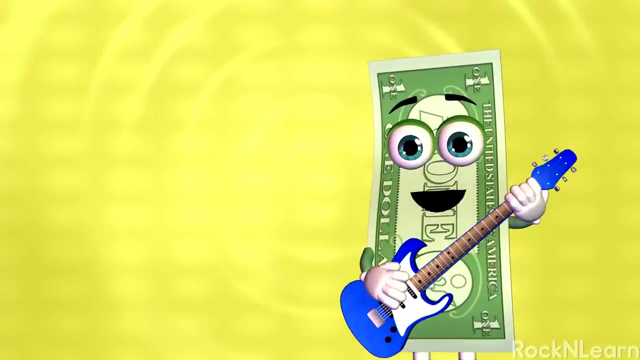 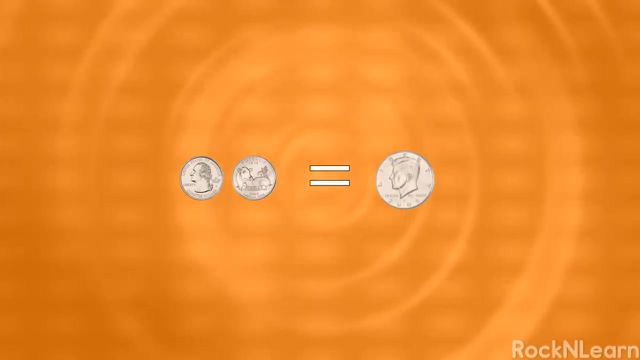 Or two dimes and five pennies. That's right, And it takes five dimes to equal a half dollar and ten dimes to equal a dollar. Quarters are my favorite coins because there are so many different designs. It takes two quarters to equal a half dollar. 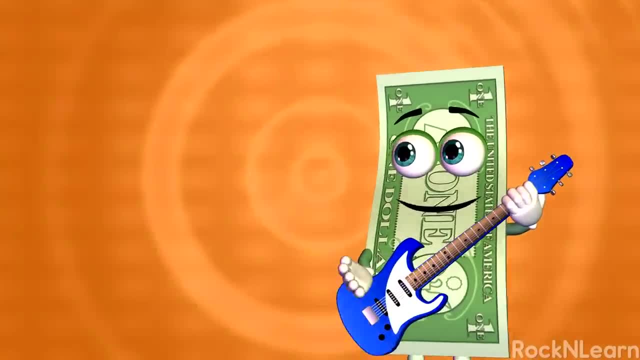 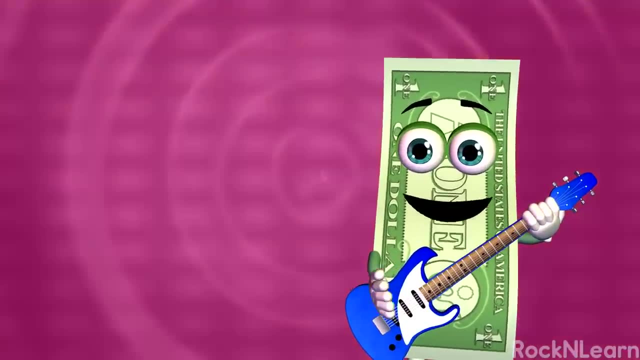 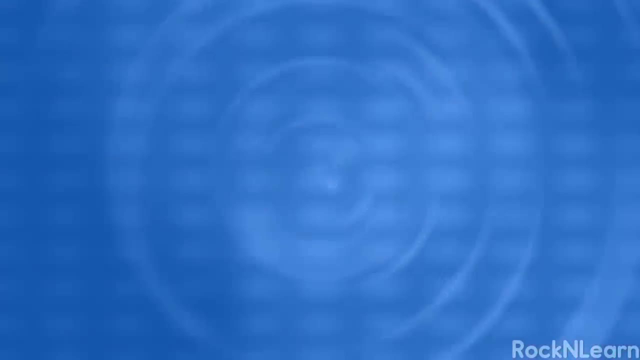 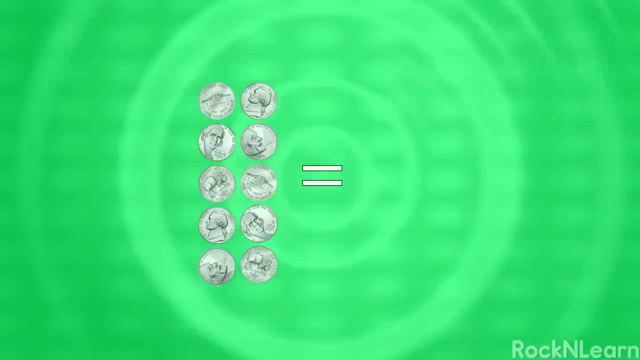 equal a dollar. that's a lot of pennies penny. I like having coins that are worth more, like the nickel, because you don't have to carry as many. it takes two nickels to equal a dime, five nickels to equal a quarter, 10 nickels to equal a half dollar. 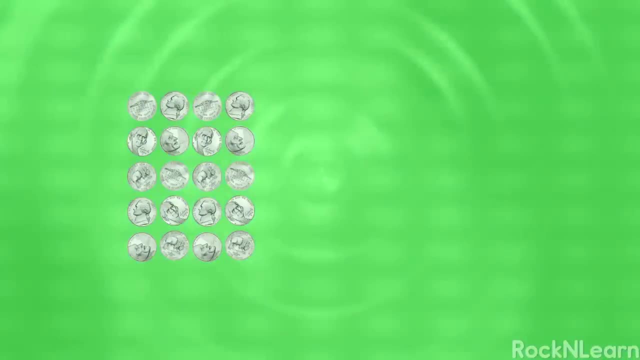 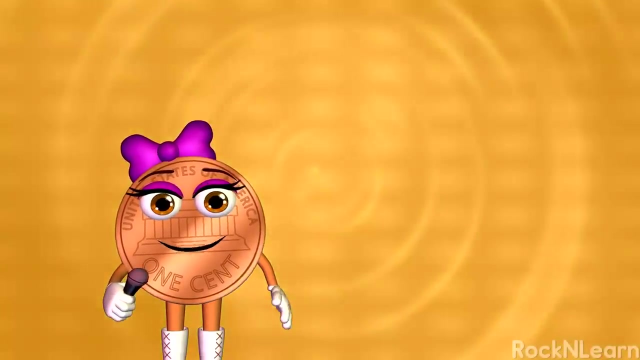 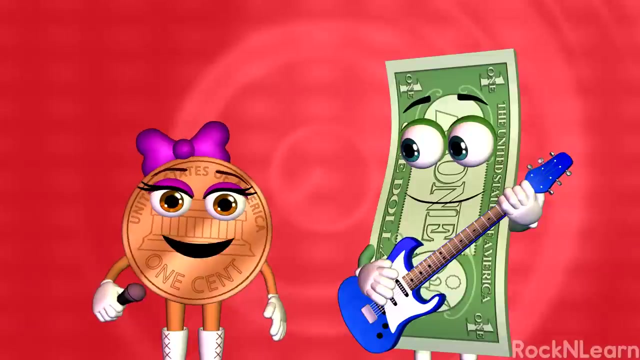 and 20 nickels to equal a dollar. dimes are pretty cool because they're worth more and they're smaller. however, you have to be careful when you're writing money. however, they are kind of tricky. what do you mean? dimes are tricky. well, we can't. 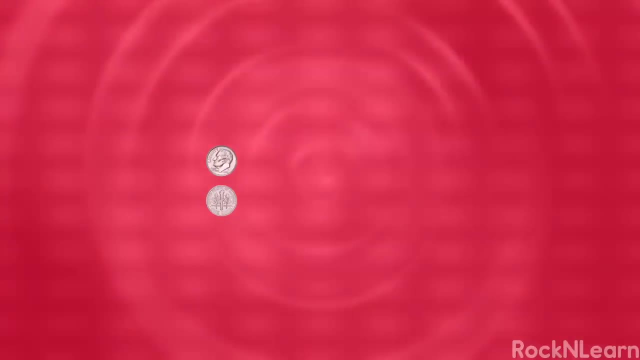 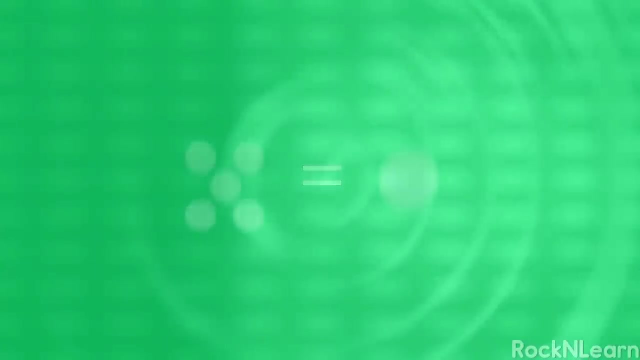 use only dimes to equal a quarter. we need two dimes and a nickel to equal a quarter. for two dimes and five pennies, lets wait. and it takes 5 times to equal a half-dollar n. 10 times equal dollar ENC either. this just happens every one, for example in your past life. it's almost like a coin is written kind with capital D on it. 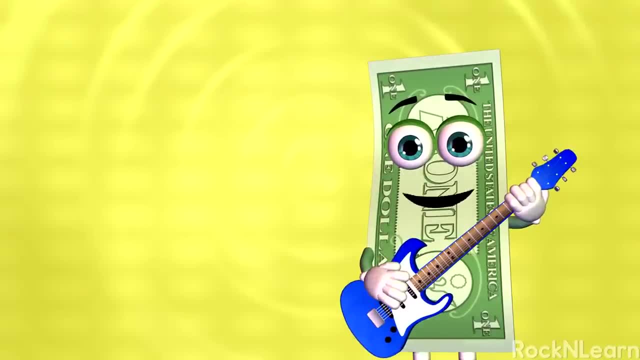 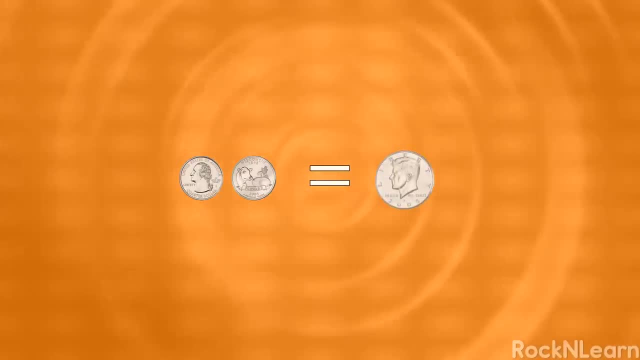 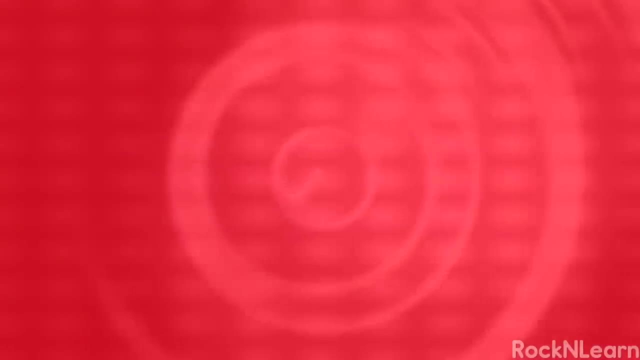 one with an ört or the number of years. aereo is round, quarter, 20area either. Quarters are my favorite coins because there are so many different designs. It takes two quarters to equal a half dollar and four quarters to equal a dollar. Half dollars are hard to find, but you only need two of them to equal a dollar. 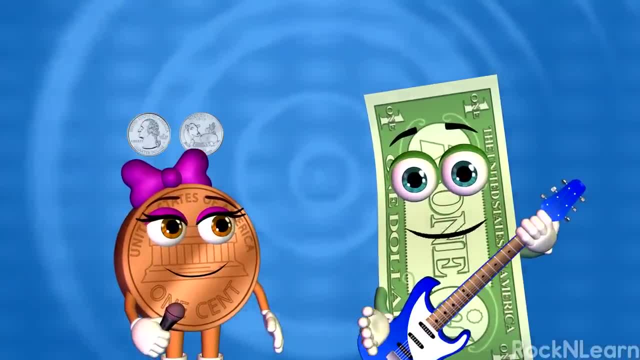 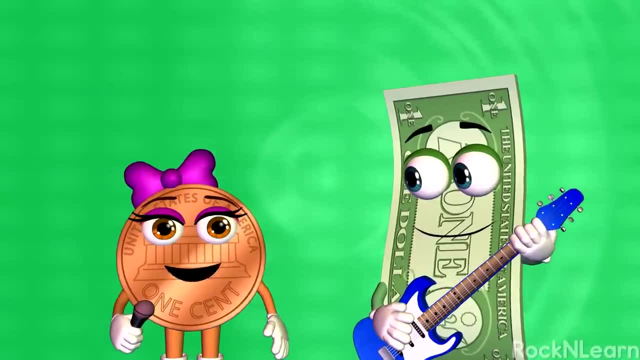 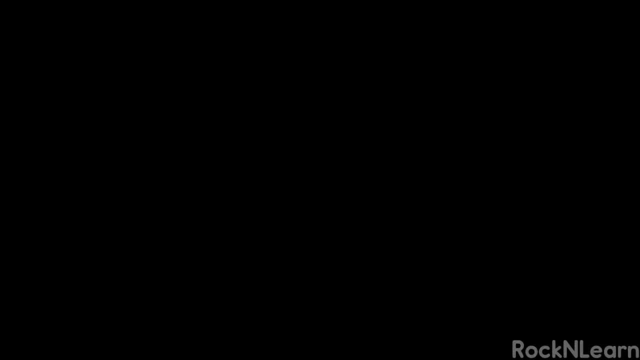 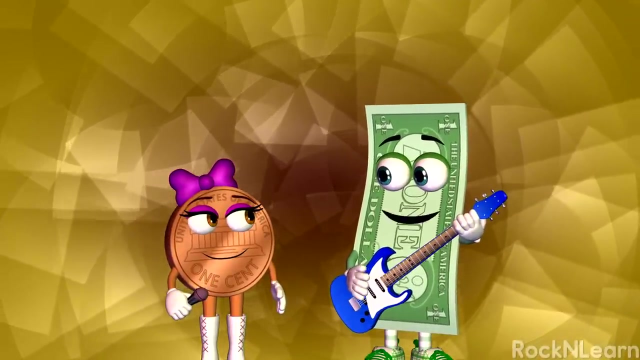 Since you don't see them very often, you might have to put two quarters, with the half dollar to equal a dollar. It's fun making coin combinations. The more you practice, the better you get. Whenever I empty my piggy bank, the first thing I do is separate the coins so that I have all the pennies in one pile. 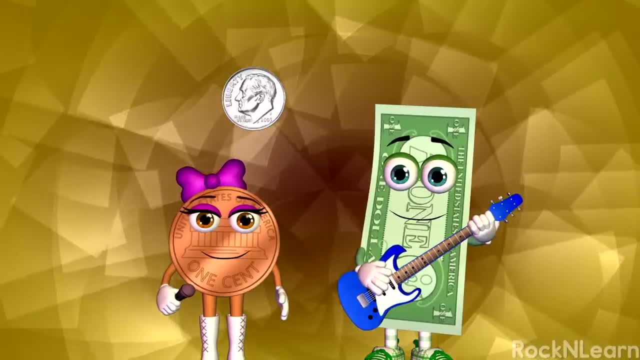 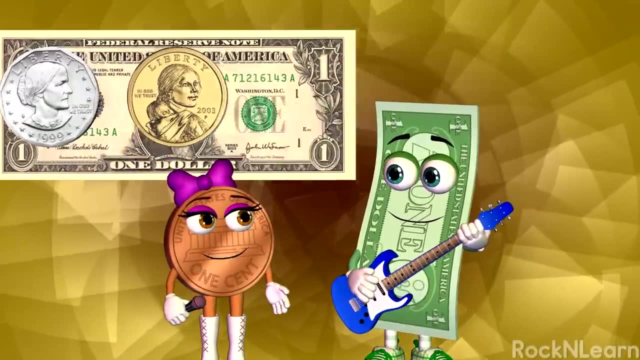 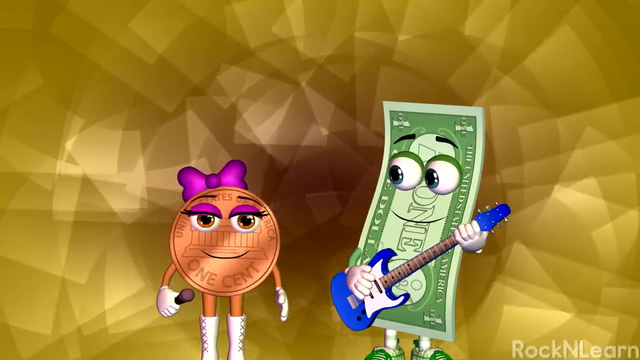 all the nickels in another, the dimes in another, then the quarters, then the half dollars and finally the dollar coins and bills. That's it. That makes it easier to count how much money you have. Start with the large coins and use. skip counting to put all of the coins into dollar piles. 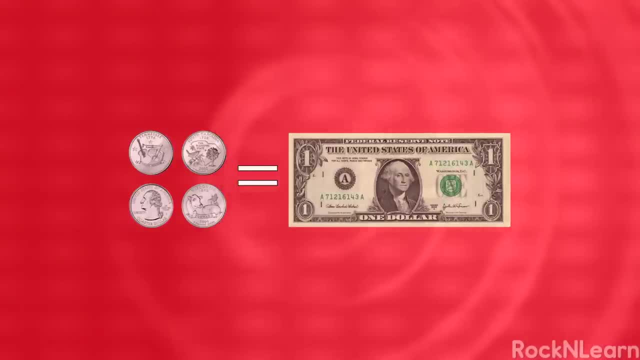 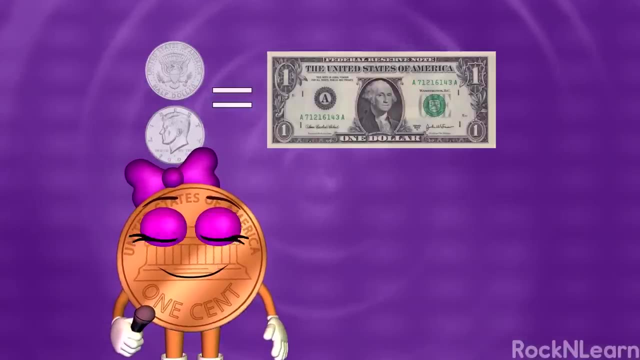 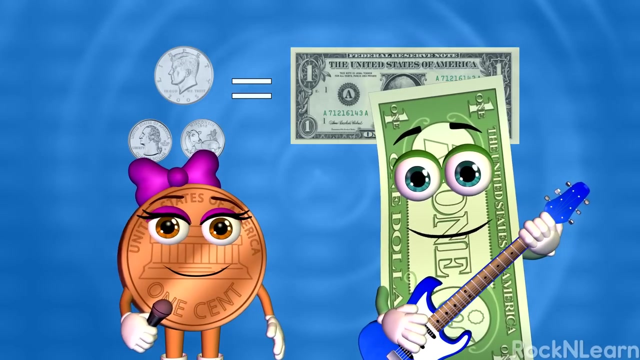 and four quarters to equal a dollar. Half dollars are hard to find, but you only need two of them to equal a dollar. Since you don't see them very often, you might have to put two quarters with the half dollar to equal a dollar. 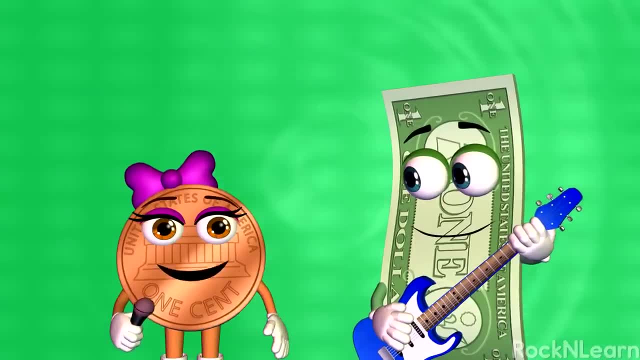 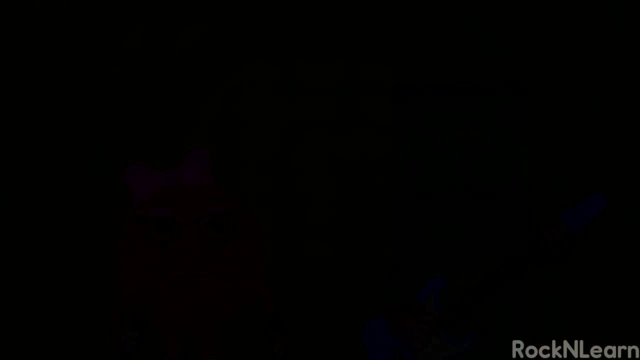 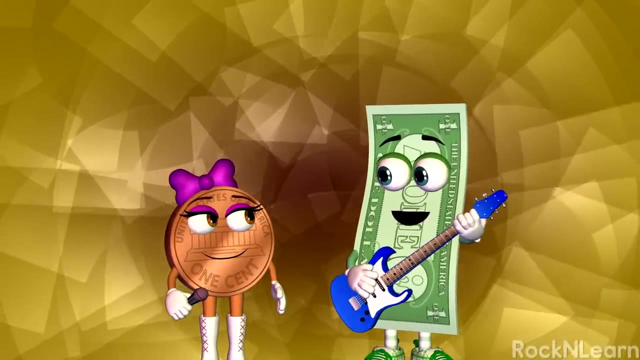 It's fun making coin combinations. The more you practice, the better you get. Whenever I empty my piggy bank, the first thing I do is separate the coins so that I have all the pennies in one pile, all the nickels in another. 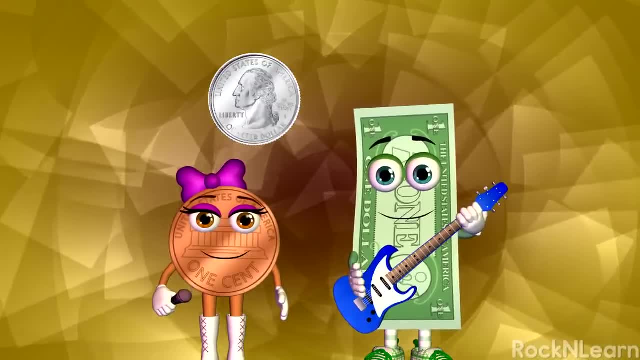 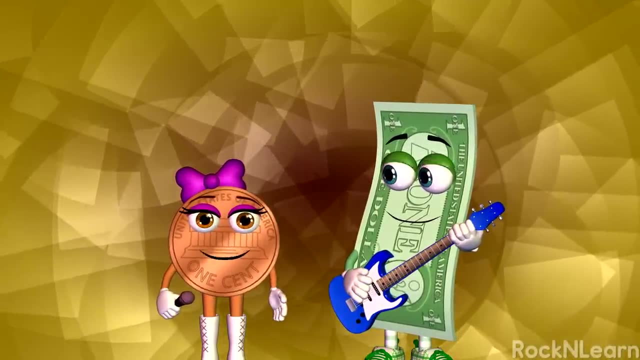 the dimes in another, then the quarters, then the half dollars and finally the dollar coins and bills. That makes it easier to count how much money you have. Start with the large coins and use. skip counting to put all of the coins into dollar piles. 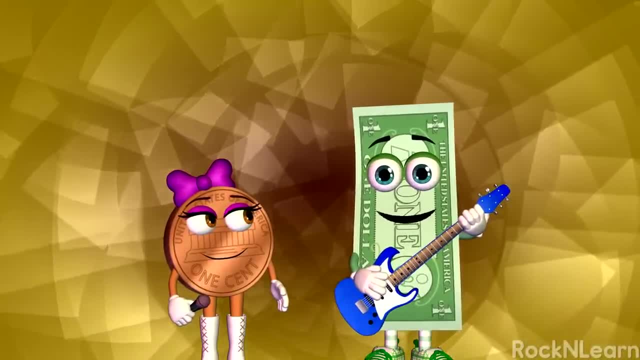 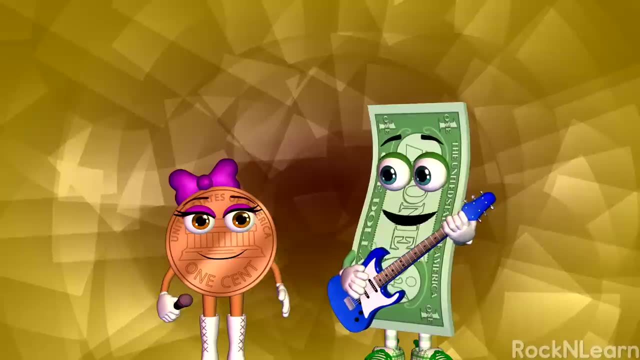 Sometimes I don't have the right number of coins to do the skip counting all the way up to a dollar, so I just use some of the smaller coins to finish up the dollar. Hey, Penny, why don't we count the money in your piggy bank? 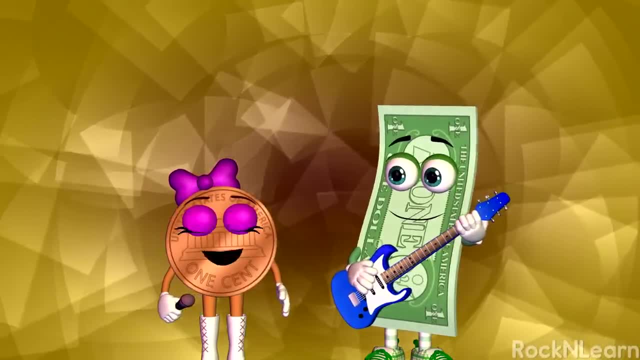 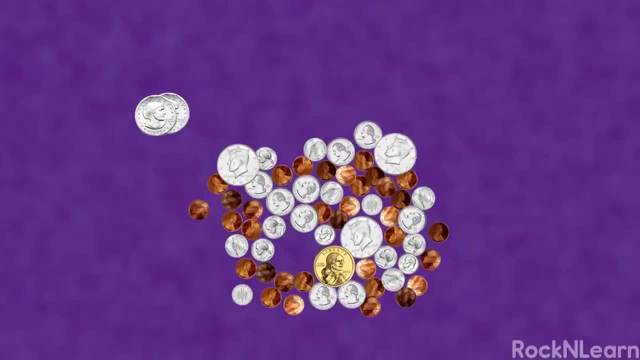 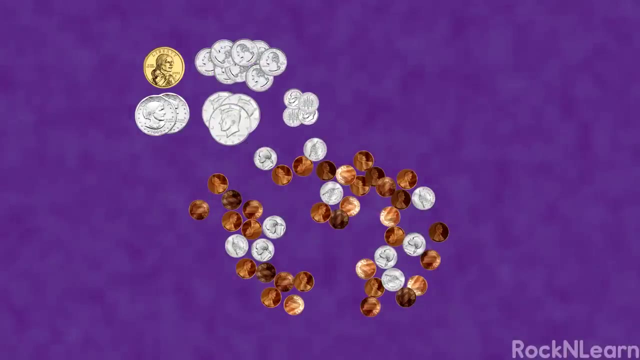 Maybe we can get our speaker fixed. Okay, first we'll separate the coins. Here are two Susan B Anthony dollars, one Sacagawea dollar, three half dollars, nine quarters, four dimes, ten nickels and a whole pile of pennies. 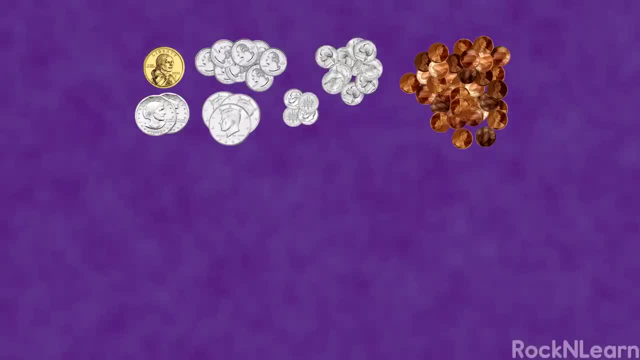 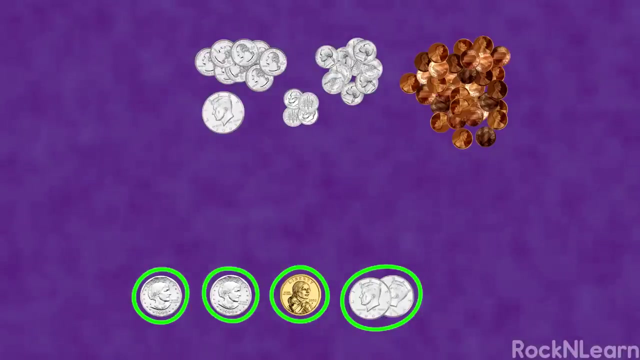 Let's put the coins in groups that are equal to a dollar, so we can count how many dollars we have. Here's one, two, three dollars from the dollar coins. Let's count two of the half dollars: Fifty a dollar. That brings us to four dollars. 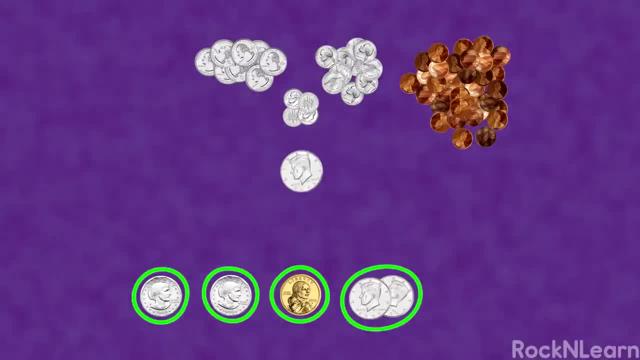 We have another half dollar left. If we put two of the quarters with it, that makes another dollar. Five dollars total, That leaves us with seven quarters. Let's add them slowly: Twenty-five, fifty, seventy-five a dollar, That's six dollars so far. 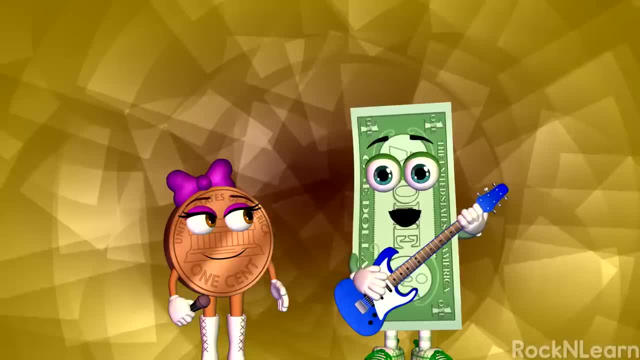 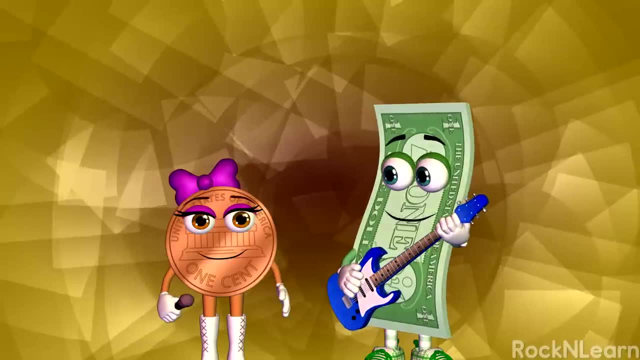 Sometimes I don't have the right number of coins to do the skip counting all the way up to a dollar, so I just use some of the smaller coins to finish up the dollar. Hey, Penny, why don't we count the money in your piggy bank? Maybe we can get our speaker fixed. 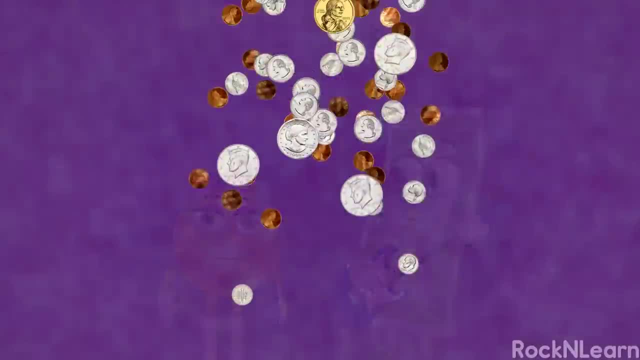 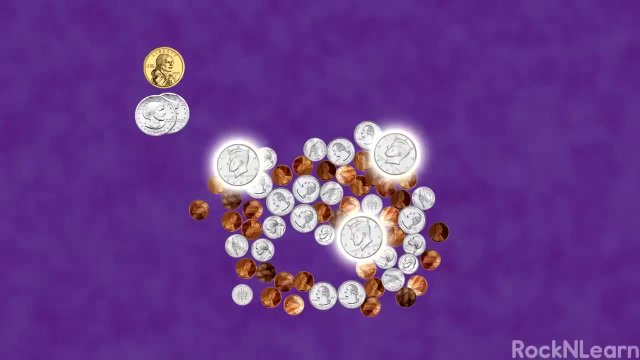 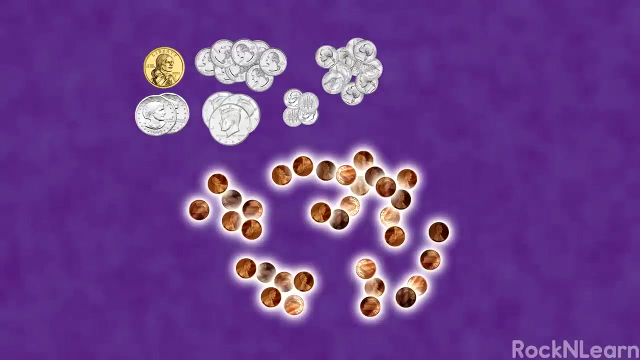 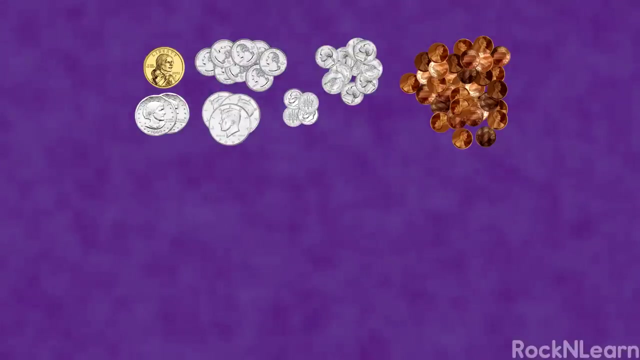 Okay, first we'll separate the coins. Here are two Susan B Anthony dollars, one Sacagawea dollar, three half dollars, nine quarters, four dimes, ten nickels and a whole pile of pennies. Let's put the coins in groups that are equal to a dollar so we can count how many dollars we have. 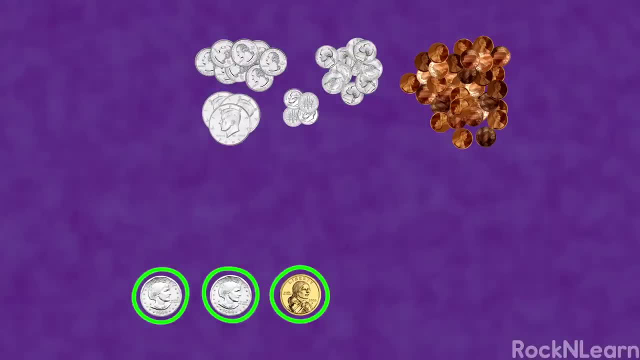 Here's one, two, three dollars from the dollar coins. Let's count two of the half dollars. Fifty a dollar That brings us to four dollars. We have another half dollar left. If we put two of the quarters with it, that makes another dollar. 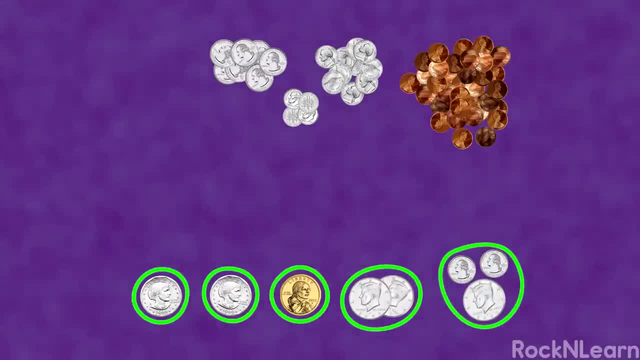 Five dollars total, That leaves us with seven quarters. Let's add them slowly. Twenty-five, fifty, seventy-five. a dollar, That's six dollars so far. Now let's count the other three quarters. Twenty-five, fifty, seventy-five. 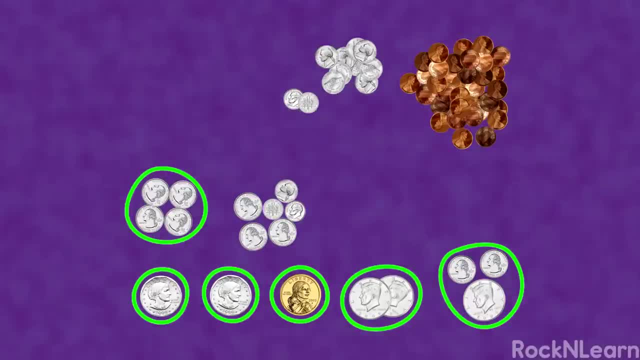 And if we add two of the two, five dimes and a nickel, that will make another dollar. Now we have seven dollars counted. That leaves us with two dimes, Ten, twenty, twenty cents. We can skip count using the nickels from there. 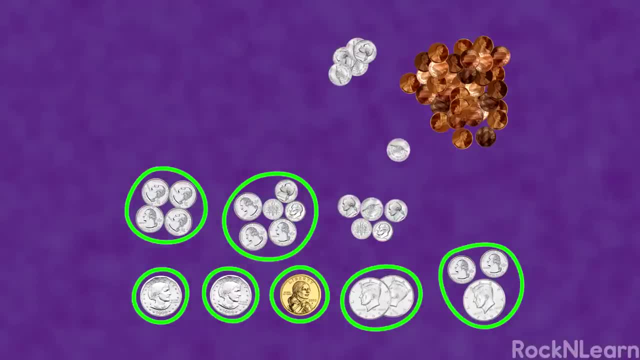 Twenty-five, thirty, thirty-five, forty, Forty-five, fifty, fifty-five, sixty, sixty-five cents. Let's see if we can get to a dollar with the pennies. One more would make sixty-six. Now let's skip. count two pennies at a time. 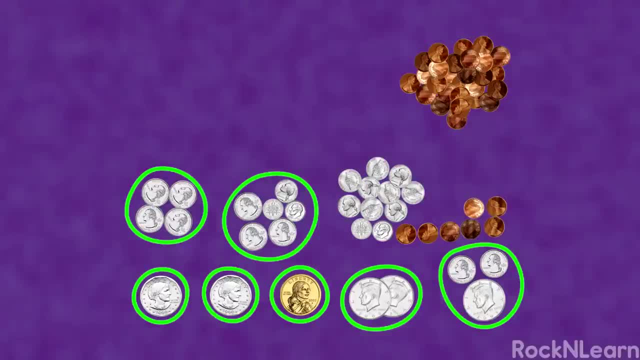 Sixty-eight, seventy, seventy-two, seventy-four, seventy-six, seventy-eight, eighty, Eighty-two, eighty-four, eighty-six, eighty-eight, ninety, Ninety-two, ninety-four, ninety-six, ninety-eight, Uh-oh, only one more. 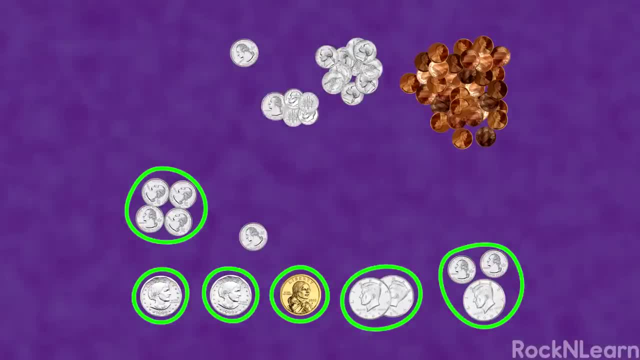 Now let's count the other three quarters- Twenty-five, fifty, seventy-five- and if we add two of the dimes and a nickel, that will make another dollar. Now we have seven dollars counted. That leaves us with two dimes. 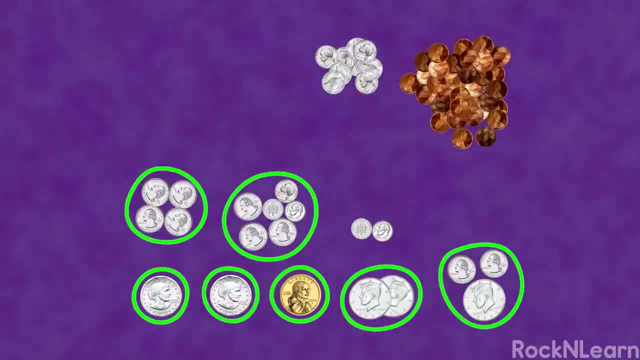 Ten, twenty, twenty cents- We can skip count using the nickels from there: Twenty-five, thirty, thirty-five, forty, forty-five, fifty, fifty-five, sixty, sixty-five cents. Let's see if we can get to a dollar with the pennies. 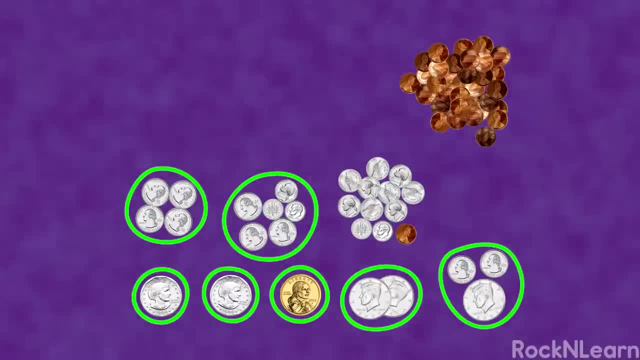 One more would make sixty-six. Now let's skip count two pennies at a time. Sixty-eight, seventy, seventy-two, seventy-four, seventy-six, seventy-eight, eighty, Eighty-two, eighty-four, eighty-six, eighty-eight. 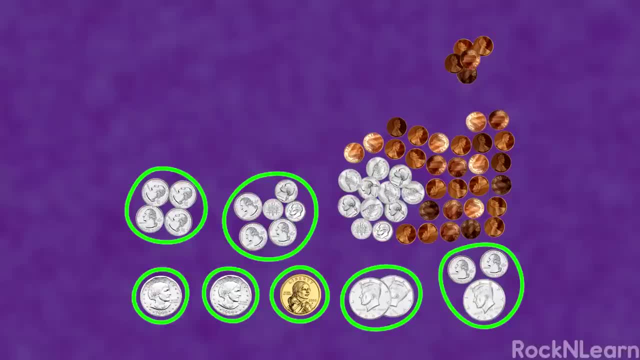 ninety, Ninety-two, ninety-four, ninety-six, ninety-eight, uh-oh, Only one more: Ninety-nine, ninety-nine. That makes one, two, three, four, five, six, seven dollars and ninety-nine cents. 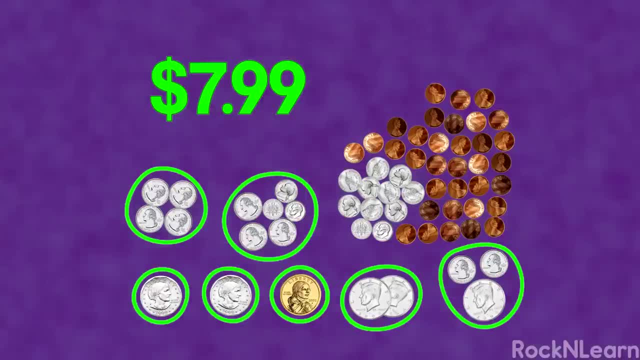 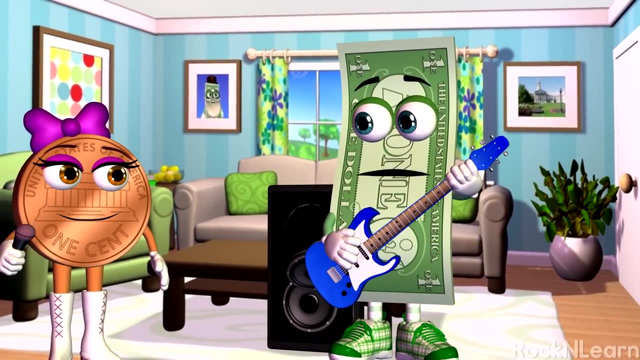 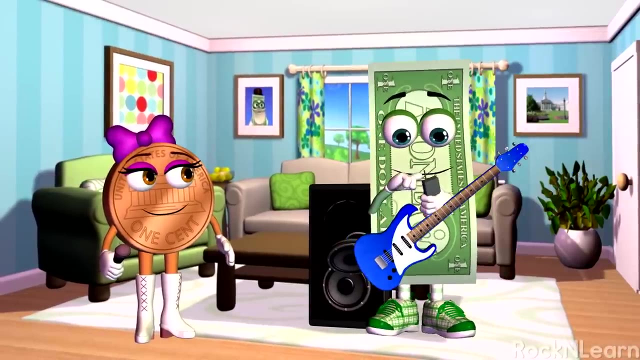 Wait, I just remembered I found a penny on the sidewalk this morning. Now we have eight whole dollars. That may not be enough to get the speaker fixed. Hmm, maybe I should call our friend Dylan at the music store to see if he can help us out. 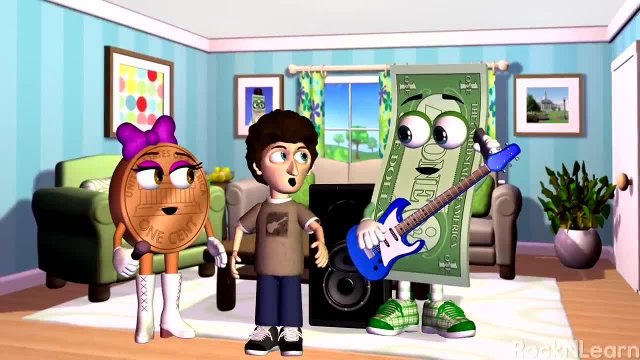 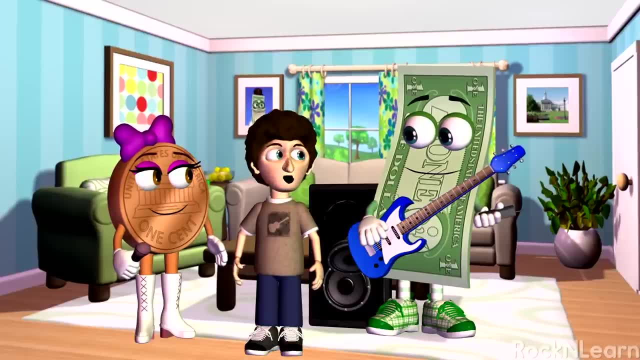 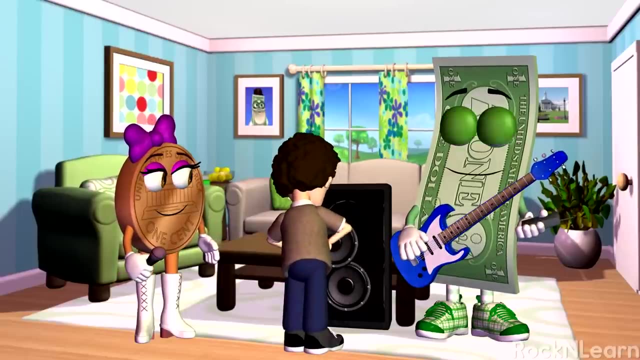 Maybe he can loan us a speaker to use. You don't have to call me man, I'm right here. I thought I'd drop by to see how things are going. Dude, do you think you can fix our speaker? Let me take a look. 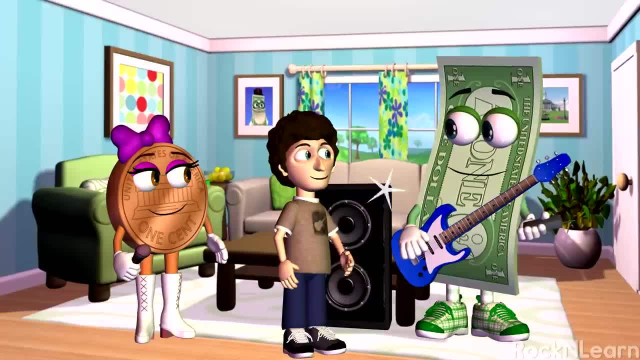 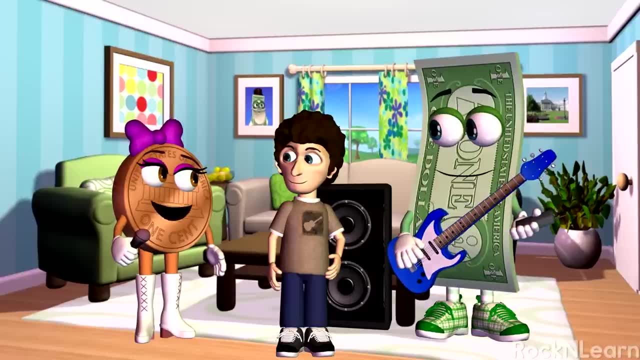 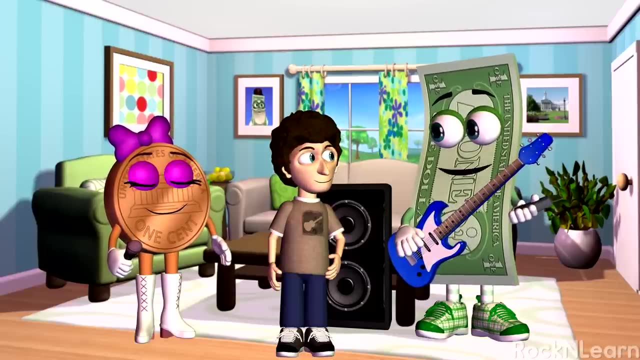 Hmm, no problem, It's just a loose wire. I won't charge you anything. Whoa, Dylan, You're pretty amazing. The speaker works and I get to keep my piggy bank full. Yeah, thanks, Dylan, You're a great friend. 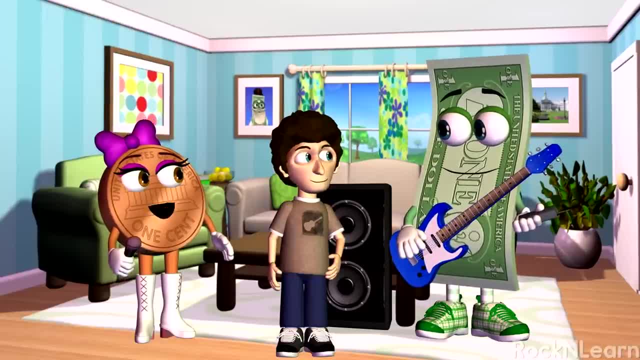 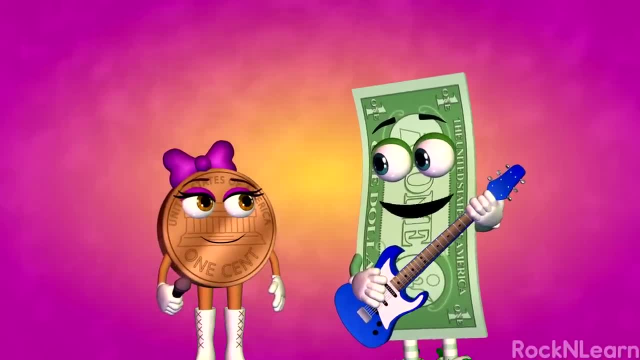 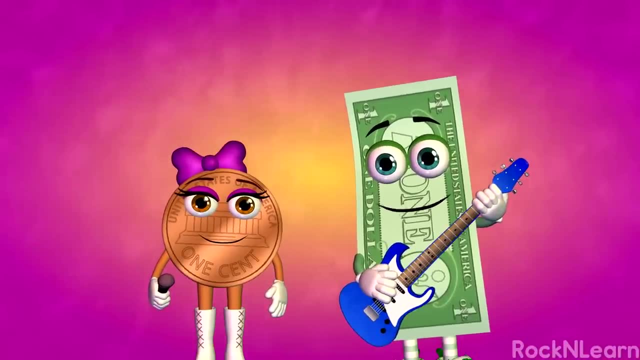 and now we can rock tonight after all Groovy. Now that we've counted the money in your piggy bank, let's practice some more. Remember: start counting with the largest coin and use skip counting wherever you can. Five, ten. 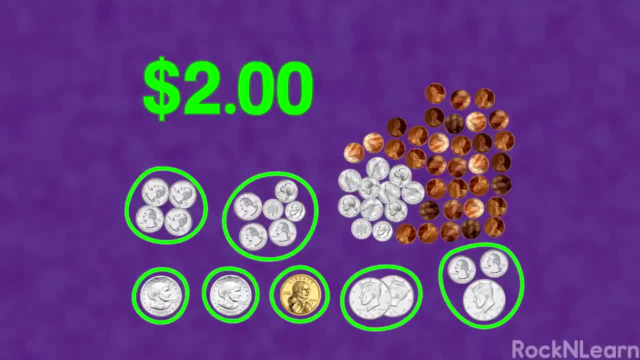 Ninety-nine. That makes one, Two, three, four, five, six, seven dollars and ninety-nine cents. Wait, I just remembered I found a penny on the sidewalk this morning. Now we have eight whole dollars. That may not be enough to get the speaker fixed. 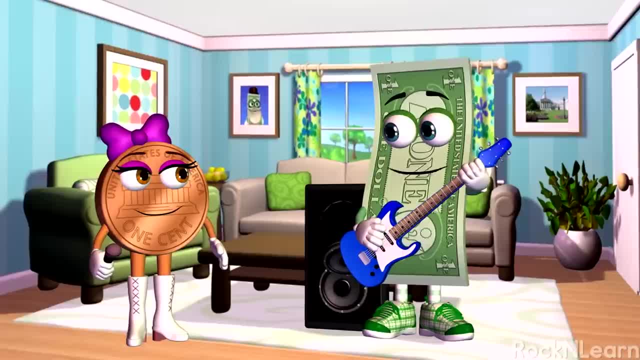 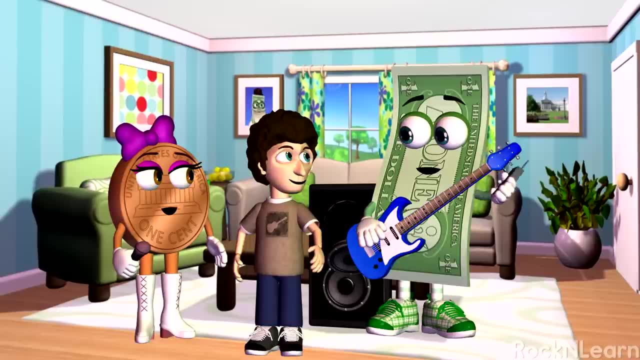 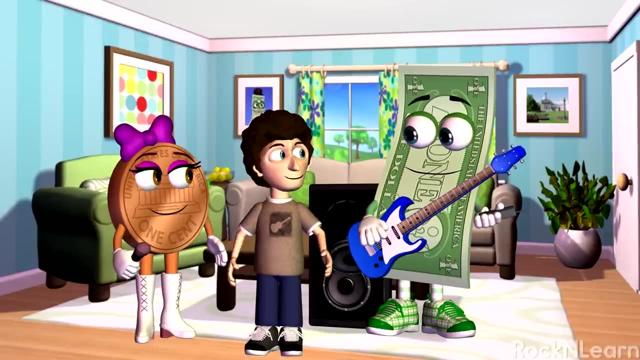 Hmm, maybe I should call our friend Dylan at the music store to see if he can help us out. Maybe he can loan us a speaker to use. You don't have to call me, man, I'm right here. I thought I'd drop by to see how things are going. 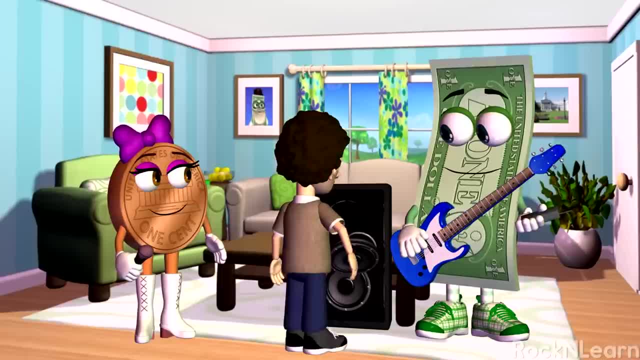 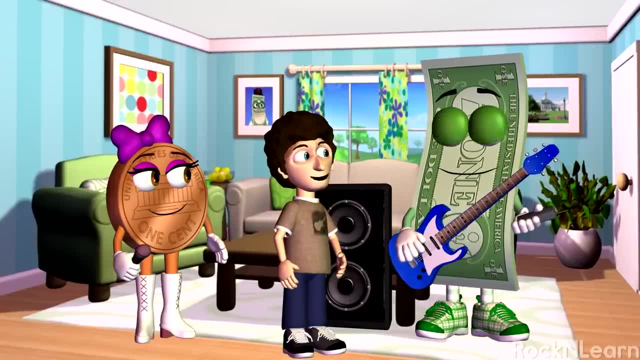 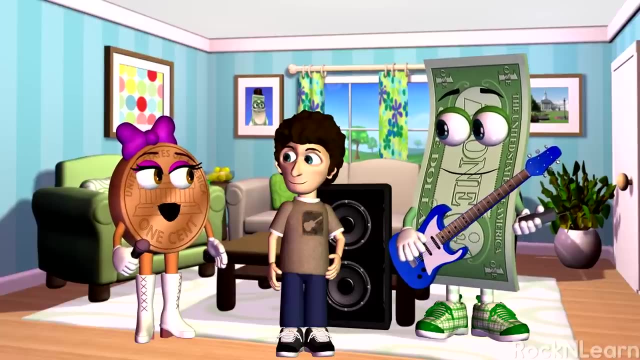 Dude, do you think you can fix our speaker? Let me take a look. Hmm, no problem, It's just a loose wire. I won't charge you anything. Whoa Dylan, you're pretty amazing. My speaker works and I get to keep my piggy bank full. 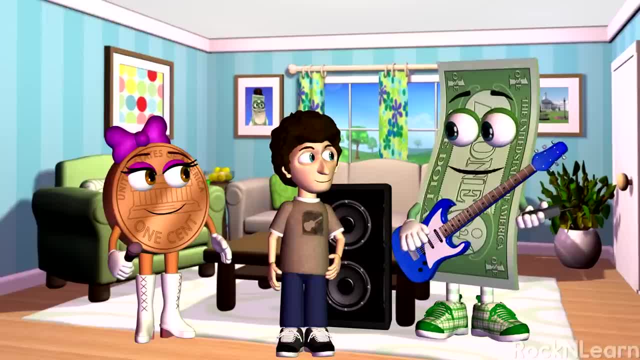 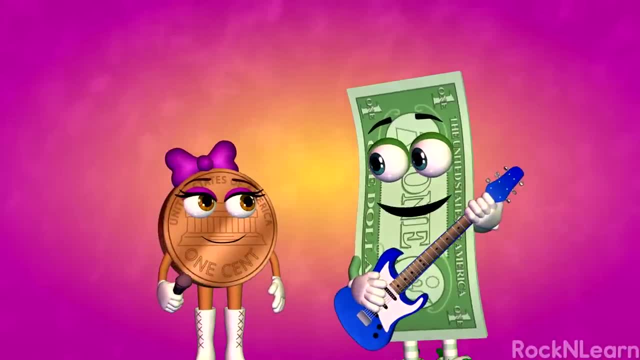 Yeah, thanks Dylan. You're a great friend and now we can rock tonight after all Groovy. Now that we've counted the money in your piggy bank, let's practice some more. Remember: start counting with the largest coin. 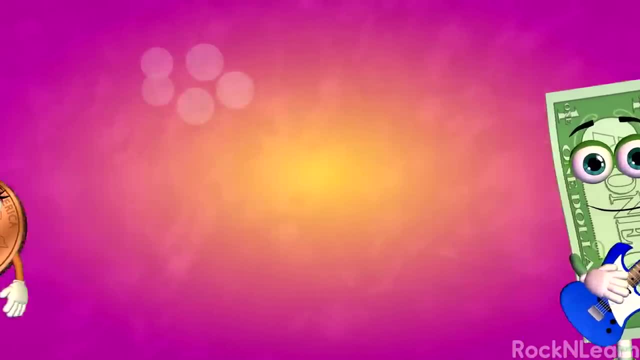 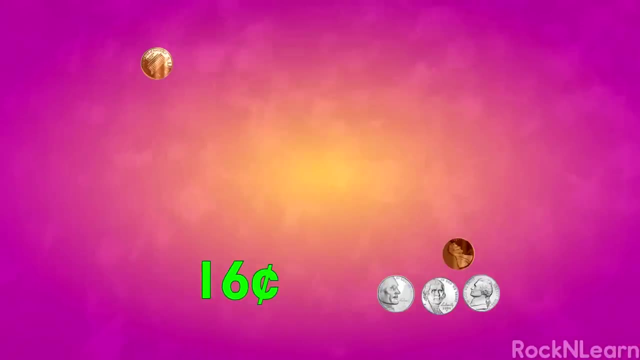 and use. skip counting wherever you can. 5, 10,, 15,, 16,, 17,, 17 cents. 10,, 20,, 25,, 30,, 35,, 36,, 36 cents. 25, 30, 31, 32, 32 cents. 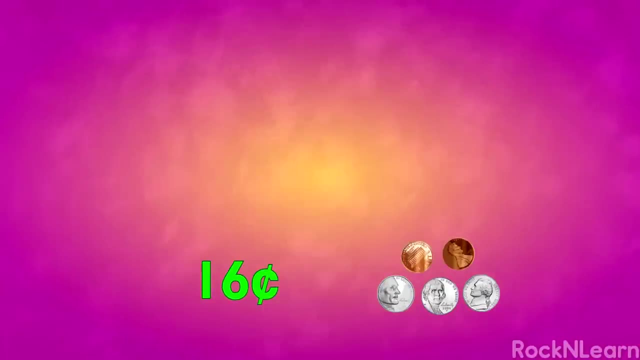 fifteen, sixteen, seventeen, seventeen cents Ten, twenty, twenty-five, thirty, thirty-five, thirty-six, thirty-six cents Twenty-five, thirty, thirty-one, thirty-two, thirty-two cents Twenty-five, fifty, sixty, seventy. 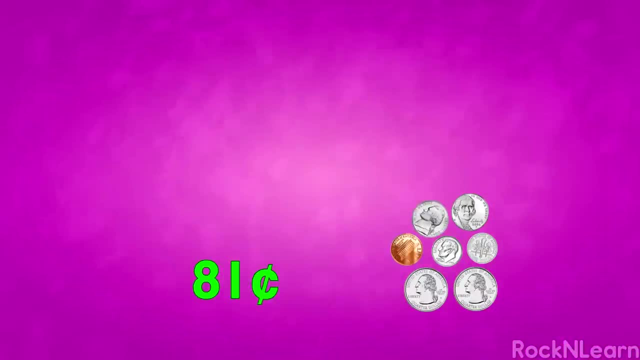 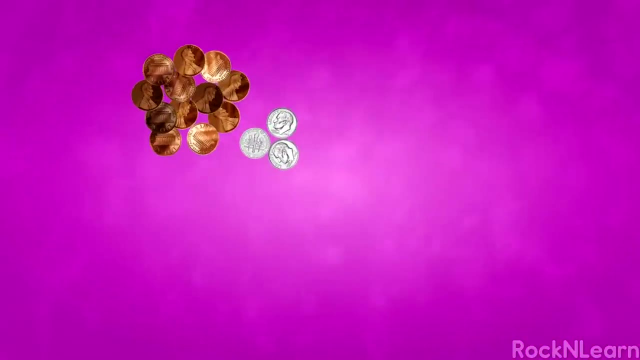 seventy-five, eighty, eighty-one, eighty-one cents Ten, twenty, thirty, thirty-two, thirty-four, thirty-six, thirty-eight, forty, forty-two, forty-two cents Twenty-five, thirty-five, forty-five, fifty, fifty-five. 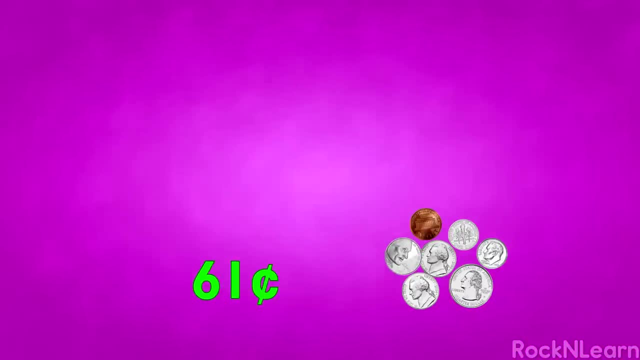 sixty sixty-one, That gives us sixty-one cents Twenty-five, fifty, seventy-five, eighty-five, eighty-six, eighty-seven, eighty-eight, eighty-eight cents Twenty-five, fifty, fifty-five, fifty-six, fifty-seven, fifty-eight. 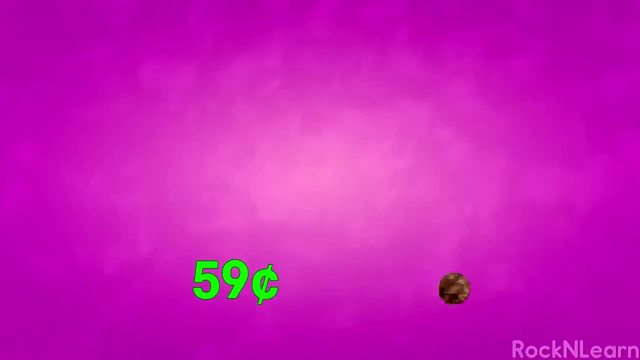 fifty-nine, fifty-nine cents- Wow, These coins. Twenty-five, fifty, seventy-five, eighty-five, ninety, ninety-five, ninety-six, ninety-eight, one-hundred, one-hundred-two, one-hundred-two cents, Or a dollar and two cents. 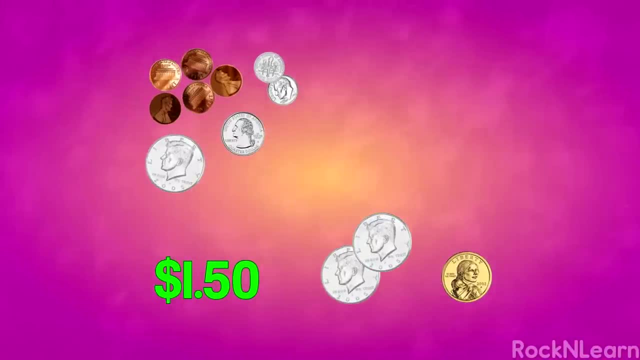 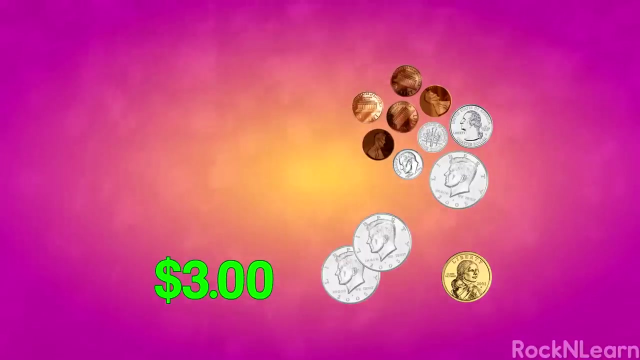 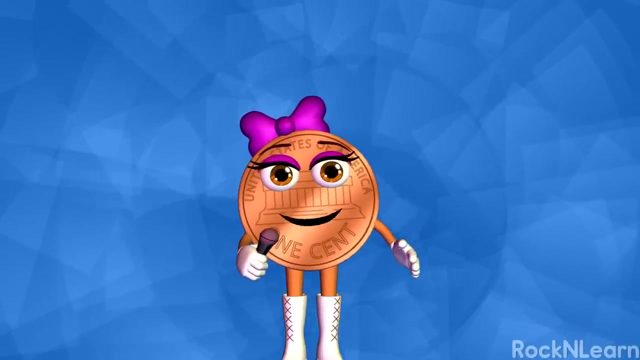 One dollar fifty one-hundred makes two dollars. Fifty, seventy-five, eighty-five, ninety-five, ninety-six, ninety-seven, ninety-eight, ninety-nine one-hundred, That's another dollar for three dollars total Great. Now let's play a game called Count the Coins. 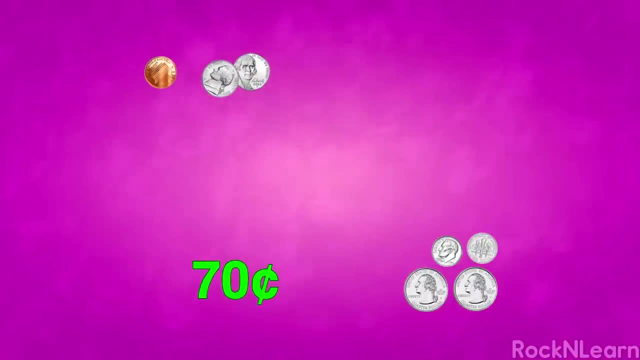 25, 50, 60, 70, 75, 80, 81, 81 cents. 10, 20, 30, 32, 34, 36, 38, 40, 42, 42 cents. 25, 35, 45, 50, 55, 60, 61. that gives us 61 cents. 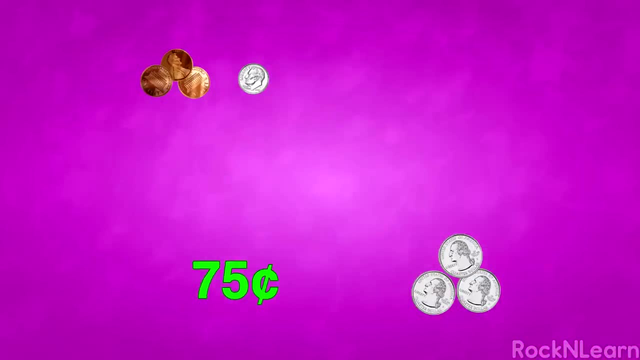 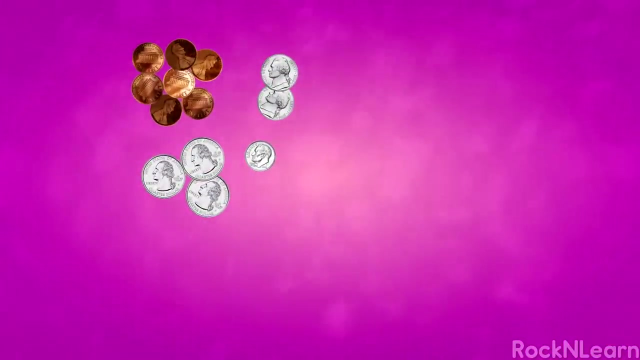 25, 50, 75, 85, 86, 87, 88, 88 cents. 25, 50, 55, 56, 57, 58, 59, 59 cents. Wow, look at all these coins. 25, 50, 75, 85, 90, 95. 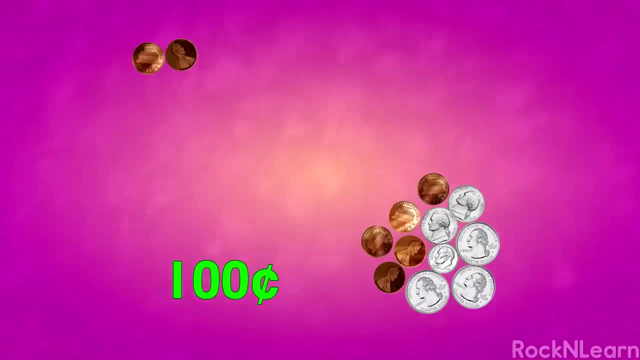 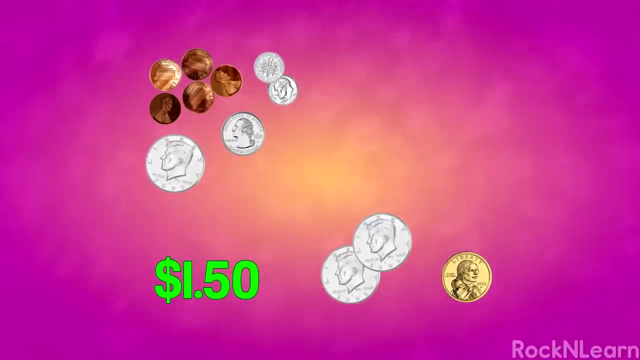 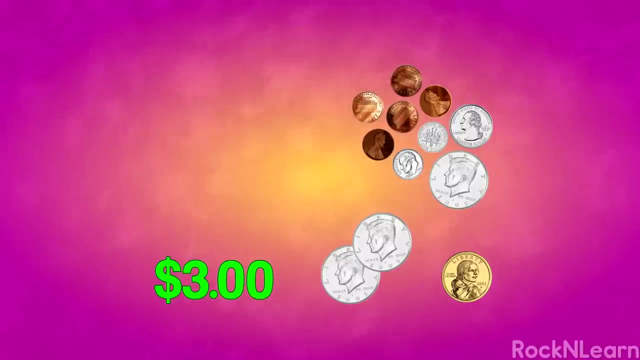 96 98 100, 102, 102 cents or a dollar and two sense. $1 50, 100 makes two dollars. 50, 75, 85, 95, 96, 97, 98, 99, 100. that's another dollar for three dollars total. 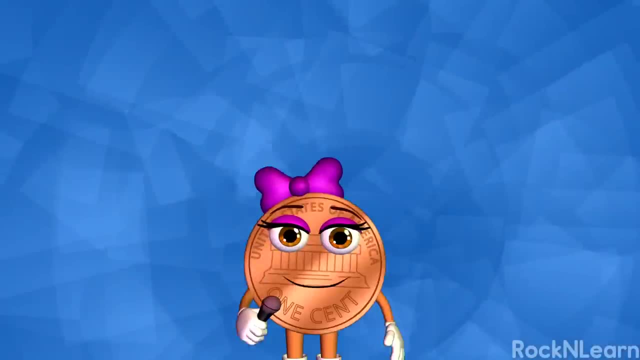 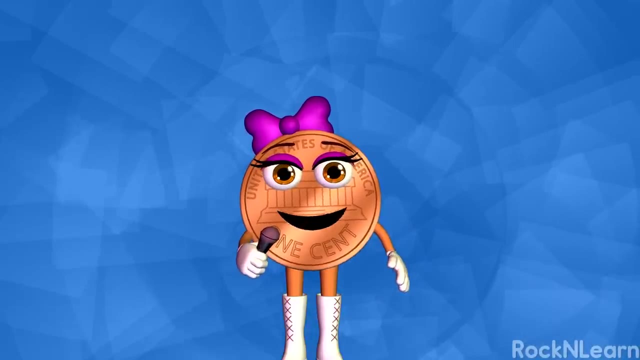 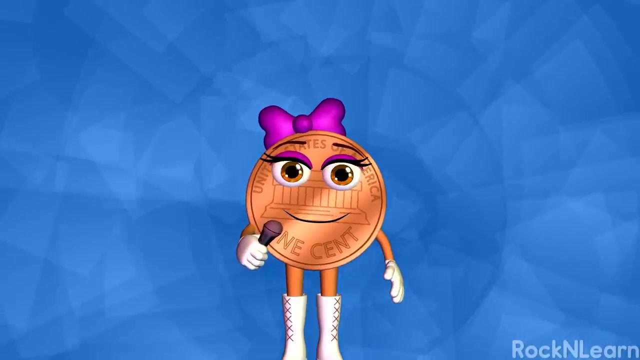 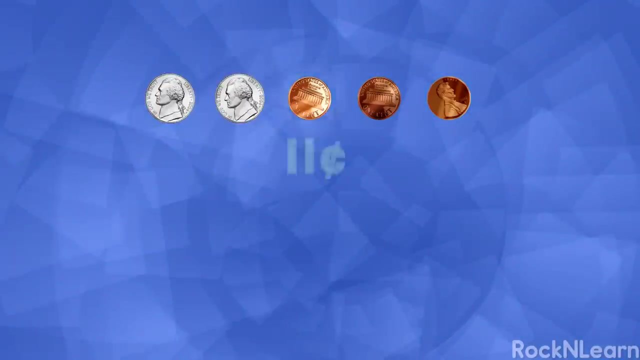 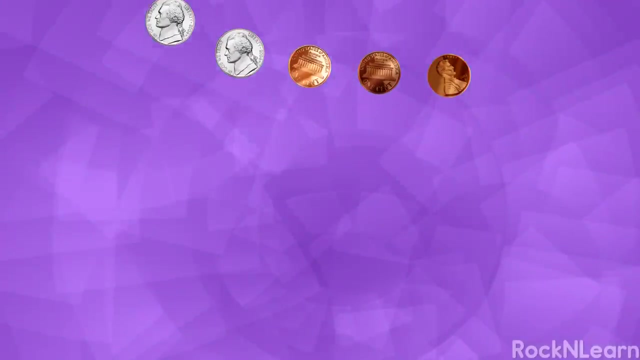 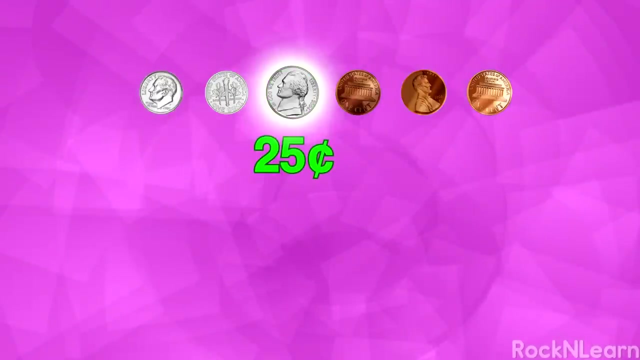 Great. Now let's play a game called Count the Coins. See if you can count the coins faster than we do. We'll give you a little help on the first few. then you're on your own Ready. Thirteen cents, Twenty-eight cents. 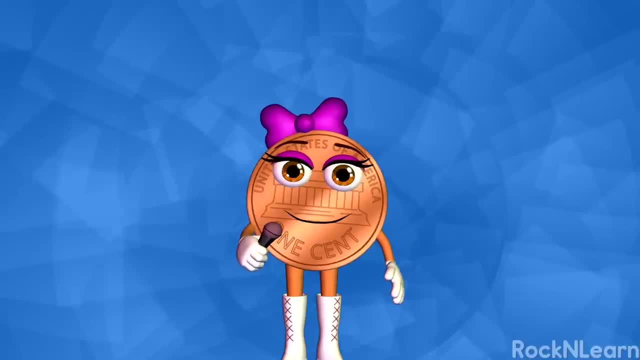 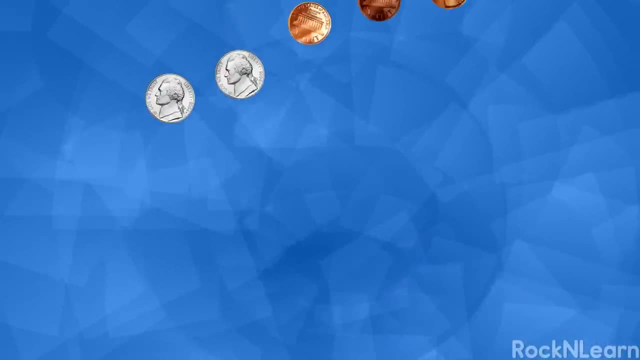 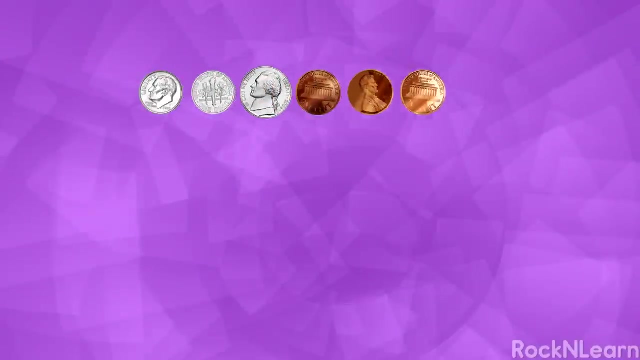 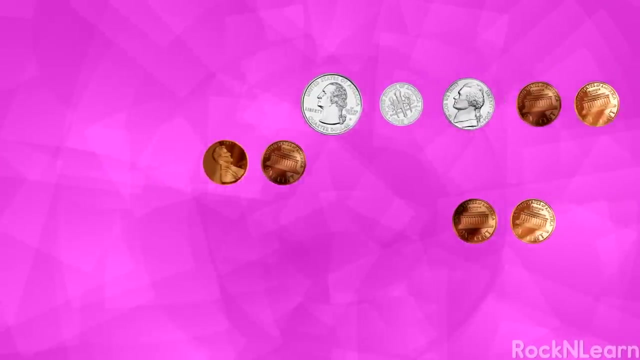 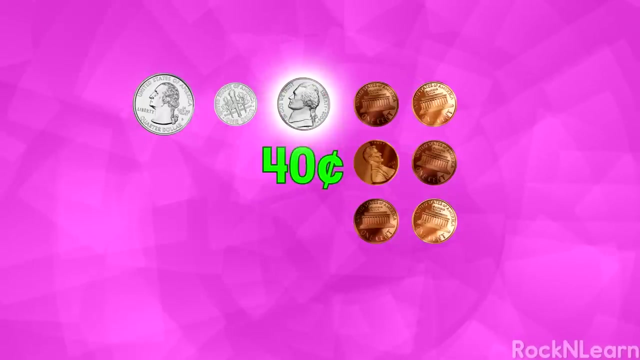 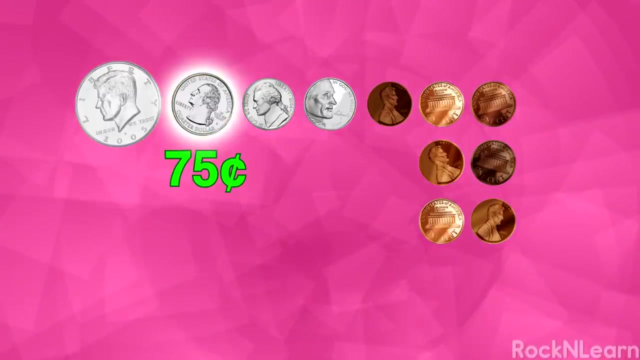 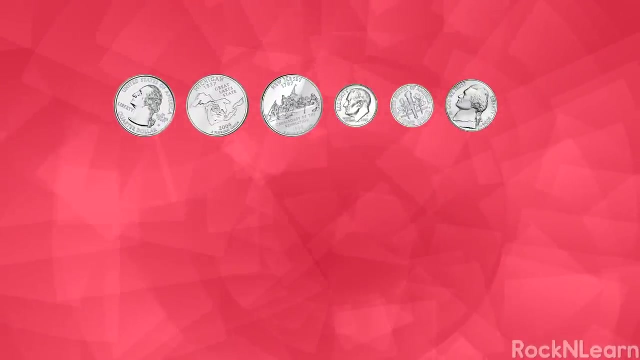 See if you can count the coins faster than we do. We'll give you a little help on the first few, then you're on your own Ready. Thirteen cents, Twenty-eight cents, Forty-six cents, Ninety-two cents, One-hundred cents. 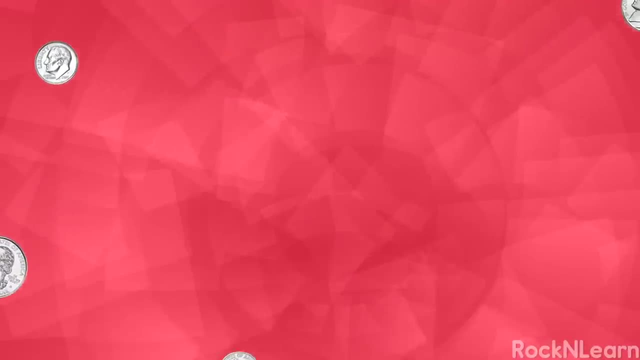 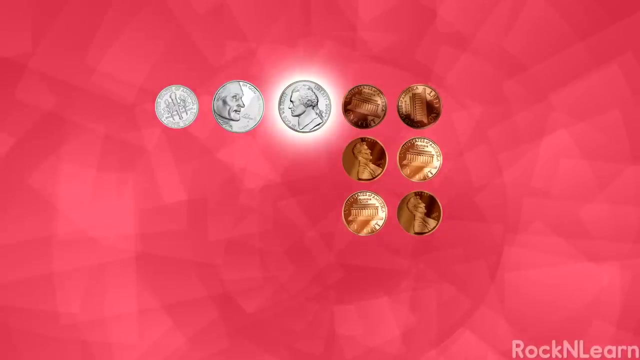 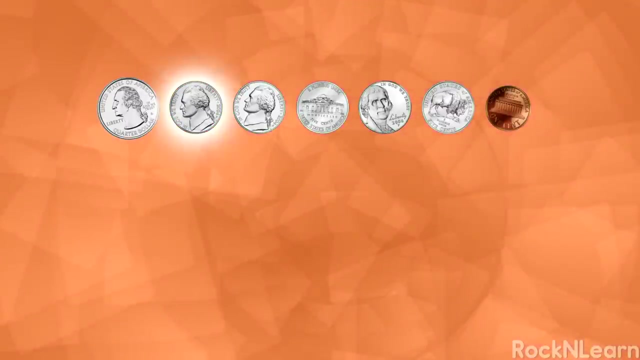 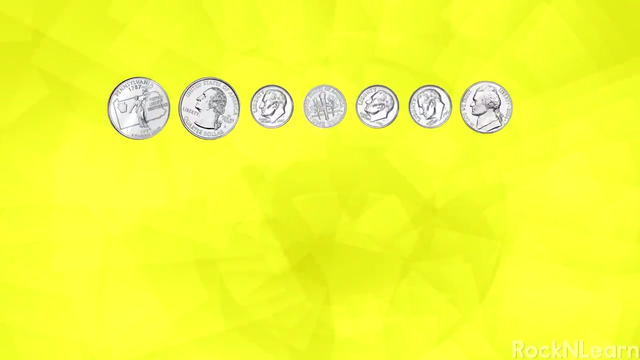 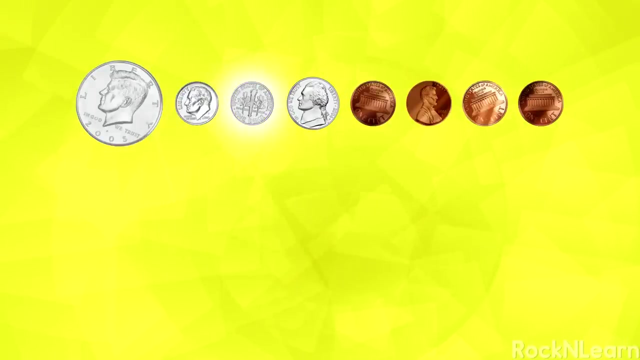 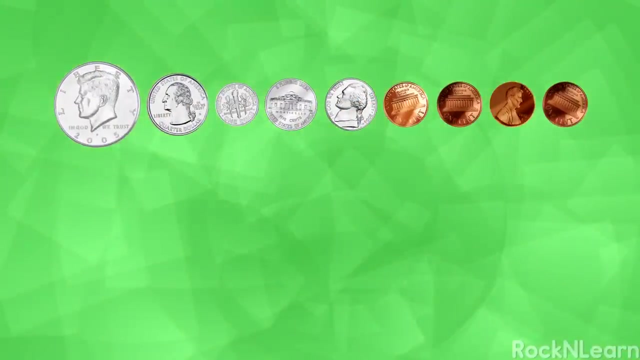 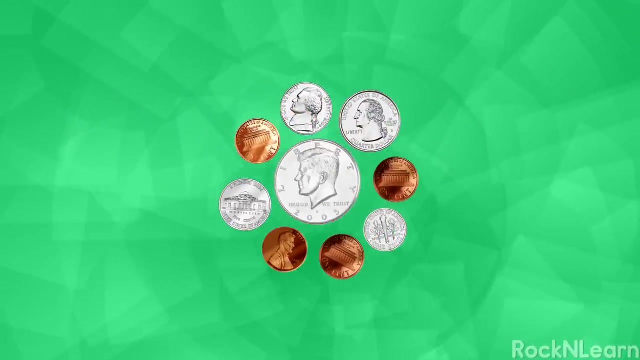 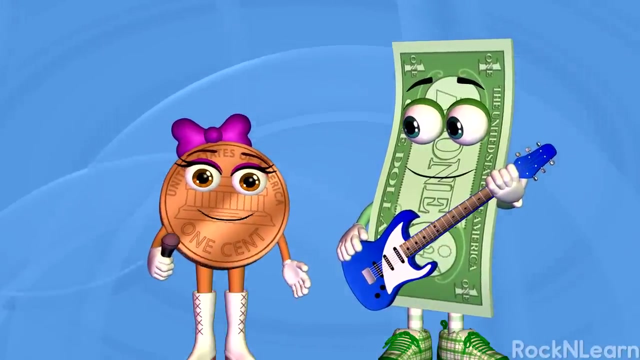 or one dollar. Twenty-six cents, Fifty-one cents, $0.95- $0.79- $0.99- Count-tastic. Now that we know how to count money, we will know if we have enough to buy certain things. Um, count-tastic. 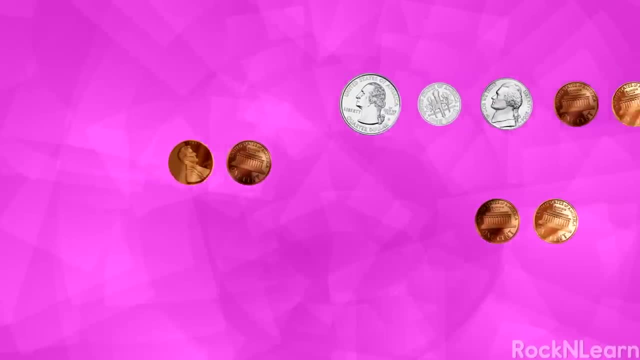 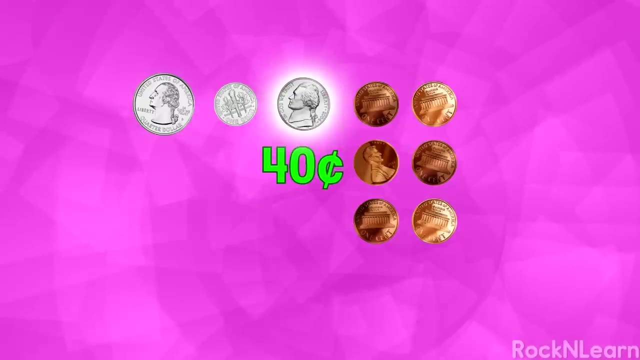 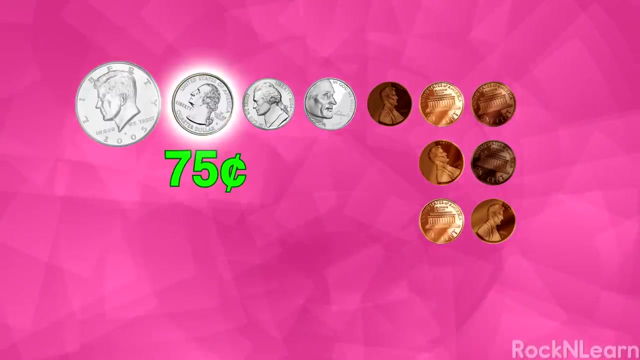 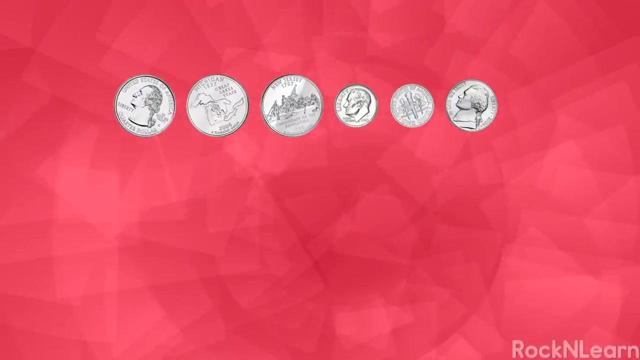 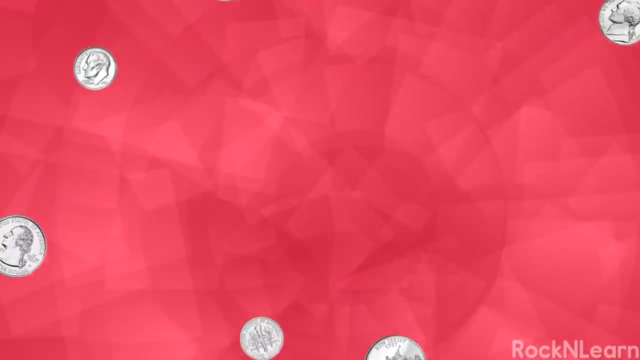 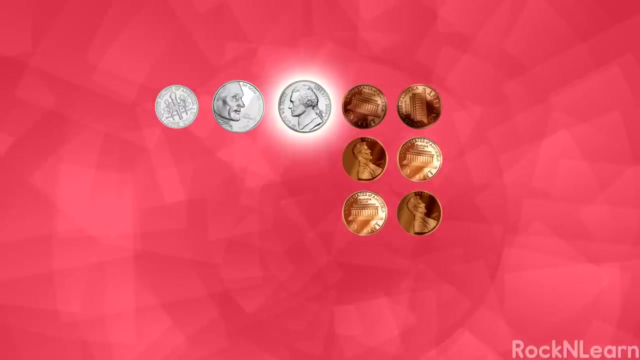 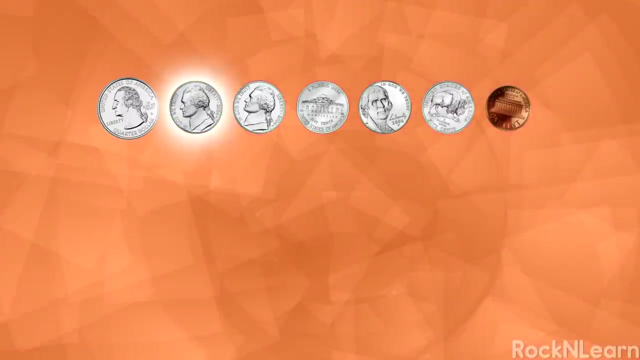 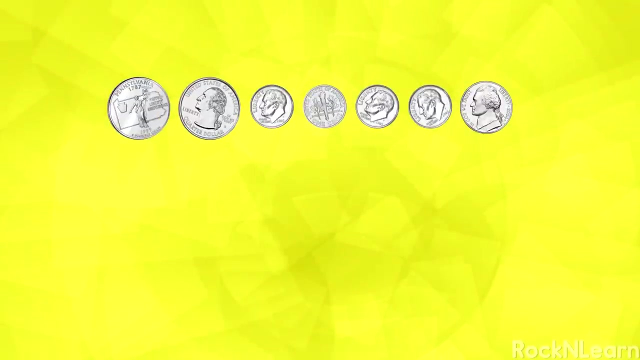 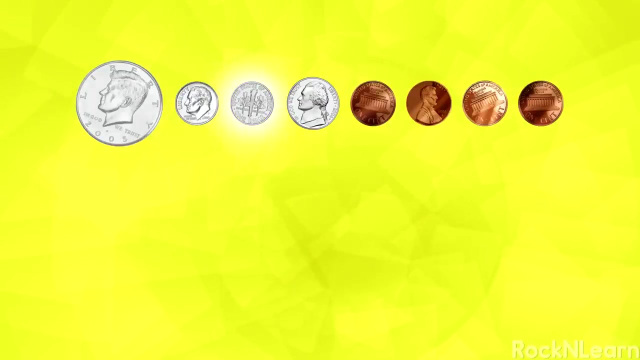 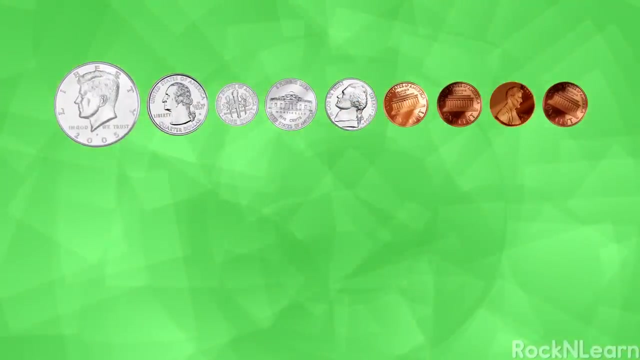 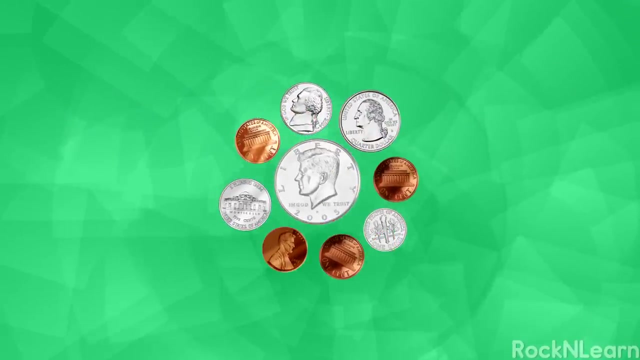 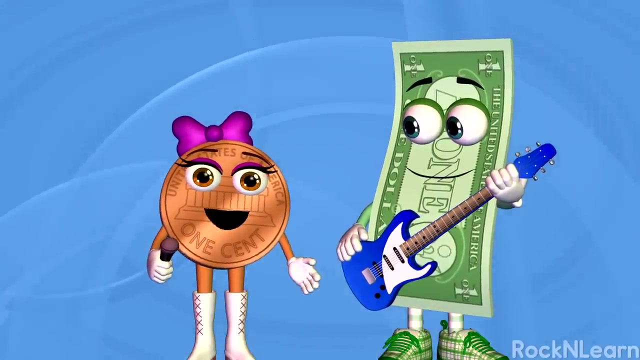 Forty-six cents, Ninety-two cents, Fifteen cents, One hundred cents, or one dollar Twenty-six cents, Fifty-one cents, Ninety-five cents, Seventy-nine cents, Ninety-nine cents. Count-tastic. Now that we know how to count money, we will know if we have enough to buy certain things. 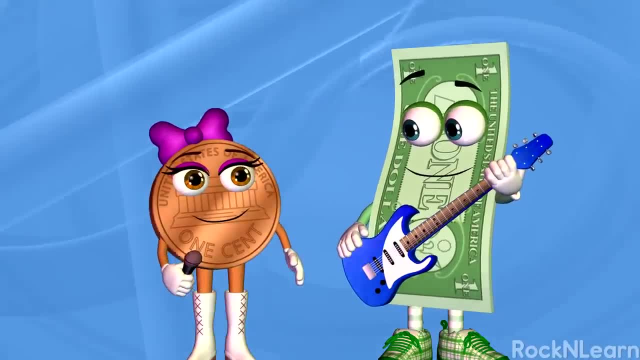 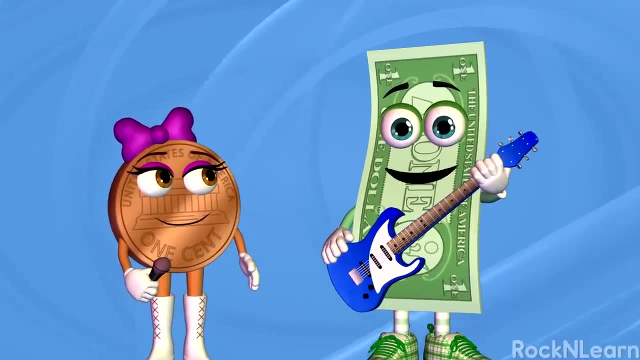 Um, count-tastic? I'm not sure that's a word. It is now. Okay, then let's do some count-tastic, make-believe shopping to practice. On the left side of the screen we'll show some things we might want to buy. 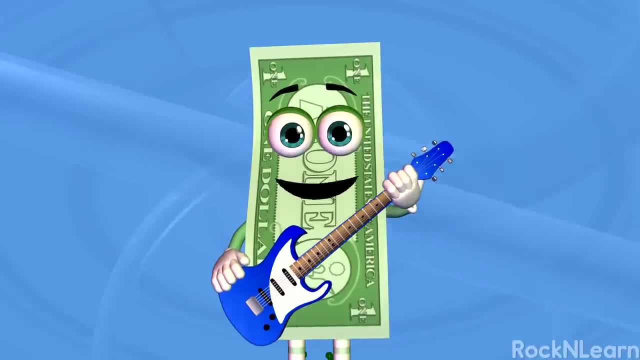 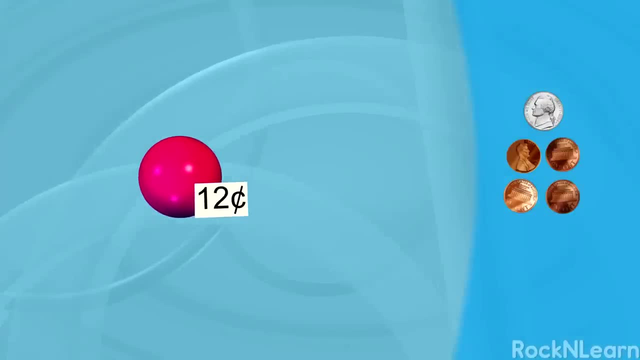 On the right side of the screen we'll show the money we have. Let's practice shopping First. let's see how much money we have. Five, six, seven, eight, nine, nine cents. Nine is less than the twelve cents that the gumball costs. 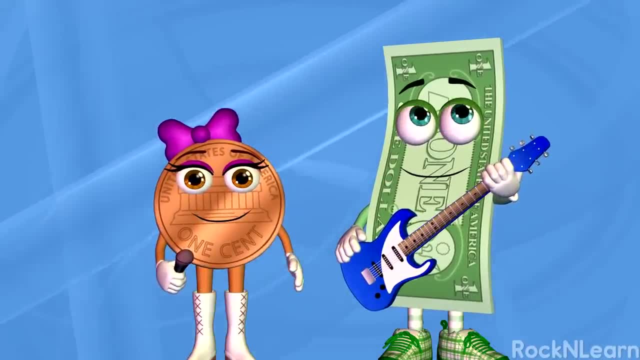 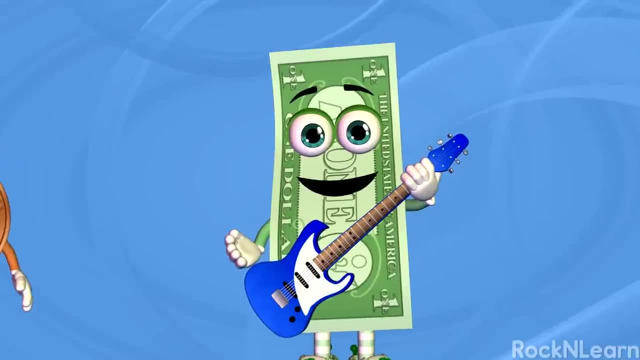 I'm not sure that's a word. It is now. Okay, then let's do some count-tastic, make-believe shopping to practice On the left side of the screen. we'll show some things we might want to buy On the right side of the screen. 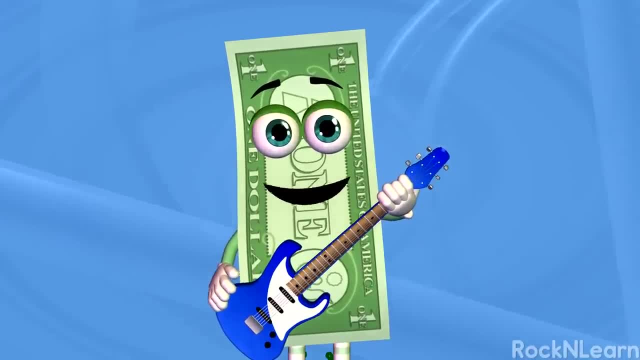 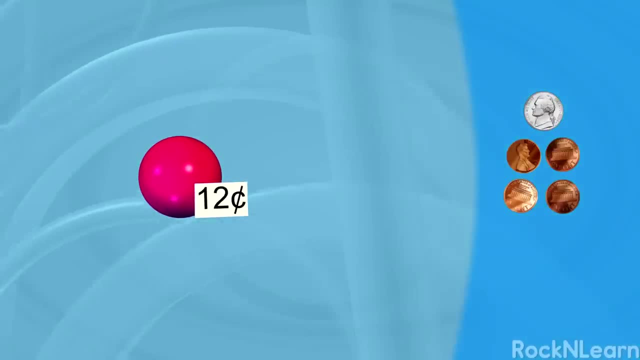 we'll show the money we have available. Let's practice shopping First. let's see how much money we have. Five, six, seven, eight, nine, nine cents. Nine is less than the twelve cents that the gumball costs. 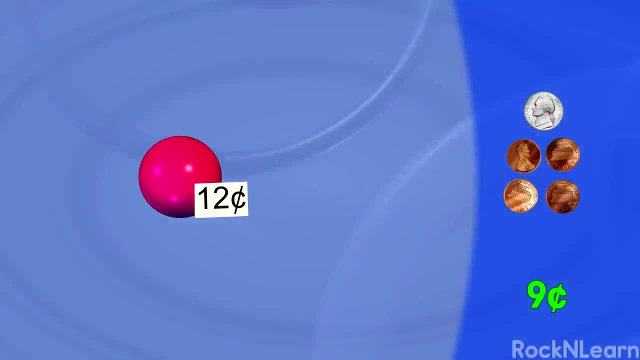 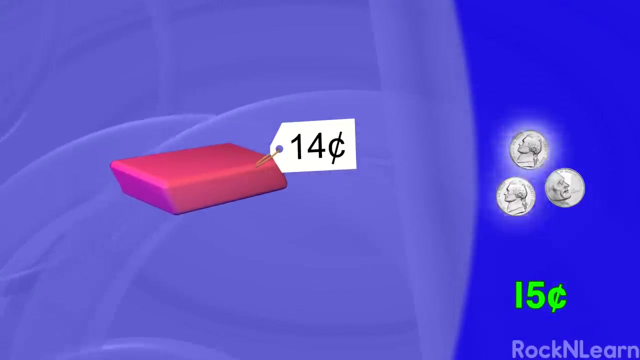 So we don't have quite enough money to get the gum. Guess, we'll have to chew, chew, chew something else. Hmm, Five, ten, fifteen, fifteen cents Fifteen is one one cent more than the fourteen cents that this eraser costs. 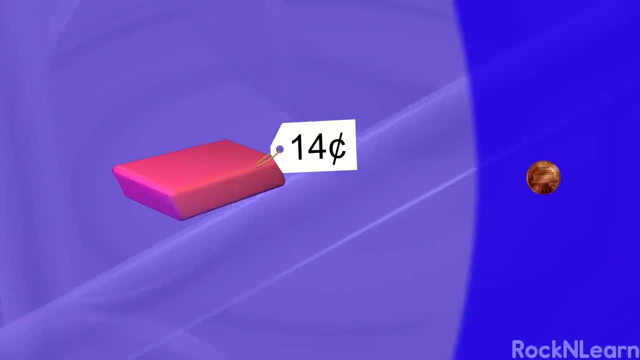 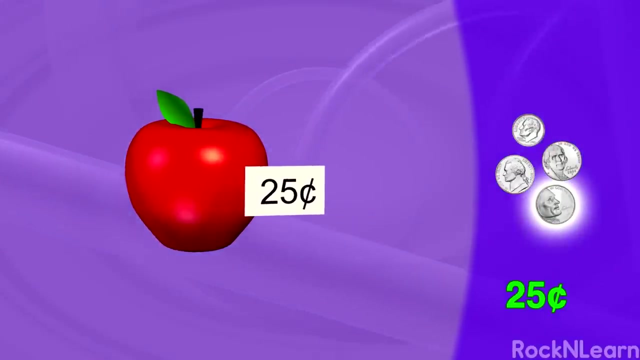 So we can buy the eraser and get one penny or one cent back. That'll work. Good job. Ten, fifteen, twenty, twenty-five, twenty-five cents- Hey, that's exactly what we need. to buy this apple Ten. 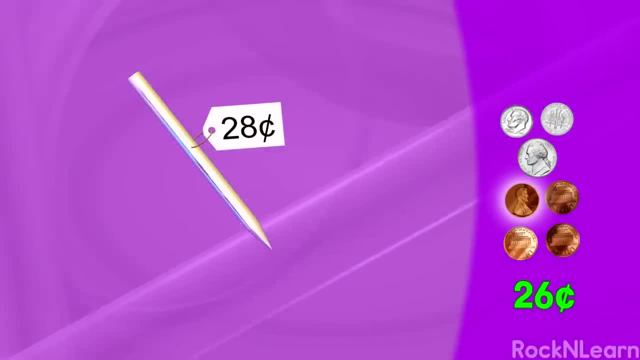 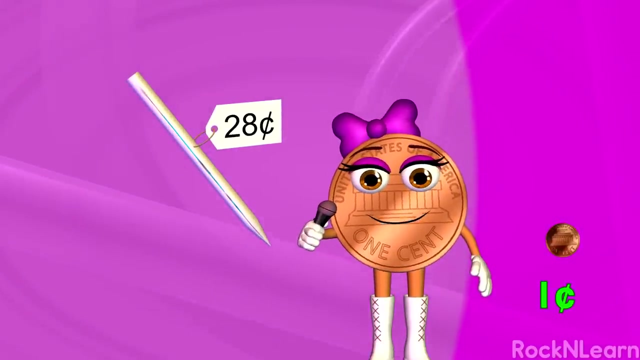 twenty, twenty-five, twenty-six, twenty-seven, twenty-eight, twenty-nine, Twenty-nine cents, But we only need twenty-eight cents. We get the pencil and we get to keep one penny. I've always got at least one penny Me. 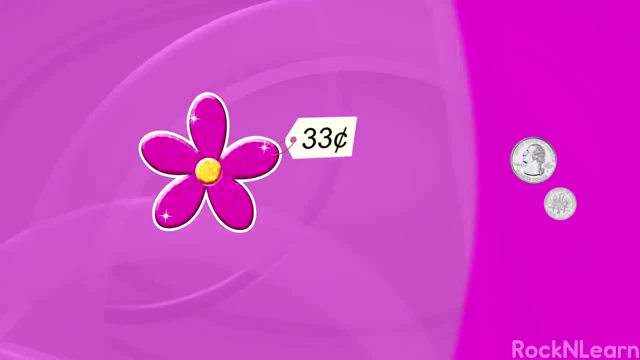 Ha, ha ha. Twenty-five, thirty-five, thirty-five cents- That's more than we need for this cool sticker. To know how much change we should get back, we'll start at the price of the sticker and count up to how much money we have. 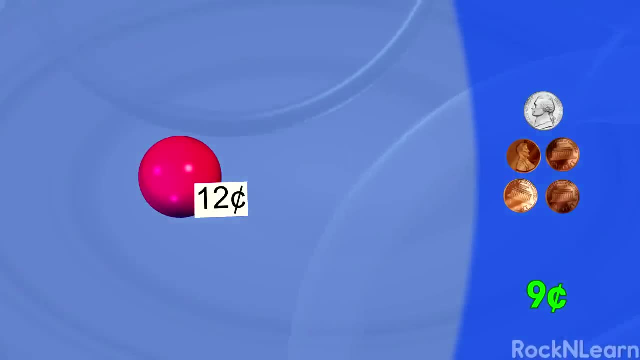 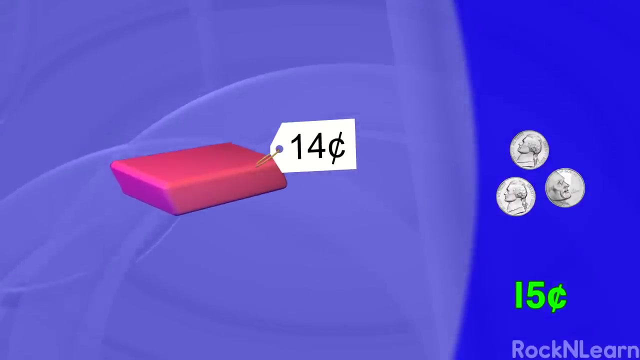 So we don't have quite enough money to get the gum. Guess, we'll have to chew, chew, chew something else. Hmm, five, ten, fifteen, fifteen cents Fifteen is one cent more than the fourteen cents that this eraser costs. 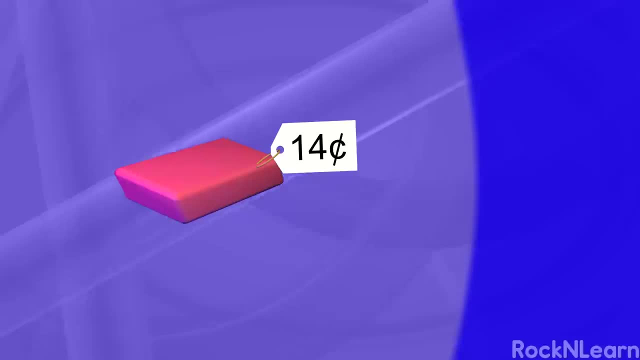 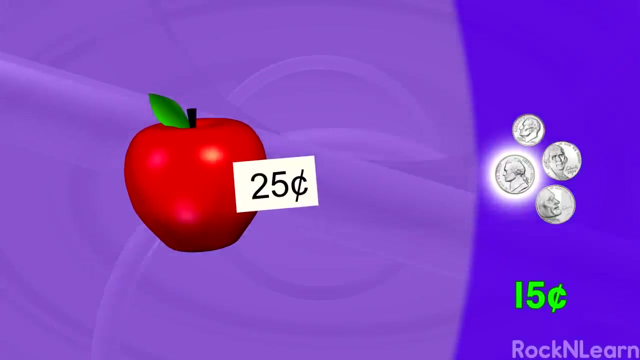 So we can buy the eraser and get one penny or one cent back. That'll work. Good job. Ten, fifteen, fifteen, Twenty, twenty-five, twenty-five cents- Hey, that's exactly what we need to buy this apple. 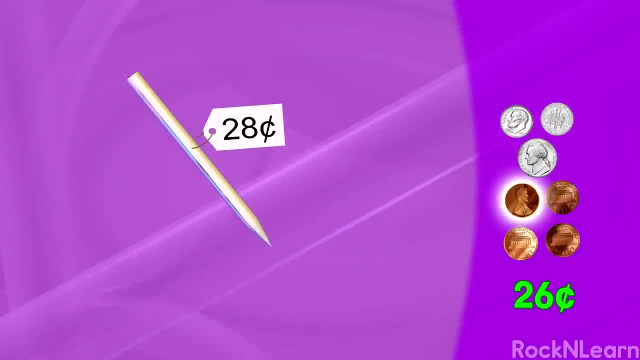 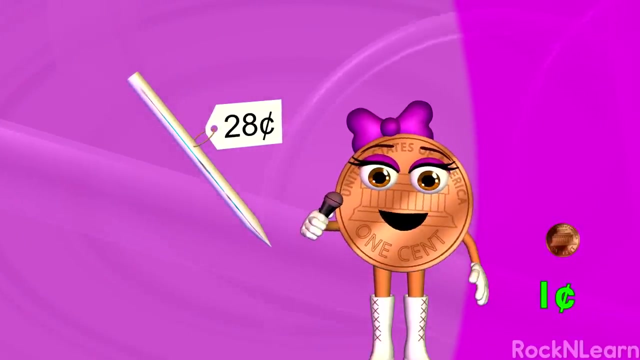 Ten, twenty, twenty-five, twenty-six, twenty-seven, twenty-eight, twenty-nine, Twenty-nine cents, But we only need twenty-eight cents. We get the pencil and we get to keep one penny. I've always got at least one penny Me. 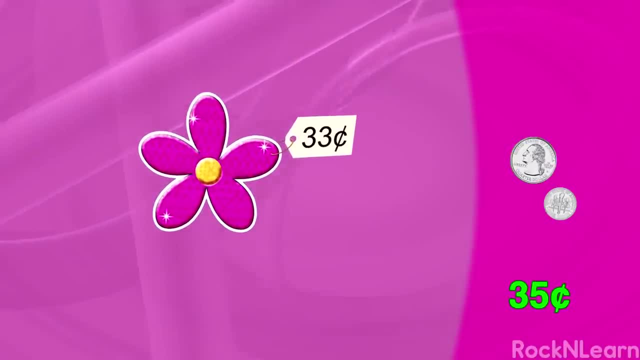 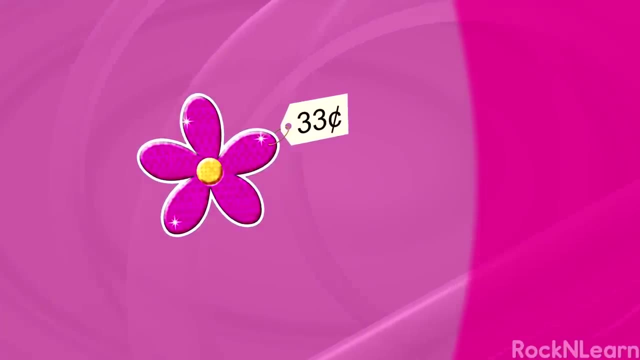 Twenty-five, thirty-five, thirty-five cents. That's more than we need for this cool sticker. To know how much change we should get back, we'll start at the price of the sticker and count up to how much money we have. The sticker is thirty-three cents. 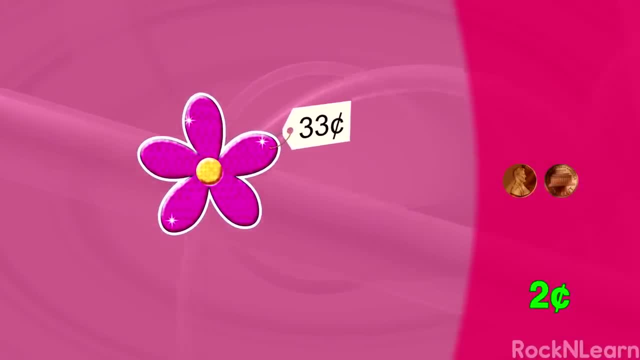 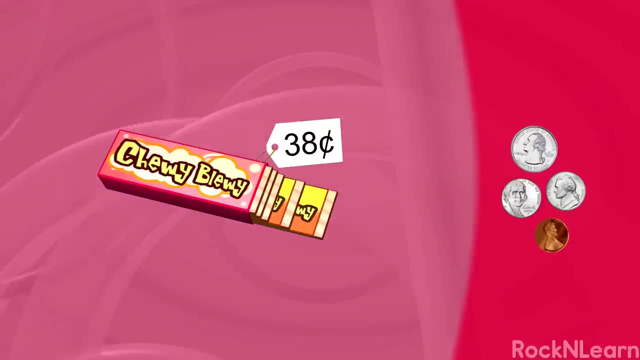 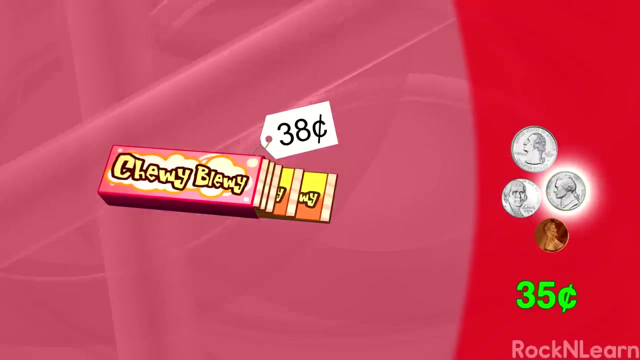 Thirty-four, thirty-five, That's two cents. we'll get back More gum. Well, okay, let's try it. Twenty-five, thirty, thirty-five, thirty-six. Oh, we need two pennies to get this pack of gum. 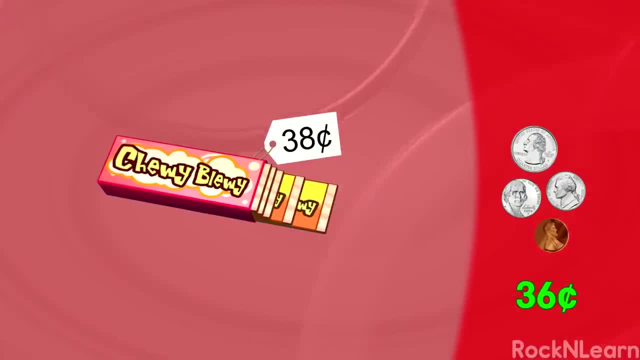 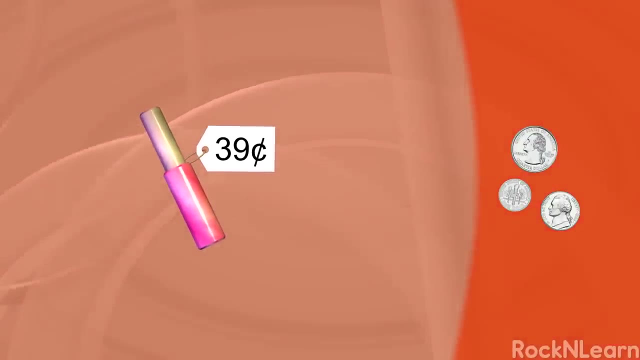 Say: could we use the two cents we had left over from the sparkly sticker? Sure, but I get a piece of gum too. You got it. Ah, Mmm, strawberry lip gloss. Oh brother, Hey, I want to buy this. 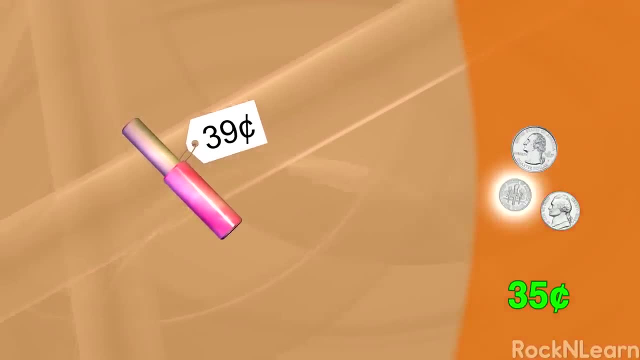 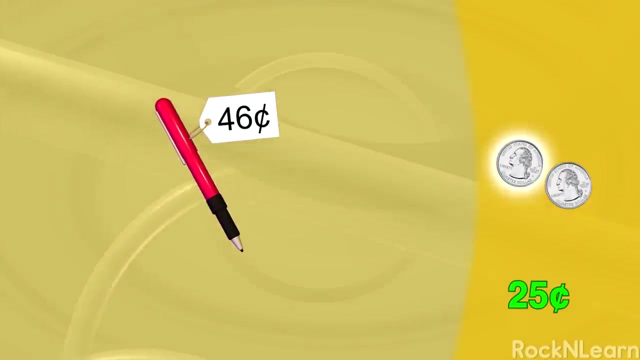 Let's see. I have twenty-five, thirty-five, forty, forty cents. I can get the lip gloss and a penny back. We have twenty-five, fifty, fifty cents. That's more than enough to get this pen. But let's see how much we'd get back. 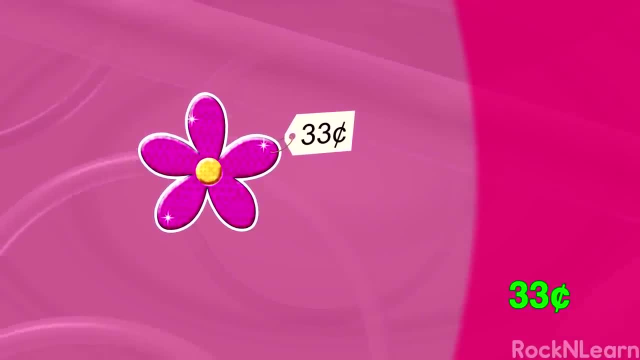 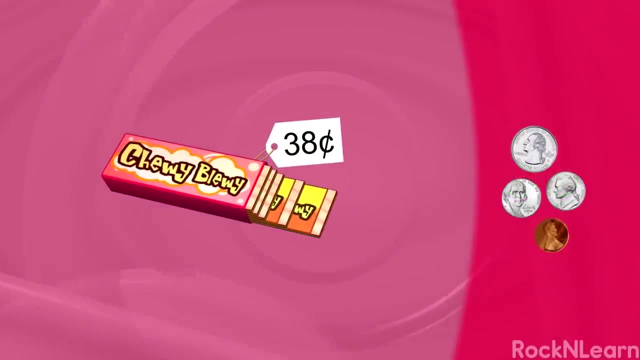 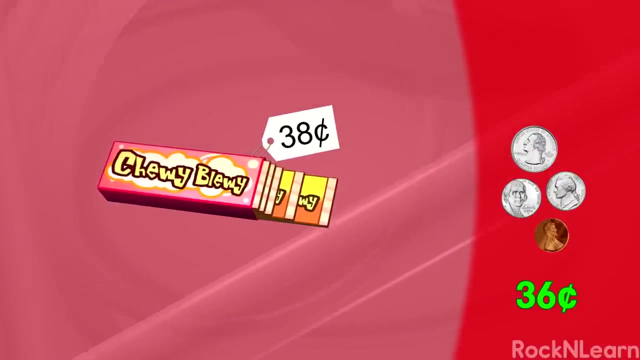 The sticker is thirty-three cents. Thirty-four, thirty-five, That's two cents. we'll get back More gum. Well, okay, Let's try it. Twenty-five, thirty, thirty-five, thirty-six. Oh, we need two pennies to get this pack of gum. 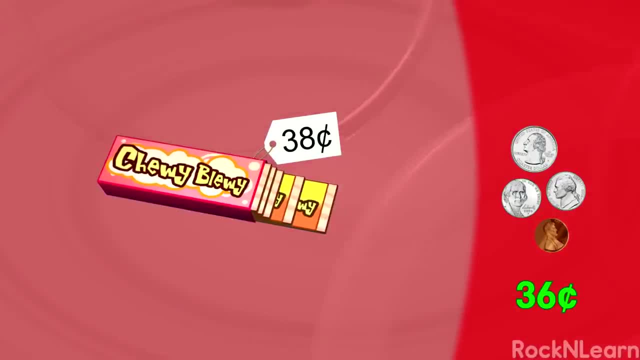 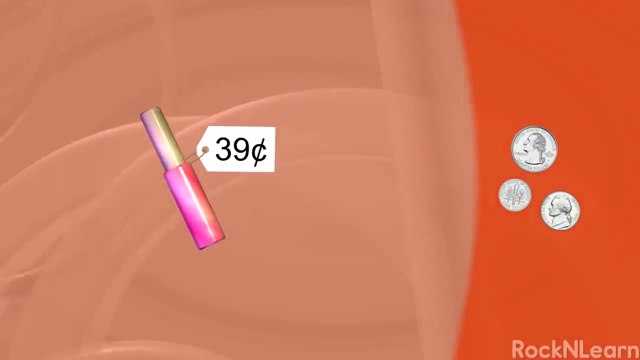 Say: could we use the two cents we had left over from the sparkly sticker? Sure, but I get a piece of gum too. You got it. Mmm. strawberry lip gloss. Oh brother, Hey, I want to buy this. 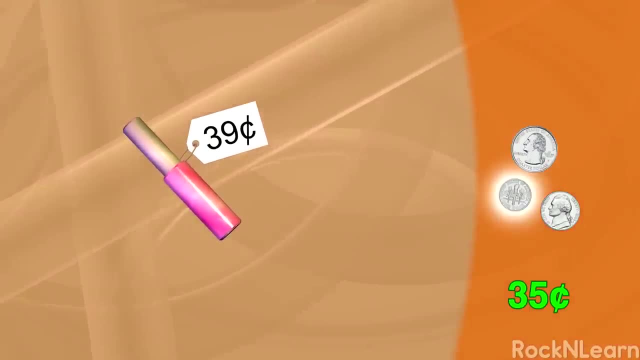 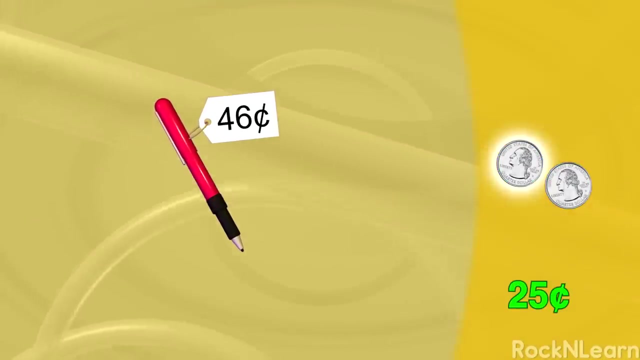 Let's see. I have twenty-five, thirty-five, forty, forty cents. I can get the lip gloss and a penny back. We have twenty-five, fifty, fifty cents. That's more than enough to get this pen. But let's see how much we'd get back. 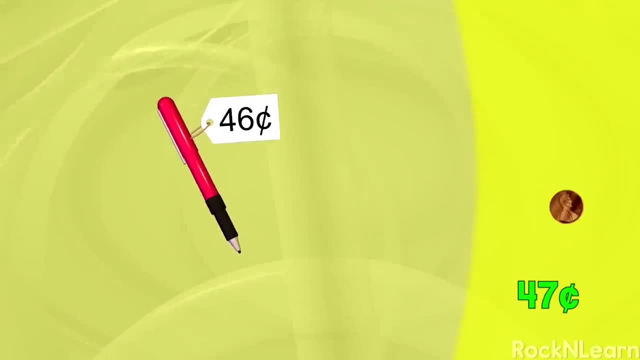 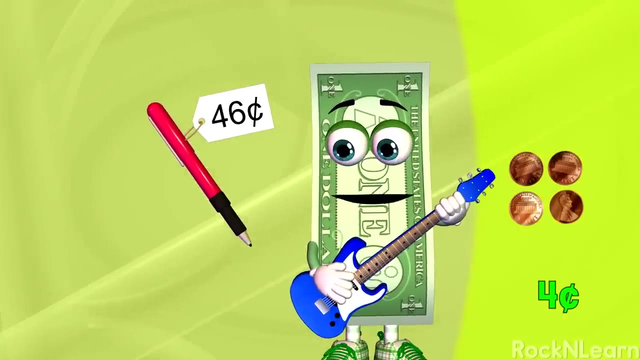 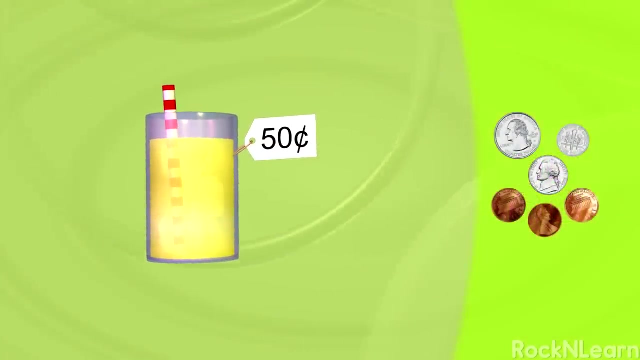 The price is forty-six, forty-seven, forty-eight, forty-nine, fifty, That's four cents back. Aw. one more cent and we'd get a nickel Yum lemonade. Do we have enough? Twenty-five, thirty-five, forty. 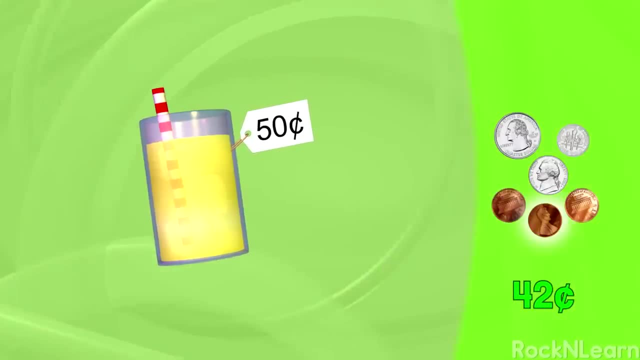 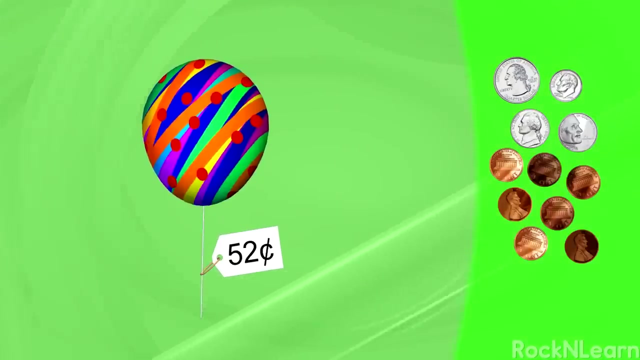 Forty-one, forty-two, forty-three, forty-three cents. Looks like we'll have to find a water fountain instead. Cool. Look at this unusual balloon. Let's see if we have enough to get it. Twenty-five, thirty-five, forty, forty-five, forty-six. 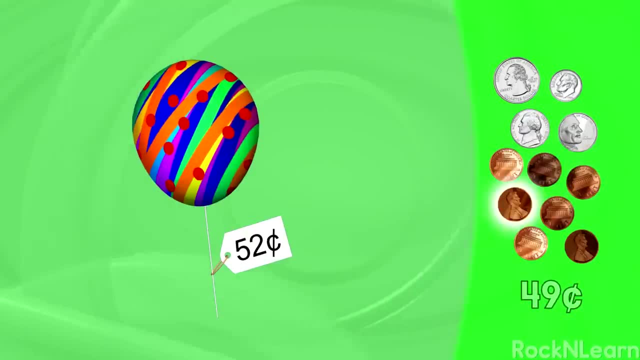 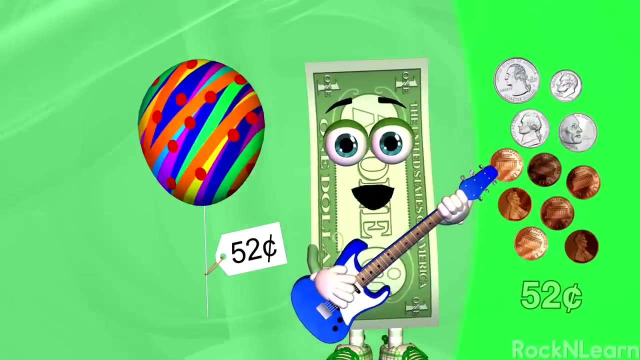 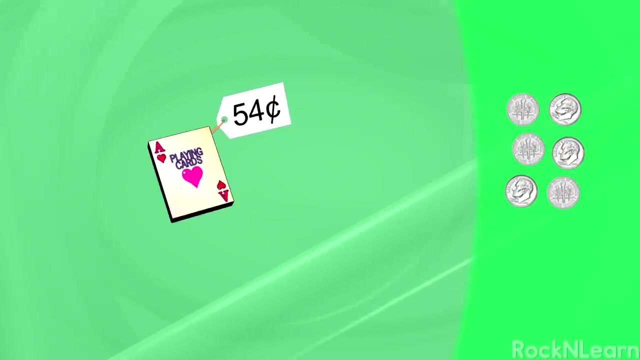 Twenty-five, thirty-five, forty-six, Forty-seven, forty-eight, forty-nine, fifty, fifty-one, fifty-two, fifty-two cents. Whew, just enough. We won't get any change back. Oh, how cute. Look how small these cards are. 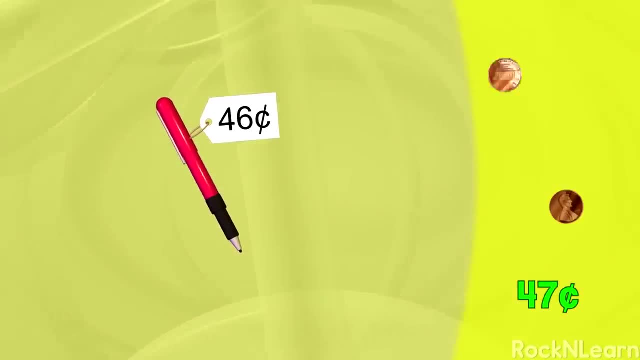 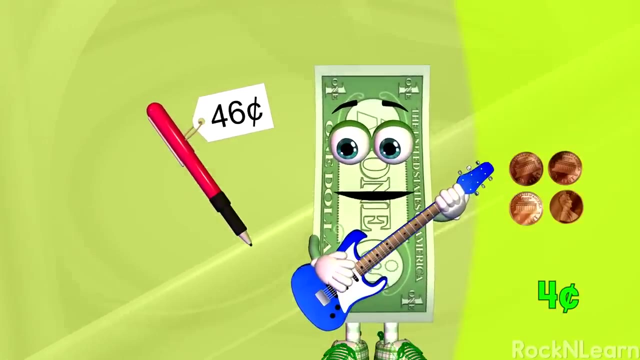 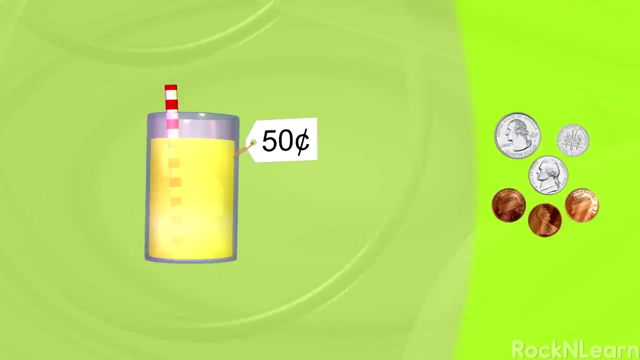 The price is forty-six, forty-seven, forty-eight, forty-nine, fifty, That's four cents back. Aw. one more cent and we'd get a nickel Yum lemonade. Do we have enough? Twenty-five, thirty-five, forty, forty-one, forty-two, forty-three, forty-three cents. 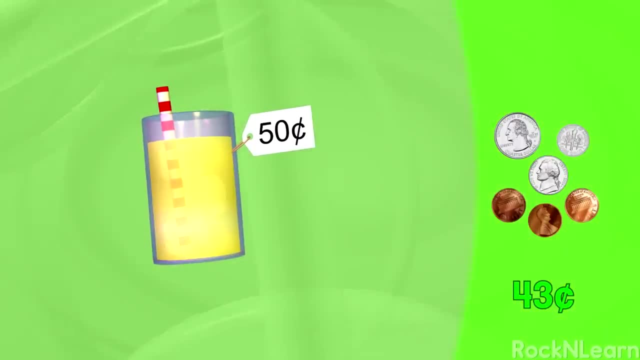 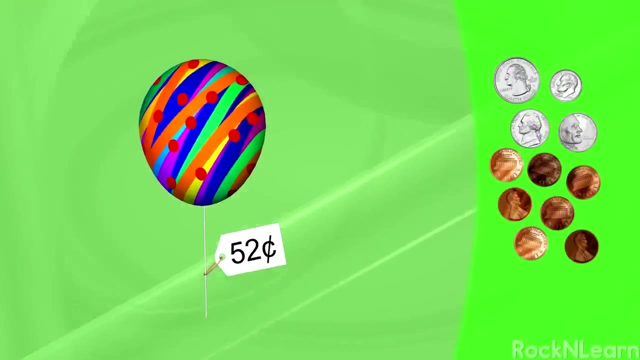 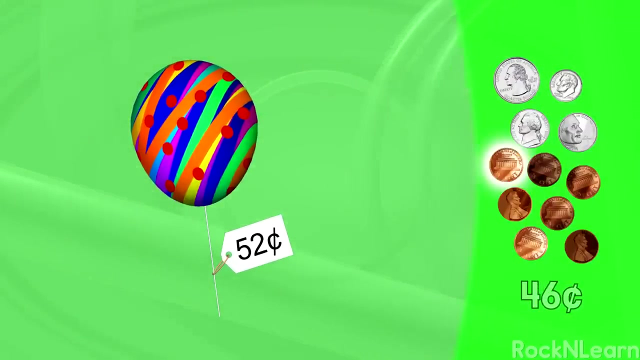 Looks like we'll have to find a water fountain instead. Cool, Look at this unusual balloon. Let's see if we have enough to get it. Twenty-five, thirty-five, forty, forty-five, forty-six, forty-seven, forty-eight, forty-nine, fifty, fifty-one, fifty-two, fifty-two cents. 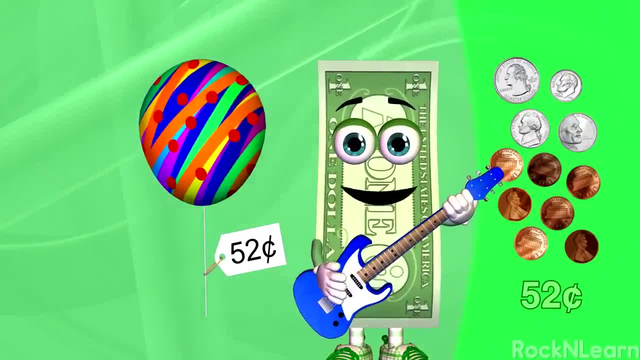 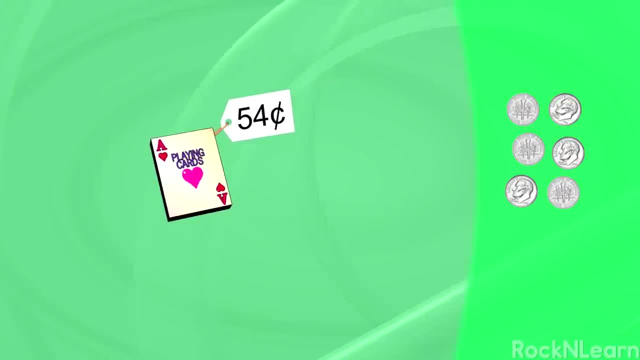 Whew, just enough. We won't get any change back. Oh, how cute. Look how small these cards are. We have ten, twenty, thirty, forty, fifty, sixty, sixty cents. That's more than enough for the cards. 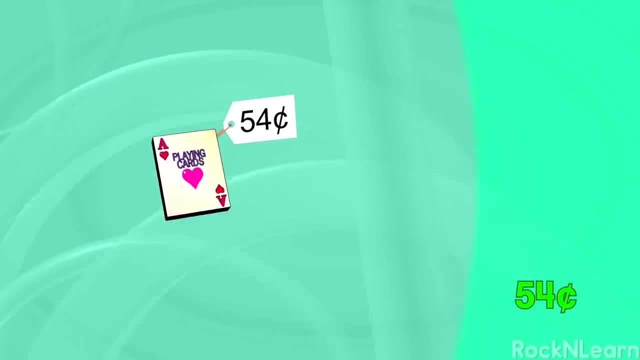 Now to calculate the change, Start with the price of fifty-four cents. Fifty-five, fifty-six, fifty-seven, fifty-eight, fifty-nine, sixty. That makes six cents. So we could get back six pennies, or one nickel and one penny. 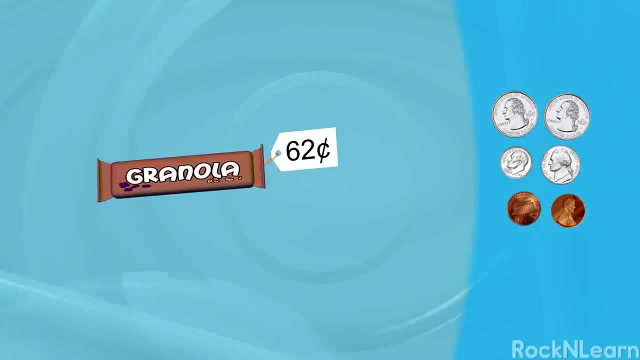 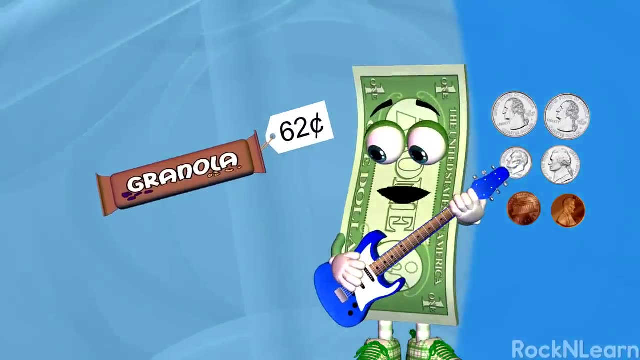 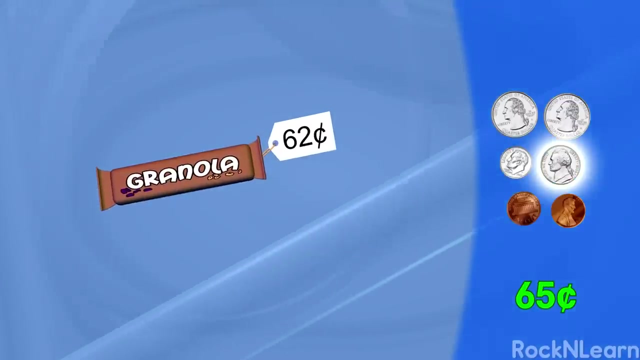 Hmm, a granola bar with nuts and raisins, And it's only sixty-two cents. That sounds raisin-able. Ugh, just count the money. Twenty-five, fifty, sixty, sixty-five, sixty-six, sixty-seven… 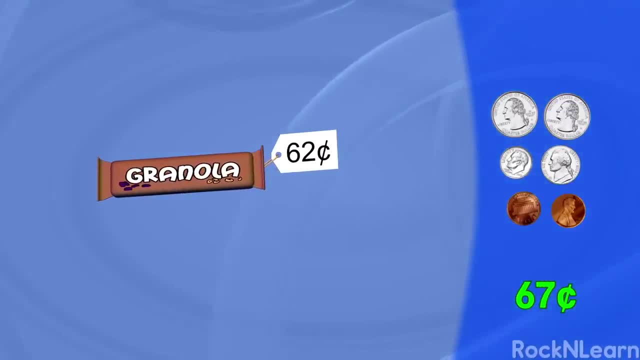 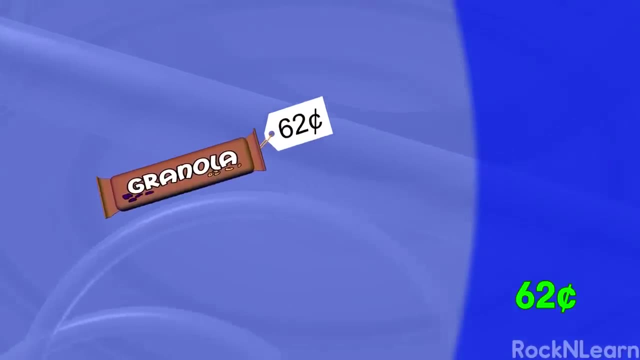 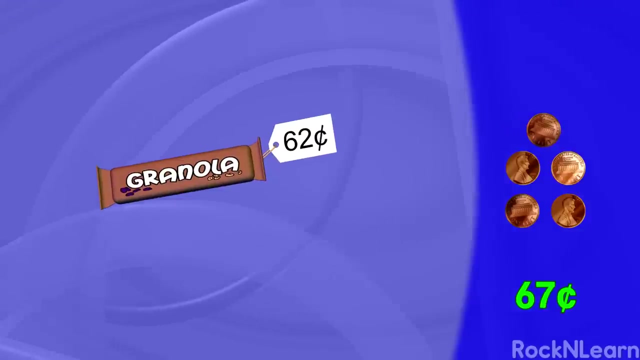 Sixty-six, sixty-seven, sixty-seven cents. That's more than enough for this granola bar. The granola bar costs sixty-two cents, And we have sixty-three, sixty-four, sixty-five, sixty-six, sixty-seven. That's five cents more than we need. 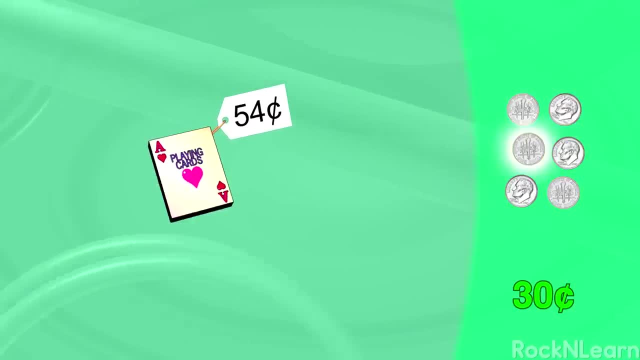 We have ten, twenty, thirty, forty, fifty, sixty, Sixty cents. That's more than enough for the cards. Now, to calculate the change, Start with the price of fifty-four cents. Fifty-five, fifty-six, fifty-seven, fifty-eight, fifty-nine, sixty. 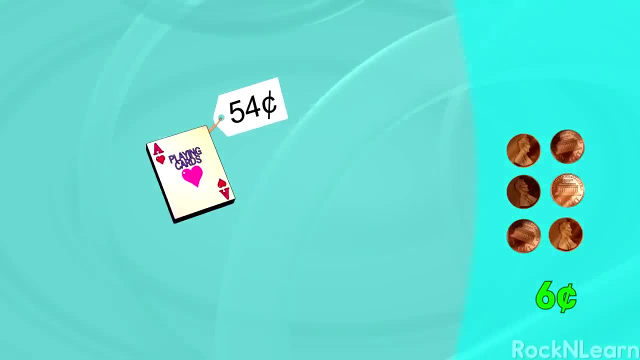 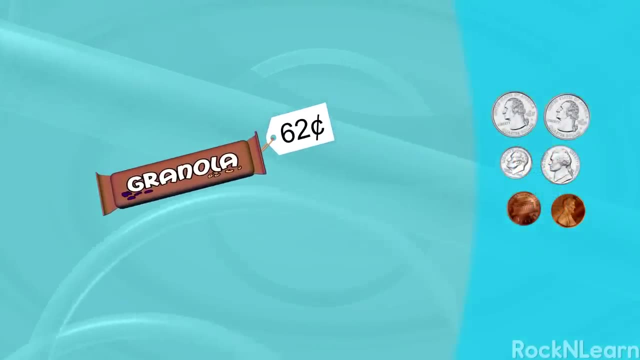 That makes six cents. So we could get back six pennies, or one nickel and one penny. Mmm, Mmm, Mmm. A granola bar with nuts and raisins, And it's only sixty-two cents. That sounds raisin-able. 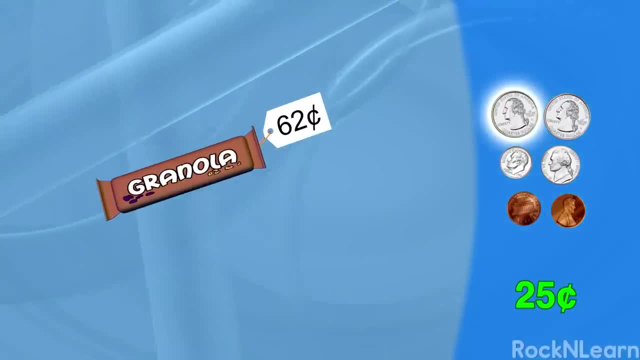 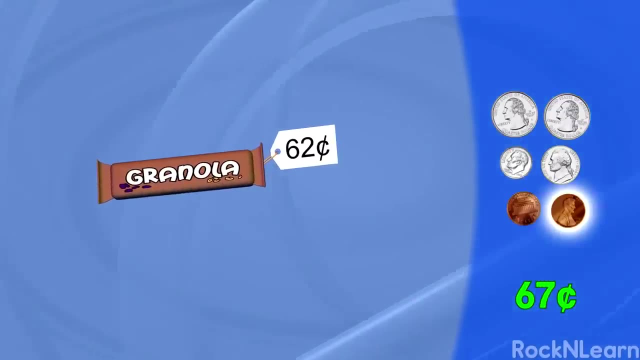 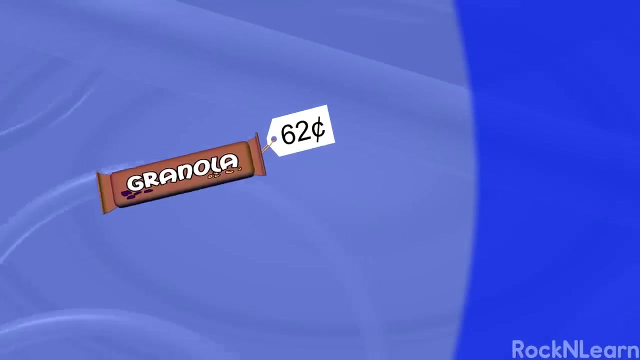 Just count the money: Twenty-five, fifty, sixty, sixty-five, sixty-six, sixty-seven, sixty-seven cents. That's more than enough for this granola bar. The granola bar costs sixty-two cents And we have sixty-three cents. 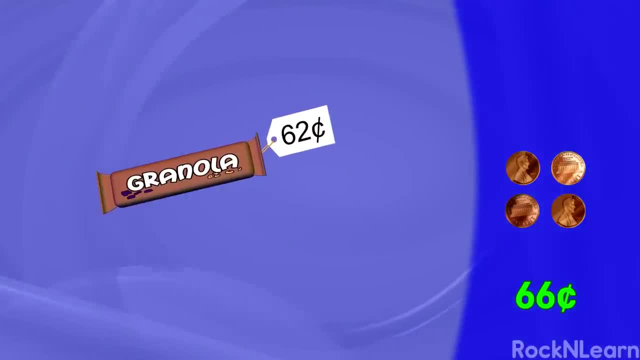 Sixty-three, sixty-four, sixty-five, sixty-six, sixty-seven- That's five cents more than we need. That means we get to keep the nickel and get the granola bar Sometimes, instead of counting all of our money first. 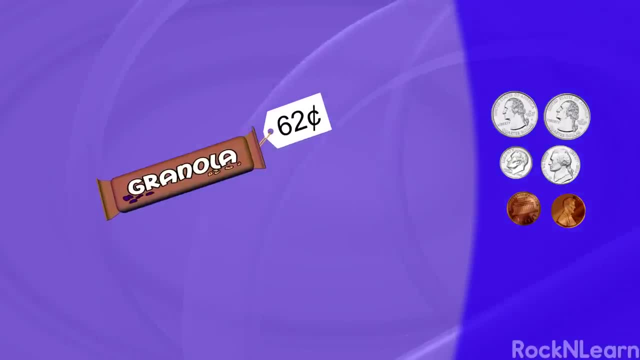 when we get close to the price of what we want, we can try to make exact change with the coins we have left. For example, if we counted this again: twenty-five, fifty, sixty, sixty-seven, sixty-eight, Sixty sixty. 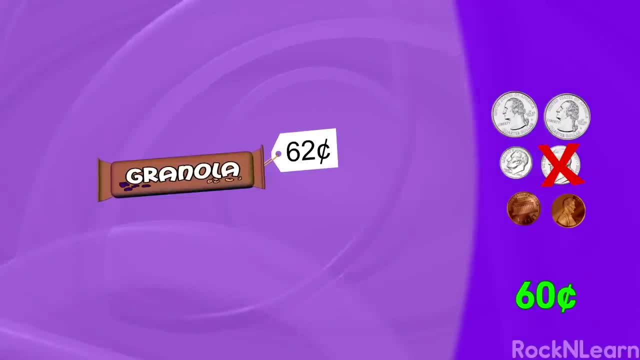 We know that the next nickel would put us over the price, So we can look to see if the pennies could give us exact change. Sixty-one, sixty-two And they can, So we don't even have to count the nickel. 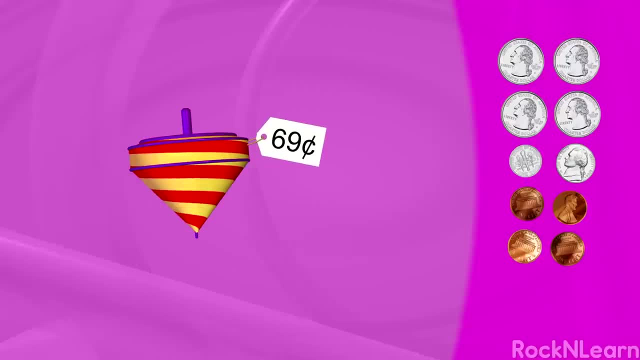 I know that four quarters make a dollar, so we have more than enough to buy this toy top. Hey Bill, why don't we use what we just learned to see if we can make exact change, No problem, Start with the biggest coins first. 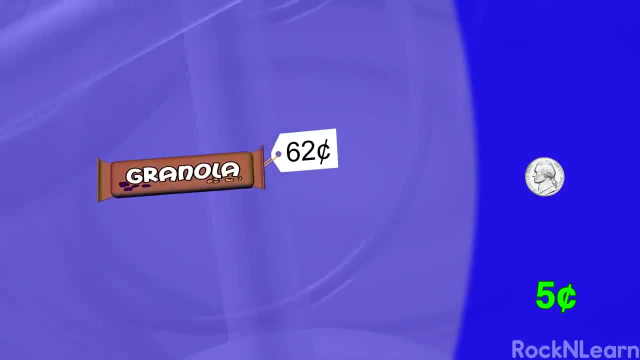 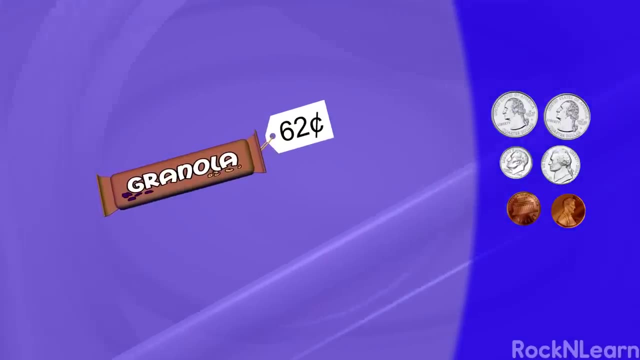 That means we get to keep the nickel and get the granola bar. Sometimes, instead of counting all of our money first, when we get close to the price of what we want, we can try to make exact change with the coins we have left. 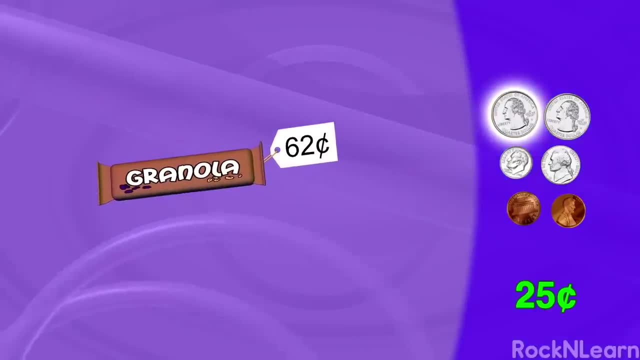 For example, if we counted this again, twenty-five, fifty, sixty, we know that the next nickel would put us over the price. So we can look to see if the pennies could give us exact change. Sixty-one, sixty-two, and they can. 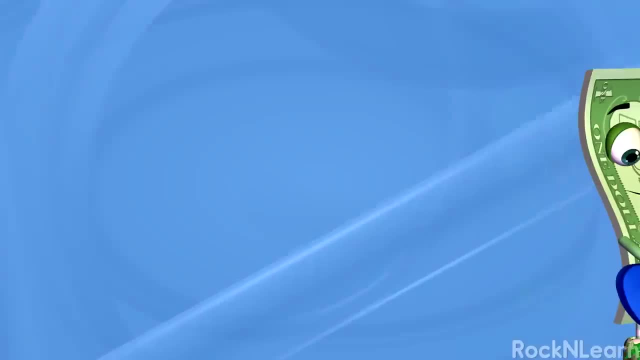 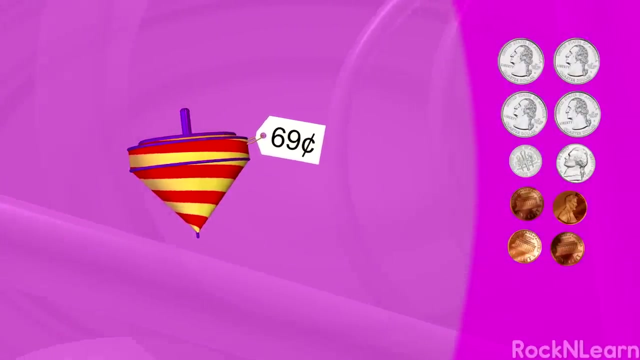 So we don't even have to count the nickel. I know that four quarters make a dollar, so we have more than enough to buy this toy top. Hey Bill, why don't we use what we just learned to see if we can make exact change? 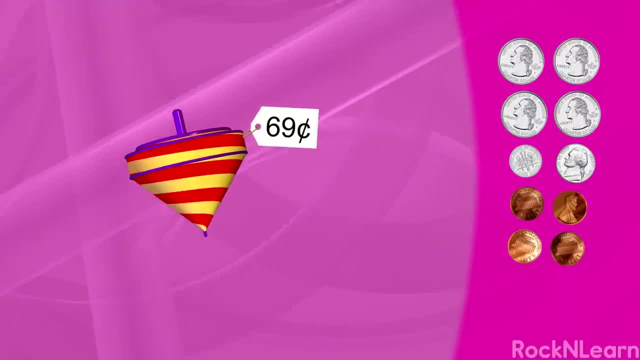 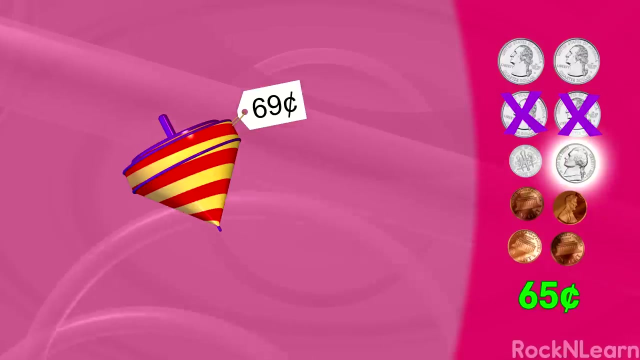 No problem, Start with the biggest coins first, Twenty-five, fifty, But stop there. One more quarter would put us over the price. Let's add the dime, That brings us to sixty cents Now, the nickel, Sixty-five, And we'll add pennies until we reach the price. 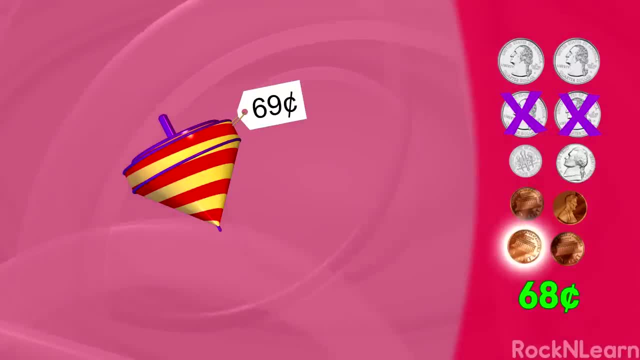 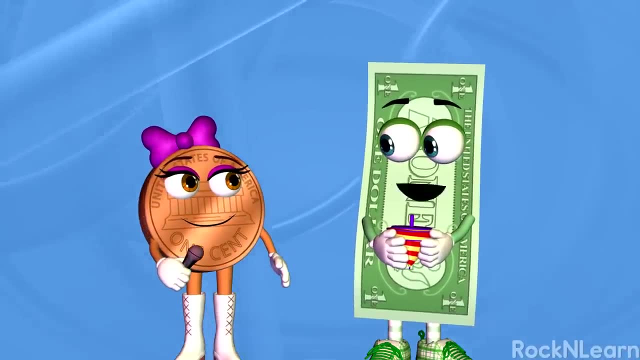 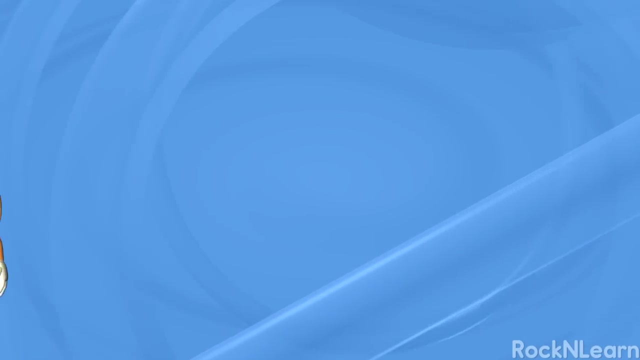 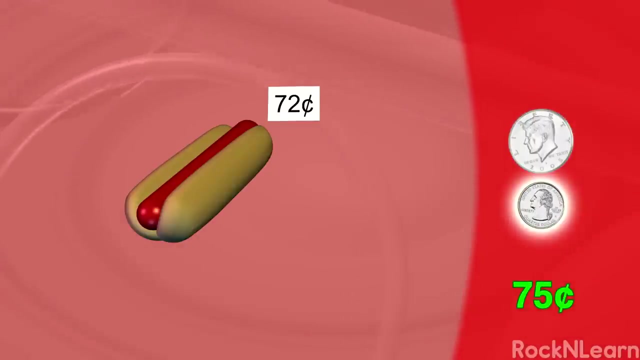 Sixty-six, sixty-seven, sixty-eight, sixty-nine, Hooray, We made exact change. Now, what do we do with a toy top? You spin it silly, Okay, Uh, This is easy. Fifty, seventy-five, we have seventy-five cents. 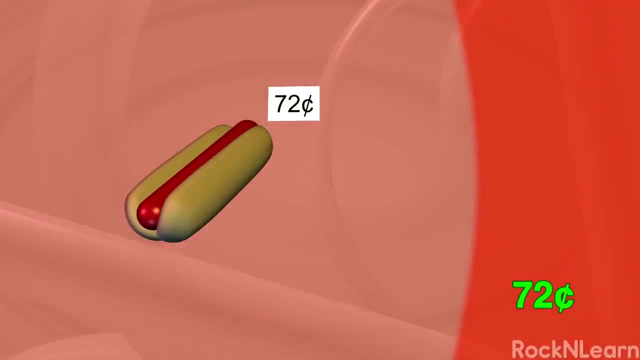 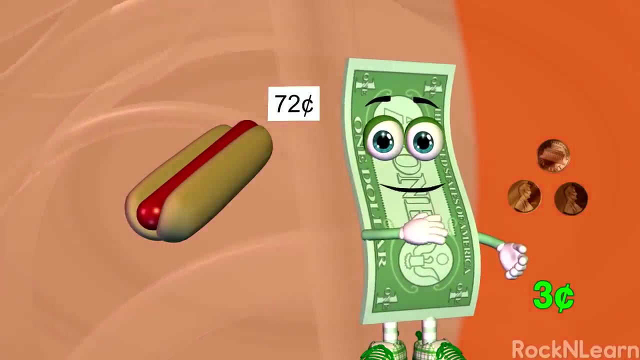 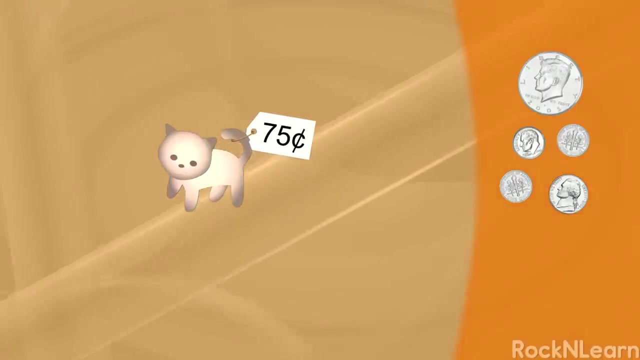 Since the hot dog is seventy-two cents, we should get seventy-three, seventy-four, seventy-five, three cents back. Hot dog, Hahaha. Oh, I love kitties. Can we buy this pin? 50, 60, 70? the other dime would put us over, but the nickel gives us 75 cents. 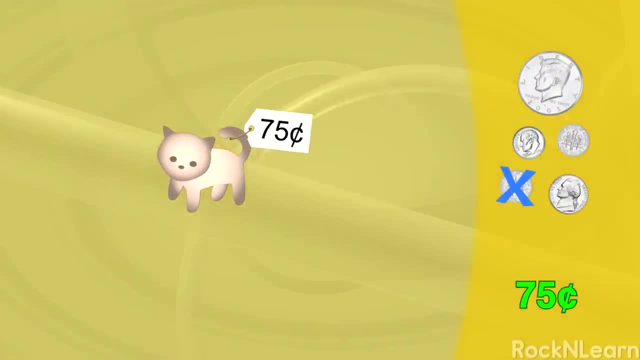 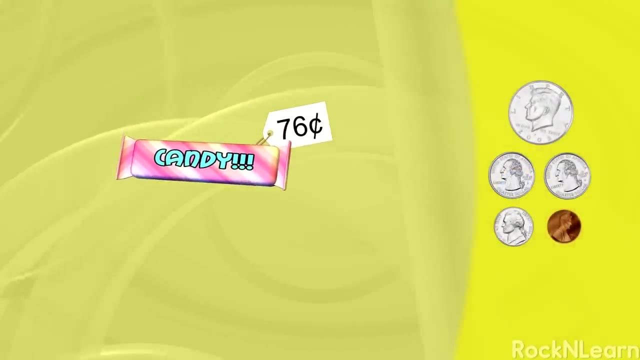 Exactly what we need. Great, I can get the pin and we can keep one dime. Mmm, that's my favorite candy bar. Let's see: 50, 75, another quarter would be over and a nickel would be over too. but one penny makes the. 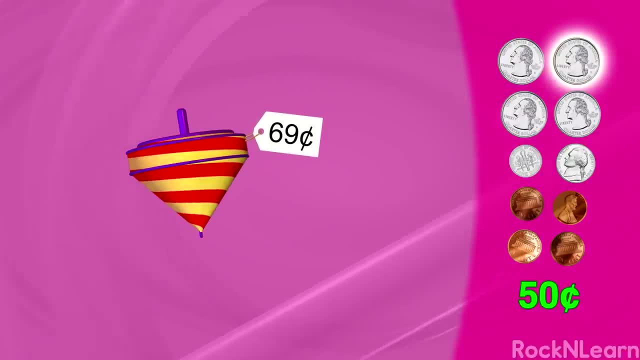 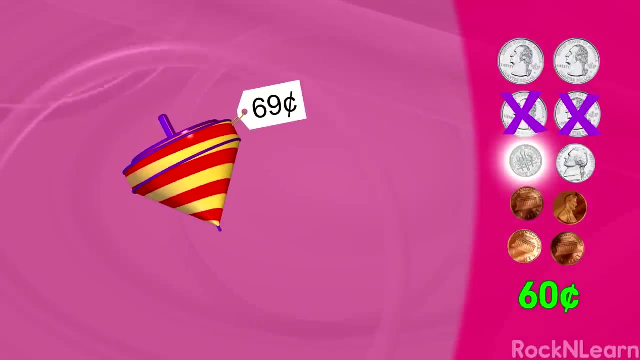 Twenty-five, fifty, but stop there. One more quarter would put us over the price. Let's add the dime, That brings us to sixty cents Now the nickel, Fifty-five, And we'll add pennies until we reach the price. 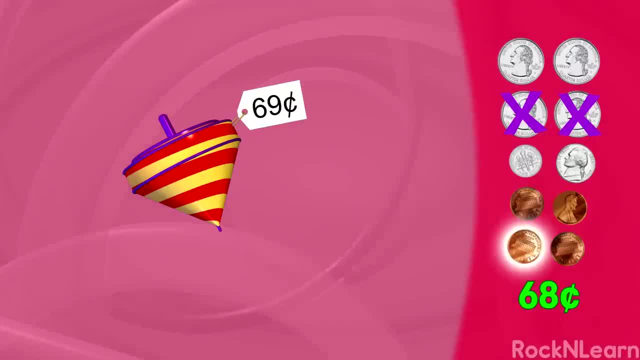 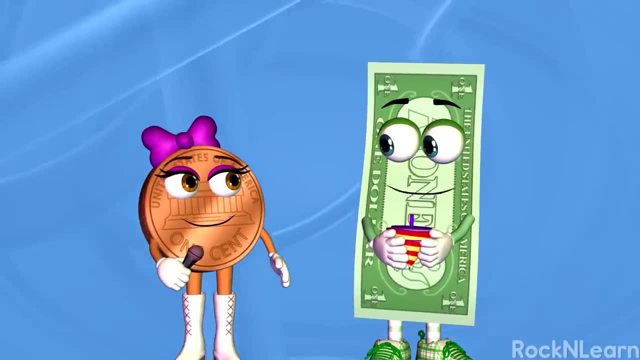 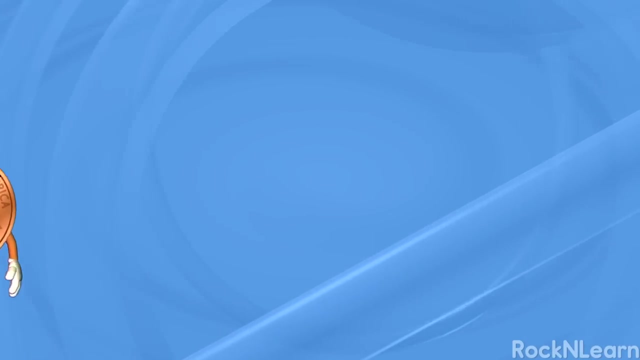 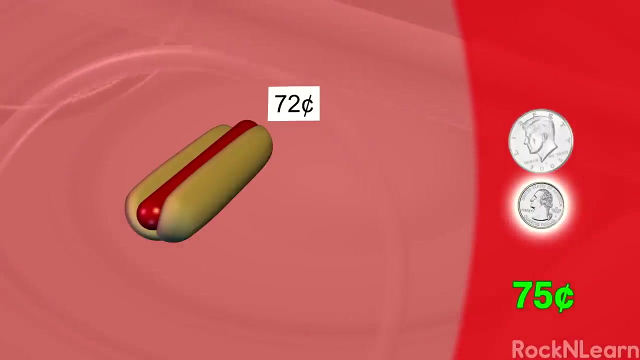 Sixty-six, sixty-seven, sixty-eight, sixty-nine. Hooray, We made exact change. Now what do we do with a toy top? You spin it silly. Okay, Ugh, This is easy. Fifty seventy-five. 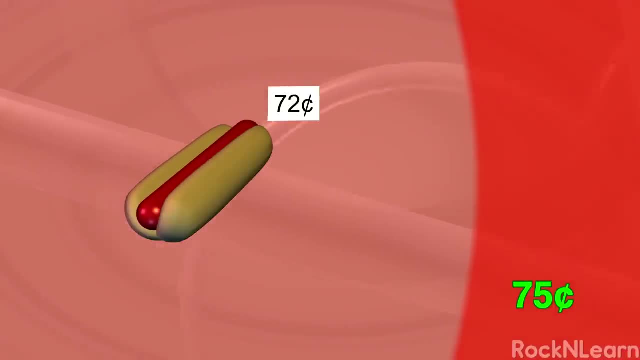 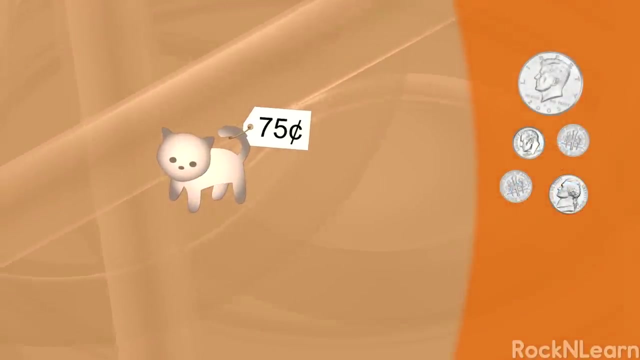 We have seventy-five cents. Since the hot dog is seventy-two cents, we should get seventy-three, seventy-four, seventy-five, three cents back. Hot dog, Oh, I love kitties. Can we buy this pin? Fifty sixty, seventy. 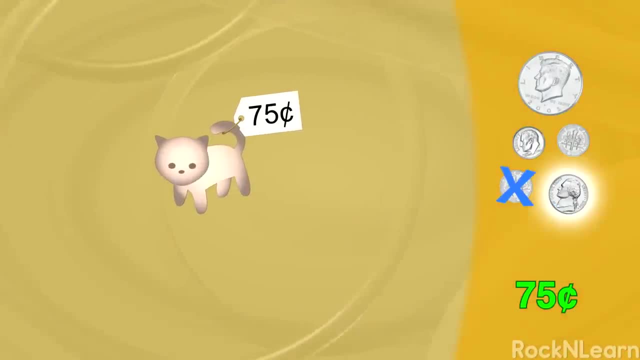 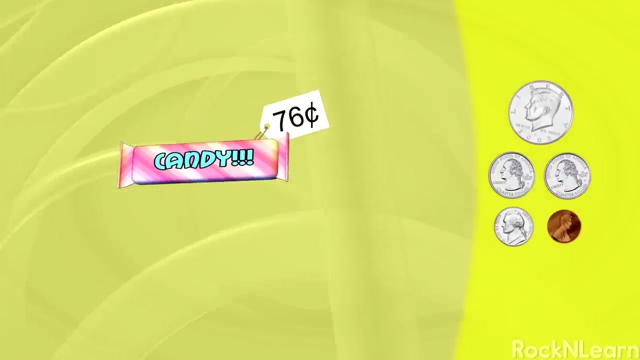 The other dime would put us over, But the nickel gives us seventy-five cents, Exactly what we need. Great, I can get the pin And we can keep one dime. Mmm, That's my favorite candy bar. Let's see. 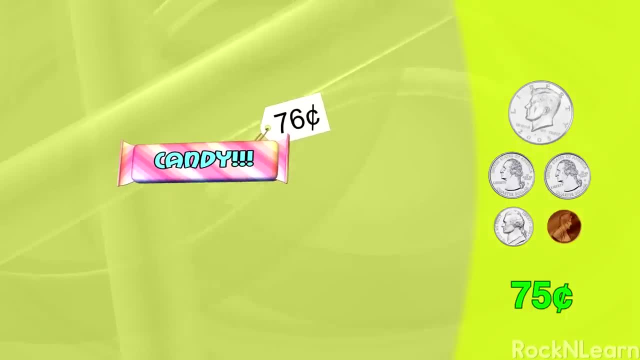 Fifty, seventy-five, Another quarter would be over And a nickel would be over too. But one penny makes the seventy-six cents we need. Cool, We had exact change And we get to keep the nickel and one quarter That makes thirty cents we can save. 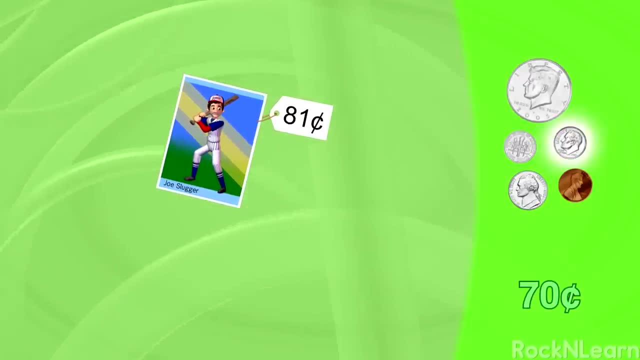 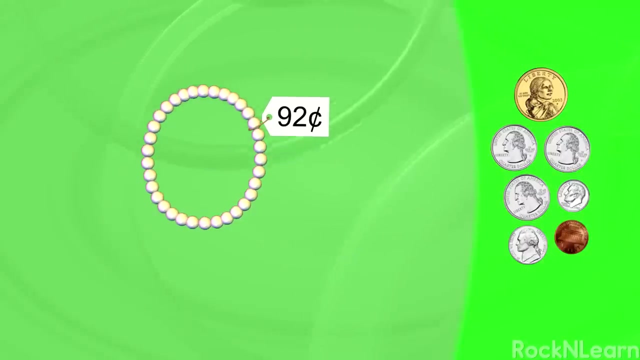 Fifty, sixty, seventy, Seventy-five, seventy-six, Only seventy-six cents. Oh man, We'll have to save up some more to get this trading card. Hmm, We could just use the dollar coin and get some change back. 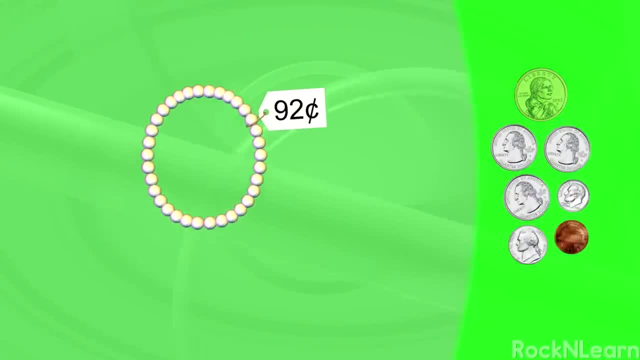 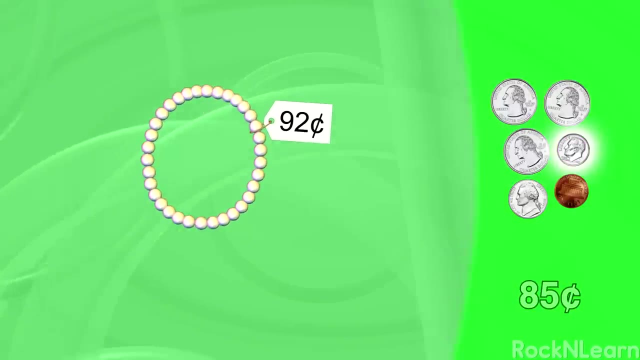 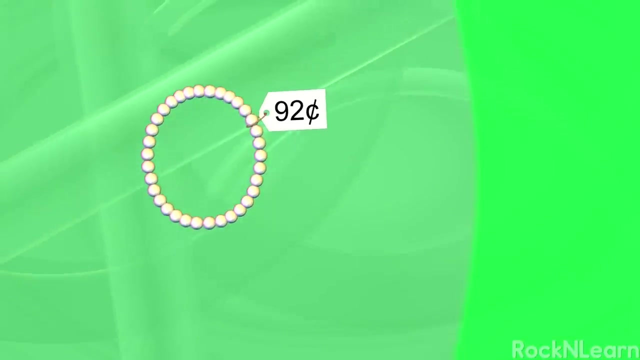 But maybe we have exact change. Let's count it and see: Twenty-five, Fifty, Seventy-five, Eighty-five, Ninety, Ninety-one- Only one penny off. Looks like you're going to have to use the dollar coin. 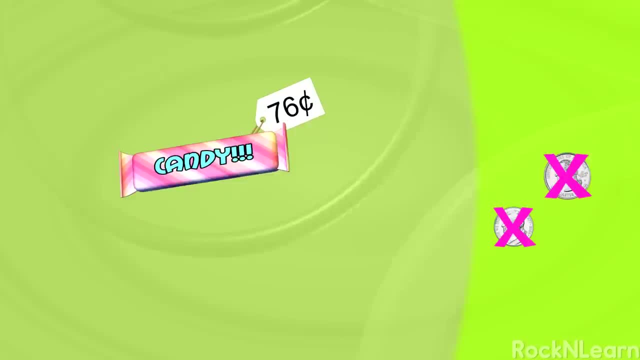 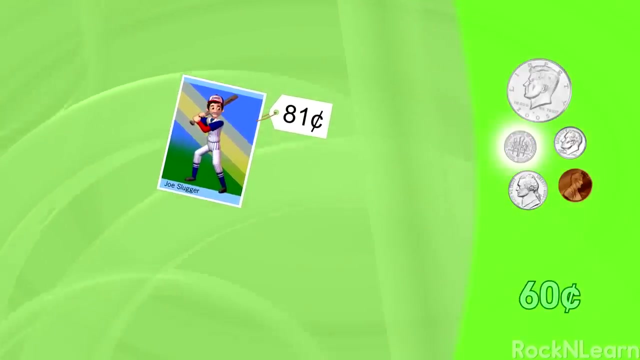 76 cents. we need Cool. we had exact change and we get to keep the nickel and one quarter. That makes 30 cents. we can save 50, 60, 70, 75, 76 only, Oh man, we'll have to save up some more to get this trading card. 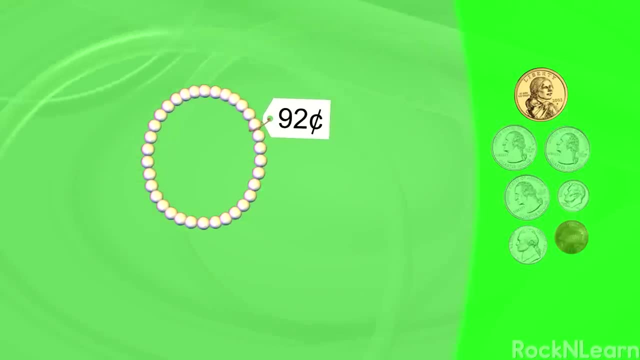 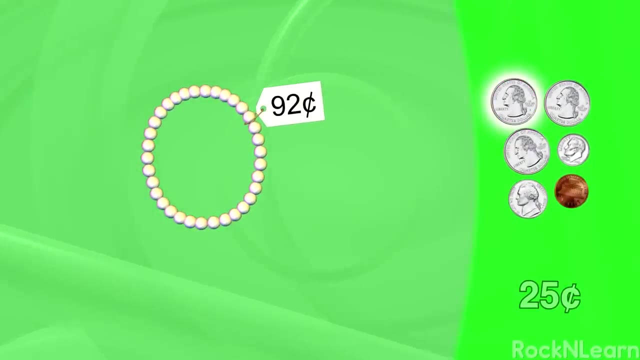 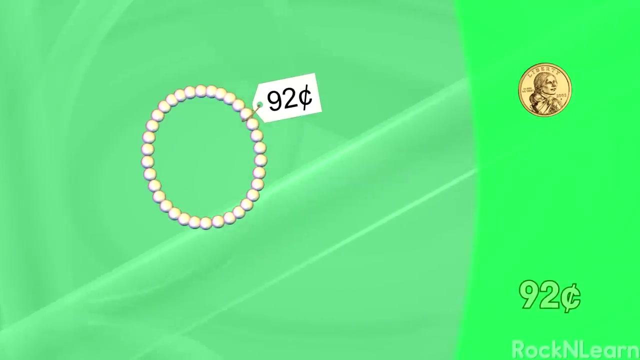 Hmm, we could just use the dollar coin and get some change back. But maybe we have exact change. Let's count it and see: 25, 50, 75, 85, 90, 91. ah, only one penny off. Looks like you're going to have to use the dollar coin. The bracelet is 92 cents. 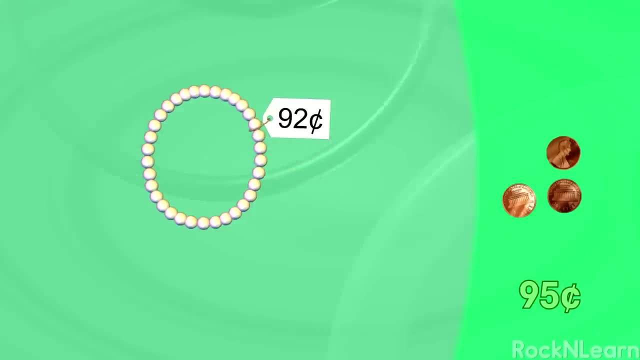 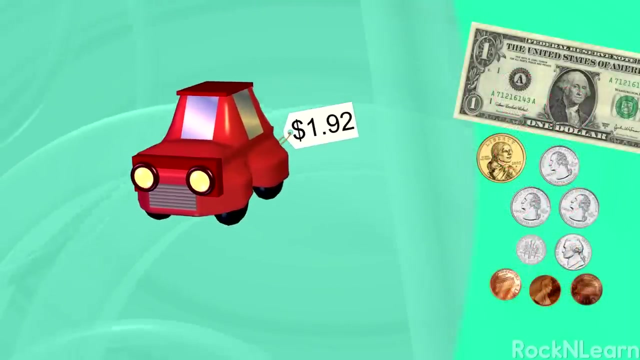 93 94 95, That's three pennies and five more cents. or a nickel brings us to the dollar, I get eight cents change and you get to keep the quarters dime, nickel and penny. now That's what I call a compact car. I get to sit up front. 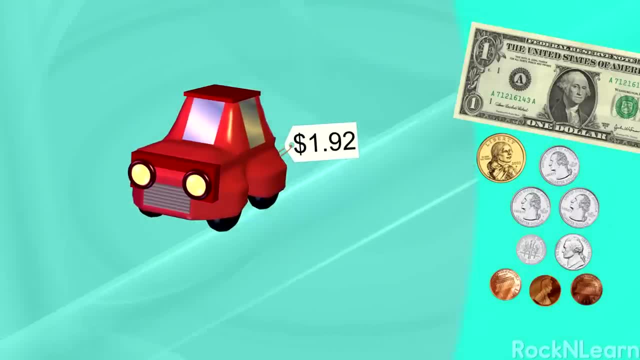 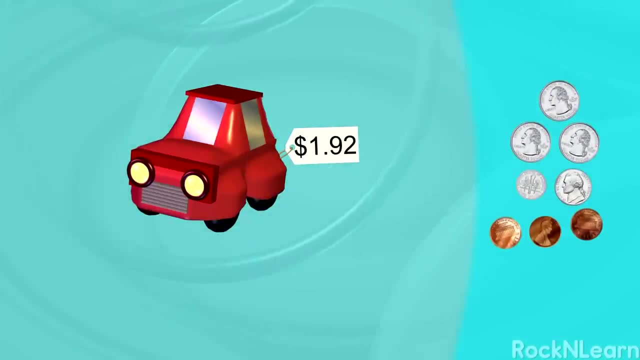 Only if you're the size of a penny. We could just use the dollar bill and the dollar coin. But let's check to see if we can make exact change: 25, 50,, 75,, 85,, 90,, 91,, 92.. 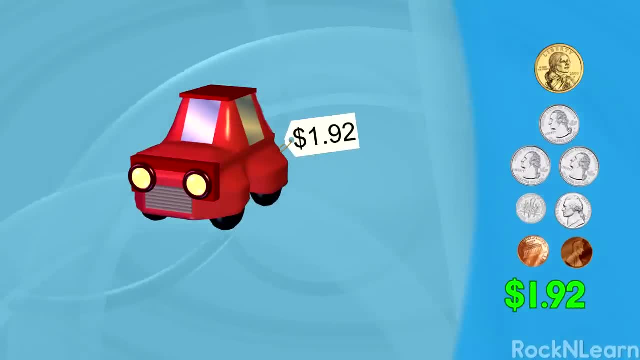 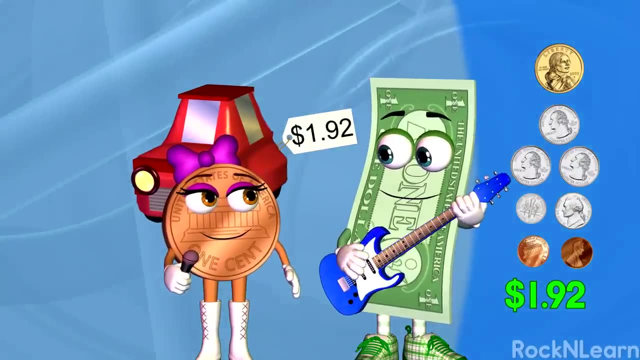 Hey, we can. Let's use the dollar coin with the $0.92 you counted to buy the toy car. Yeah, the dollar bill won't be as heavy in my pocket. Um, maybe I should carry that in my purse. You can drive the car. 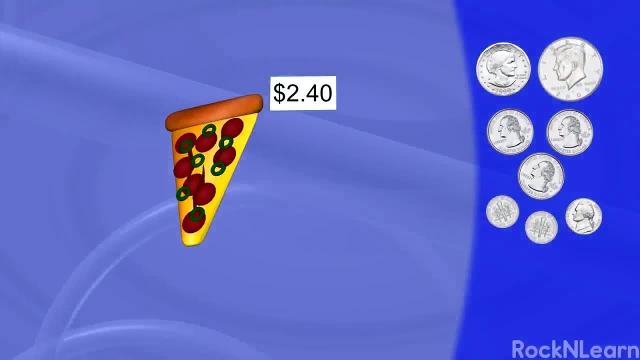 Mamma mia, pepperoni and green olives with anchovies. Ew, Let's see $1,, 50,, 75,, $2,, 20.. 25,, 35. Another dime would be too much, But the nickel makes exactly the $2.40. 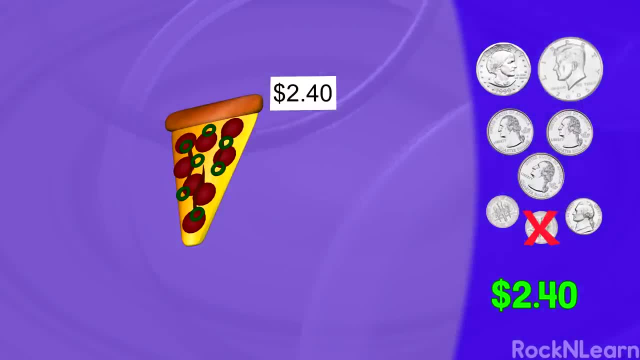 we need for that icky pizza slice, Exactly Exact change that is, And we have one of the dimes left over. I have a feeling that pizza's going to be left over too. It might actually be good if it didn't have the anchovies. 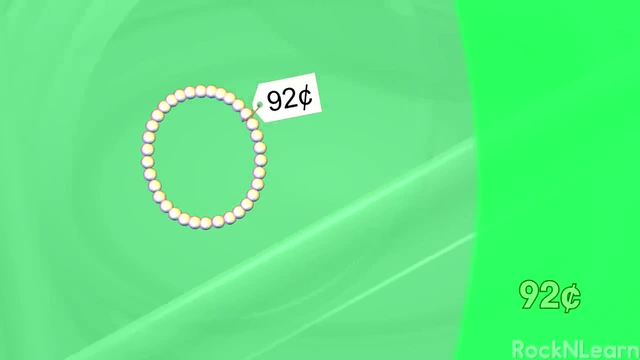 The bracelet is ninety-two cents, Ninety-three, Ninety-four, Ninety-five, That's three pennies And five more cents, or a nickel brings us to the dollar. I get eight cents change And you get to keep the quarters dime, nickel and penny. 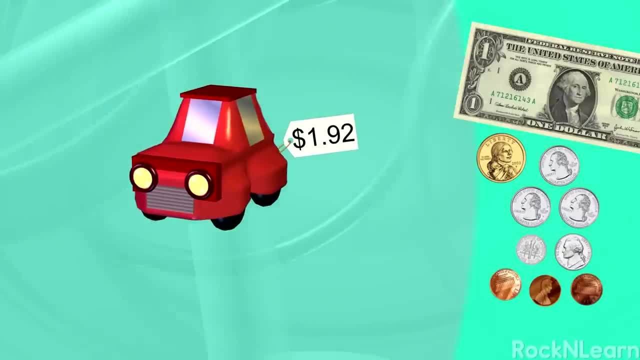 Now that's what I call a compact car. I get to sit up front Only if you're the size of a penny. We could just use the dollar bill and the dollar coin. But let's check to see if we can make exact change. 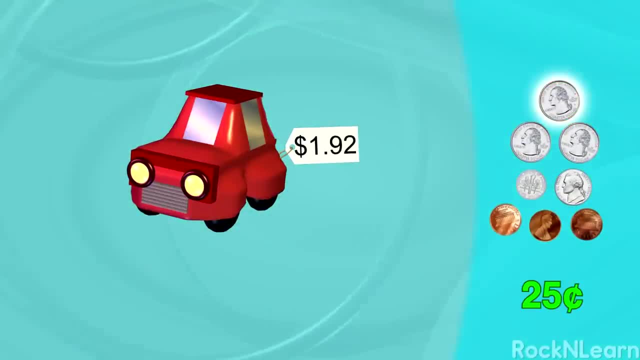 Twenty-five, Fifty, Seventy-five, Eighty-five, Ninety, Ninety-one, Ninety-two. Hey, We can. Let's use the dollar coin with the ninety-two cents you counted to buy the toy car. Yeah, The dollar bill won't be as heavy in my pocket. 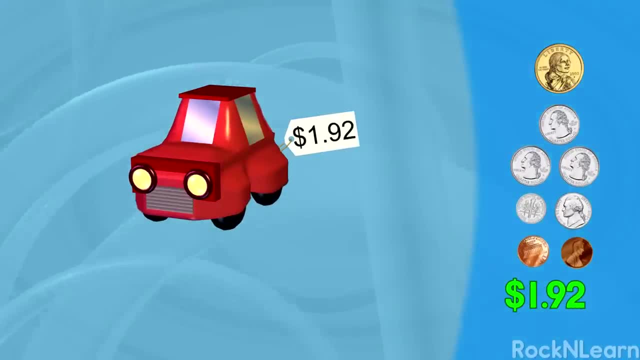 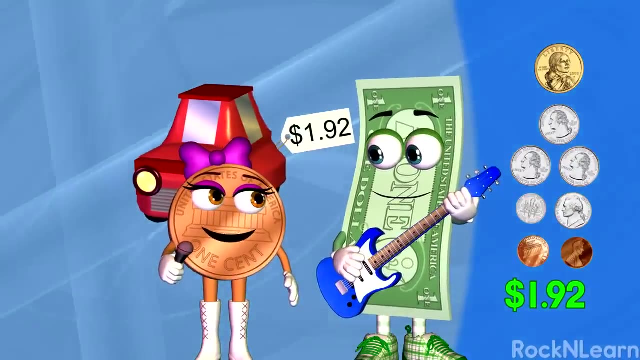 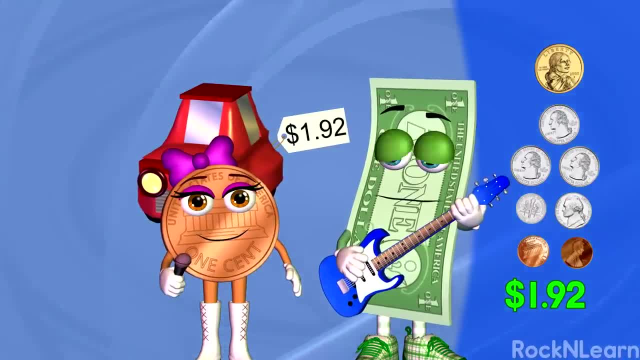 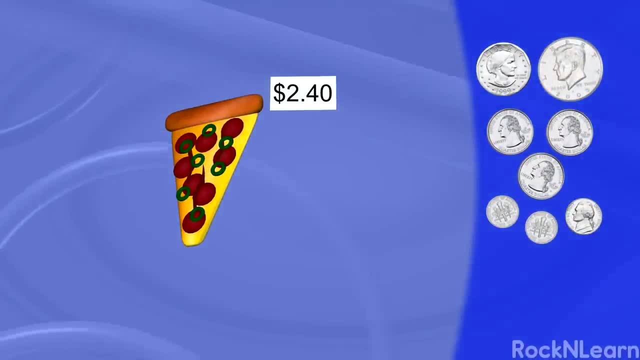 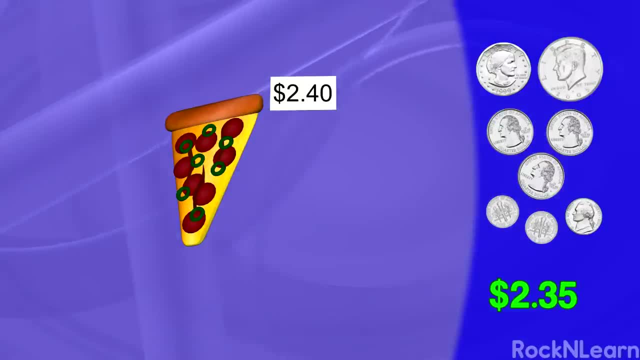 Twenty-five, Thirty-five, Another dime would be too much, But the nickel makes exactly the two dollars and fifty cents. At least that's how much the dollar will be equivalent to one dollars. Yeah, Exactly, At least that's how much the dollar will be equivalent to one dollars. 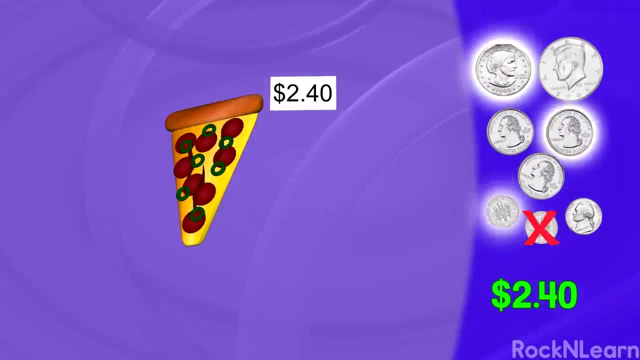 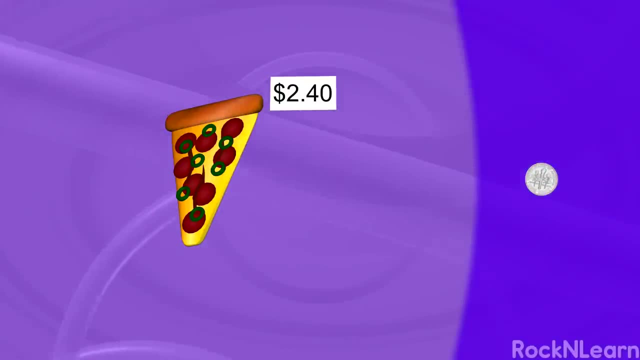 and 40 cents we need for that icky pizza slice- Exactly Exact change that is, And we have one of the dimes left over. I have a feeling that pizza's gonna be left over too. It might actually be good if it didn't have the anchovies. 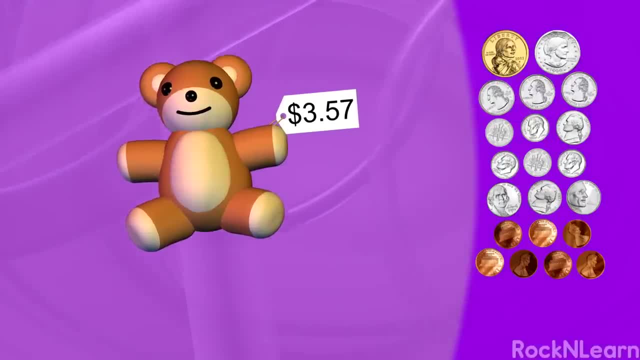 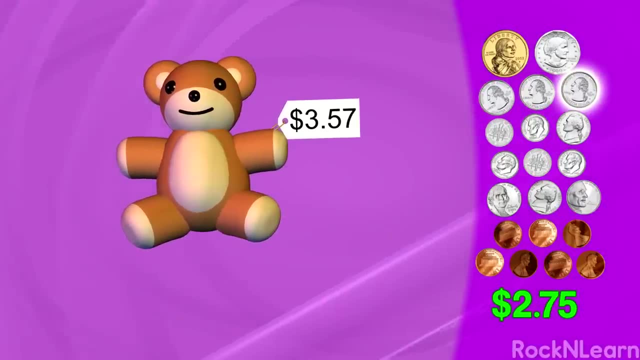 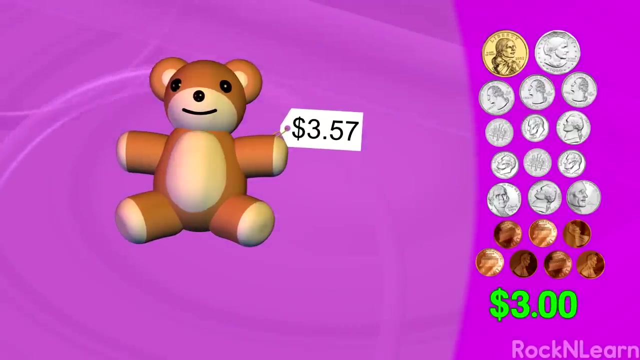 What a cute bear. Ooh, do we have enough? $1,, $2,, $25,, $50,, $75,, $85,, $95, and one of the nickels makes $3.. Now back to the dimes. 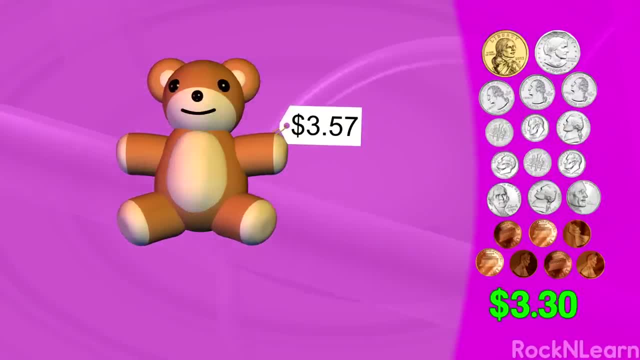 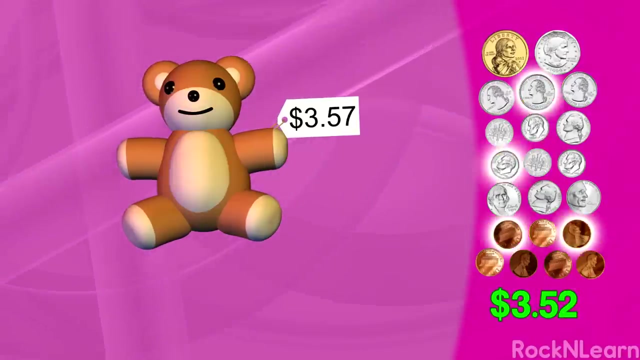 $10, $20, $30,, the remaining nickels $35, $40, $45, and the pennies $46, $47,, $48,, $49,, $50, $51.. $52.. Aw, we're five cents short. 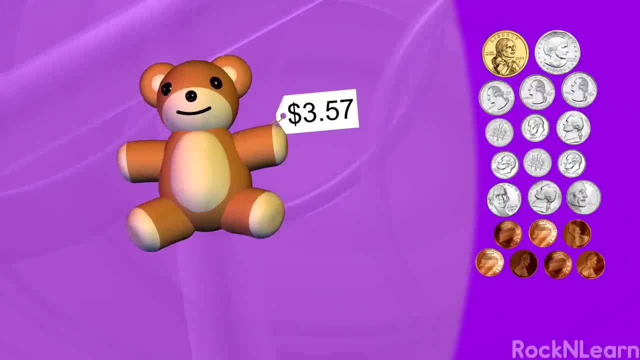 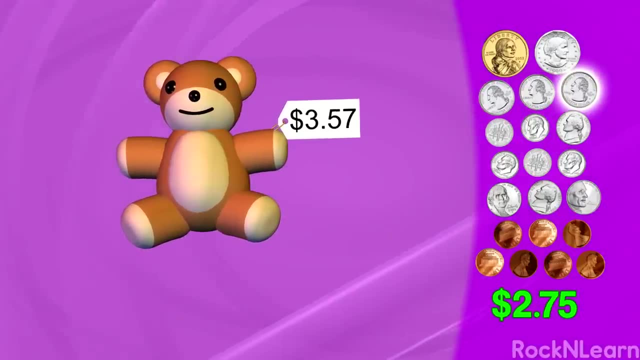 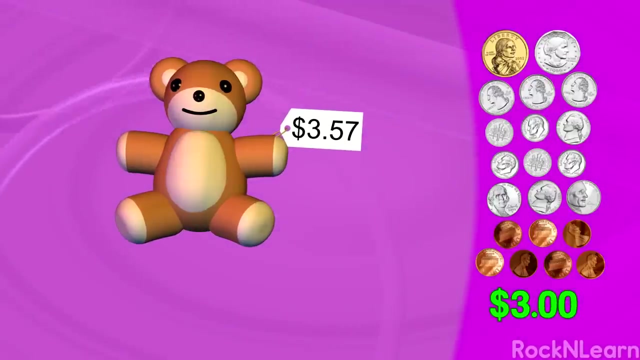 What a cute, A cute bear. Ooh, do we have enough? $1,, $2,, 25,, 50,, 75,, 85,, 95.. And one of the nickels makes $3.. Now back to the dimes. 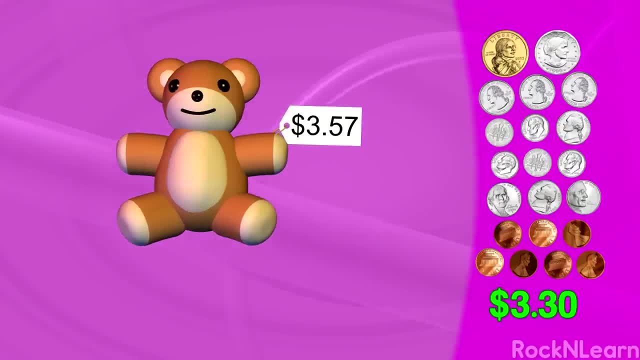 10,, 20, 30.. The remaining nickels 35,, 40, 45. And the pennies 46,, 47, 48.. $2.70.. $2.70.. Forty-nine, fifty, fifty-one, fifty-two. 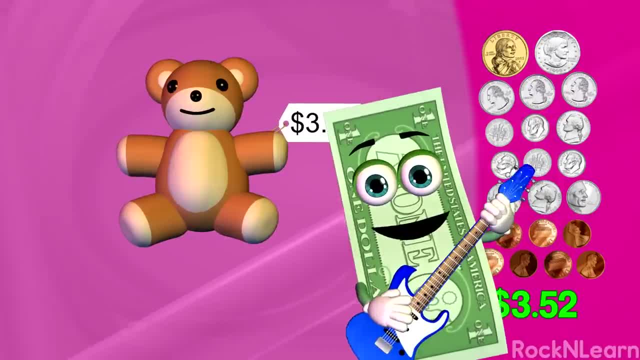 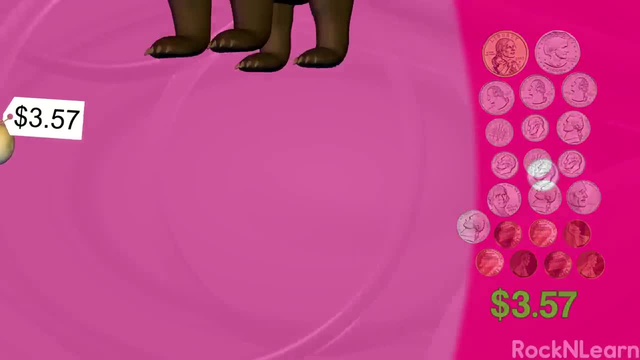 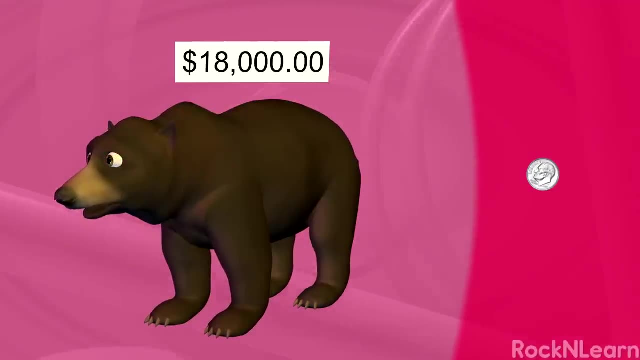 Aw, we're five cents short. I can barely stand it Here. I found a nickel in the parking lot. Thanks, Bill. Hey, look A real bear. Can I take him home? Are you kidding? That bear would eat everything in sight. 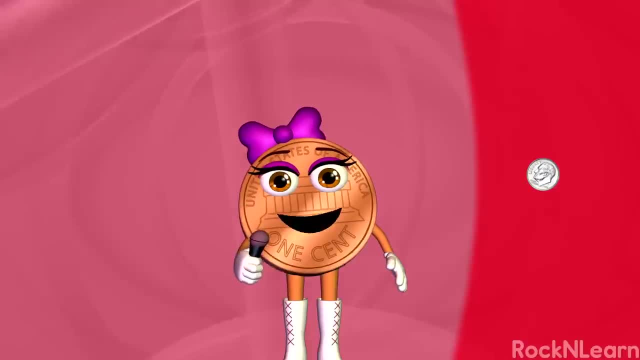 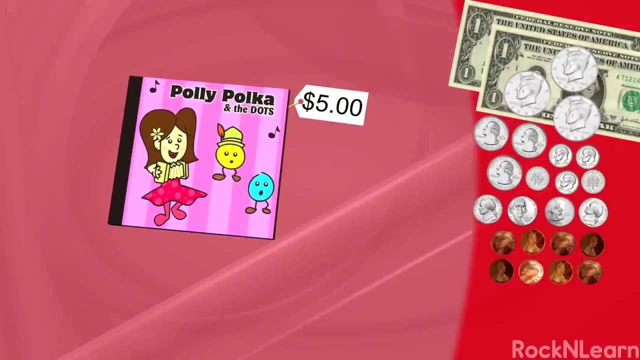 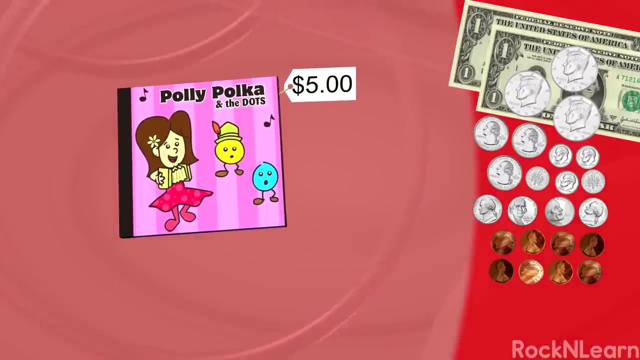 You're probably right. Besides, I think we may be a little short on change. Check out this CD I found in the bargain bin. I'll bet it's hilarious And it's only five dollars. Let's see if we have enough. 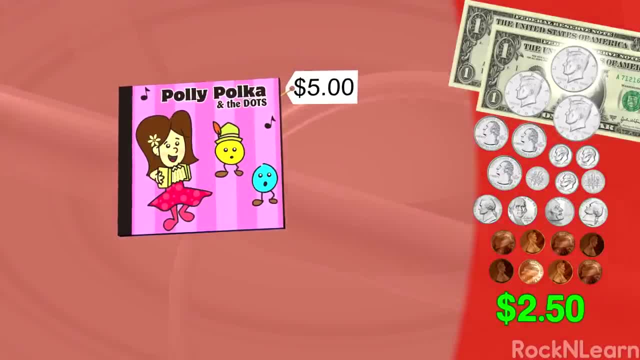 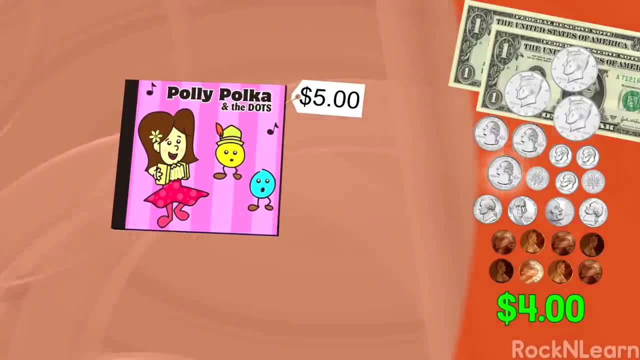 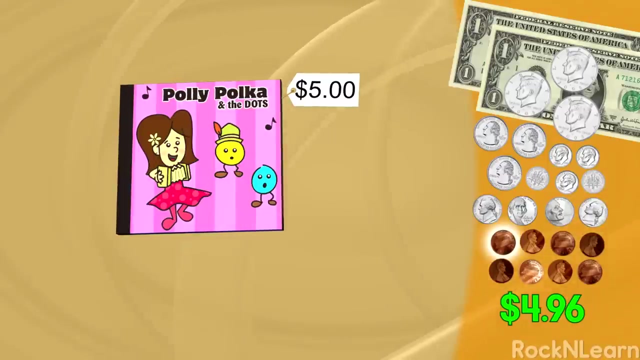 One dollar, two dollars, fifty cents. Three dollars fifty, seventy-five, Four dollars twenty-five, thirty-five, Forty-five, fifty-five, sixty-five, seventy-five, Eighty, eighty-five, ninety, ninety-five, Ninety-six, ninety-seven, ninety-eight, ninety-nine. 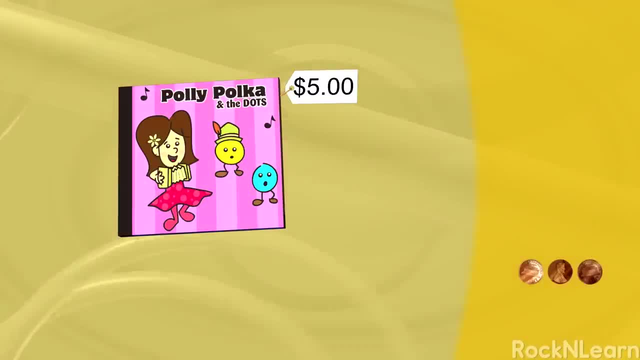 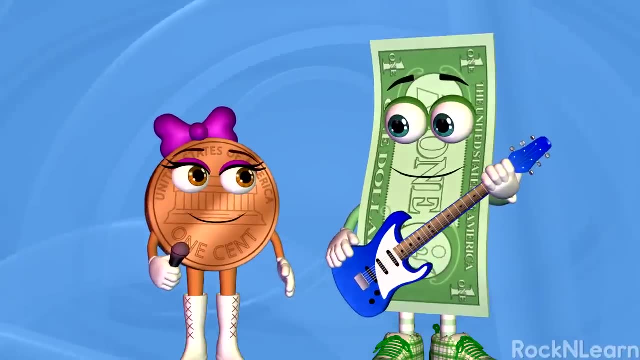 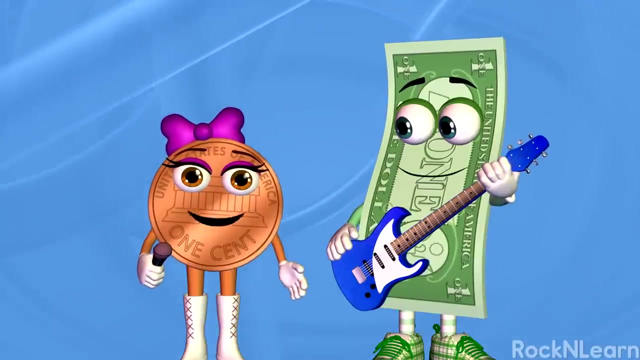 Five dollars. So we get the CD and we have three pennies left over. You know the price tag on an item is not always the final sales price. Yeah, sometimes they add on tax at the register. So if you wanna buy something, be sure you have enough money to pay. 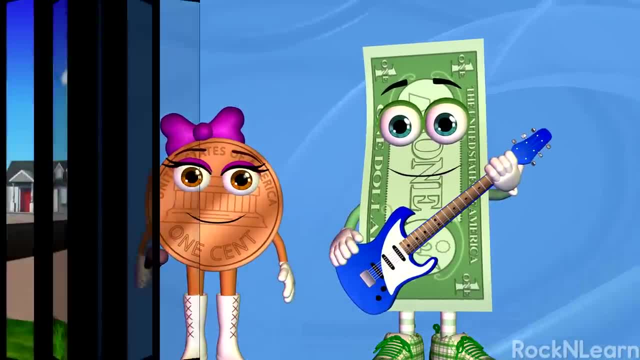 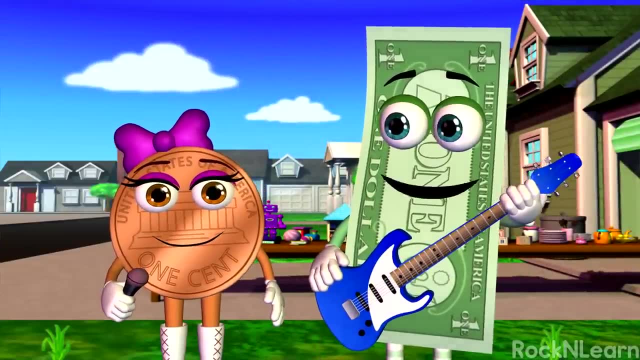 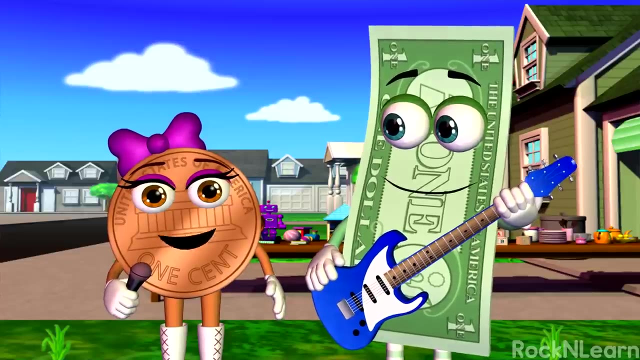 for it and cover the sales tax. There are times when you need to be the person that makes correct change, Like at a lemonade stand or a bake sale, Or if you help out at a garage sale. Yeah, So it's a good idea to know how to make change. 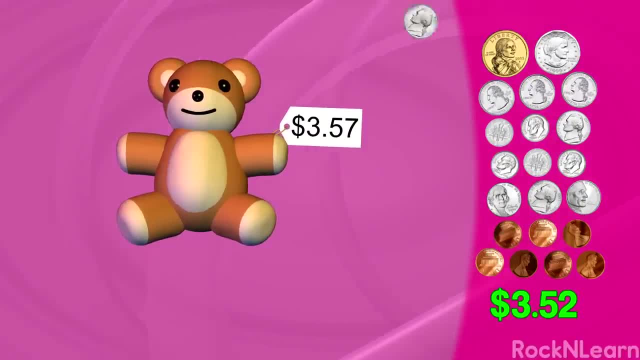 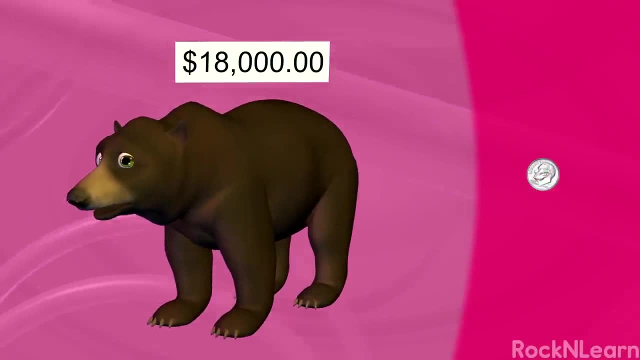 I can barely stand it Here. I found a nickel in the parking lot. Thanks, Bill. Hey, look a real bear. Can I take him home? Are you kidding? That bear would eat everything in sight. You're probably right. 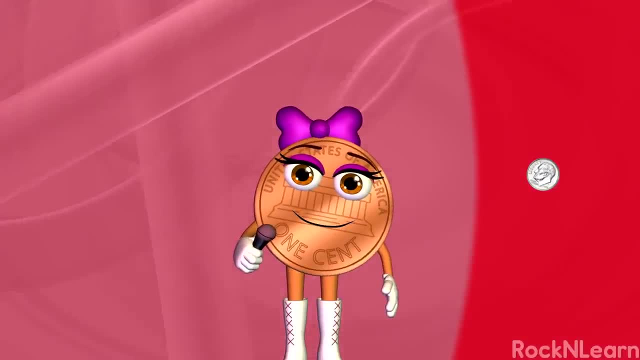 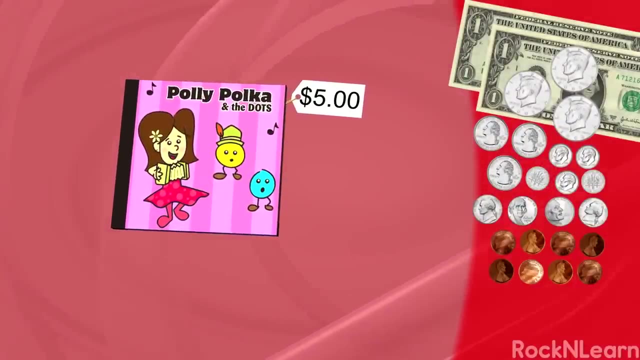 Besides, I think we may be a little short on change, I hope. Alright, then I'll buy you some peanuts. We'll have the 경량. I like the wind and wind. Let's get started. Check out this CD I found in the bargain bin. 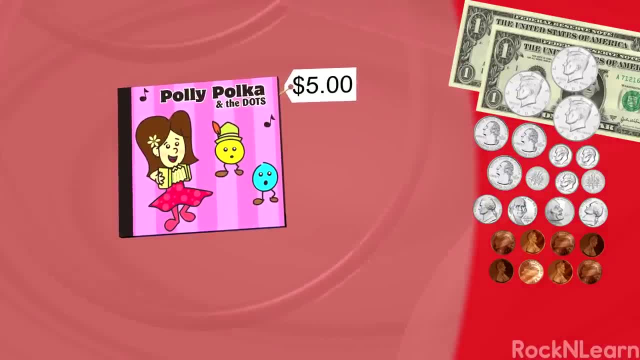 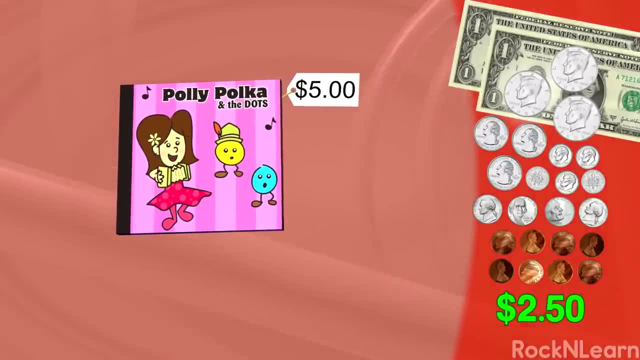 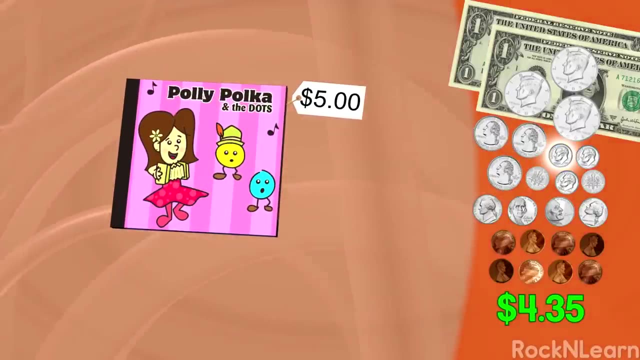 I'll bet it's hilarious And it's only $5.. Let's see if we have enough. $1, $2, 50 cents, $3, $50, $75.. $4, $25, $35, $45, $55, $60.. 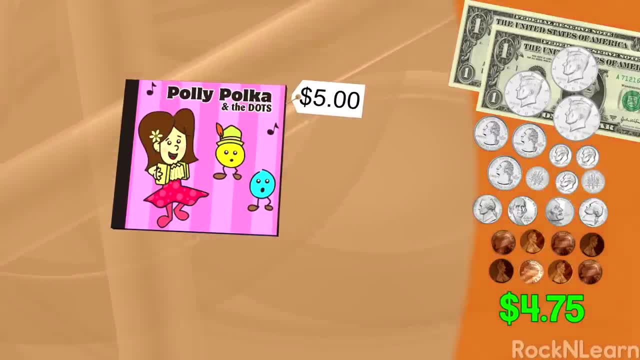 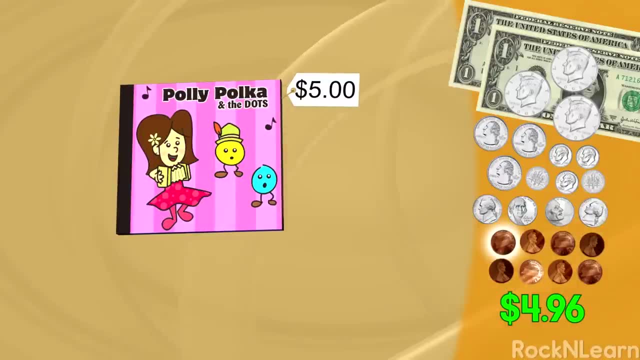 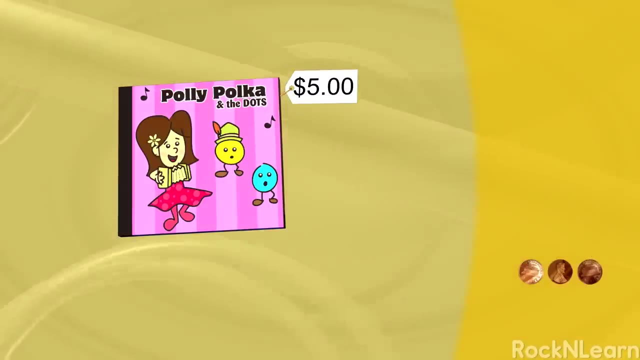 $10,, $45,, $55,, $65.. 65,, 75,, 80,, 85,, 90,, 95,, 96,, 97,, 98,, 99,, $5.. So we get the CD and we have three pennies left over. 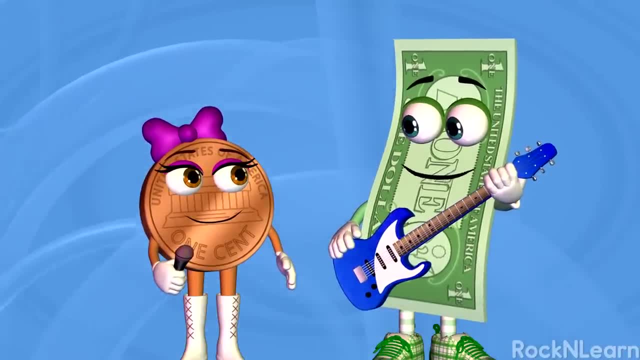 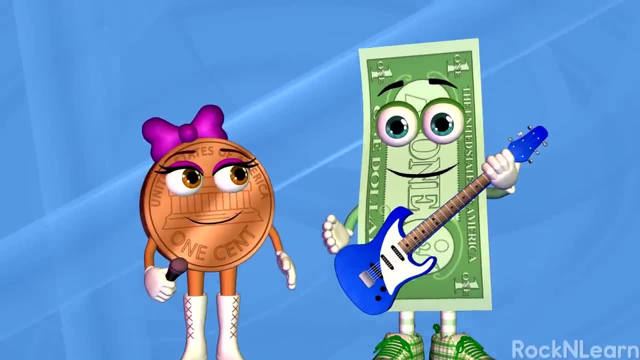 You know the price tag on an item is not always the final sales price. Yeah, sometimes they add on tax at the register. So if you want to buy something, be sure you have enough money to pay for it and cover the sales tax. 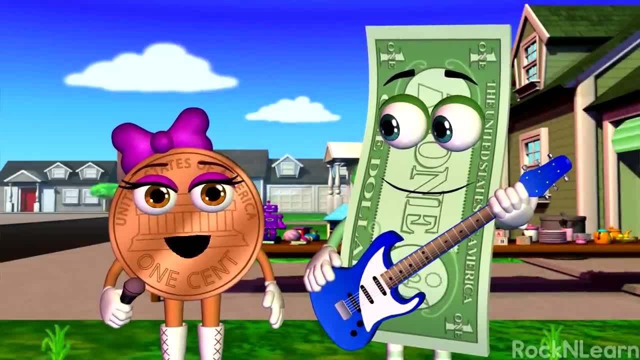 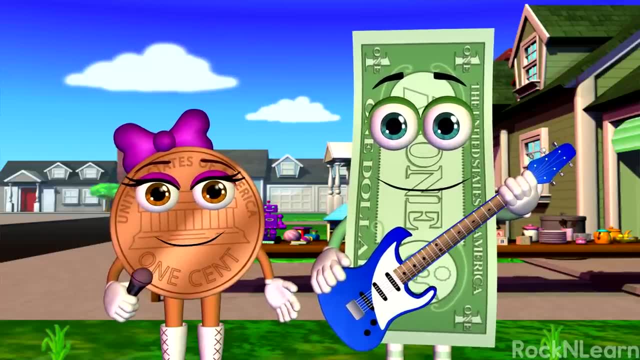 There are times when you need to be the person that makes correct change, Like at a lemonade stand or a bake sale, Or if you help out at a garage sale, Yeah, so it's a good idea to know how to make change. 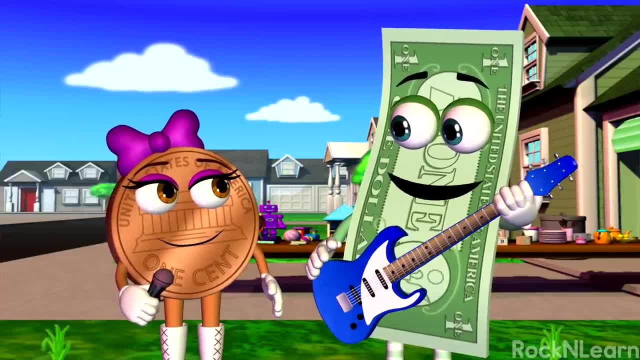 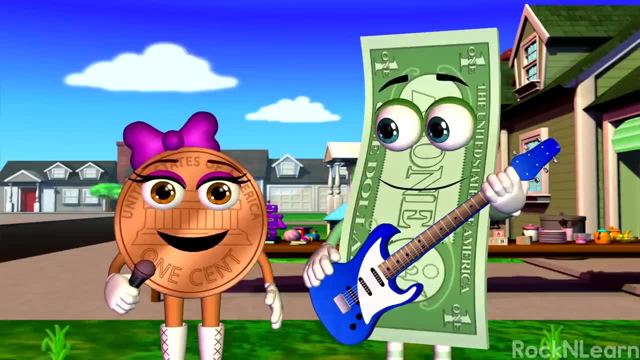 I like to make change by starting with the price of the item sold and counting up to the amount of money the customer gave me. Another tip is to start using pennies and smaller coins to get to a point where you can skip count using larger coins. 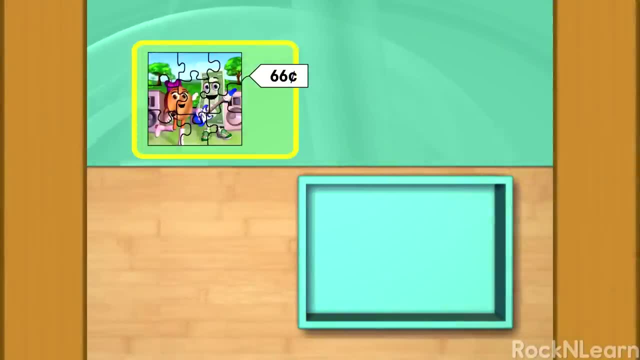 Let's do some examples. On the left side of the screen you will see an item from our garage sale with the price tag. The amount of money the customer is giving us will be below the item. On the bottom right side of the screen you'll see the amount of change. 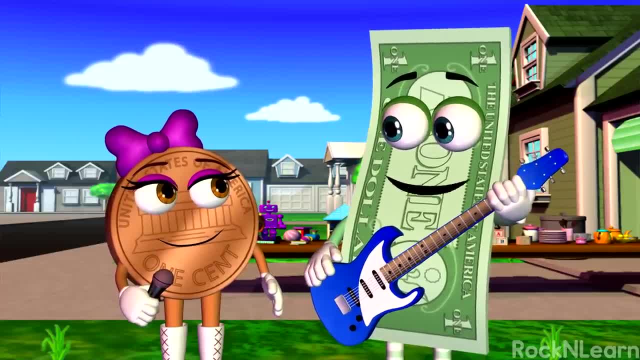 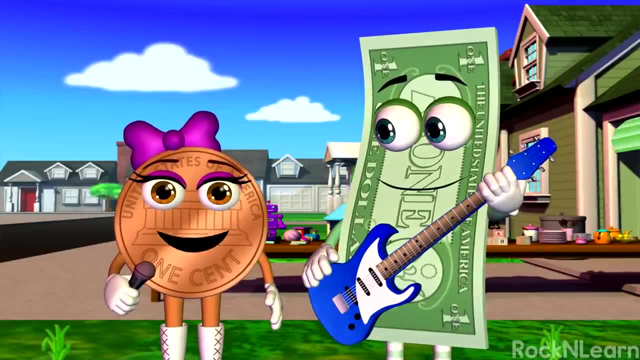 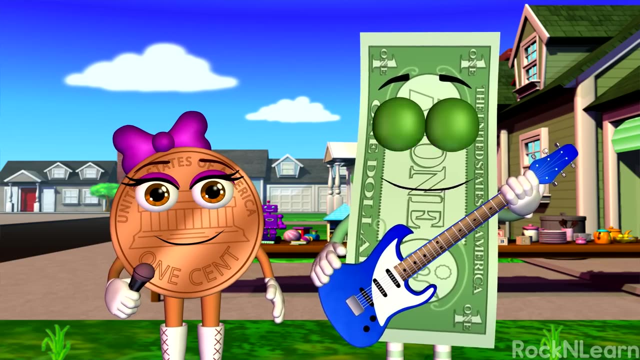 I like to make change by starting with the price of the item sold and counting up to the amount of money the customer gave me. Another tip is to start using pennies and smaller coins to get to a point where you can skip count using larger coins. Let's do some examples. On the left side of the screen you will. 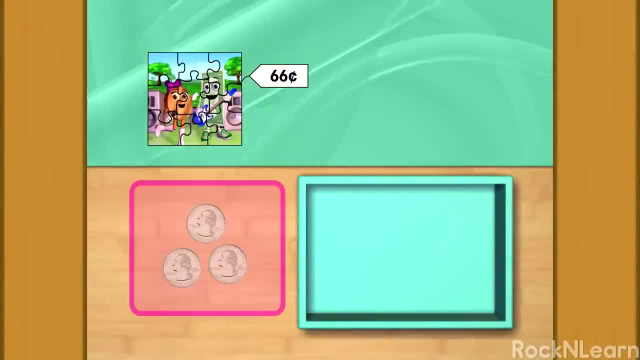 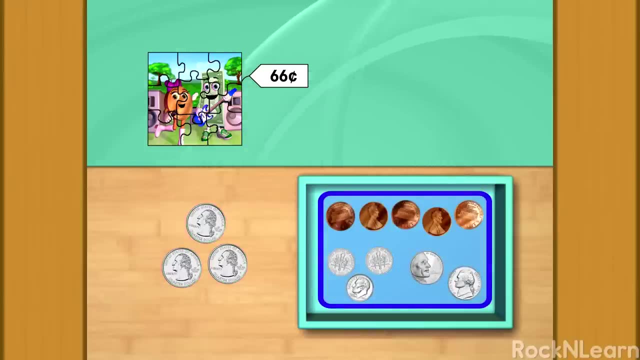 see an item from our garage sale with the price tag. The amount of money the customer is giving us will be below the item. On the bottom right side of the screen you'll see the amount of change we have available to give back. As we count out the change, we'll move it to the top of the screen. 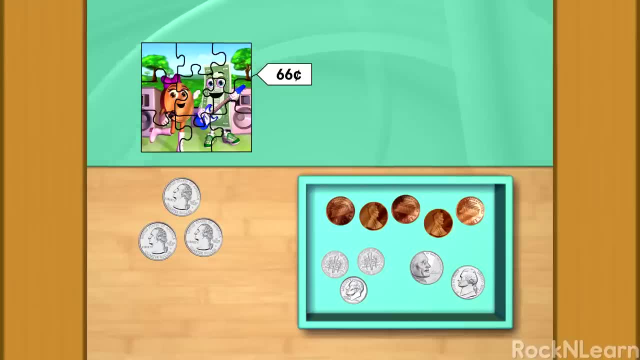 We need to know how much money they're paying first, then we can count the change. Let's see this puzzle is 66 cents and the money given is three quarters or twenty-five fifty cents. Let's see how much money they're paying. Let's see how much money they're paying. Let's. 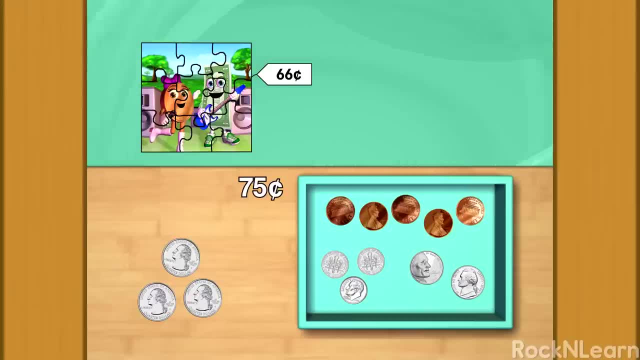 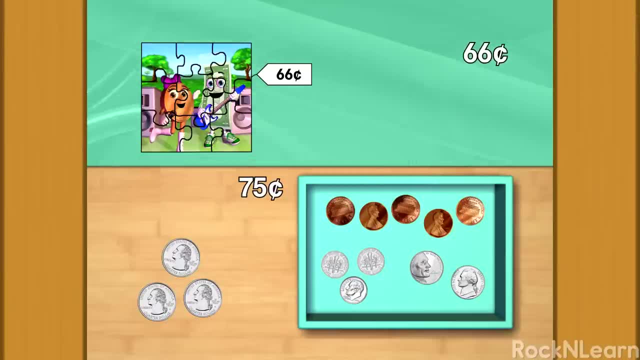 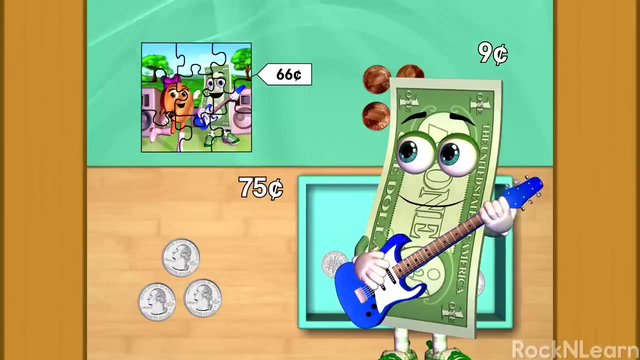 Starting at 66 cents, four pennies would make 68,, 70, and one nickel would bring us to 75 cents. So they get back four pennies and one nickel: Nine cents. Hey, that's us on that puzzle. How puzzling. Let's try another one. 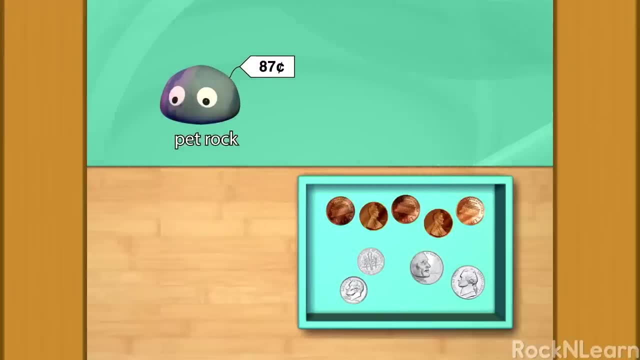 Hey look, This thing really rocks. It's easy to see that they're paying with one dollar, So all we really have to count is the change Starting at the price: 87, 88,, 89,, 90. And one of the dimes makes a dollar. 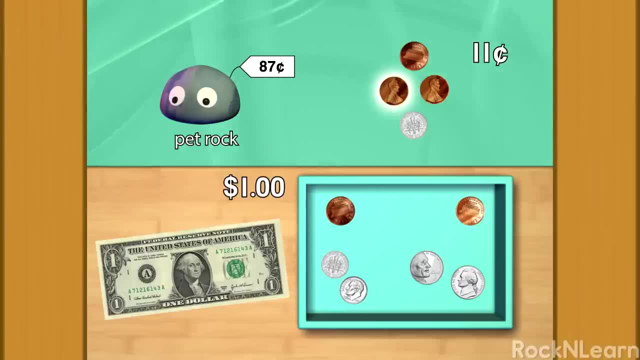 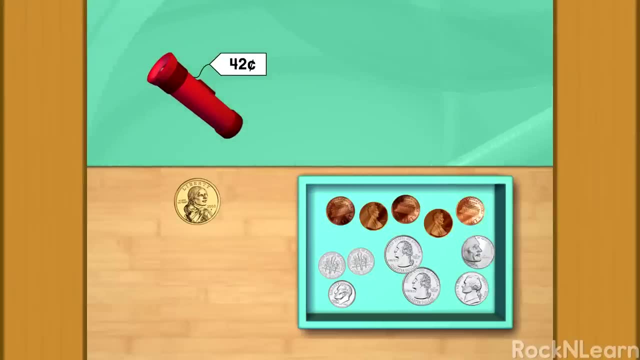 So the change they get is 10,, 11,, 12, 13 cents. Let's count the change for this dollar Starting at 42,. we count pennies 43,, 44,, 45.. Now we can use a nickel: 50. 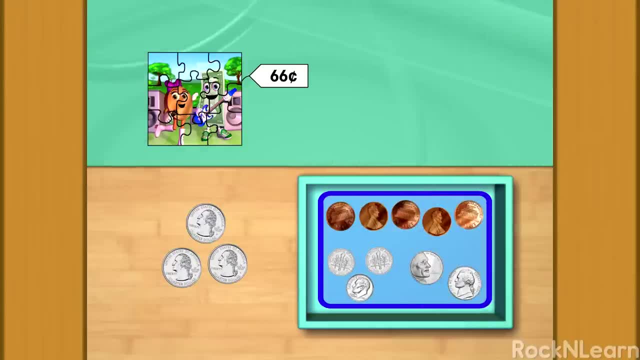 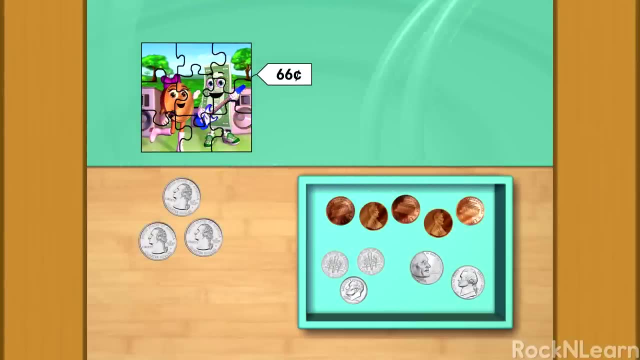 that we have available to give back. As we count out the change, we'll move it to the top of the screen. We need to know how much money they're paying first, Then we can count the change. Let's see, this puzzle is 66 cents. 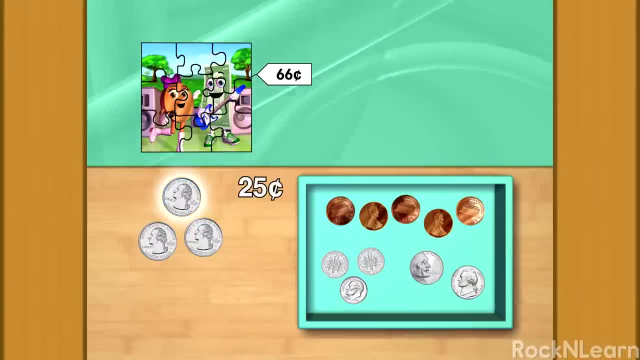 And the money given is three quarters, or 25,, 50,, 75 cents. Now we'll count up from the price of the puzzle until we reach the amount of change. This is the amount the customer paid, Starting at 66 cents. four pennies would make 68, 70. 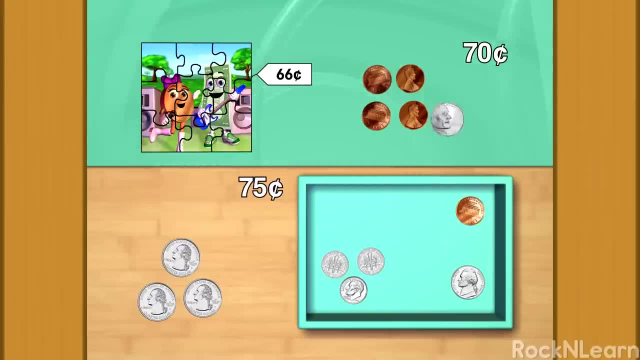 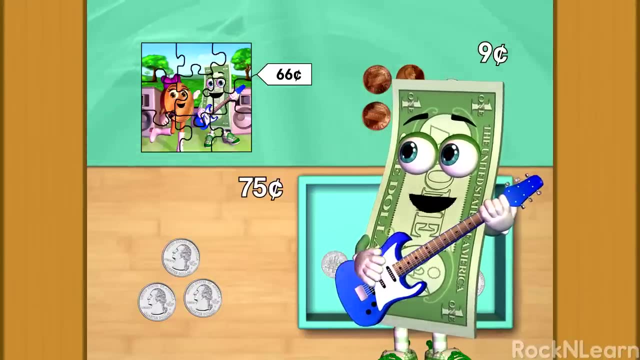 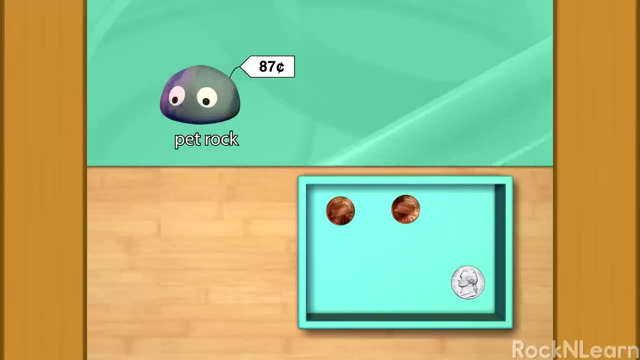 and one nickel would bring us to 75 cents. So they get back four pennies and one nickel- Nine cents. Hey, that's us on that puzzle. How puzzling. Let's try another one. Hey look, This thing really rocks. 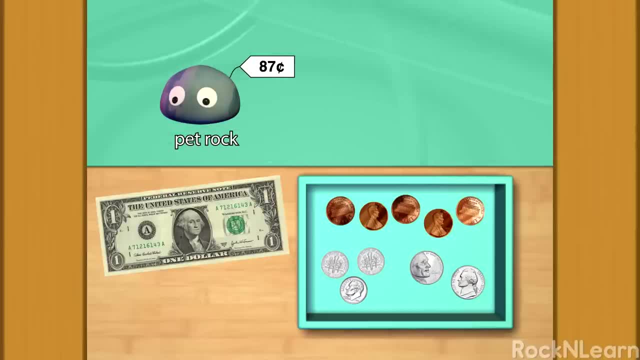 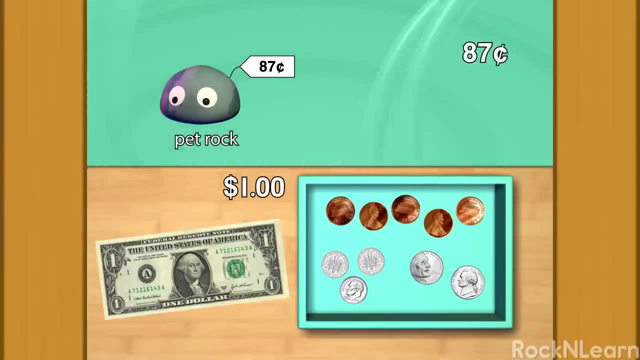 It's easy to see that they're paying with one dollar, So all we really have to count is the change Starting at the price 87,, 88,, 89,, 90. And one of the dimes makes a dollar. 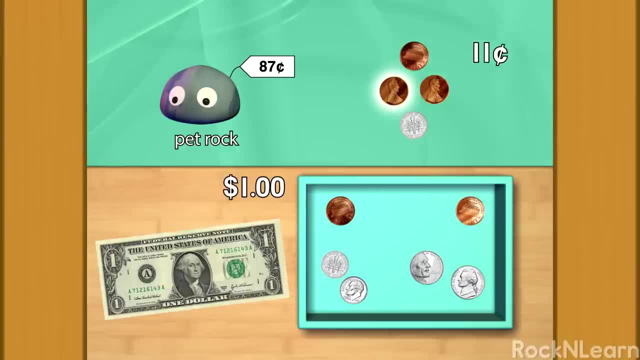 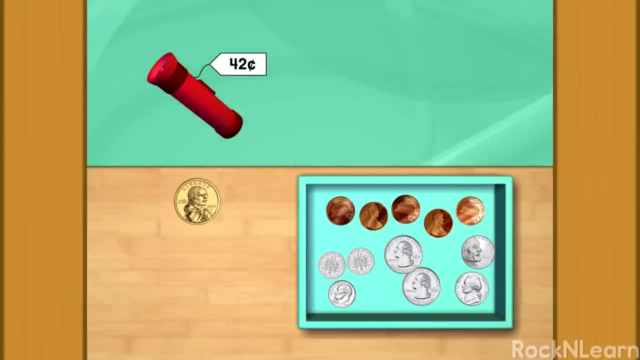 So the change they get is 10,, 11,, 12,, 13 cents. Let's count the change for this dollar, Starting at 42, we count pennies 43,, 44,, 45. Now we can use a nickel. 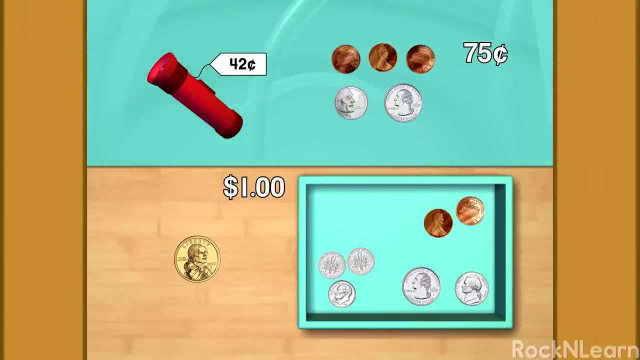 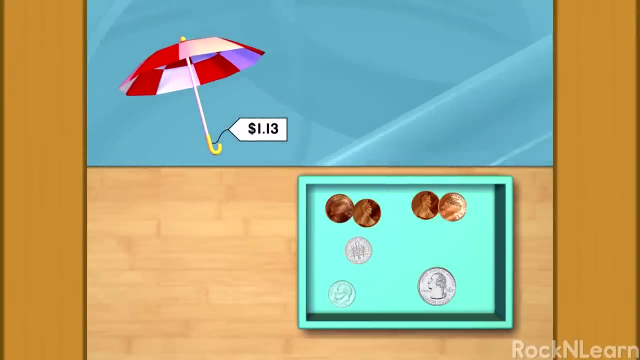 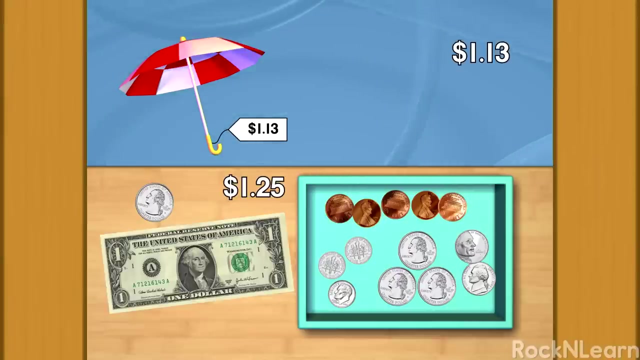 50. And then quarters to finish 75, a dollar. So they ended up getting 25,, 50,, 55,, 56,, 57,, 58 cents. They're paying one dollar and 25 cents. The price is a dollar 13.. 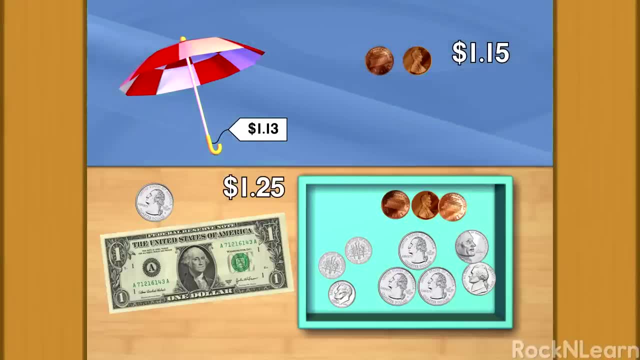 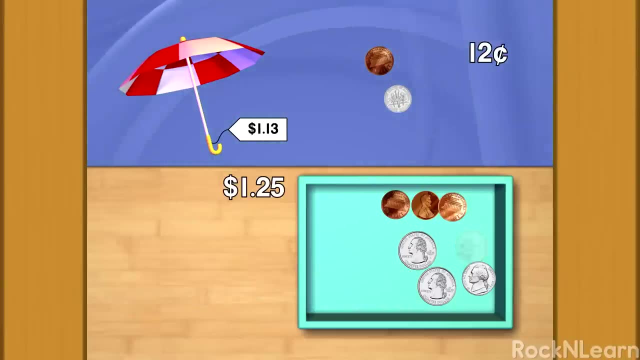 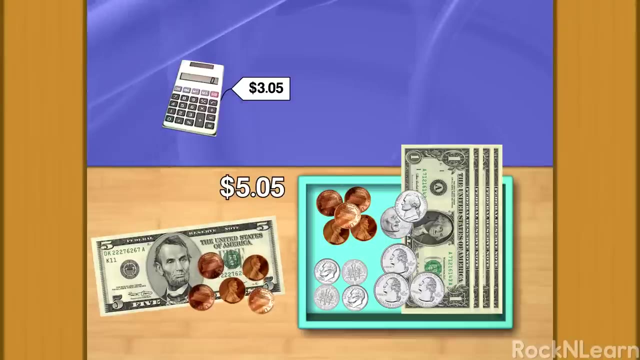 So 14,, 15, and a dime makes a dollar 25.. For a total of 12 cents change. Okay, the amount they gave us is five dollars and five cents, Or 505.. Here is another tip for making change. 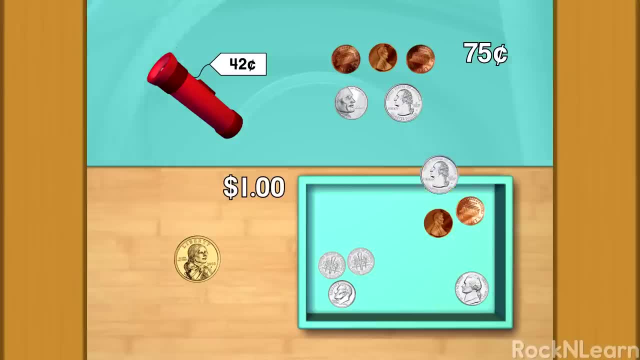 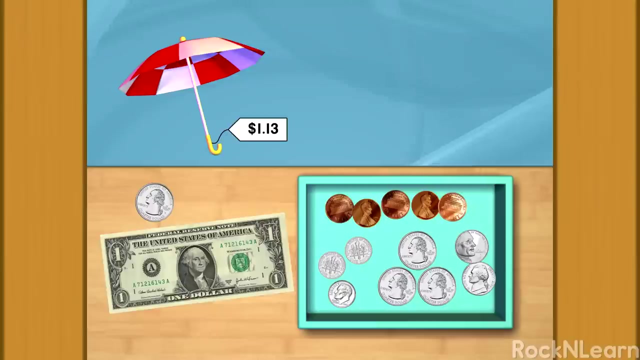 And then quarters to finish 75, a dollar. So they ended up getting 25,, 50,, 55,, 56,, 57,, 58 cents. They're paying one dollar and 25 cents. The price is a dollar 13.. 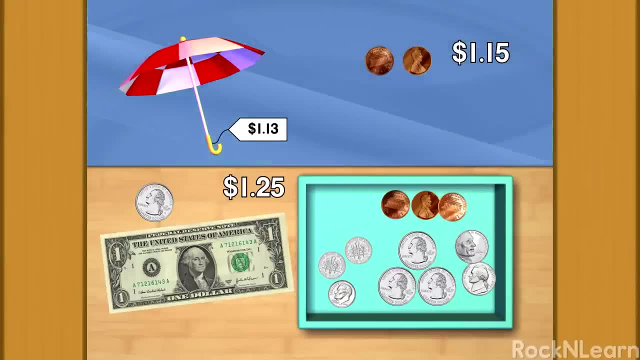 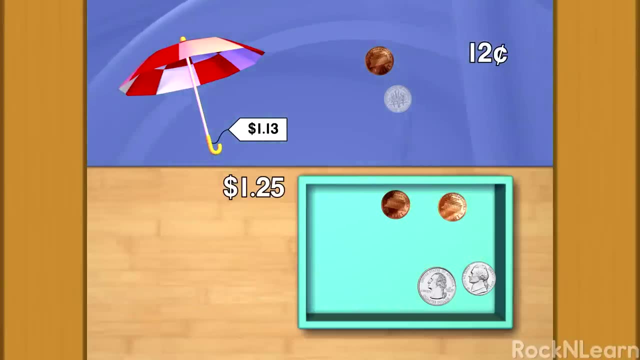 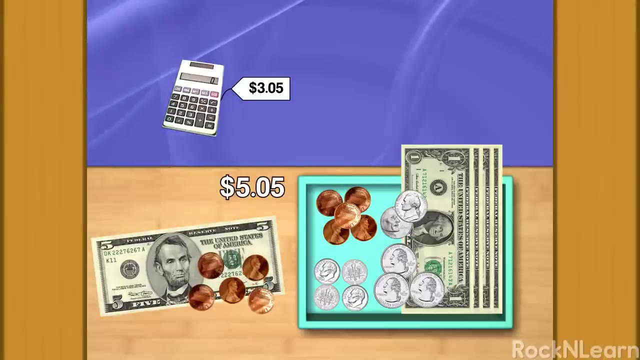 So 14,, 15, and a dime makes a dollar 25.. For a total of 12 cents change. Okay, the amount they gave us is five dollars and five cents, Or five and a half, Five and a half, Five and a half. 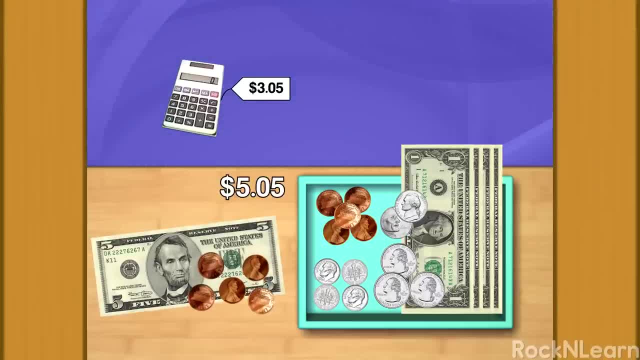 Here is another tip for making change: Look at the amount of money the customer gives you. If the coin part of what they give you is greater than or equal to the coin part of the price, make change for the coin part first. Then make change for the dollar part. 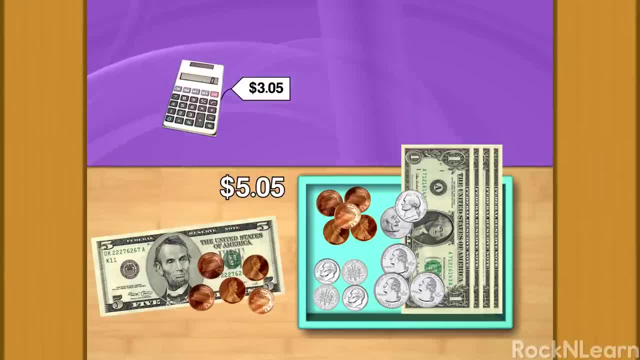 Let me see. if I have this straight, The price is 305.. The customer gave me 505.. The coin part of the price is equal to 505.. The coin part of the price is equal to the coin part. the customer paid five cents. 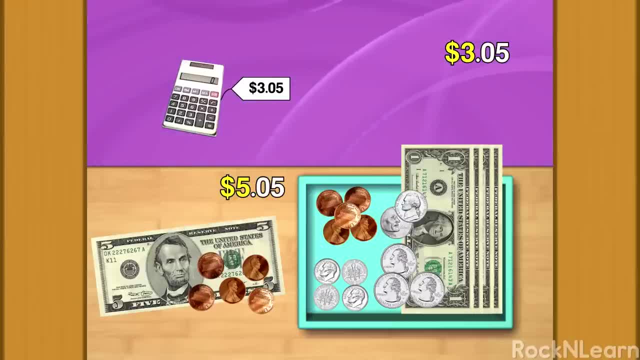 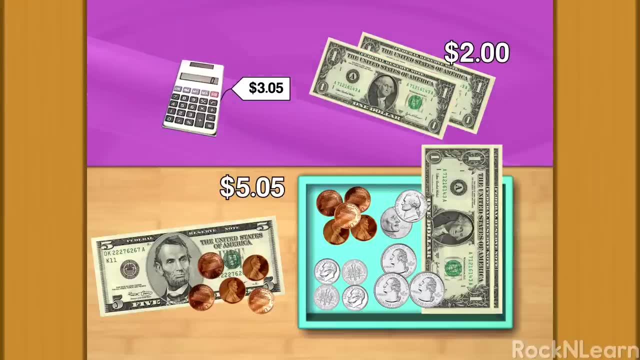 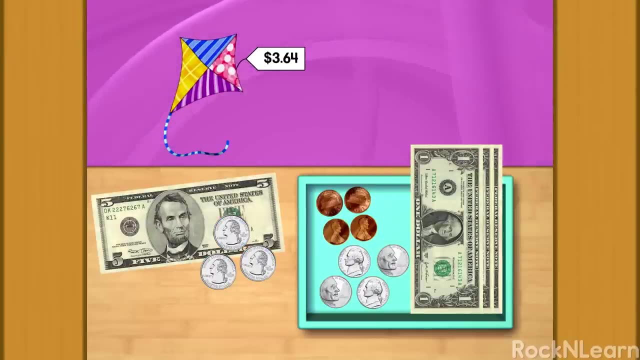 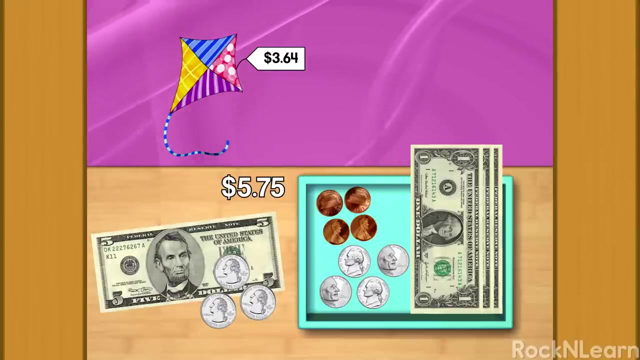 So I only have to make change for the dollars. That's right: 305,, 405, 505.. The customer gets two dollars change. This customer is paying with five dollars and 25,, 50, 75 cents. Sometimes people will give you change close to what they owe. 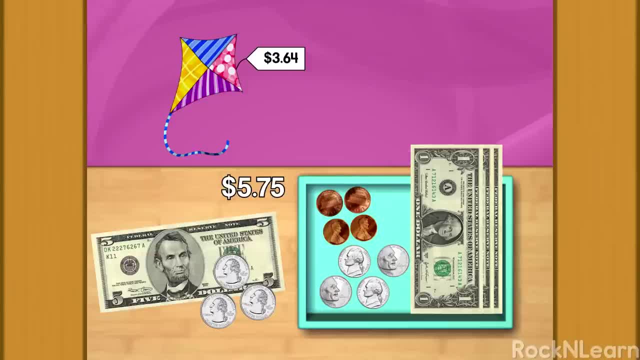 So that they don't have to carry around as many coins. Using the tip we just learned, let's look at the coin part. The 75 cents of the money given is greater than the 64 cents of the price. Let's make change for the coin part first. 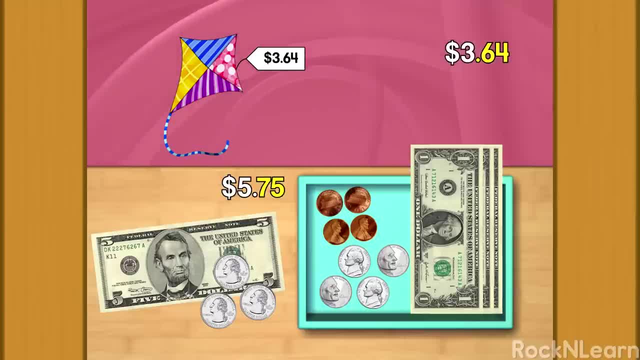 Since they owed 64 cents as the coin part of the price, we'll start counting up until we get to the 75 cents that they gave us. So 64 plus one penny goes to That gives us 65. And two of these nickels will bring us to 70, 75. 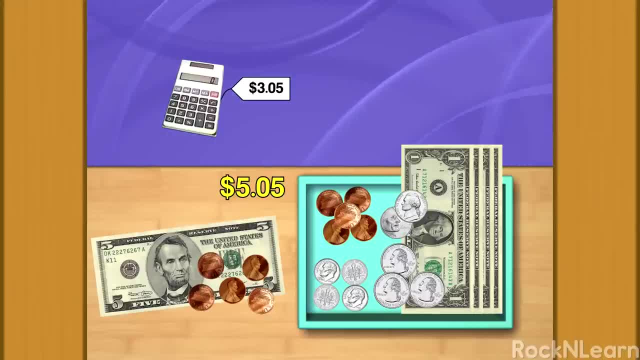 Look at the amount of money the customer gives you. If the coin part of what they give you is greater than or equal to the coin part of the price, make change for the coin part first, Then make change for the dollar part. Let me see if I have this straight. 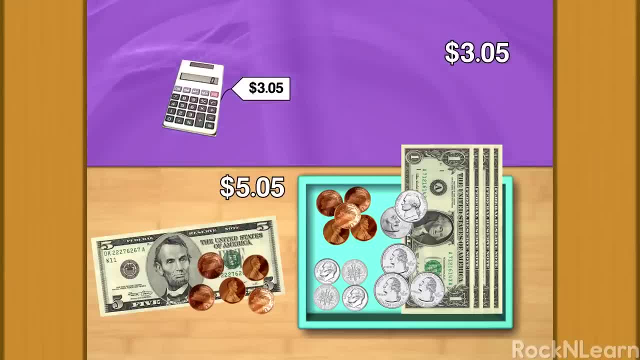 The price is 305.. The customer gave me 505.. The coin part of the price is equal to the coin part. the customer paid five cents, So I only have to make change for the dollars. That's right: 305,, 405,, 505. 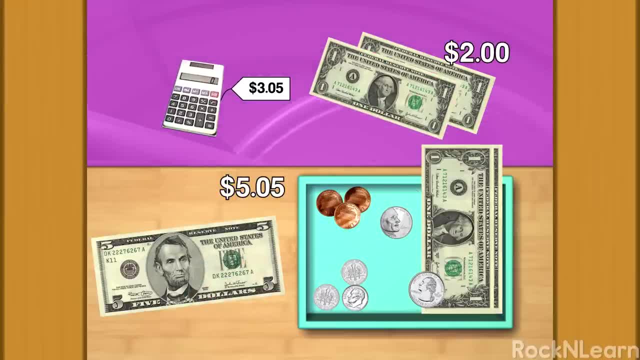 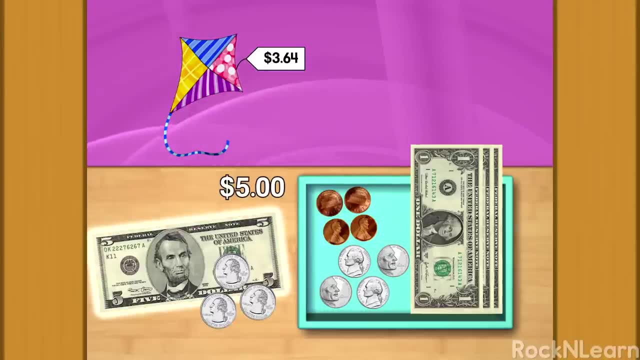 The customer gets two dollars change. This customer is paying with five dollars and 25,, 50, and 75 cents. Sometimes people will give you change close to what they owe so that they don't have to carry around as many coins. 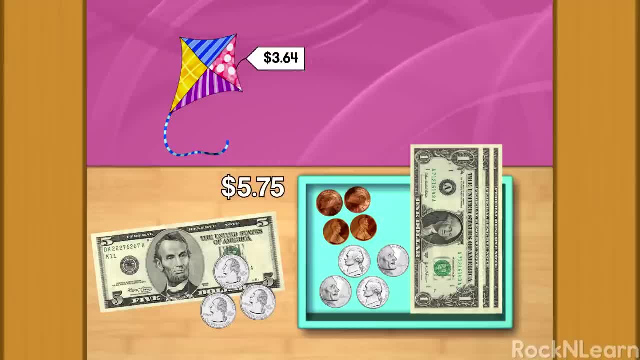 Using the tip we just learned, let's look at the coin part. The 75 cents of the money given is greater than the 64 cents of the price. Let's make change for the coin part first, Since they owed 64 cents as the coin part of the price. 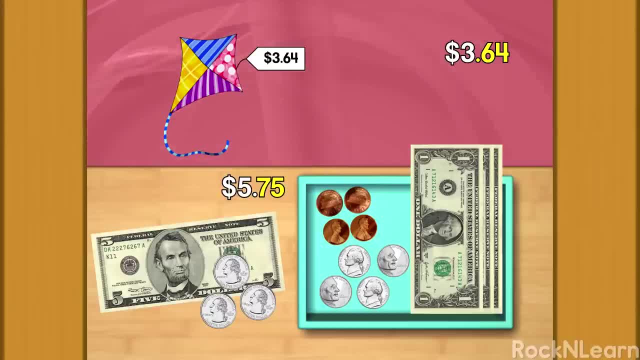 we'll start counting up until we get to the 75 cents. So 64 plus one penny gives us 65, and two of these nickels will bring us to 70, 75. If we had any dimes, we could have given them one dime instead of the two nickels. 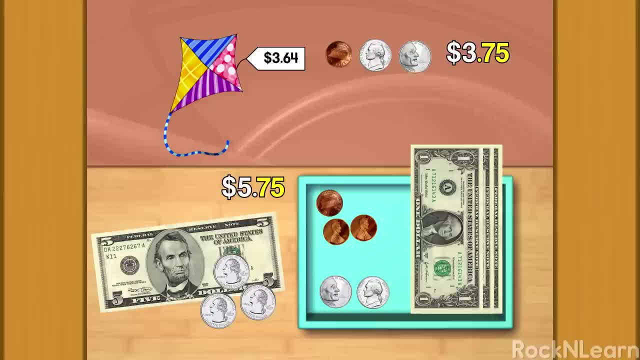 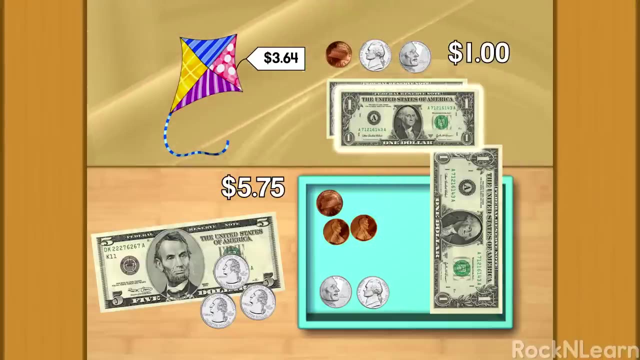 But unfortunately we can't give the smallest number of coins. if we don't have them Now, we'll make change for the dollar part. They owed three dollars. We need two more to make the four, five that they paid. They get one. 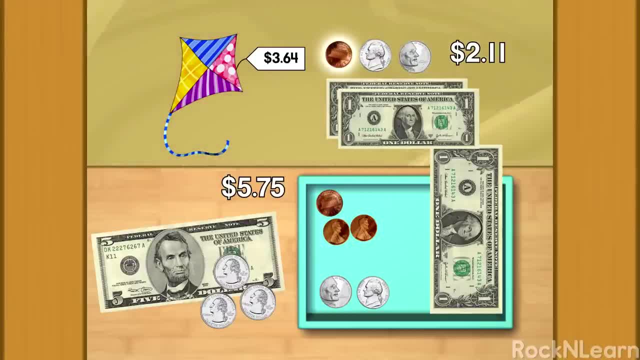 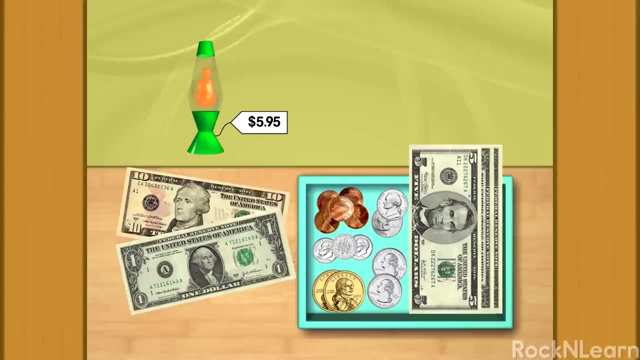 two dollars and five ten eleven cents change- Whoa cool. I love watching these things, Me too. I just don't have room for it. The lava lamp only costs 5.95,, so this person could pay with just the ten dollar bill. 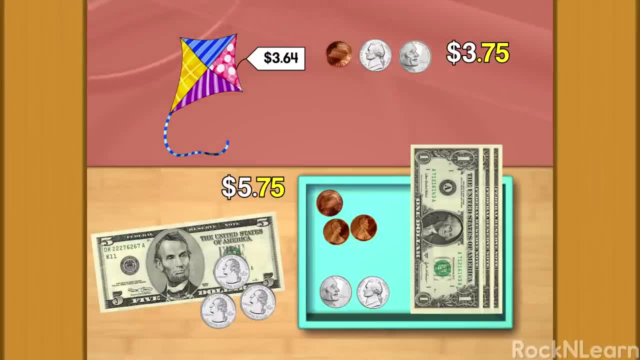 If we had any dimes we could have given them one dime instead of the two nickels, But unfortunately we can't give the smallest number of coins. if we don't have them Now, we'll make change for the dollar part. They owed three dollars. 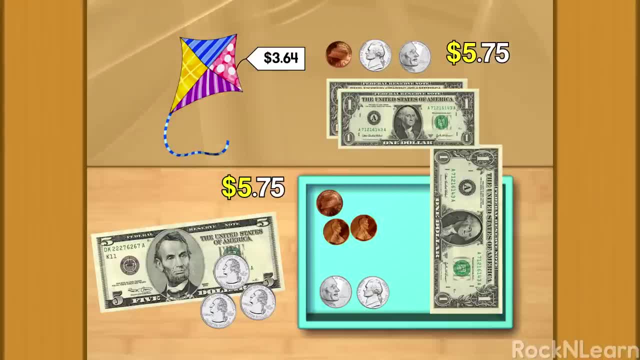 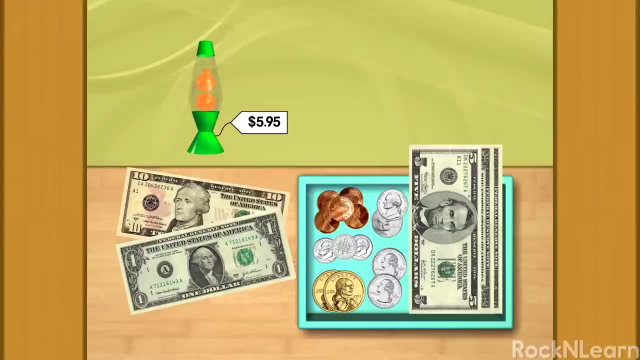 We need two more to make the four, five that they paid. They get one, two dollars And five, ten eleven cents change. Whoa cool. I love watching these things, Me too. I just don't have room for it. 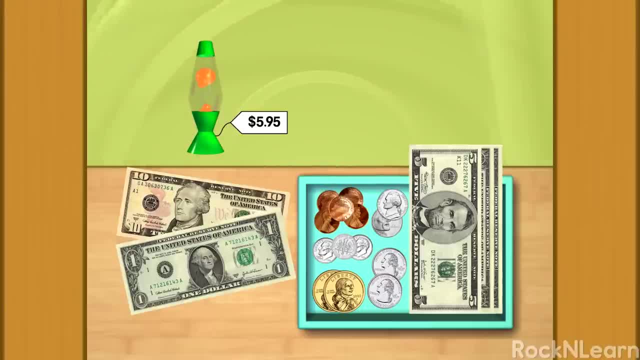 The lava lamp only costs 5.95. So this person could pay with just the ten dollar bill. But sometimes customers want to carry as few bills and coins as possible. We'll use the dollar bill to make change for the coin, part of the price. 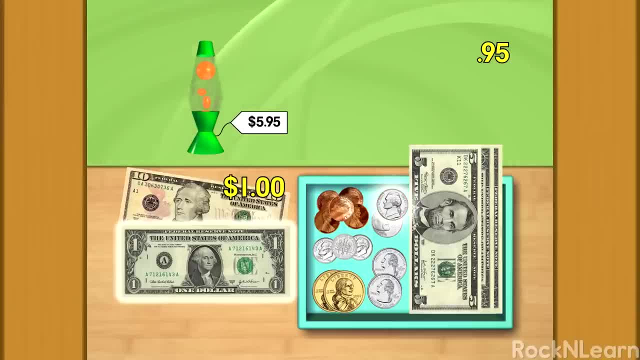 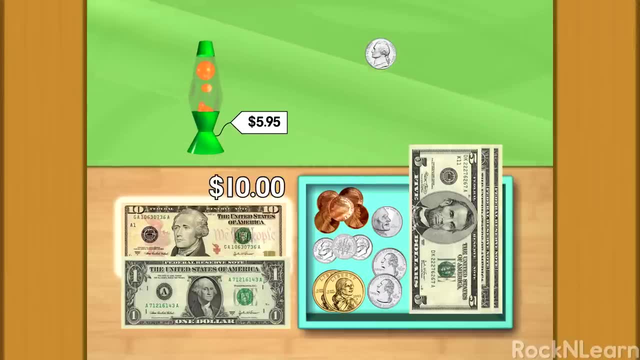 That'll be easy. We only need one nickel to bring the 95 cents to a dollar Now to make change for the ten dollar bill. The dollar part of the price is five dollars, So this five dollar bill will make it add up to the ten that they gave us. 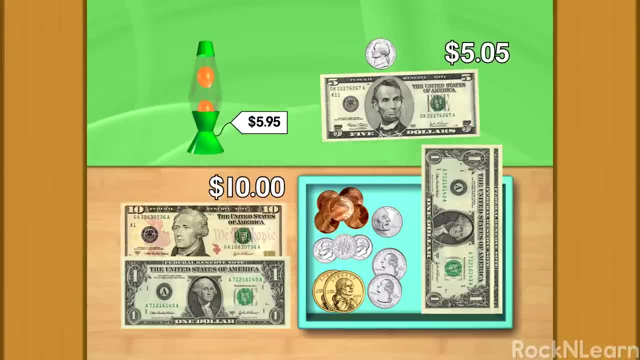 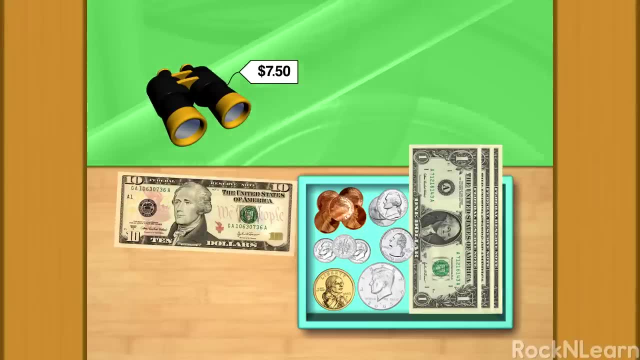 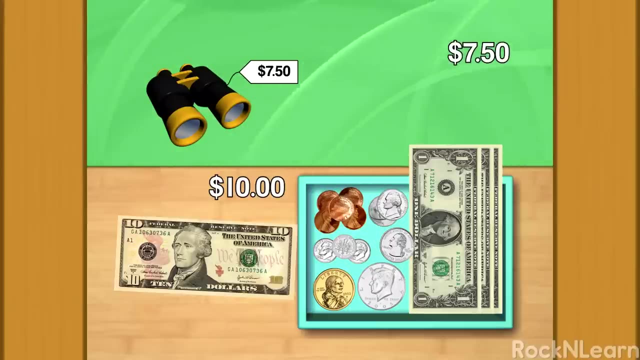 They ended up with five dollars and five cents in change. It's easy to see that they are paying with ten dollars. Let's start with the price. seven, fifty, And if we add this half dollar that brings us to eight dollars. Then we can give them either this dollar coin or a dollar bill to make nine. 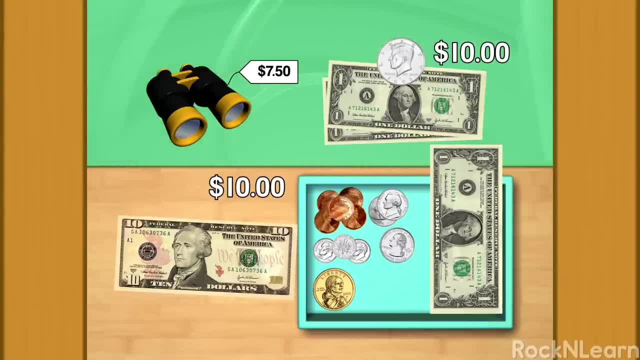 And another dollar bill brings us to ten. That's one, two dollars and fifty cents they get in change. Looks like we could have made change several different ways with the change we have available. That's right. Instead of using the half dollar, we could have used one quarter. 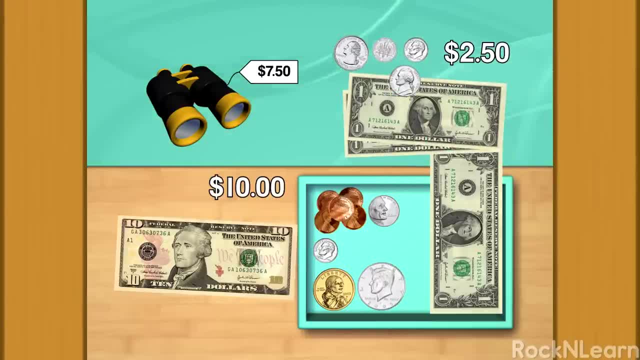 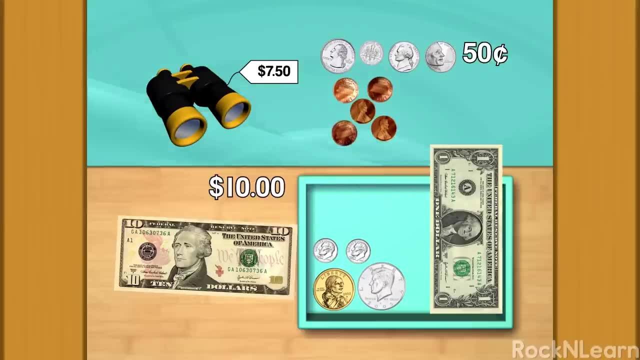 two dimes and a nickel to go with the two dollar bills. Or we could have used a quarter, one dime, two nickels and five pennies instead of the half dollar. But most of the time people don't want to carry around all of those extra coins. 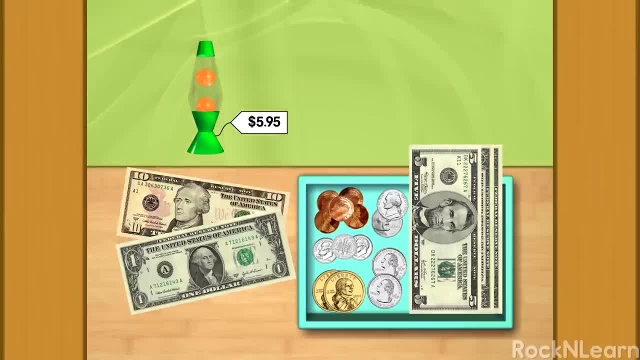 But sometimes customers want to carry as few bills and coins as possible. We'll use the dollar bill to make change for the coin part of the price. That'll be easy. We only need one nickel to bring the 95 cents to a dollar. 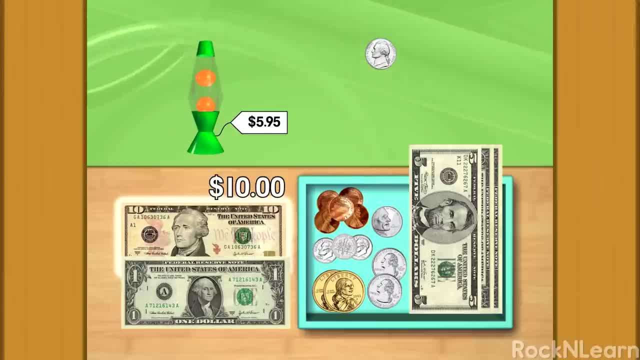 Now to make change for the ten dollar bill. The dollar part of the price is five dollars, so this five dollar bill will make it add up to the ten that they gave us. They ended up with five dollars and five cents And five cents in change. 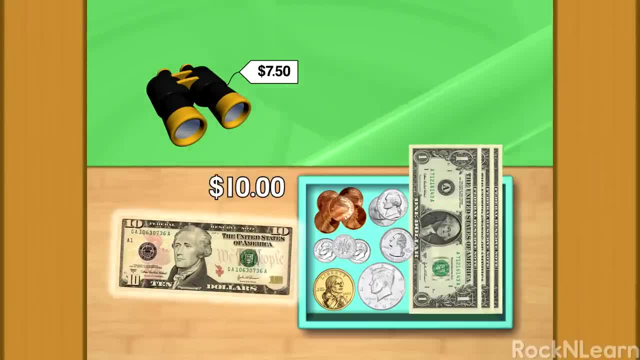 It's easy to see that they are paying with ten dollars. Let's start with the price seven, fifty, And if we add this half dollar that brings us to eight dollars. Then we can give them either this dollar coin or a dollar bill to make nine. 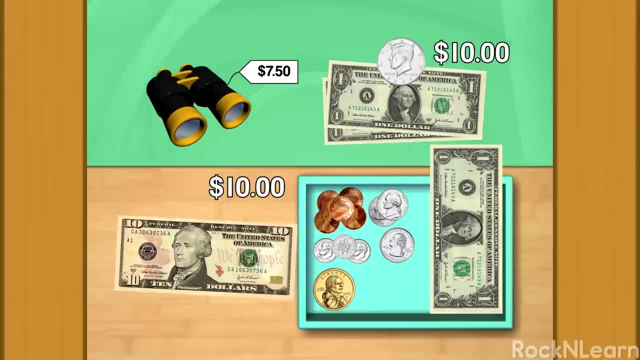 And another dollar bill brings us to ten. That's one, two dollars and fifty cents. they get in change. Looks like we could have made change several different ways with the change we have available. That's right, Instead of using the half dollar. 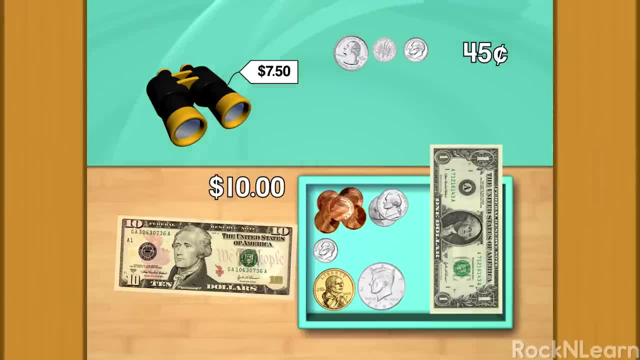 we could have used one quarter, two dimes and a nickel to go with the two dollar bills. Or we could have used a quarter one dime, two nickels and five pennies instead of the half dollar. But most of the time people don't want to carry around all of those extra coins. 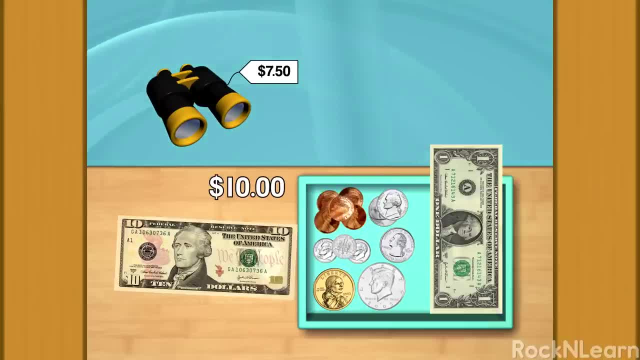 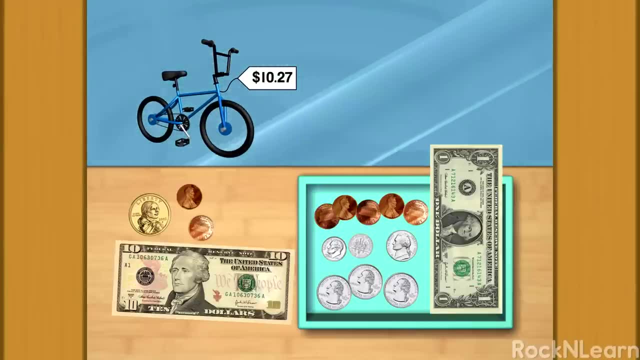 We should try to make change using the least amount of coins possible. I hope they enjoy this bike as much as I have. Let's count the amount they gave us: Ten eleven dollars and two cents. Wait a minute. They really only needed the ten dollar bill and the dollar coin. 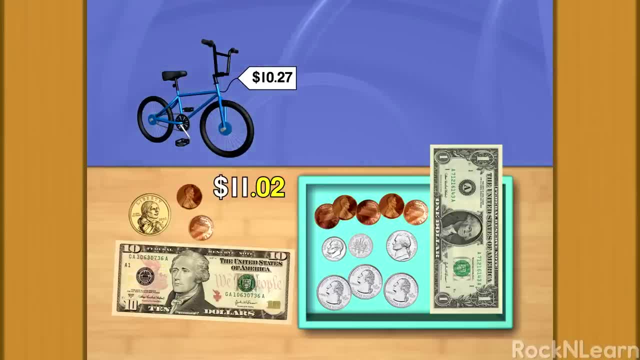 The two cents is not greater than or equal to the twenty-seven cents in the price. But sometimes people want a particular kind of change, like if they want to get back quarters for a vending machine. We'll count change like normal then see if the two pennies help us out. 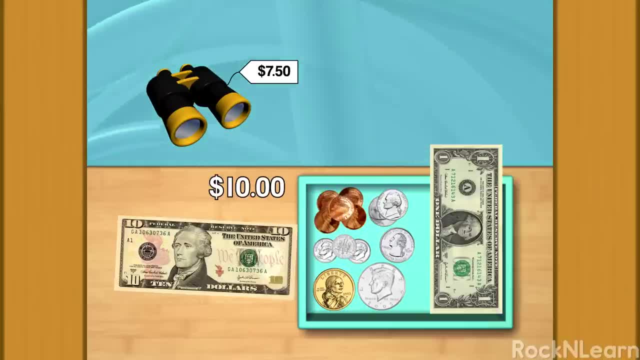 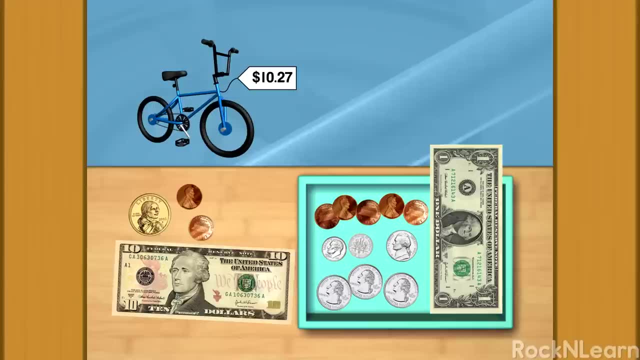 We should try to make change using the least amount of coins possible. I hope they enjoy this bike as much as I have. Let's count the amount they gave us: Ten eleven dollars and two cents. Wait a minute. They really only needed the ten dollar bill and the dollar coin. 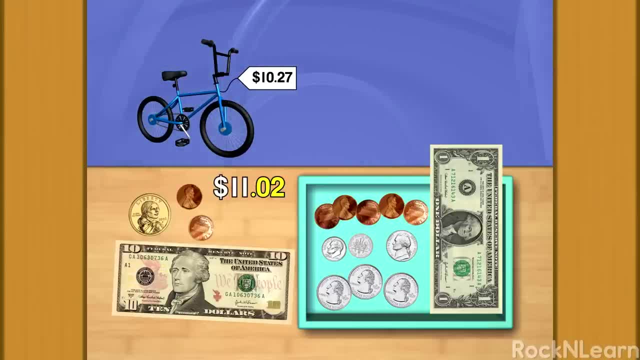 The two cents is not greater than or equal to the twenty-seven cents in the price. But sometimes people want a particular kind of change, Like if they want to get back quarters for a vending machine. We'll count change like normal, then see if the two pennies help us out. 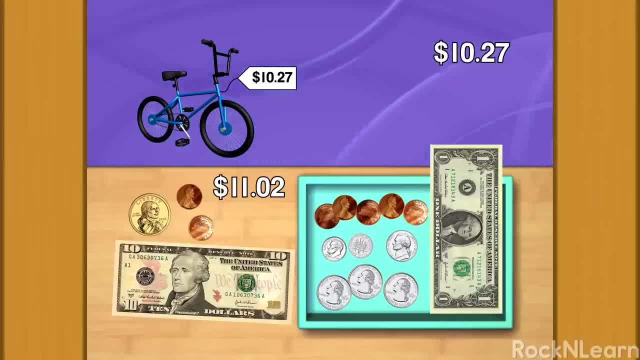 So counting from the price of ten dollars and twenty-seven cents, three pennies makes twenty-eight, twenty-nine. thirty two dimes makes forty. fifty. two quarters makes seventy-five eleven dollars. But they gave us eleven dollars and two cents. 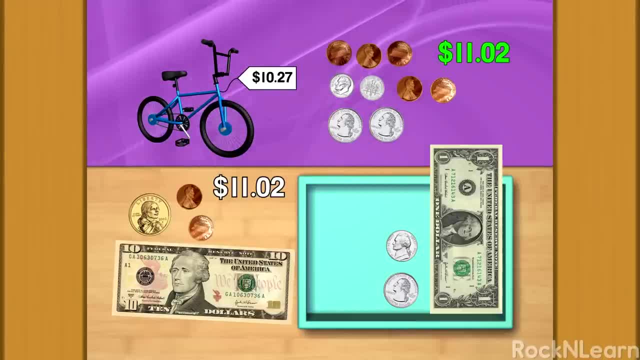 So we'll give them two more pennies. Now count the change we gave. Twenty-five, fifty, sixty, seventy, seventy-one, seventy-two, seventy-three, seventy-four, seventy-five, Seventy-five cents change. But we could give them that amount with fewer coins. 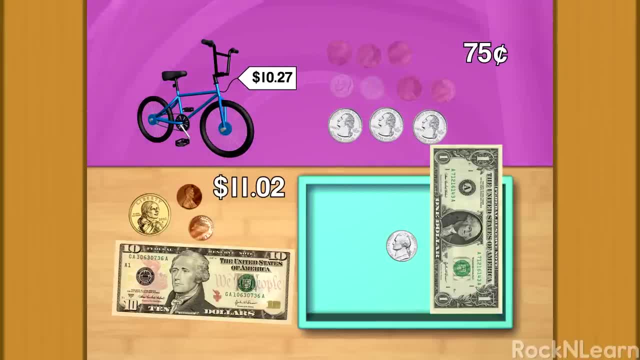 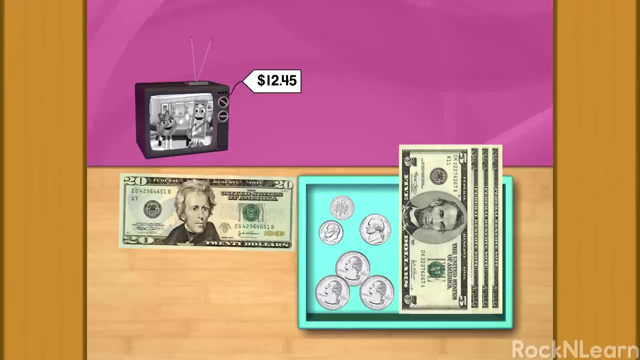 Hey, that's right. I guess they wanted three quarters instead of having to carry around two quarters, two dimes and five pennies. That's pretty cool. And now for our last garage sale item: an old TV. Wow, we get to make change for a twenty-dollar bill. 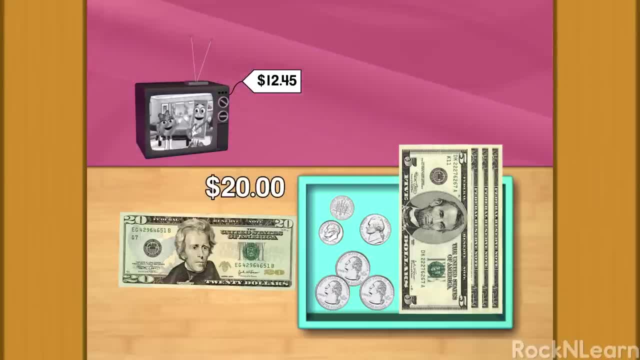 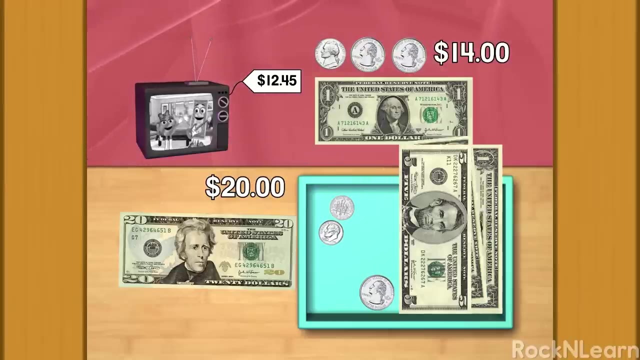 It's just as easy as all the rest. Start at the price. twelve dollars and forty-five cents A nickel brings us to twelve-fifty, Then the quarters, twelve-seventy-five, thirteen dollars, Then the dollars fourteen-fifteen. 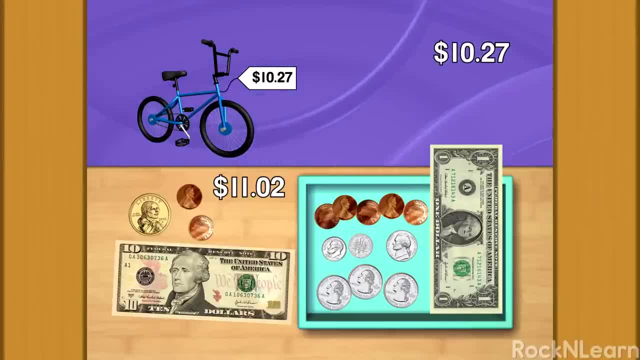 So counting from the price of ten dollars and twenty-seven cents, three pennies makes twenty-eight, twenty-nine. thirty two dimes makes forty. fifty. two quarters makes seventy-five eleven dollars. But they gave us eleven dollars and two cents. 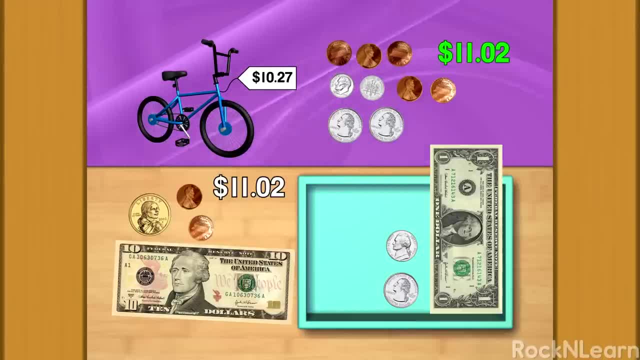 so we'll give them two more pennies. Now count the change we gave. Twenty-five, fifty, sixty, seventy, seventy-one, seventy-two, seventy-three, seventy-four, seventy-five, Seventy-five cents change, but we could give them that amount with fewer coins. 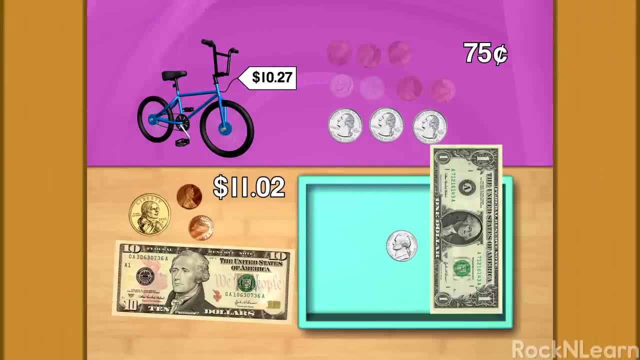 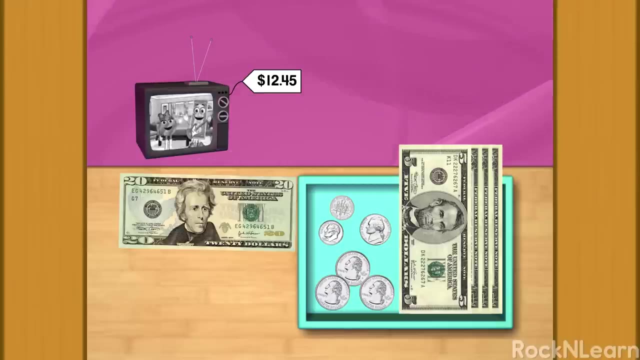 Hey, that's right. I guess they wanted three quarters instead of having to carry around two quarters. two dimes and five pennies. That's pretty cool. And now for our last garage sale item: an old TV. Wow, we get to make change for a twenty dollar bill. 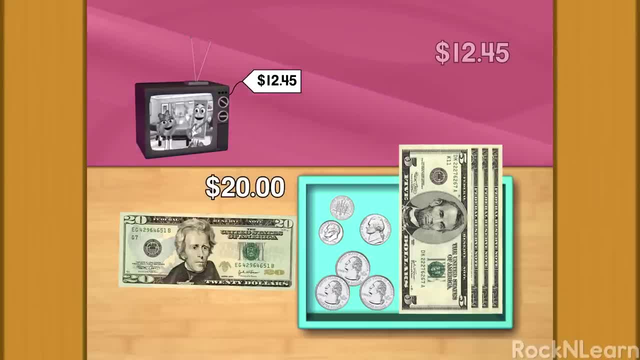 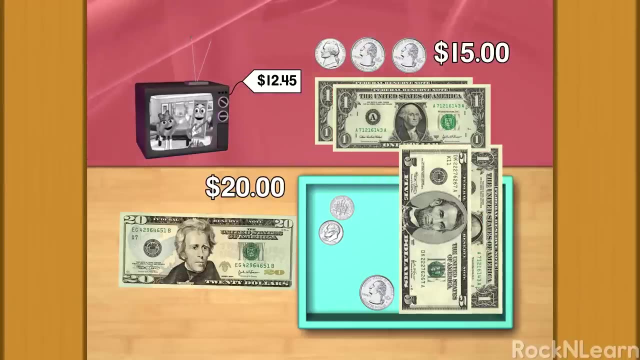 It's just as easy as all the rest. Start at the price. twelve dollars and forty-five cents A nickel brings us to twelve-fifty, then the quarters, twelve-seventy-five, thirteen dollars, Then the dollars. fourteen, fifteen. 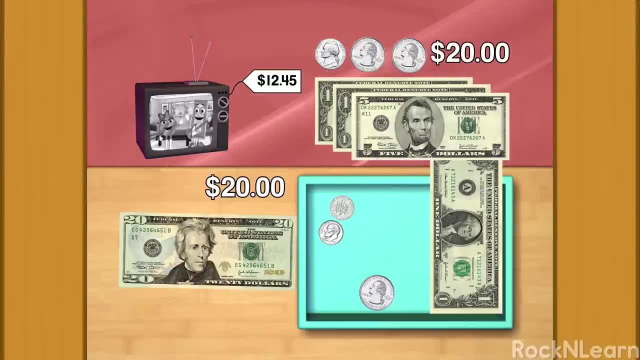 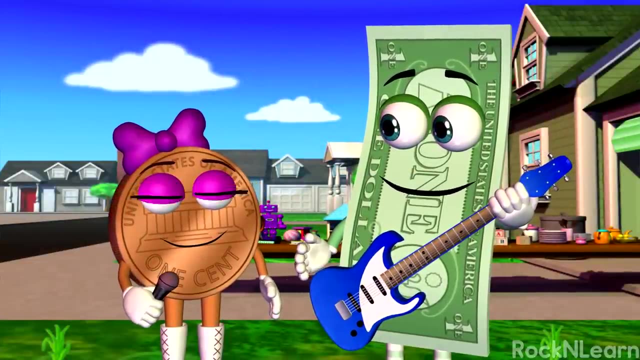 and one five dollar bill makes twenty dollars. That's five, six, seven dollars and twenty-five, fifty, fifty-five cents change. Whew, we did it. I hope they enjoy the TV. Having a garage sale is fun. We made some money. 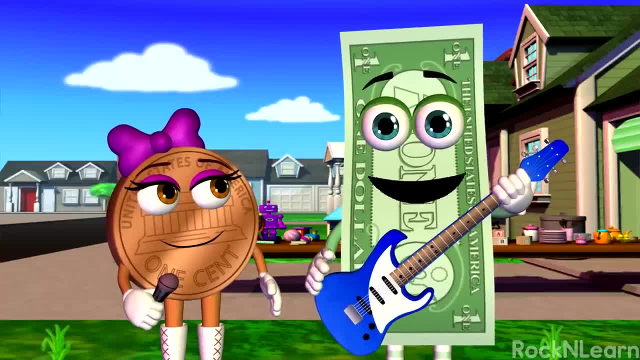 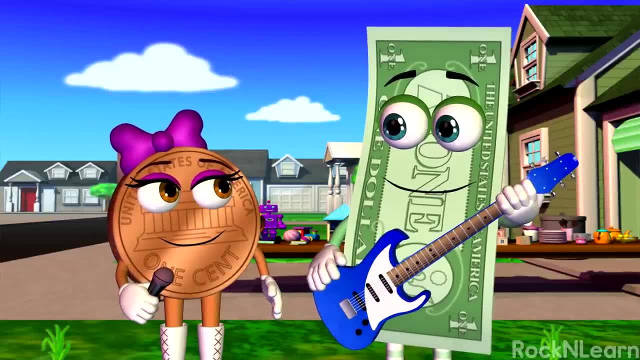 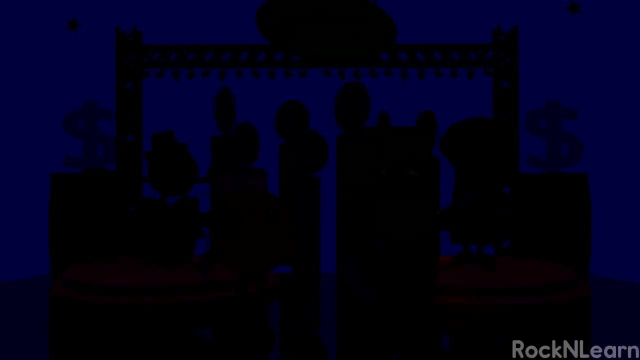 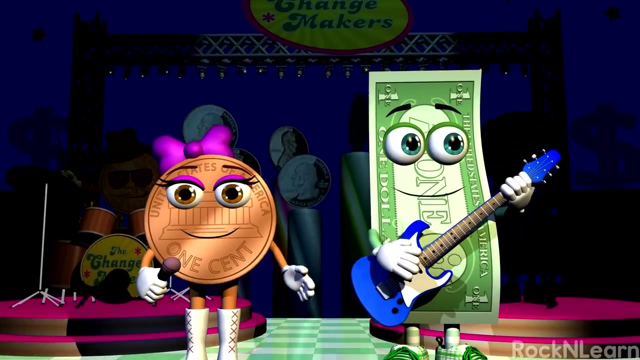 and got rid of some things we don't use or play with anymore, And we got lots of practice counting money and making change. Good evening everybody. I'm Penny Money and this is Bill Dollar. This is our band, The Change Makers. 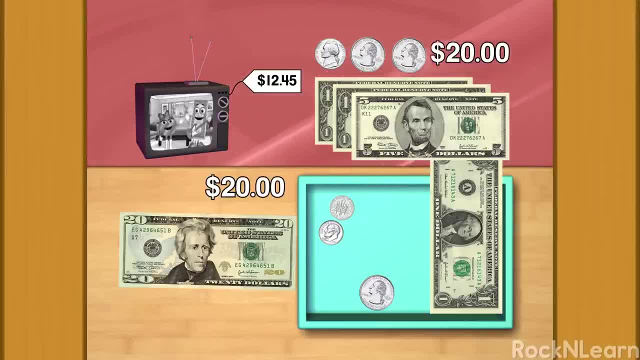 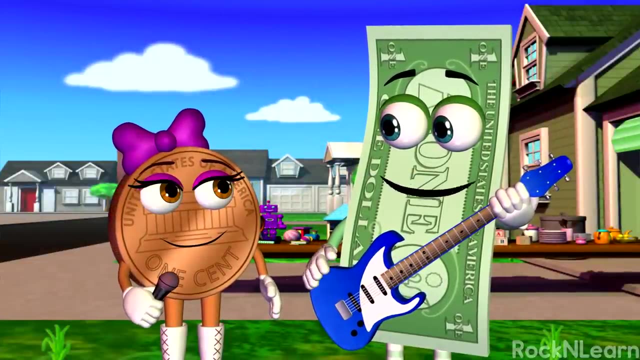 And one five-dollar bill makes twenty dollars. That's five, six, seven dollars and twenty-five, fifty, fifty-five cents change. Whew, we did it. I hope they enjoy the TV. Having a garage sale is fun. We made some money and got rid of some things we don't use or play with anymore. 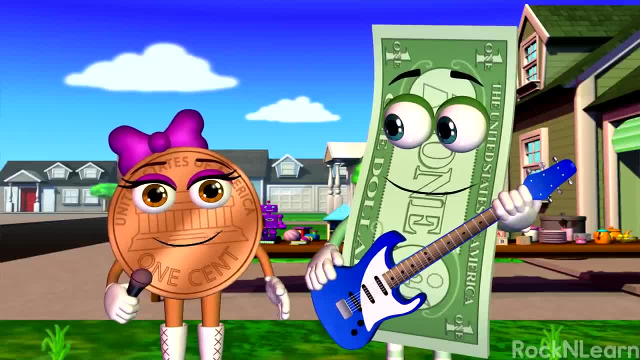 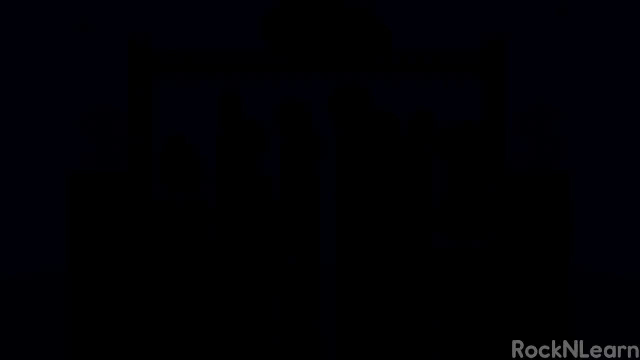 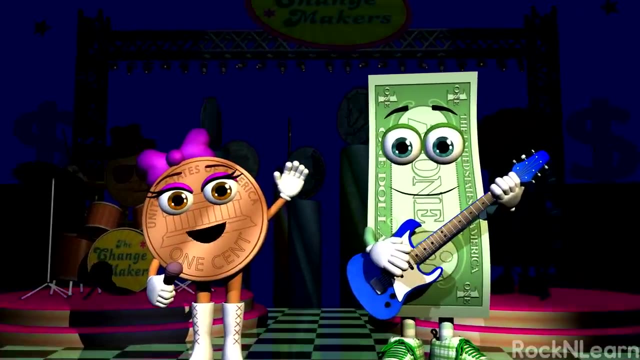 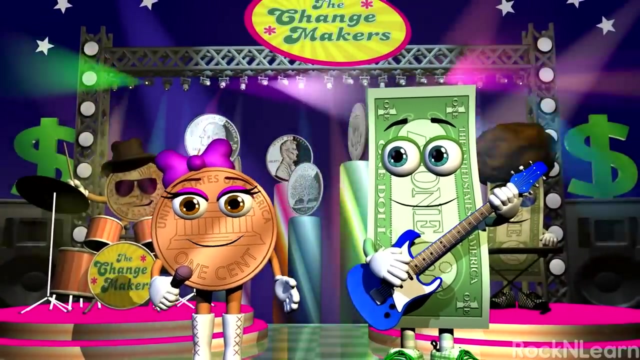 And we got lots of practice counting money and money, Practice counting money and making change. Good evening everybody. I'm Penny Money And this is Bill Dollar. This is our band, The Changemakers. We'd like to send this song out to our very special friends in the front row. 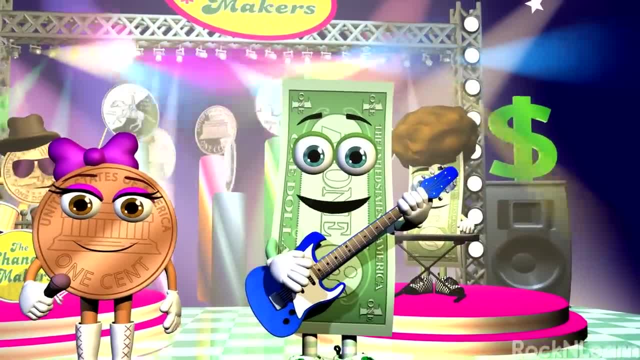 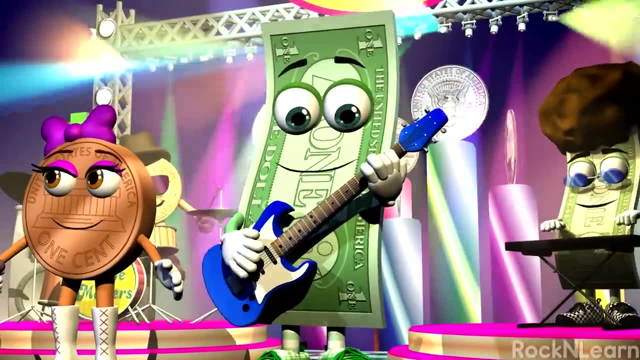 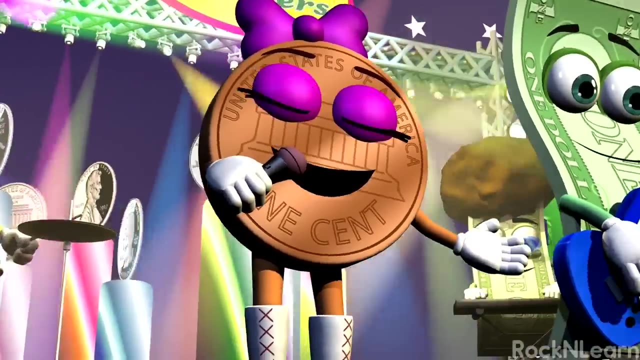 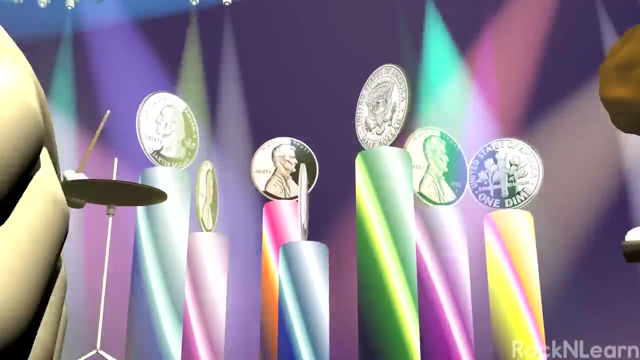 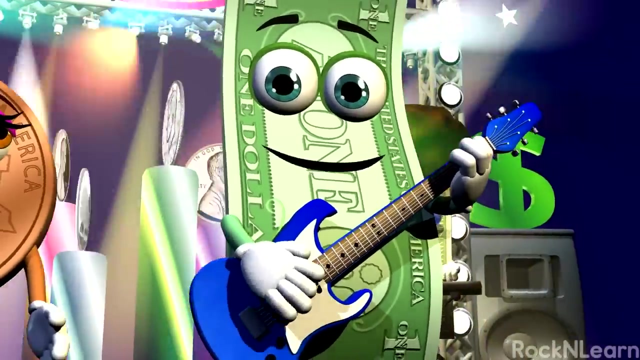 So, everybody, put your hands together and let's rock. When I need something new And I don't know what to do, I just shake, shake, shake, shake my piggy bank. I save my money when I can, So I'll have a backup plan. 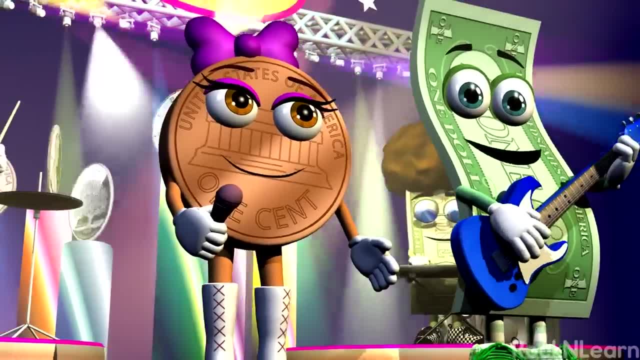 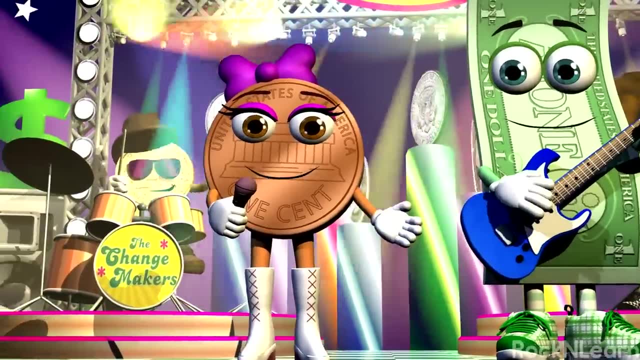 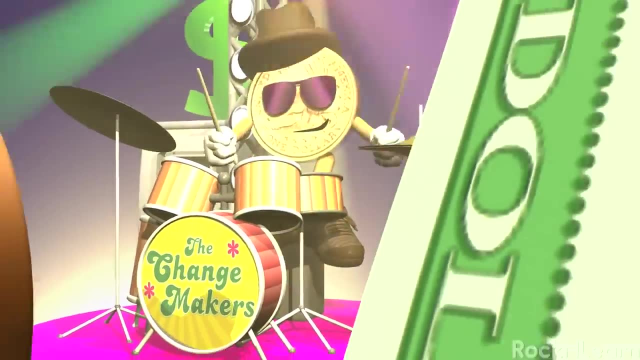 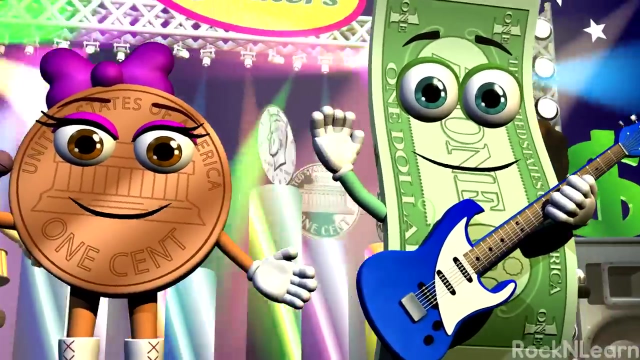 I just shake, shake, shake, shake my piggy bank. There's lots of fun to be had. No reason to be sad When you shake, shake, shake, shake your piggy bank. Quarters, dimes, nickels and pennies, Dollar coins and bills- there are so many. 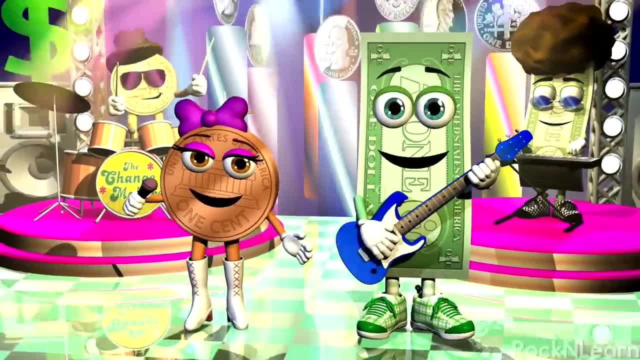 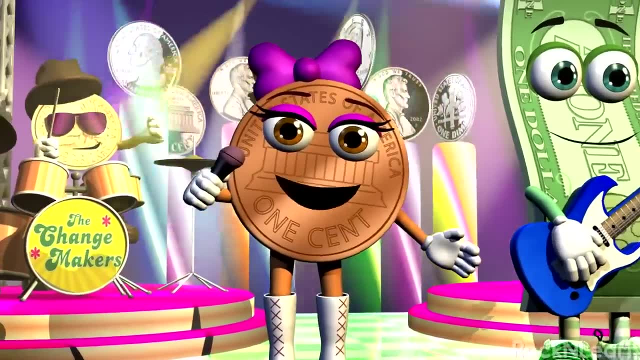 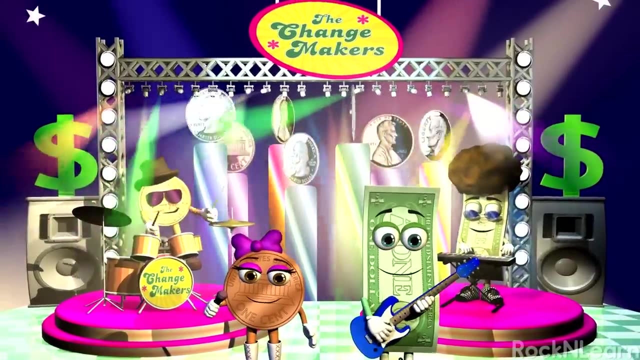 Shake, shake, shake, shake your piggy bank. Shake them all out and you can start to count All the coins in your piggy bank. Shake, shake, shake, shake your piggy bank. Shake, shake, shake, shake your piggy bank. 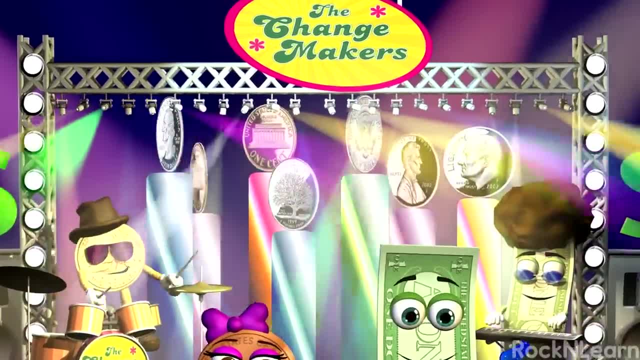